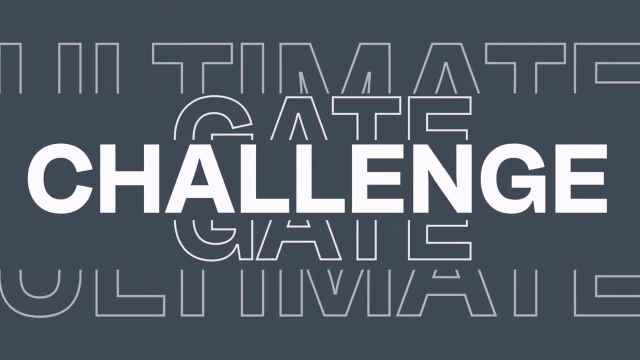 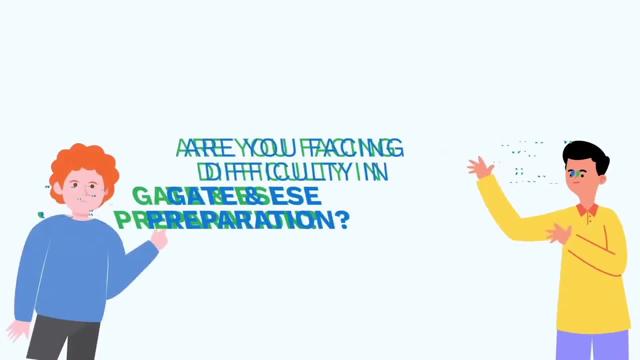 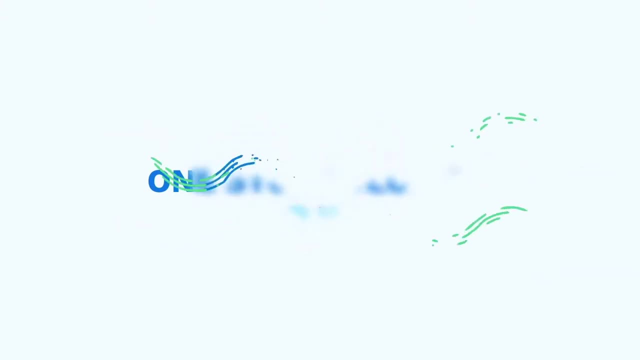 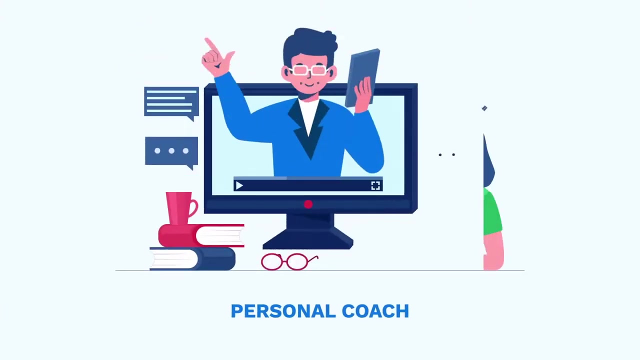 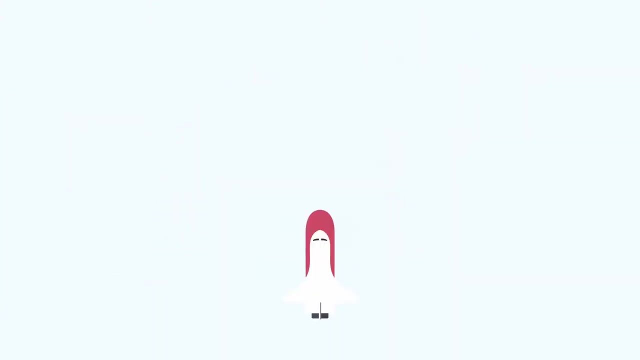 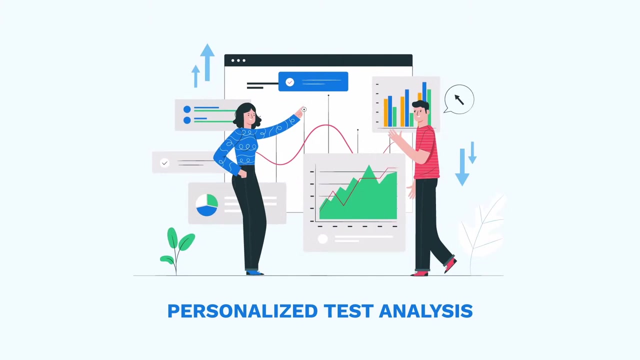 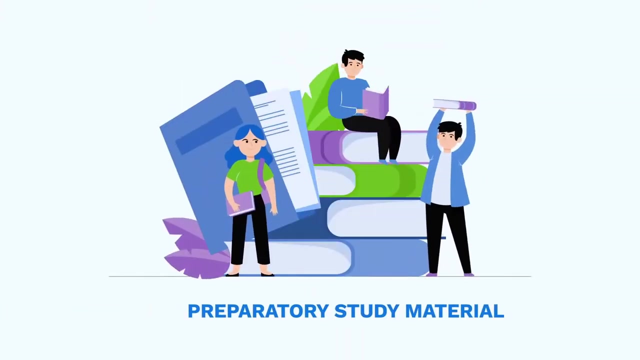 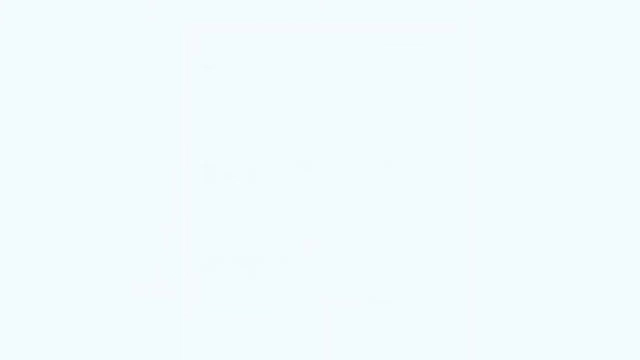 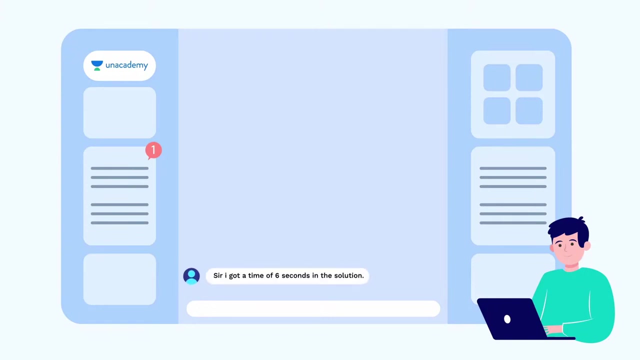 Fuel your inner fire for the ultimate GATE challenge. Unacademy Combat: Register now. Unacademy Combat arts2- crying GATE Team. Unacademy Combat: dade. Unacademy Combat: The kraft, same Greek, The Unacademy Combat. 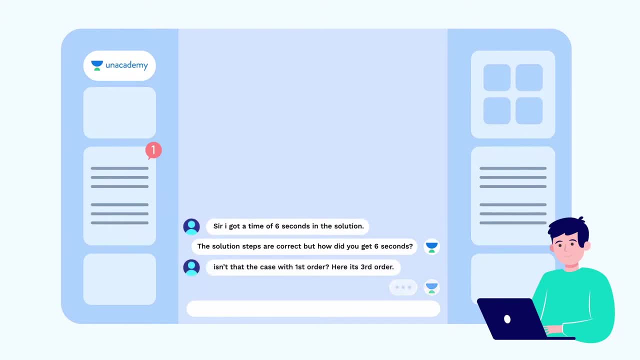 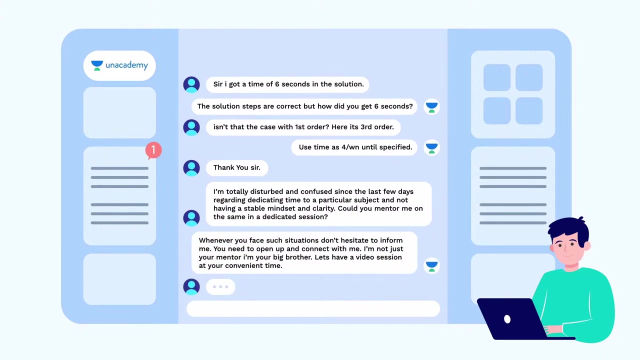 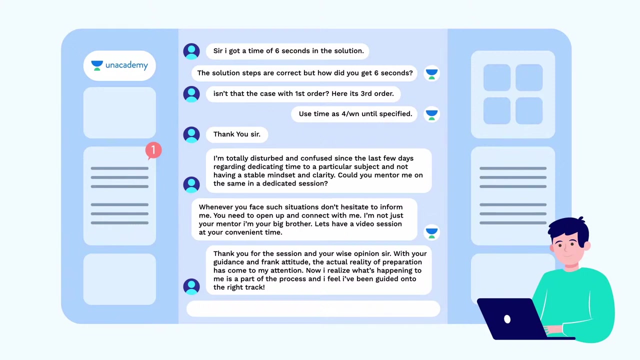 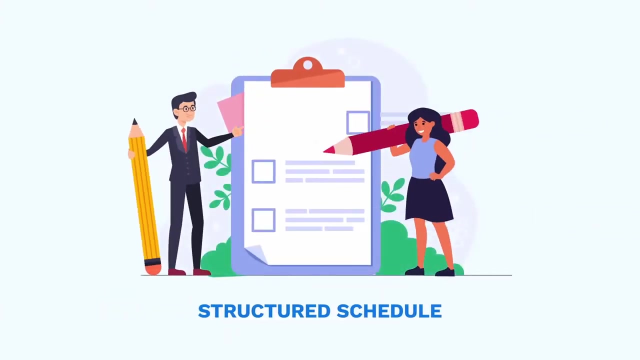 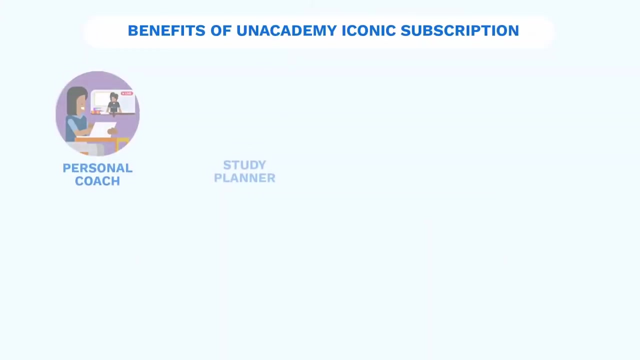 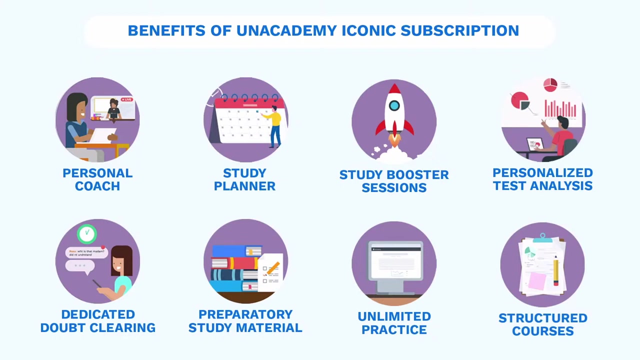 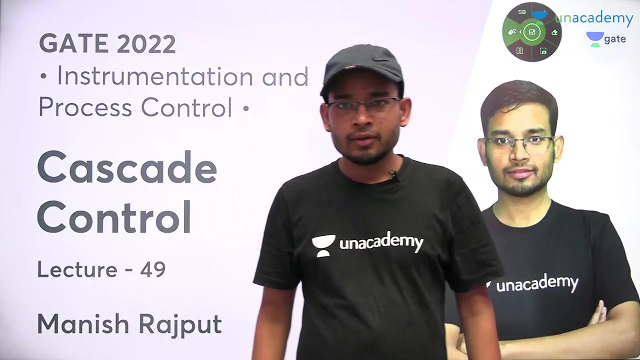 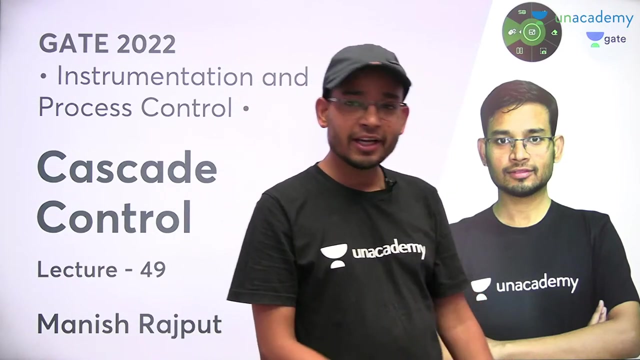 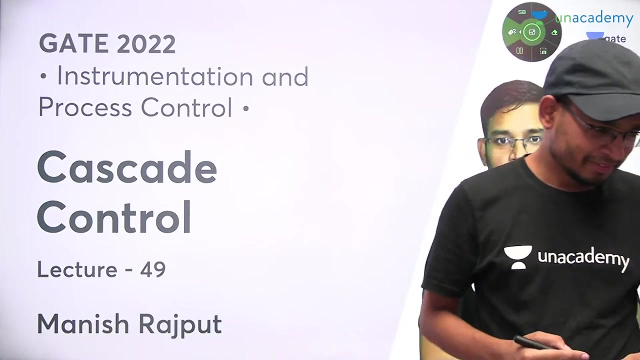 GATE Games. Thank you, Thank you. Good afternoon to all of you. Good afternoon. One thing: everyone will clear me: that audio and video are clear. Audio and video are clear. Yes, Yes, yes, Yes. good afternoon, Good afternoon to everyone. 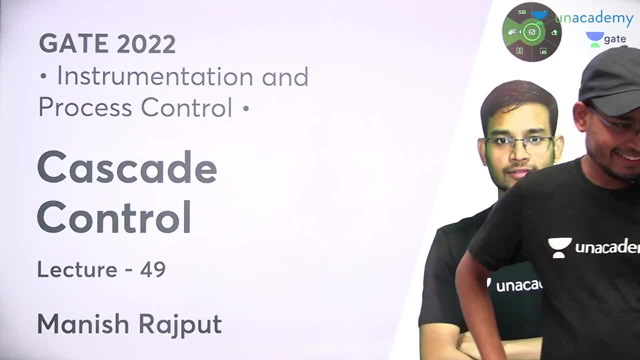 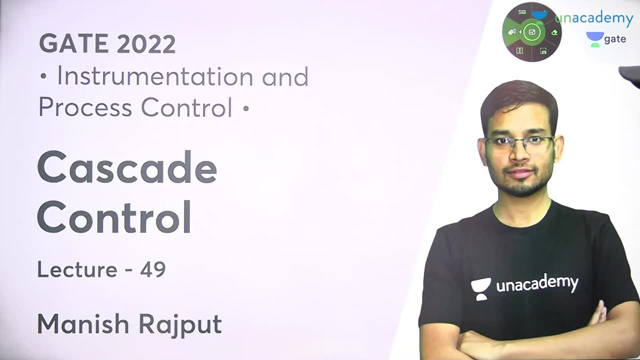 Good afternoon to all. All clear, All clear. Yes, All clear, Clear, clear, clear, Perfect. So today we will talk about here, we will talk about cascade controlling. This is like. I have already updated you, Okay. 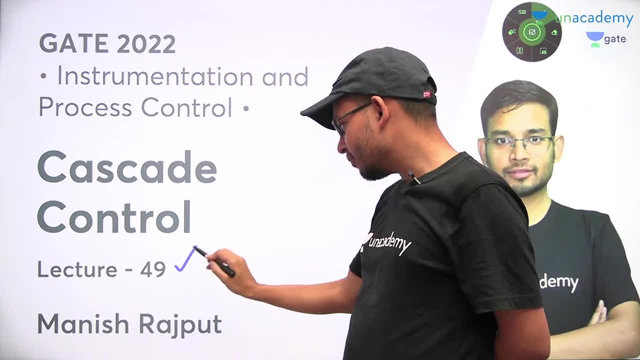 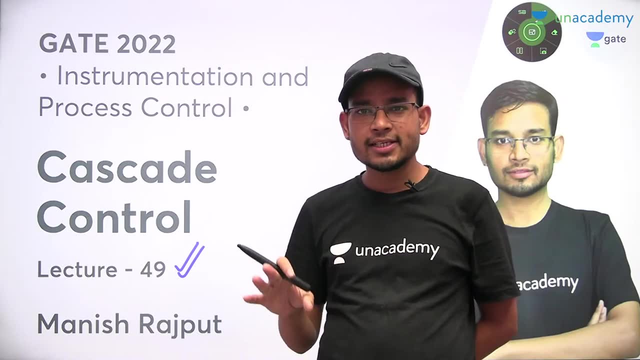 Today will be your last lecture of IPC. Okay, That is the lecture number 49.. You have done almost 49 lectures. You have done theoretical lectures, You have done numerical sessions on the app. Okay, So 49, you have done almost 20 sessions on the app. 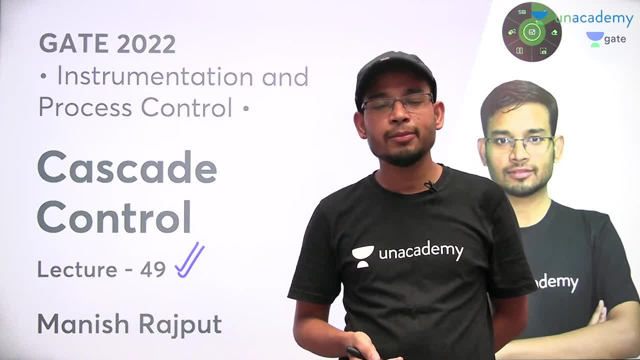 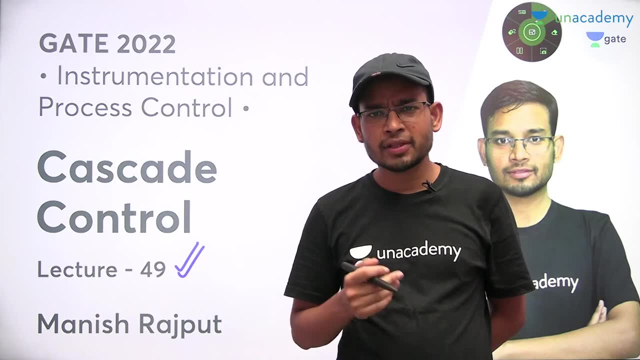 So around 70 sessions you have completed, And if I talk about completing the hour, then you have completed IPC in 120 plus hours And I have completed IPC in 120 plus hours. So I have tried to tell you properly. 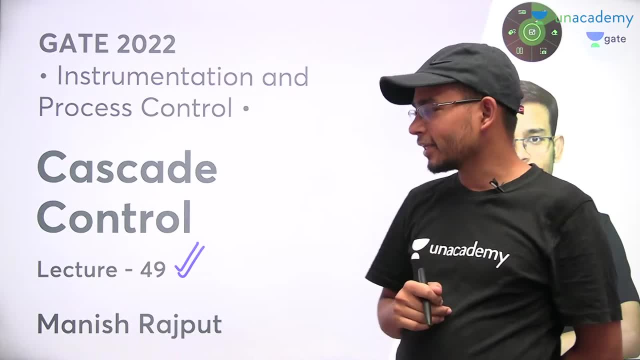 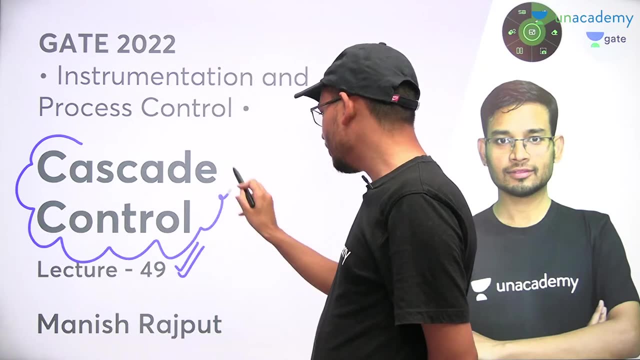 And today first we will complete this last lecture properly, Then we will talk about it. Okay, So today we have one last topic- Sometimes there is a question on it- Cascade control. Understand it a little properly, Because there is a lot of confusion of children. 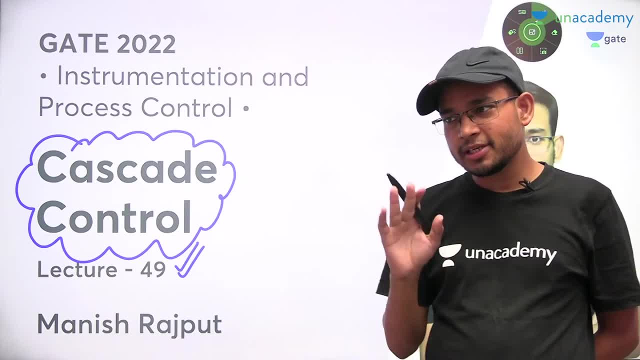 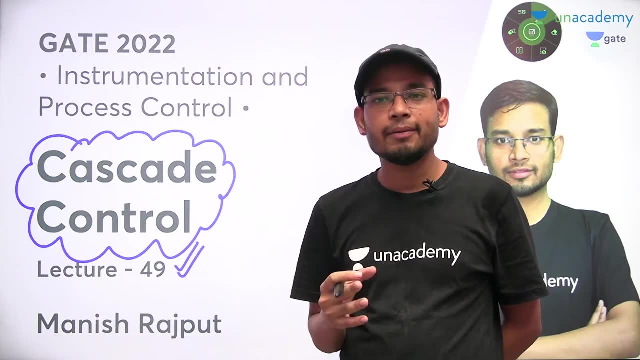 Actually the last two or three topics. I told them in detail because of this, Because there is a lot of confusion in it. Sir, feet forward control, Okay Jiggle and Nicola scone cue. There is a little issue in them. 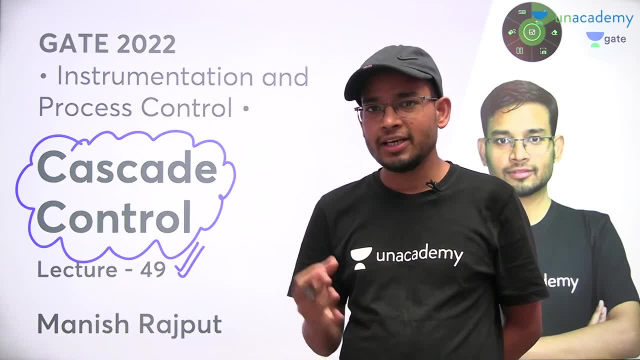 Most of the questions in it means children do not feel so comfortable. So I told them a little bit. So I told them a little bit about these things a little bit properly Today. if you will read Cascade then you will see that it was also in so much detail about Cascade. 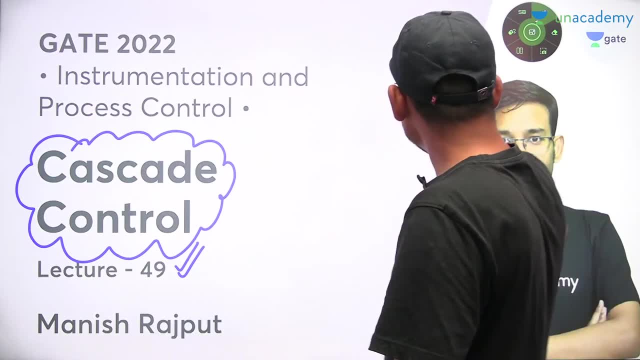 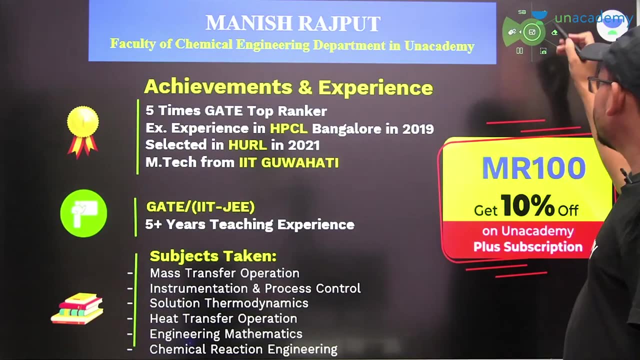 Today, we will talk about it in a very good way. Okay, Come on, So we will just talk from here. We will just talk from here. Who is our new student? Yes, Who is our new student? For them, I will just tell. 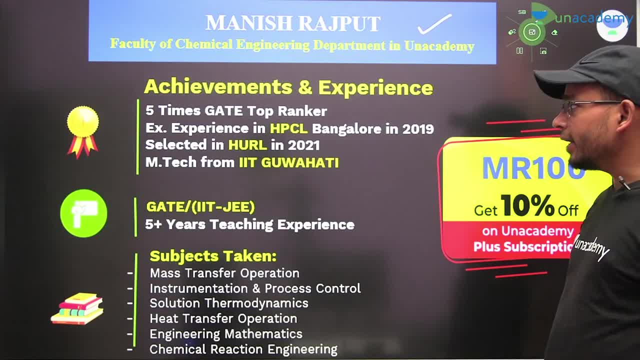 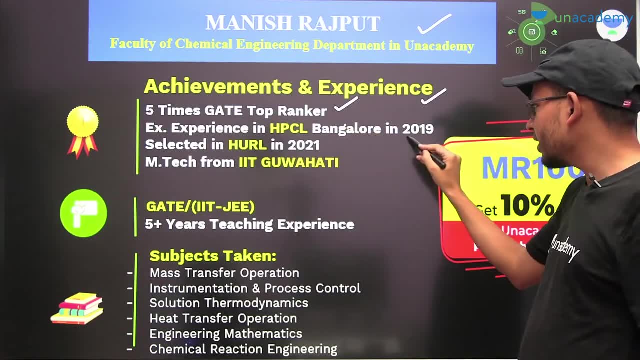 Who is our new student? So about myself, I will tell I am Manish And achievements and experience that I will just talk from here. So five times: get qualified, Okay And X experience in the HPCL Bangalore in 2019.. 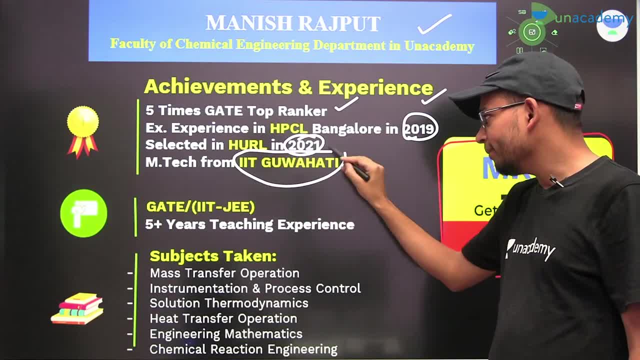 Projected in the HUR in 2021.. MTech from IIT Guwahati. Okay, So this is my achievements and teaching experience. If I talk about it, then five plus years of teaching experience in both fields. 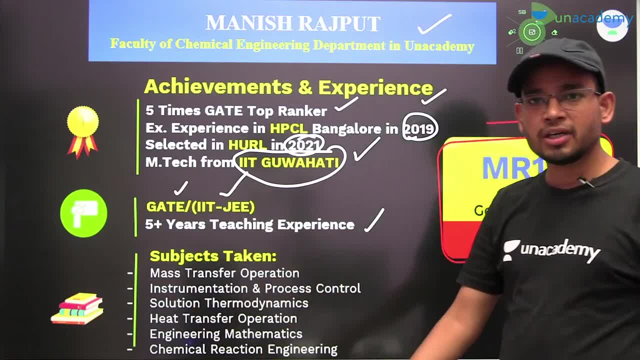 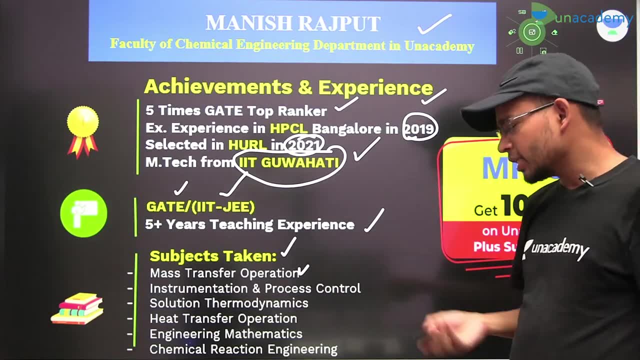 Where I have also taught math to IIT, JWE, And I have taught both offline and online subjects of my chemical engineering. Okay, If we talk about the subject from here, then you must have studied mass transfer from us. Okay, Almost all the children of India must have seen the name. 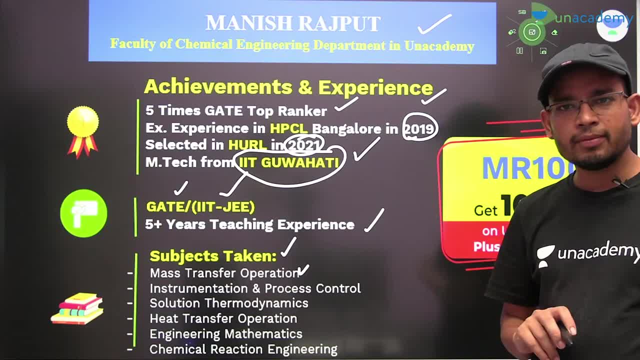 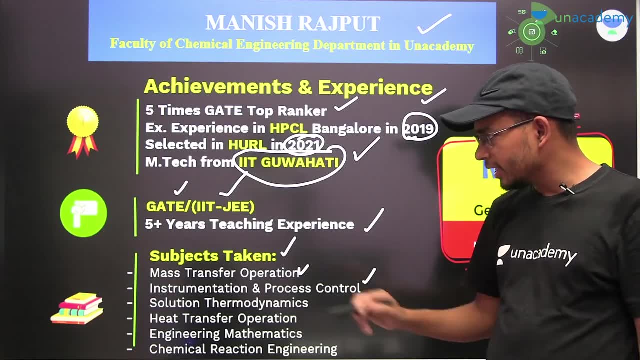 And you have studied this subject. So even IIT students also get queries like Sir. I mean I am feeling good, Good And your instrumentation and process control is going on, which is the last lecture. today I have studied solution thermodynamics by a lot of people. 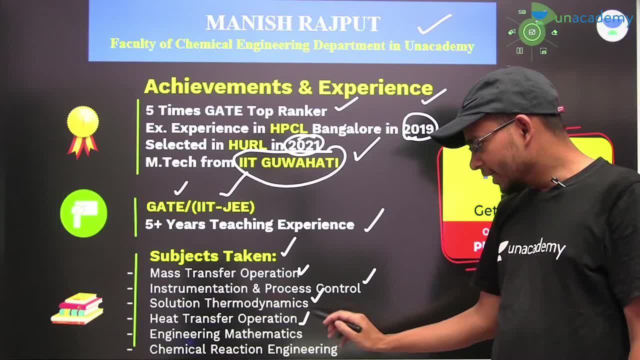 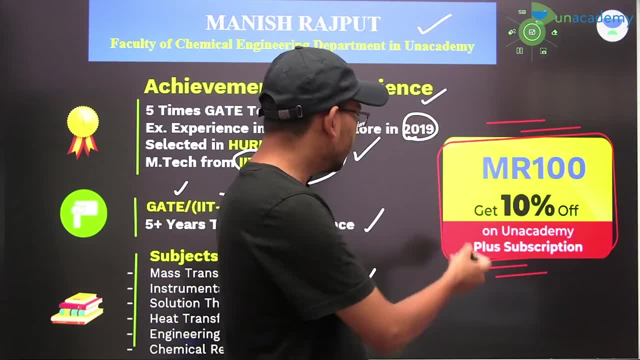 I have not studied it in this session yet. Okay, You can get it. Heat transfer engineering, mathematics and chemical reaction engineering: You can get to see all these subjects in the coming time. Okay, And this is the my code, You can use this code. duration of the joining the plus course. 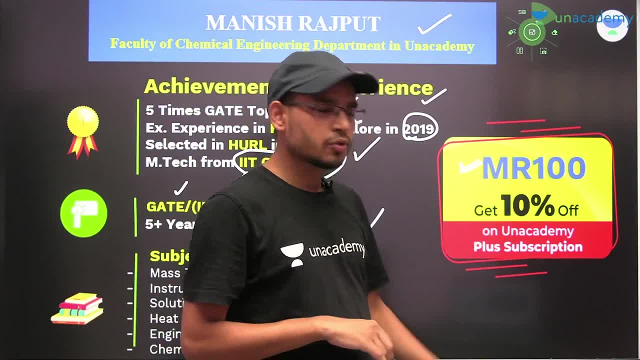 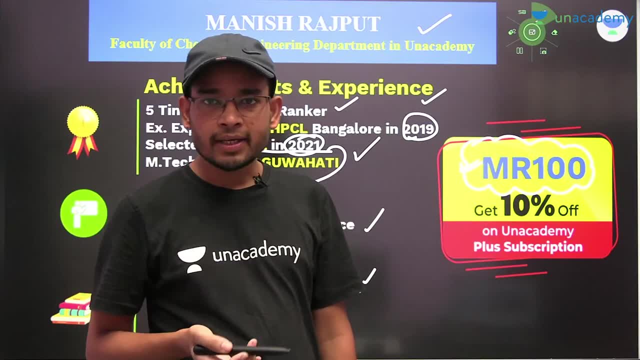 You have to move with us and work under our guidance So you can move with this code. Okay, You can get this code. It will give you a 10% discount. It will also give you planning throughout How you have to move and what planning you have to keep throughout the journey. 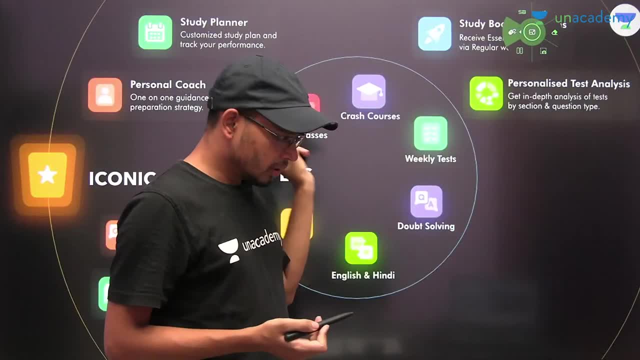 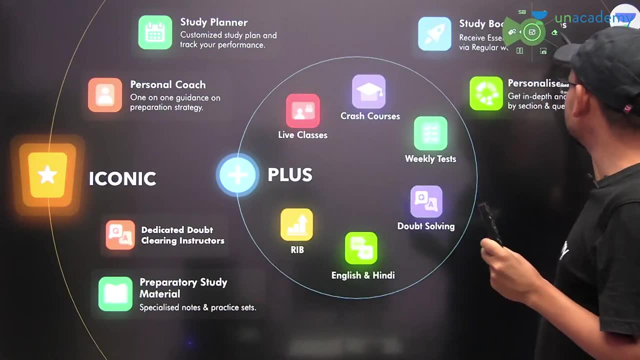 Okay, Okay, After this let me talk In case you join plus- Iconic join- then what features do we provide, And if you join plus, then what features do you get in it? I'll just tell you here, In case you join plus. 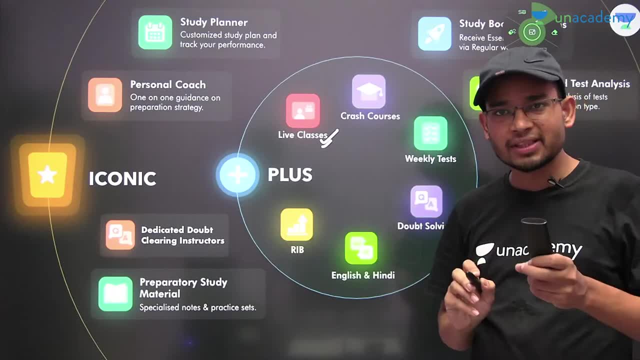 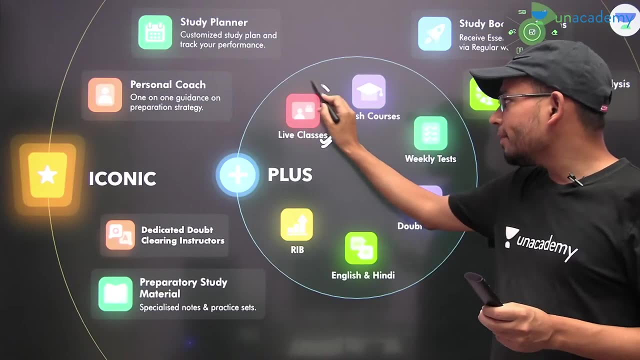 then obviously, you will get the live classes of all the subjects properly, with full content. Okay, You will get the full content properly And the important thing is that your subject will be finished within the time. Okay, Your mass transfer is going on in the current 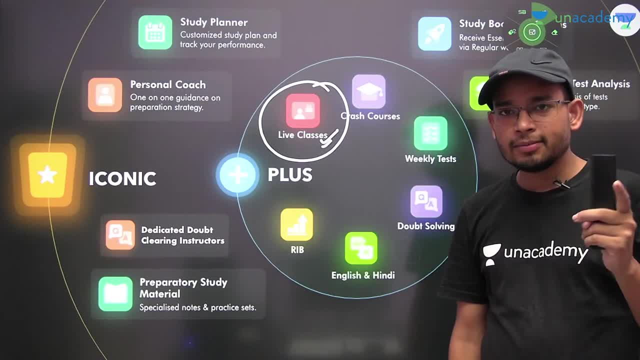 And you see I have reached the distillation. Okay, There are two lectures in distillation. I just have to talk about the boiling point diagram. Today we will talk about the boiling point diagram again. We are talking in so much detail. 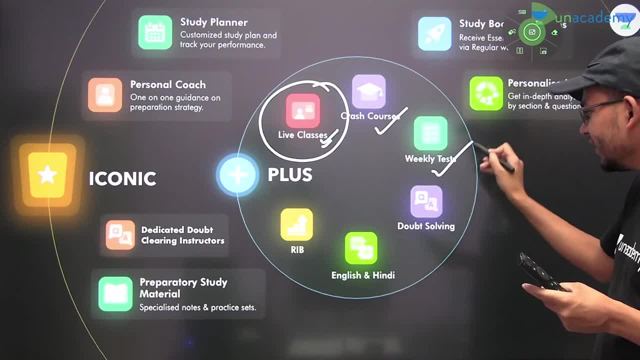 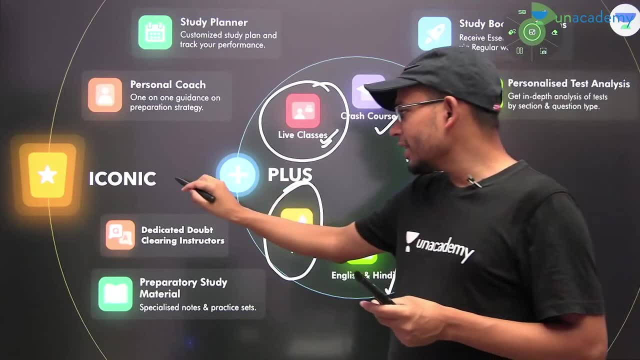 Okay, And there your subject gets finished properly. Crash course, weekly test, doubt solving session: in English: both are provided in the medium. Okay, Ramp improvement batches are also provided to you. in the last I will just talk about Iconic. 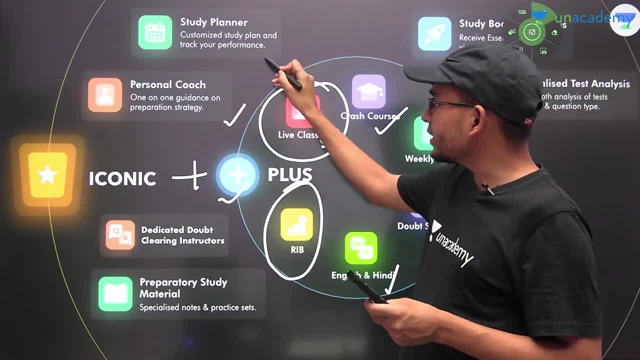 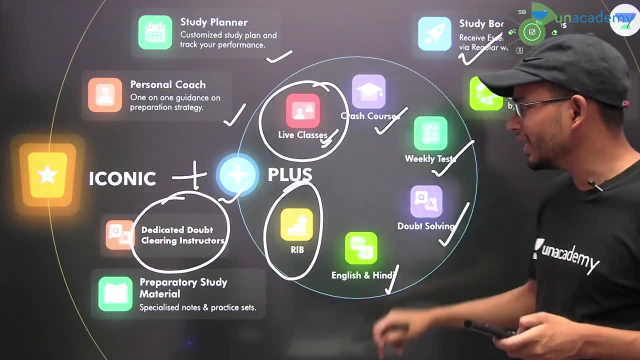 So you will get the full part of the plus. Along with this, you will get personal coach, study planner, study booster session, personal test and dedicated doubt clearing instructors are also provided to you here Right After this. I will just talk. 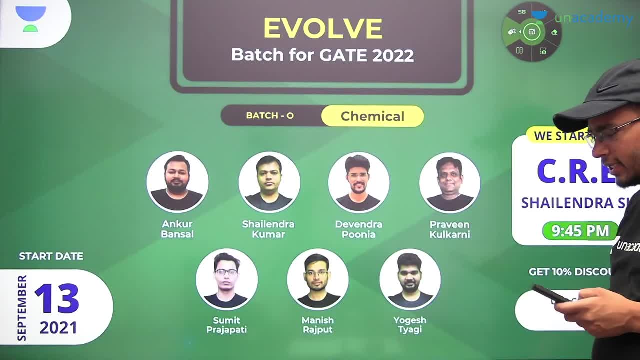 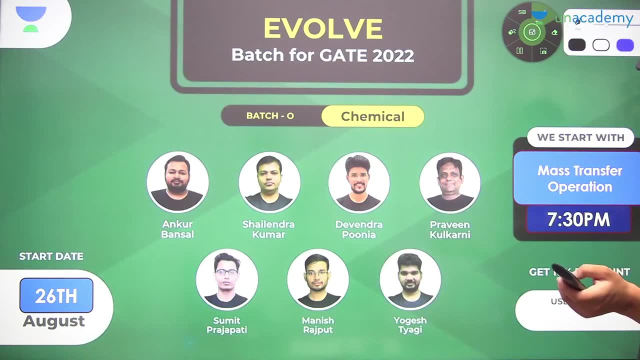 This is the new batch. Now Silencer has started CRE, So those who have not studied yet, they can watch. Okay, And now mass transfer is also going on in current, So I am teaching mass transfer for the first time. 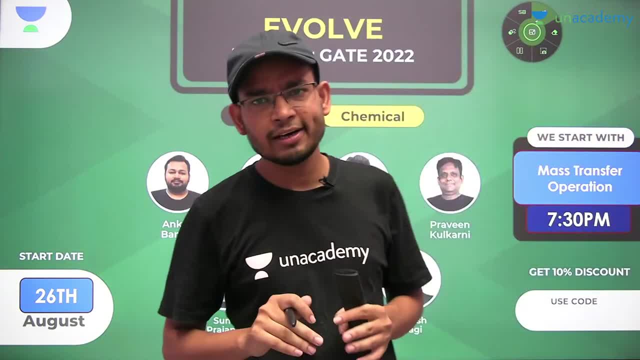 So you can enjoy it properly. Mass transfer is going on for you guys. I am teaching this for the first time. Okay, On plus. So the mass transfer that is going on on plus. its timing is 7.30 pm. 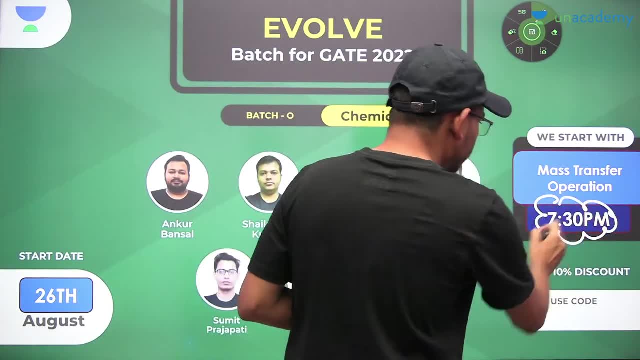 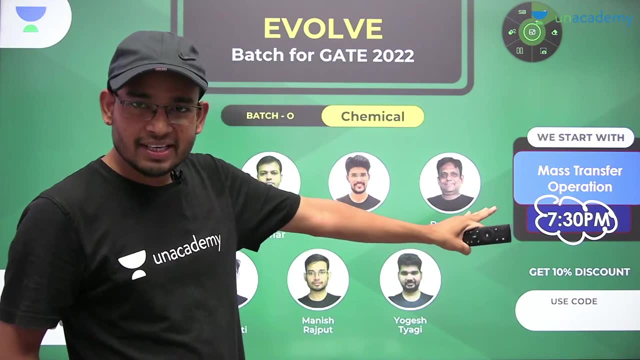 Okay, 7.30 pm. Earlier in your initial lecture I had taught at 8.30 pm. Then you guys did the timing a little early So that it is easy for all of you. You have to study mass transfer, leaving IPL properly. 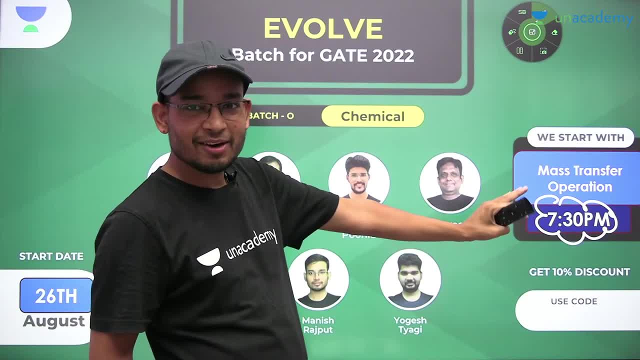 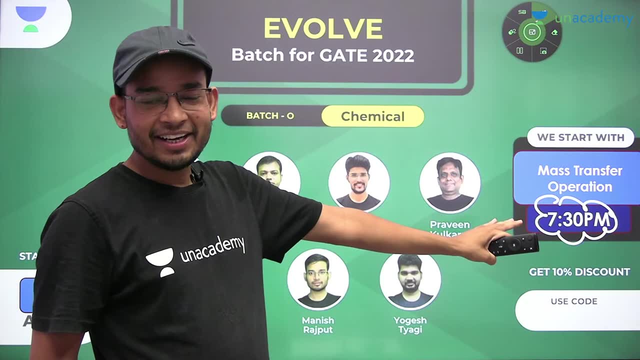 See, It is not like that. IPL has also started SR and mass transfer. Both things cannot be done at the same time. IPL will come every time, But gate will not come every time. for you, Okay, It is not like that. for you guys, that gate will be given for 10 years. 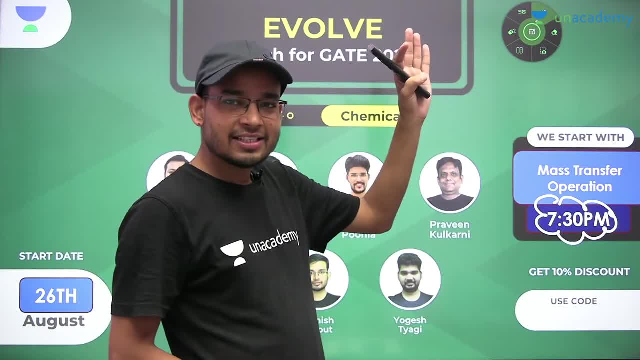 Till then it is going on 2000.. Okay, It is going on from 7.00 to 8.00 pm, So it is going on, But you don't have so many chances, Okay, So you guys will use code MR100.. 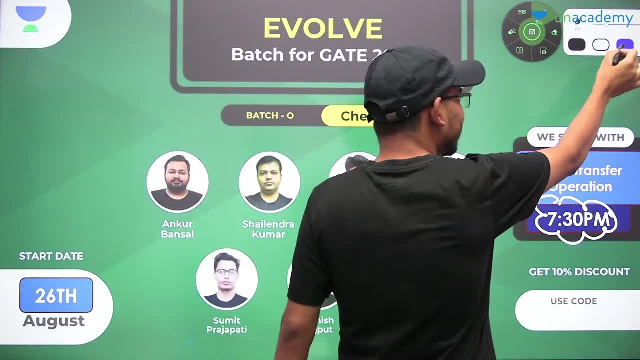 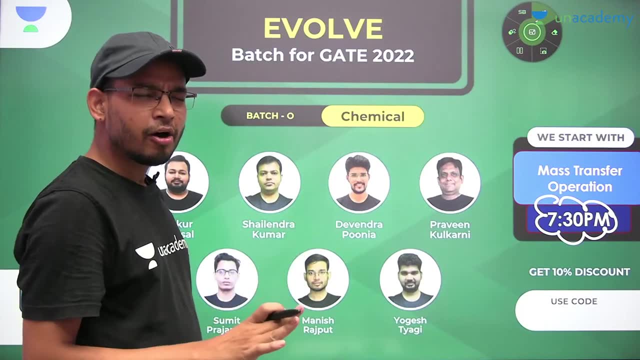 Don't be in the cycle of IPL. Okay, Yes, Read it. Then install a big TV at home. Okay, Install a big screen like this. Okay, Yesterday I was looking at this. Okay, So install a big TV at home. 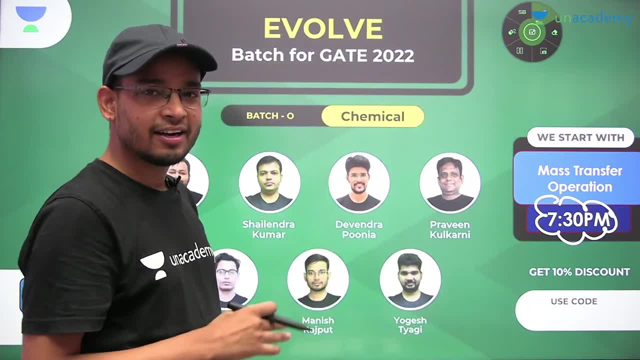 And make the environment properly. First you guys achieve what you want. Then only you have to do this. Okay, Right, First do MTech and come Or take selection in Qualify or PSU somewhere. Okay, Then only you will like it. 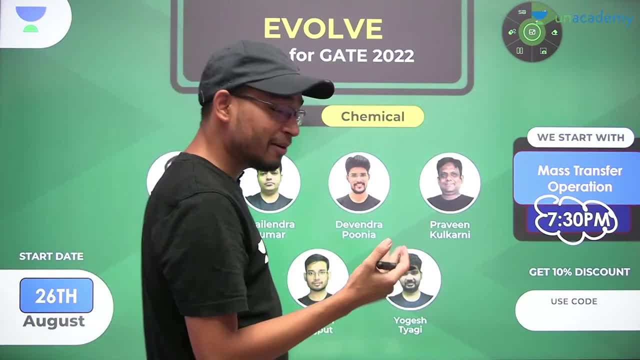 Otherwise you won't like it. Okay, I was a student, So I don't watch it. Yesterday I was watching it comfortably Because now I think that, okay, I have to study my profession. It is going on well. 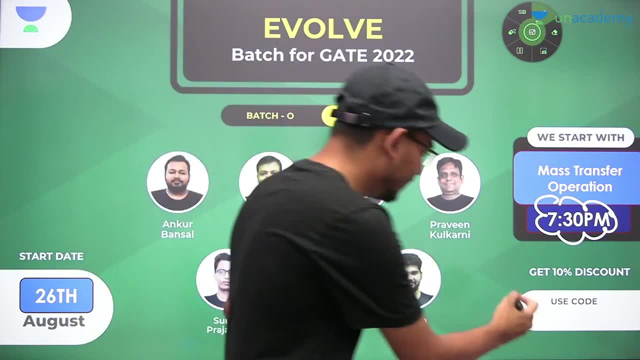 You can enjoy it. Okay, That is a different thing. I came to know You are leaving the session at the current time. You are watching it with fun. Then there will be a problem. Okay, Yes, I have not left it everywhere. 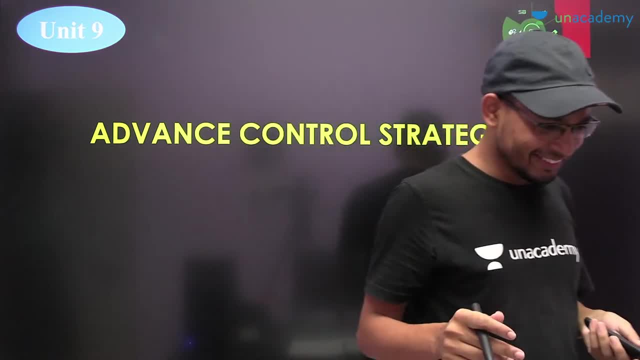 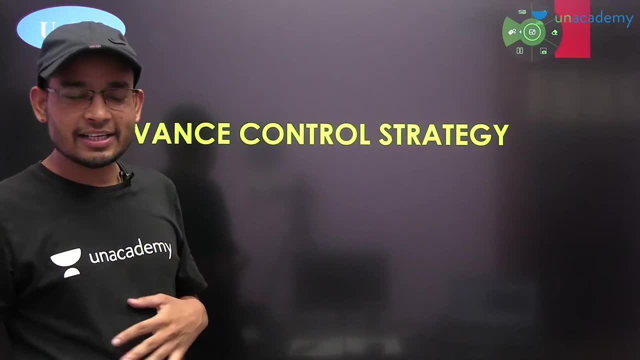 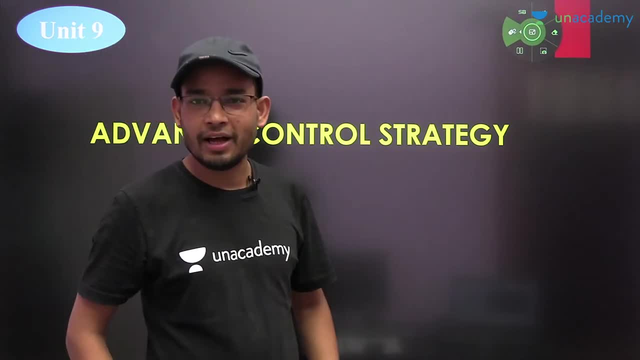 Yes, Yes, You will change the context in your own country. Yes, Sinceelaizin will remain the captain of S blade After this session And the other T20 just left it. Okay, And it is right. Cheers and test Okay. 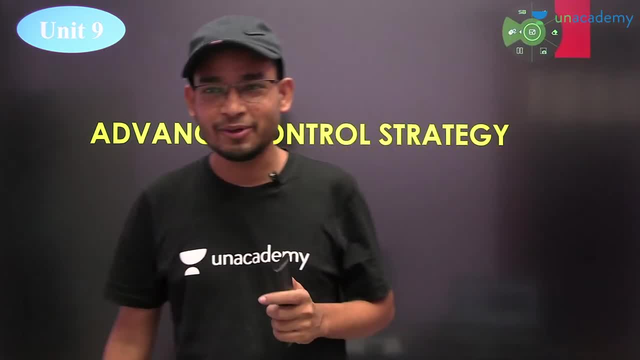 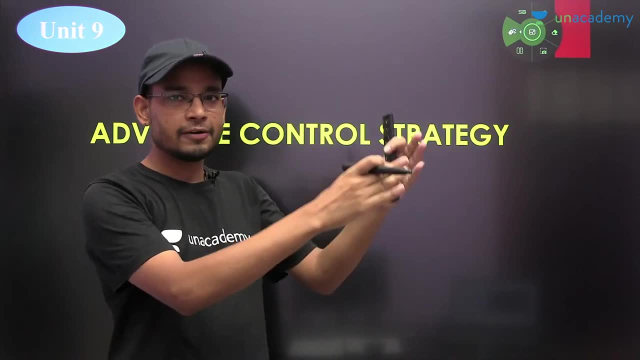 There is time, There is the time of each thing. Look, Okay, There is one time zone for every everyone. Okay, Does that time come from every single person? Pickpoint comes, Then continuously pick. time is over, Then we handendover the other things. 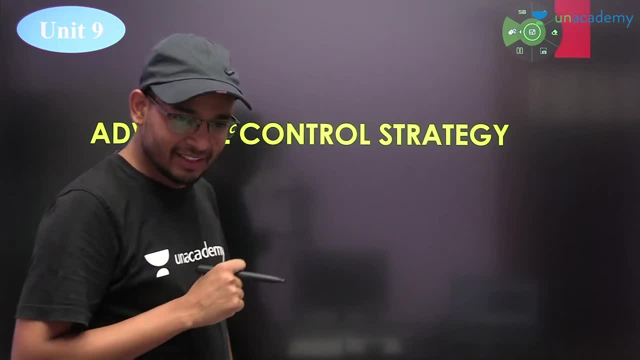 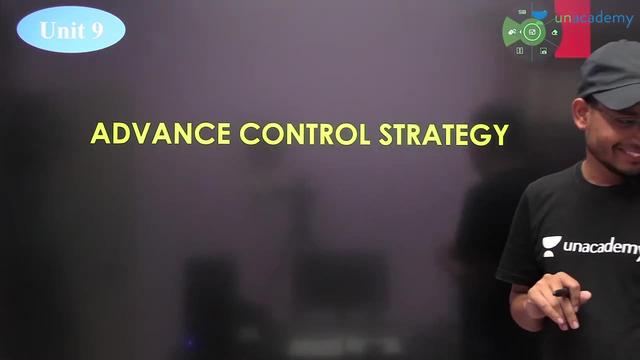 Then this is what happens. This is the process. This is the process. There is no need to be so touchy in it. Yes, Subham, Good, You didn't go to the job today. You didn't go to the job today. 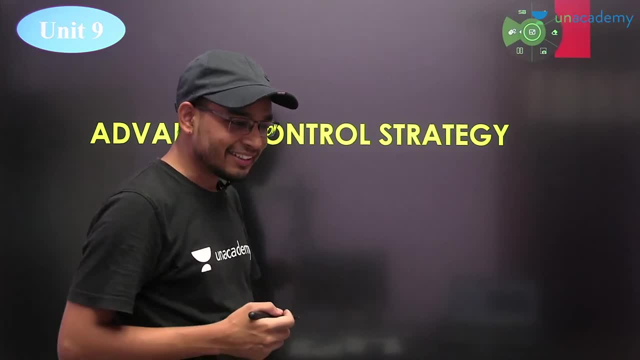 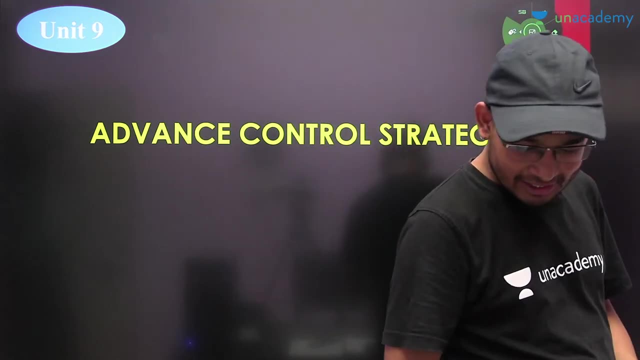 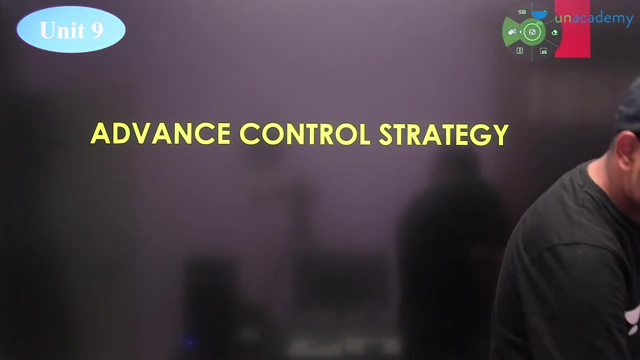 You were saying yesterday that we will go to the job. That's why we are not able to do live. Sir, my question. I will read it now. What is your question? I am just taking your question. To calculate the amplitude ratio of phi. 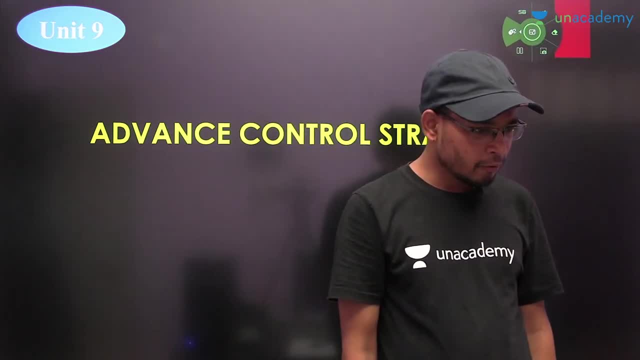 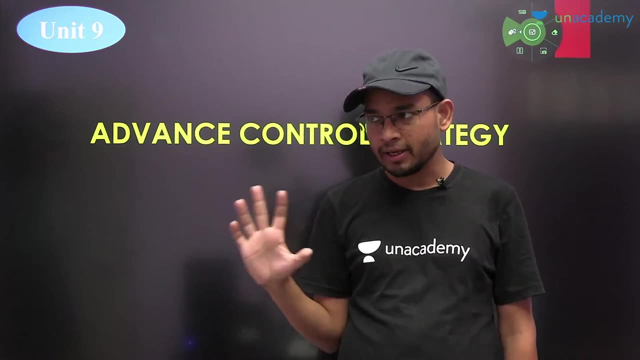 we don't have to find the transfer function of the loop, We have to find the transfer function of the open loop. What does it mean? The concept of the entire body? it considers the open loop. Who does it consider The open loop? 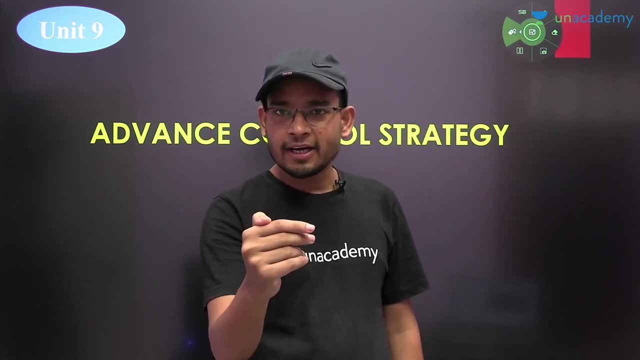 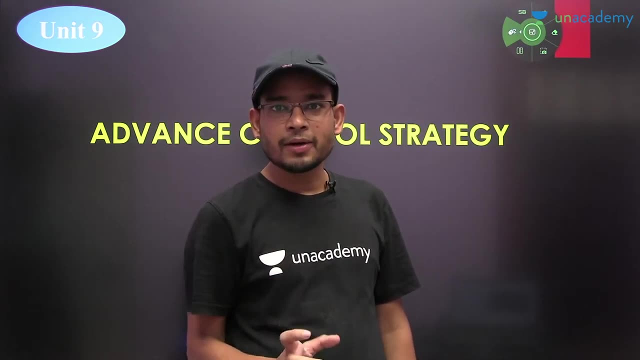 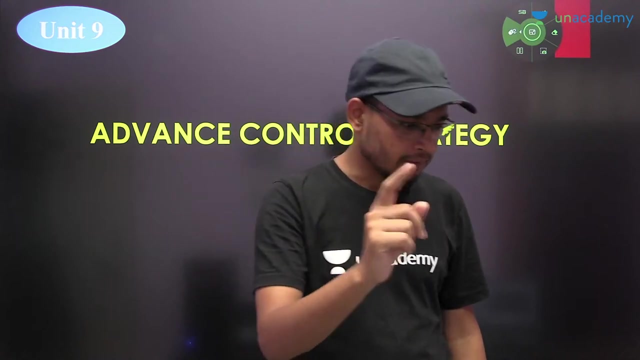 After studying the open loop. what is the stability of the closed loop? Understand this Stability tells us about the closed loop, But the process uses the open loop. Okay, So who has to calculate the amplitude ratio of the open loop? And it will tell us about the closed loop. 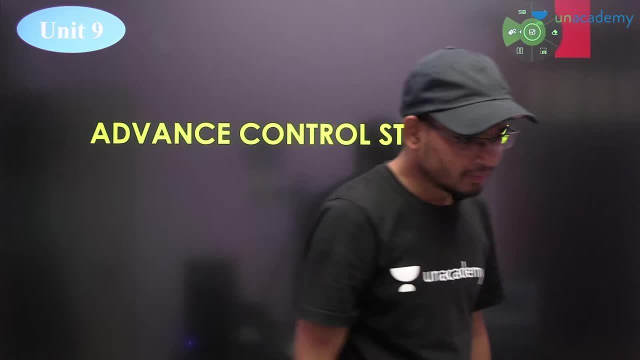 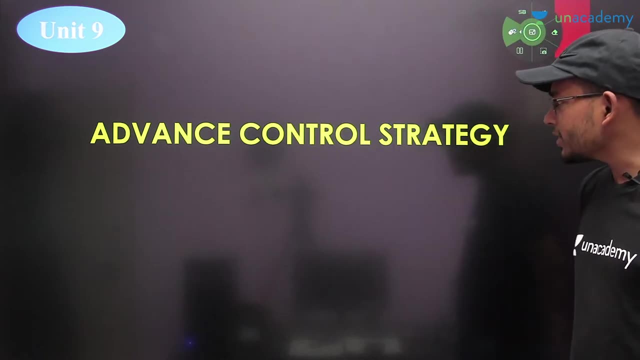 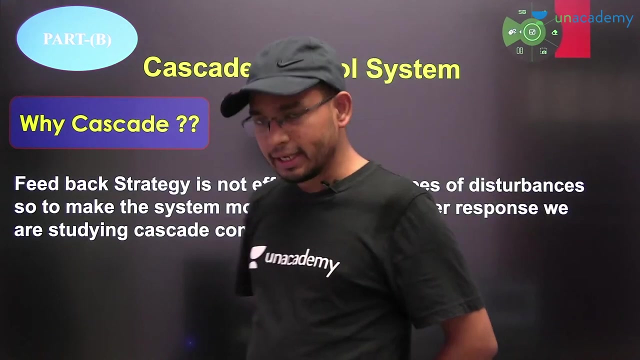 So always take care of this. Come on, Let's start the session. Everyone will write it once. Ready, Ready. Let's start the advanced control strategy, In which we will talk about the cascade control system, Part number B. Everyone will write it once. 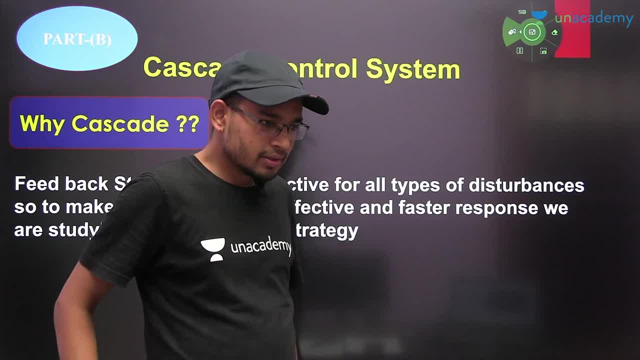 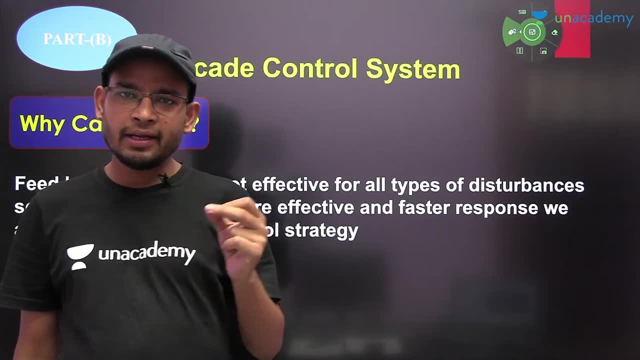 Ready, Let's start. So what is the cascade control? How does the cascade change? Let's start. Okay, Yesterday's session. I hope you all saw it. Yesterday I talked with two students. Both of them are in BARC. 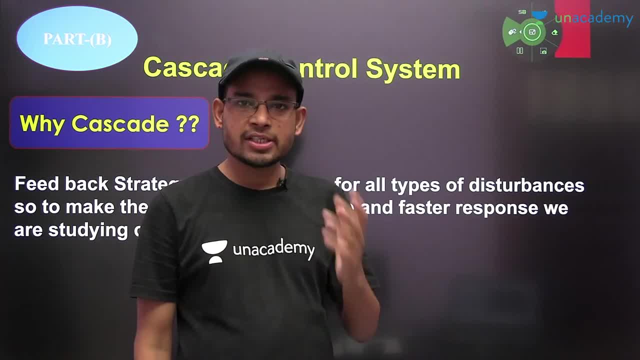 Okay, One is in Hyderabad Posting. One is in Mumbai Posting. You must have enjoyed the session yesterday, Mehek and Risabh. I hope you must have enjoyed it, And you see those who didn't. There is so much of informative video in it. 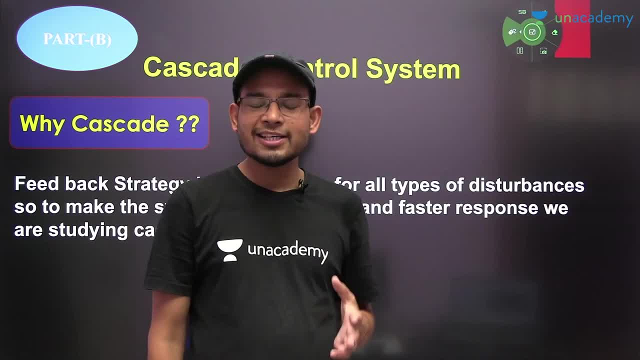 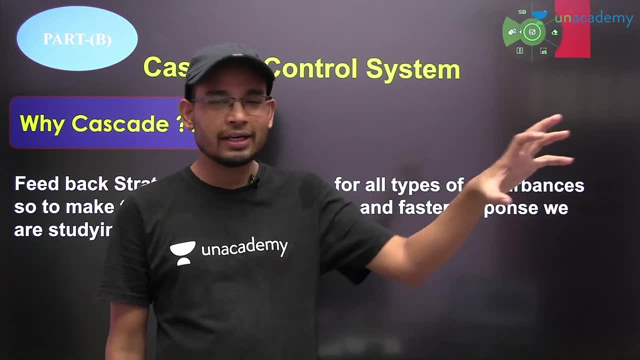 I haven't started on one thing In case. you must have attended the entire session, So you must have seen. I have taken out all the things from their exam and put it out for you. How much salary do you get? although there are many things, it is a clue. it is not told. 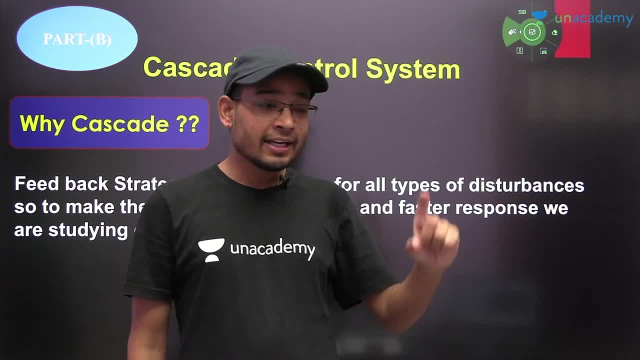 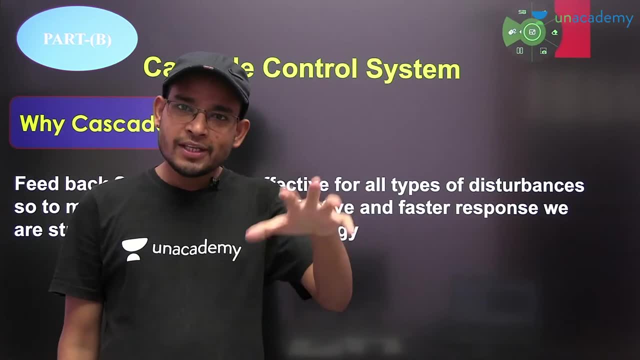 How much salary do you get? What is the time period? What projects are they working on? What is the work duty? What is the use of chemical engineering? Do you have to go to ONGC, PSU or BARC? I have talked about all these things. 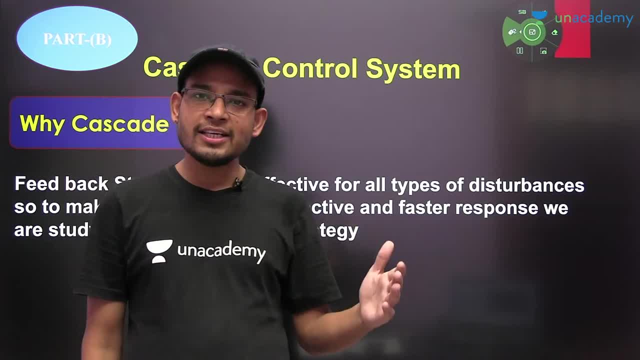 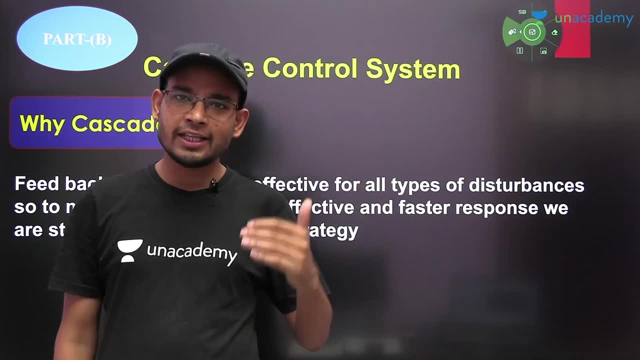 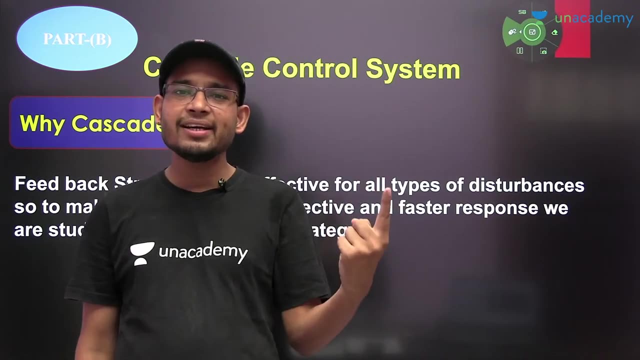 I have talked about A to Z. Who is given priority? Who is given priority? Who is given priority? How are the questions asked in the interview? What is the strategy? in the interview I have covered all the things A to Z. So see that one session, it is a complete session for BARC. 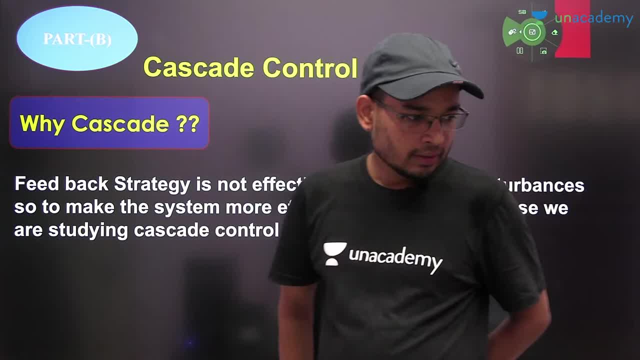 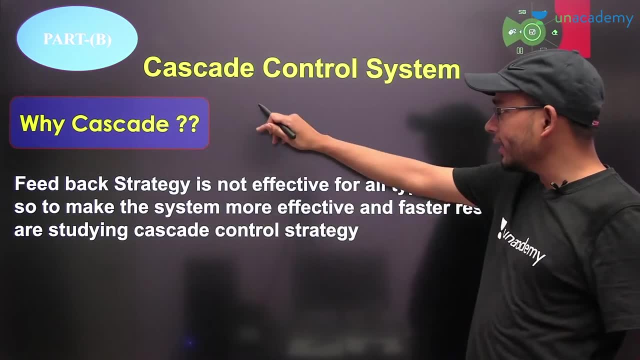 It is a complete session of BARC. They are ready, let's start. So everyone will put the heading New project. We will put the heading from the new page. Part B of the advanced control strategy, that is, the cascade control system. 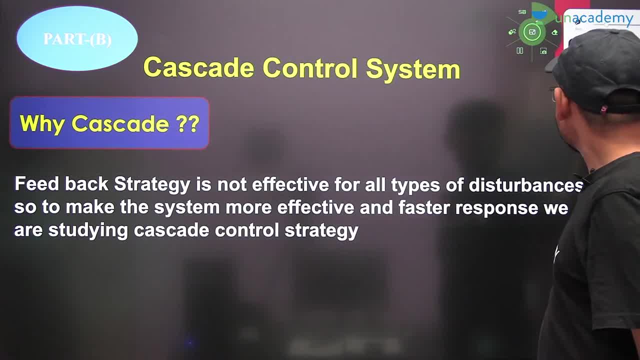 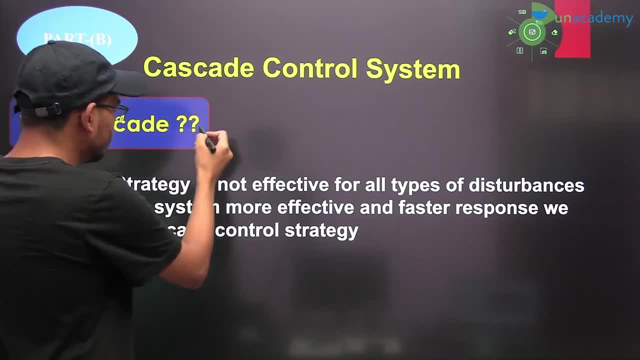 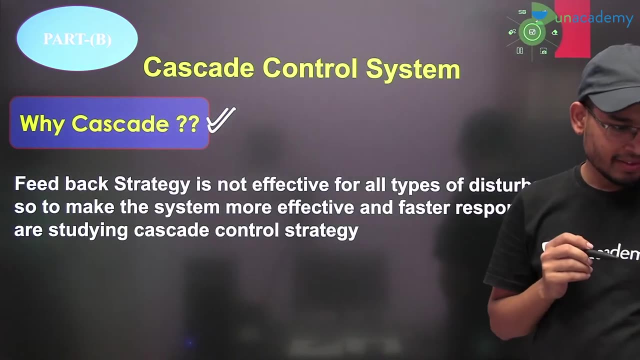 Cascade control system. Everyone will put part number B in their copy: Cascade control system. The most important thing is why we are using the cascading. Why do we do cascading? Why Work is greater- greater than ONGC? Yes, 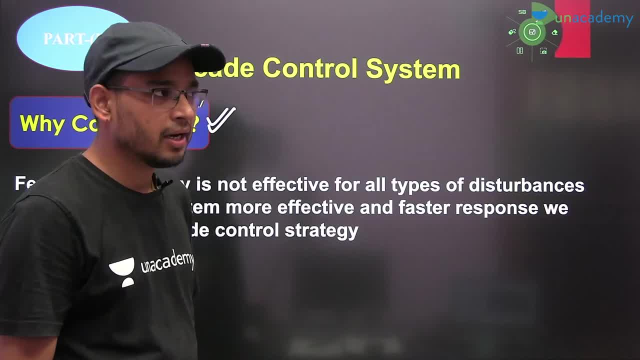 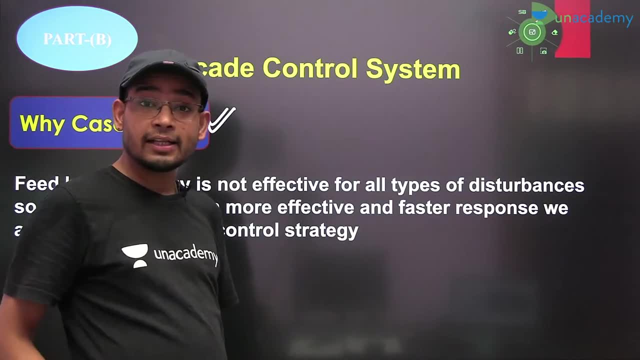 At least you can use your brain. Use your brain in the BARC, But you will not be able to use that much in ONGC. Okay, What you have read, As Rishabh was telling you yesterday That he is also designing a project. 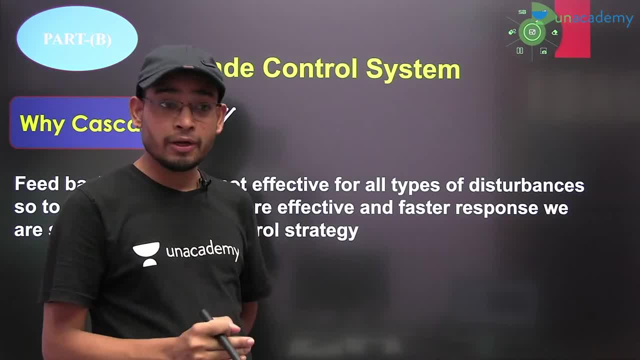 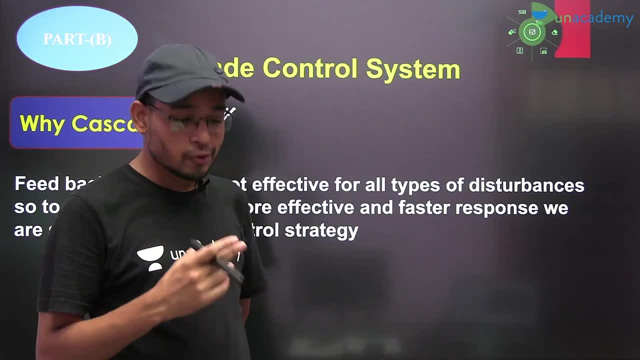 He is designing a reactor of self. Okay, And his supporters have supported him very well. You will see in the next session. He said that if you go to PSU you will not be able to think of anything. You will have to modify the things that are running there. 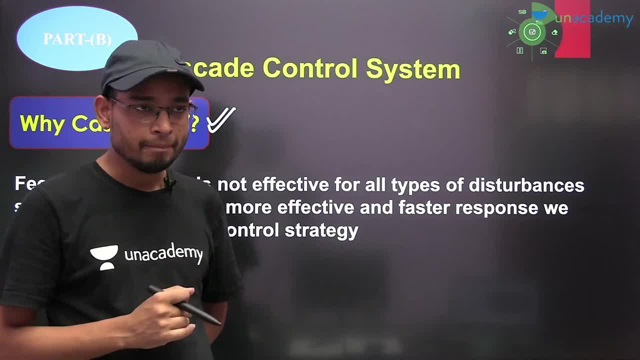 If you want to do something new, you will not be able to do it, But this is allowed in BARC, Okay. So if you want to work on a new project, you can do it, Okay. So he told this thing yesterday. 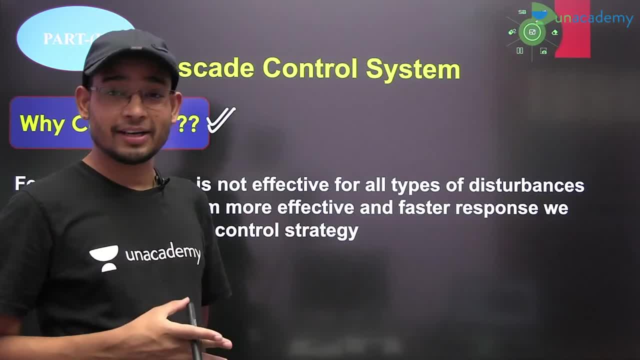 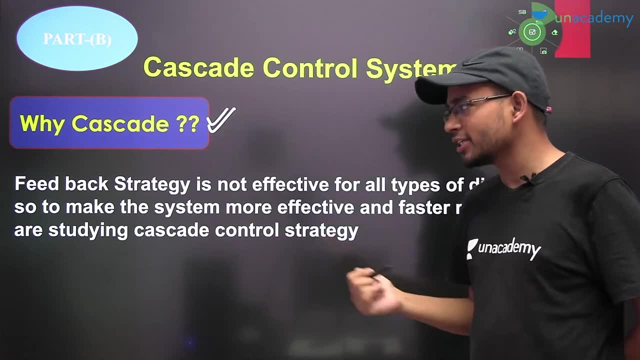 Okay, I am not telling about the BARC. He only told that the BARC is working at the current time. Okay, Come on. Why cascading? Why will we use cascading? You will understand the process. Then you will be able to understand this line very well. 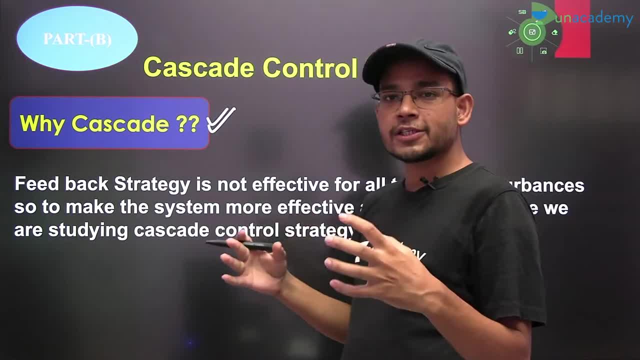 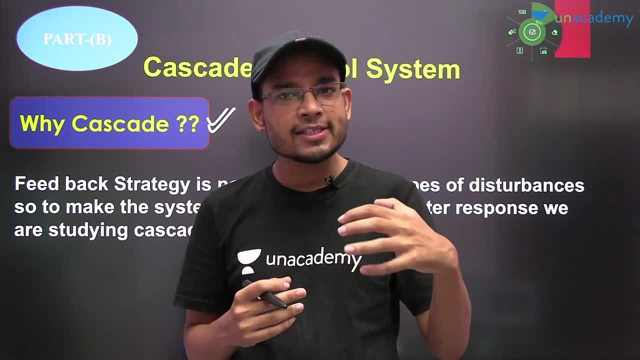 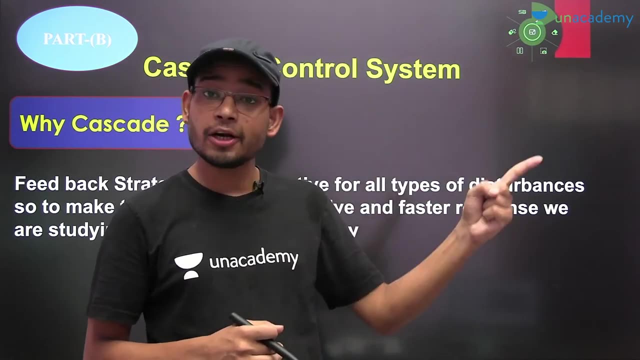 What happens As you were reading now: Feedback control system. Suppose a lot of disturbances start working together in the feedback control system. Okay, Multiple disturbances will start working together. So your controller, The controller, does not work so effectively. Okay, The controller. 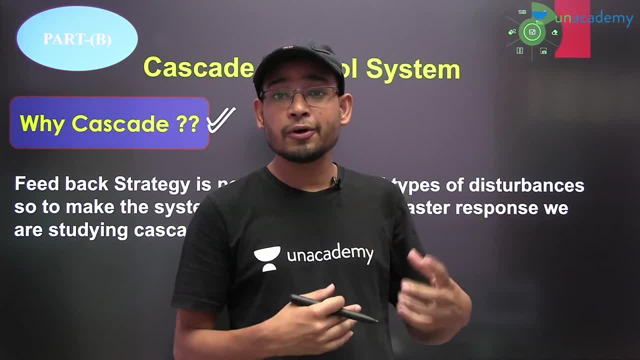 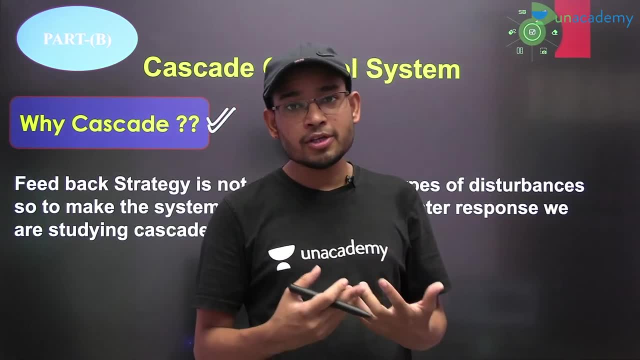 Because there are a lot of disturbances. So it gets confused Who to lead, Okay. So it gets slow. So the same controller works to make it fast. Okay, To make the response of the system fast. we read the advanced controller study. 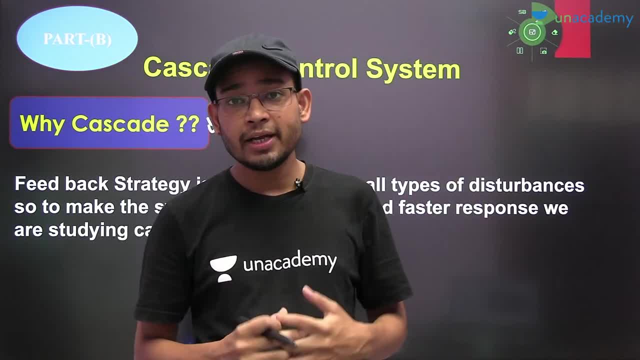 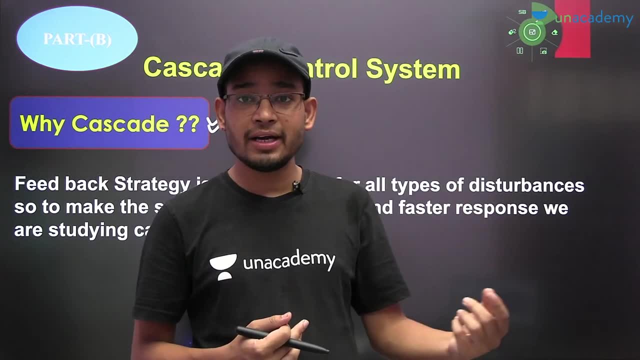 Which has one part. What is your cascading control? Okay, You want the system to respond fast. Okay, The load on one controller remains low. To reduce the load of the controller, To make the system fast. Okay, To make the system more stable. 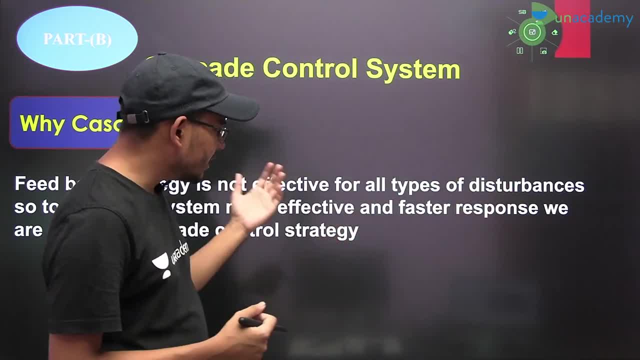 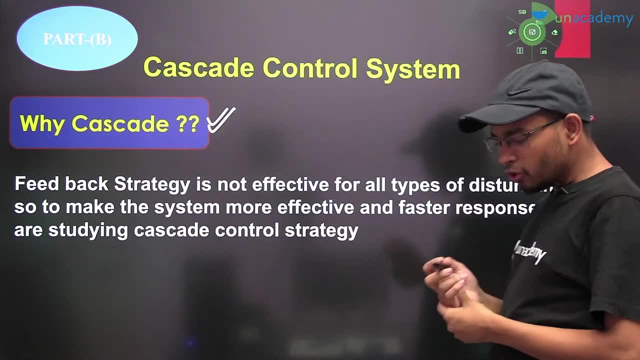 You read What is cascading. Okay, So the definition is written here. You can mention it in your copy properly, All of you quickly, Okay, So what I said It means: Why do we read The feedback system? Then a lot of disturbances. 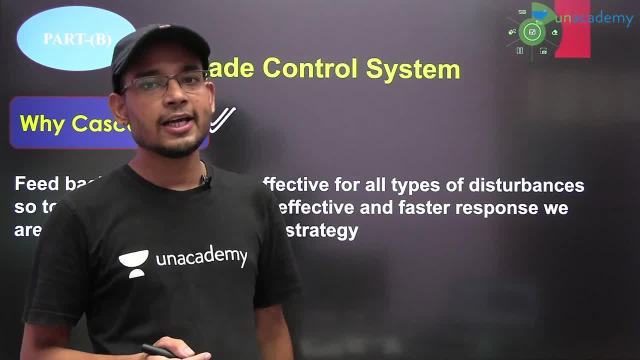 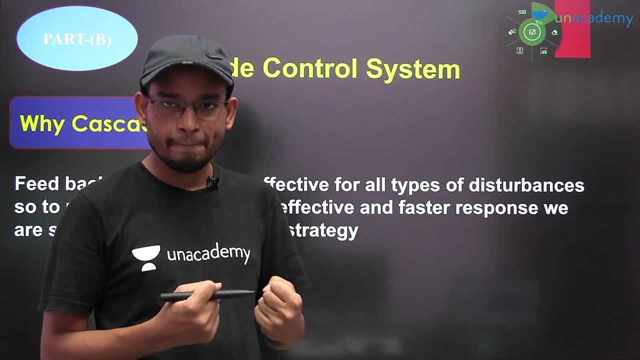 Multiple disturbances occur simultaneously. Okay, Then what do we read? Cascading. What does cascading do? It makes the work of the controller easy, Helps it. Okay, If you can't bear so much workload, Then I also came. Okay. 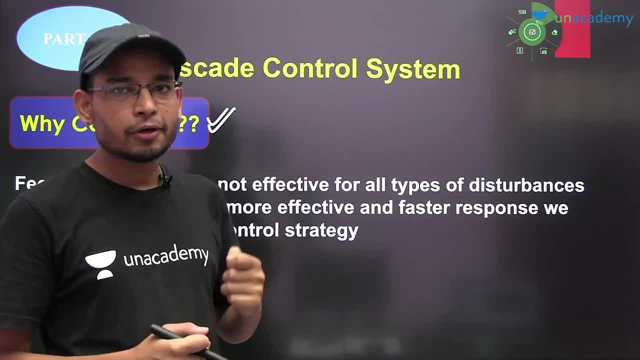 So we put another controller So that The primary controller, Its work becomes something simple, Helps it And the system will start moving fast, Because you will put a lot of work on one. Then there was a controller, So we will put a lot of work on it. 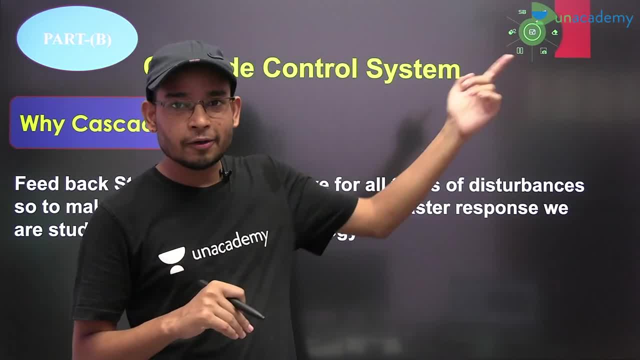 So what will he do, Brother? Work According to you. Come on, brother, Let's finish your work first, Then we will do the second work. Let's finish the work first, Then we will do the second work, But then we put another controller. 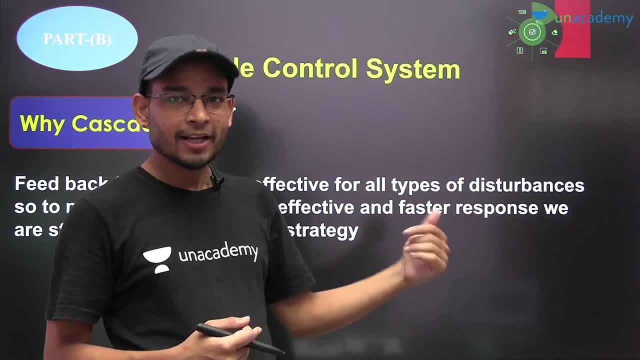 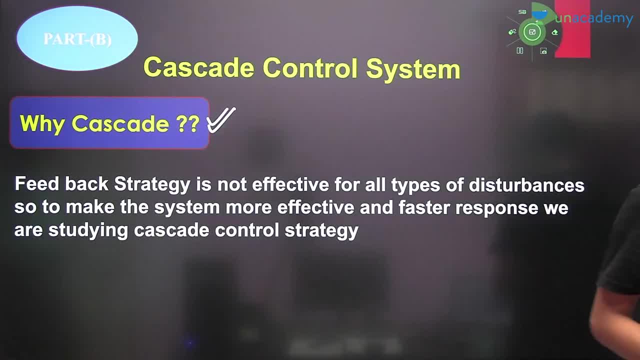 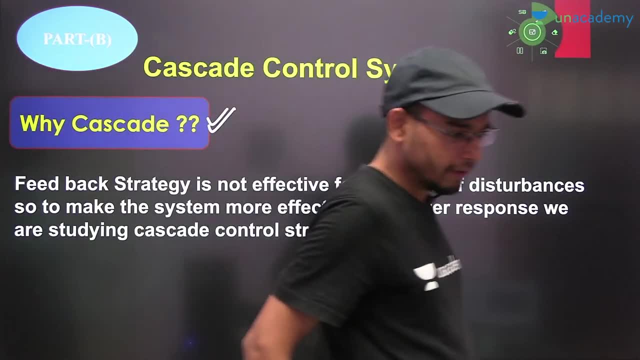 You will see now Write so much. first, All the people. Oh, yes, In this way, my Yes, my classmate is from Mtech M Shubhu. Yes, my classmate is from Mtech M Shubhu, Definitely. 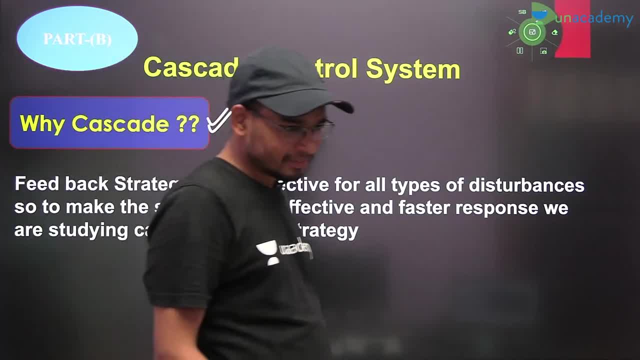 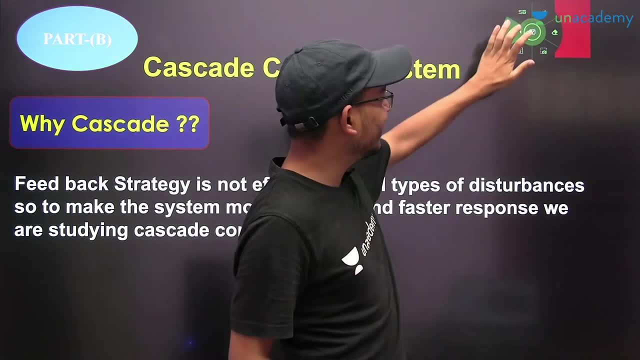 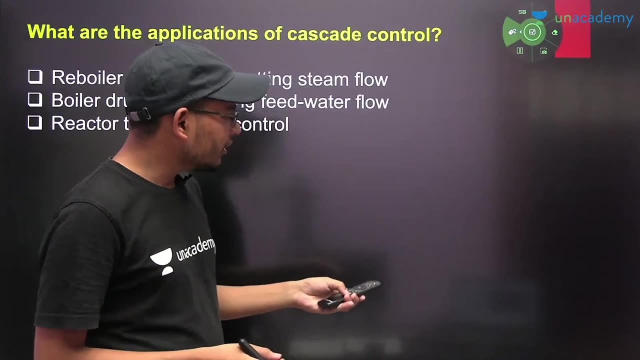 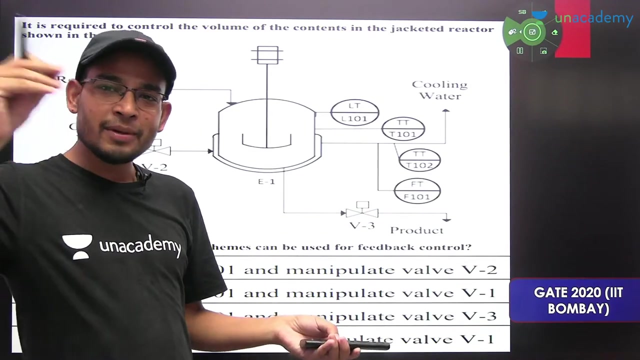 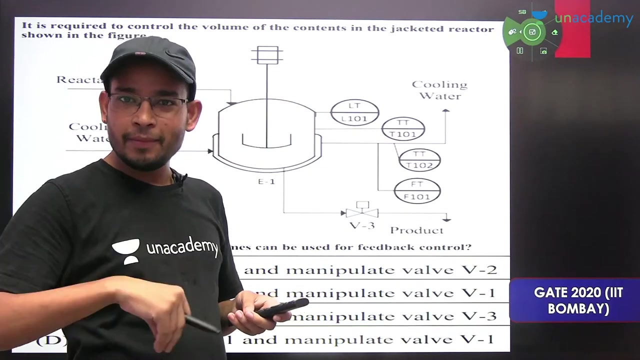 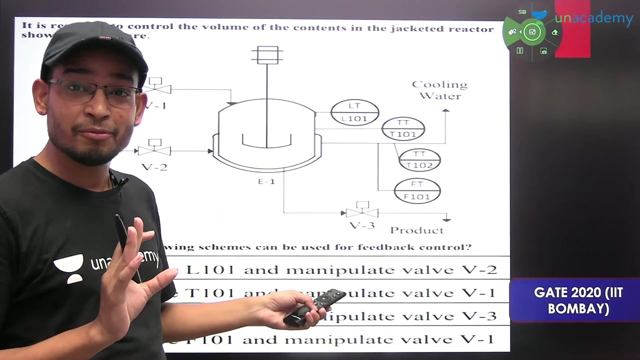 Definitely. Thank you, Yes, Yes, Yes, Yes, 2021, Kunal. Yes, Look, I got a question before you said: Don't worry, just wait for the whole lecture, you will get everything. you are talking about the same question. I brought your questions first, the questions that can come in your mind. I work for an hour before the whole session. I know that this doubt will come in the mind of the student because I am also a student. I am a student in your current state, not much old, so I know that such doubts will come. so see, this is ready from the beginning. one more ready is of 2005,. 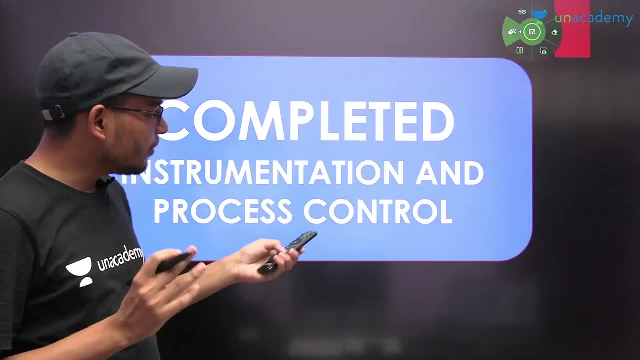 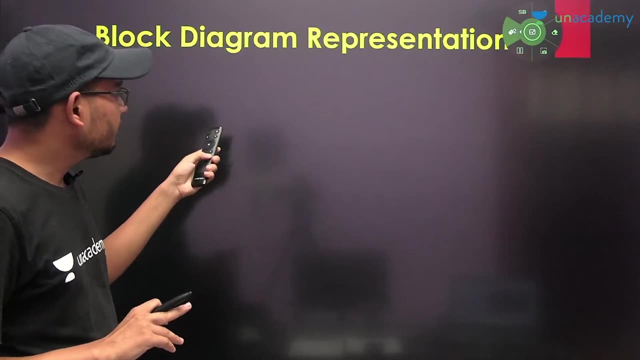 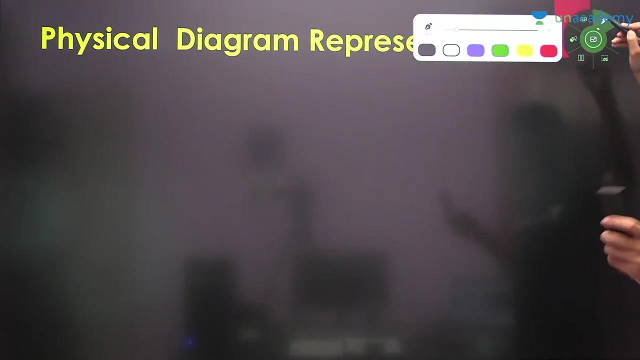 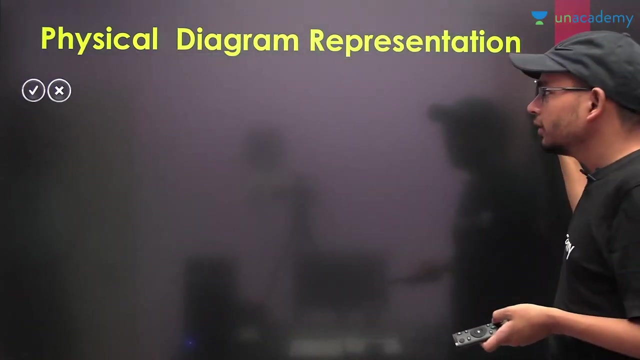 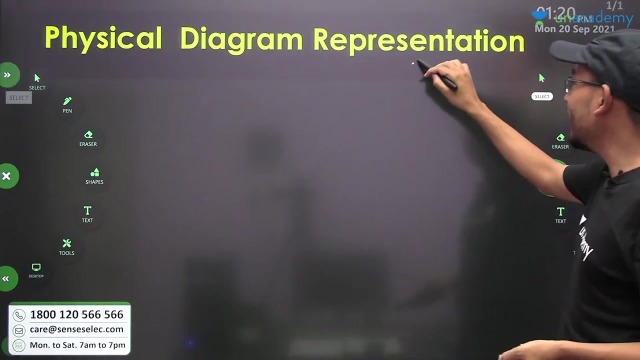 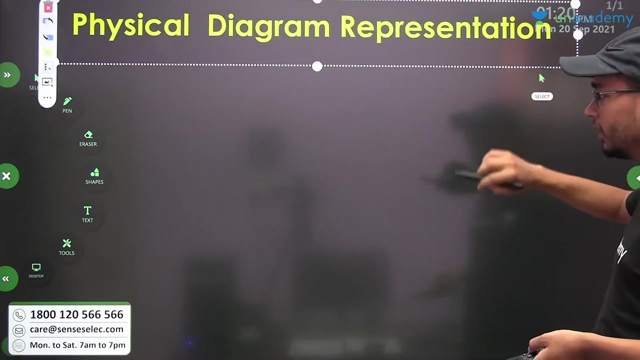 so see, this is ready from the beginning. one more ready is of 2005,. so see, this is ready from the beginning. one more ready is of 2005,. Physical Diagram Representation. We will add, adding to it Physical Diagram Representation. Properly Okay. 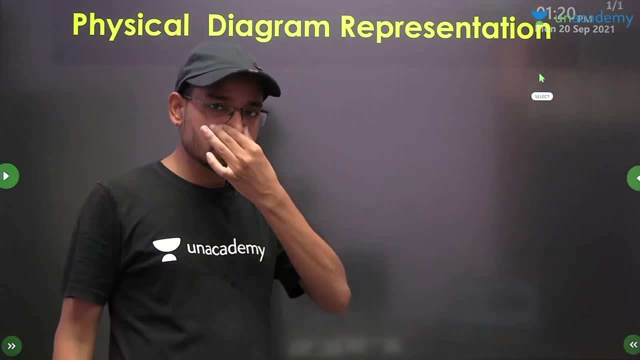 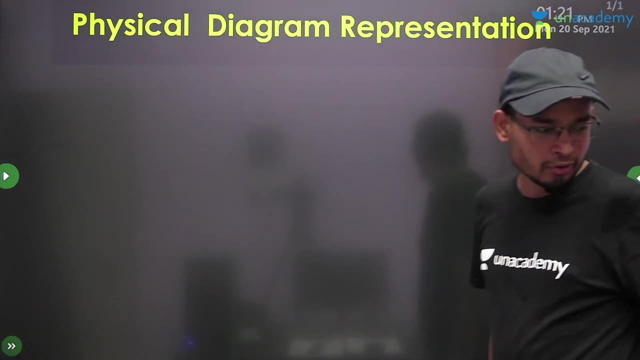 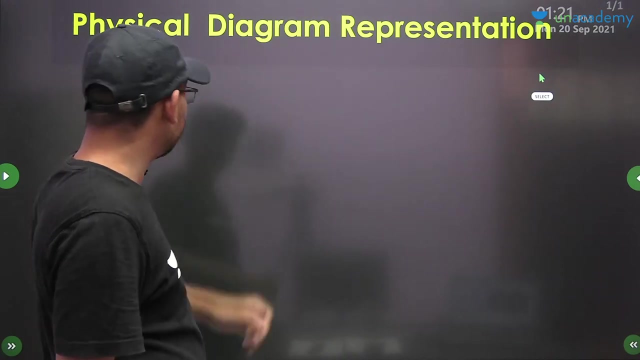 Physical Diagram Representation. We will understand it very well. We will understand the whole process very well. We will understand it by going deep. Yes, yes, yes. Wait for a moment. There is no use of that slide. Focus on it now, On this current slide. Okay, So we will talk about Physical Diagram Representation. 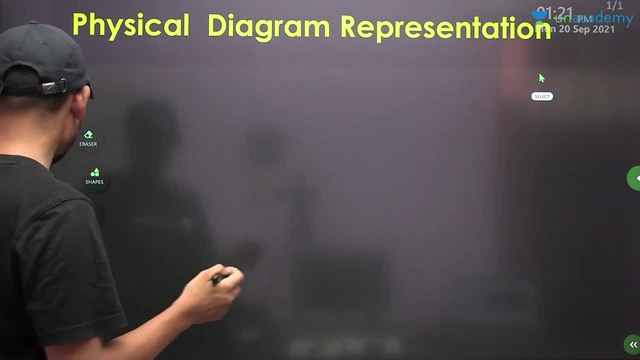 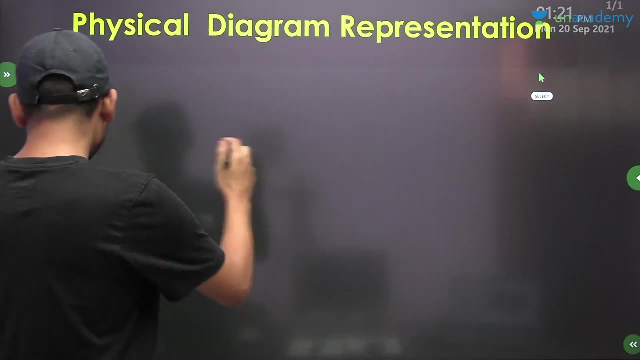 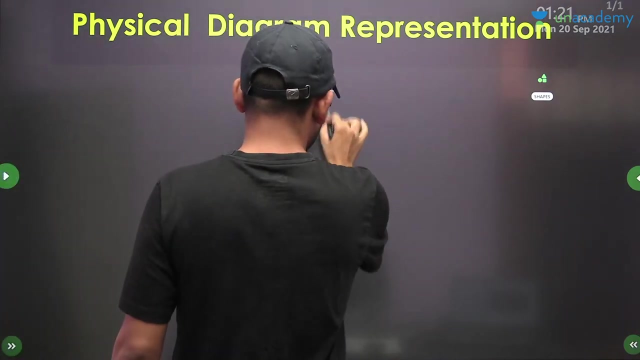 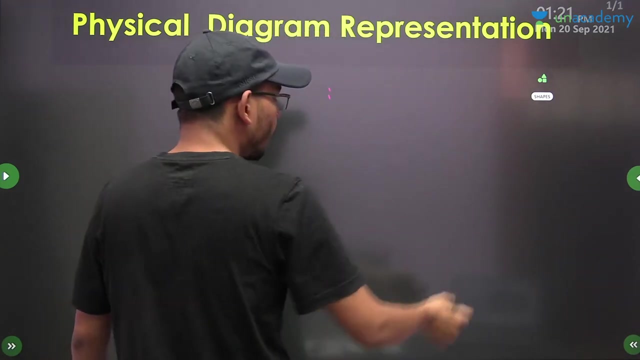 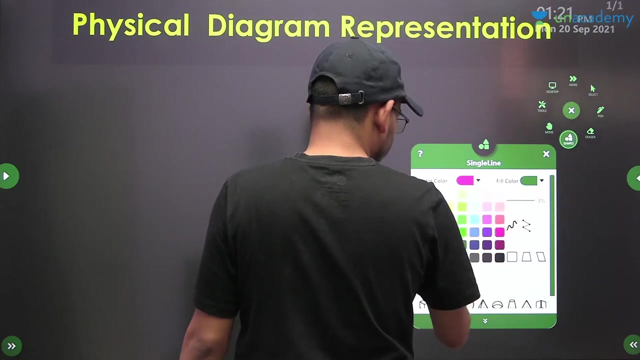 Very well, Let's go. So, first of all, We have to take a big page. All of us have to make one diagram in one page. Okay, It will be big Reactor, So we have to try it in one page. Make it one. Okay, Big, Make it big. 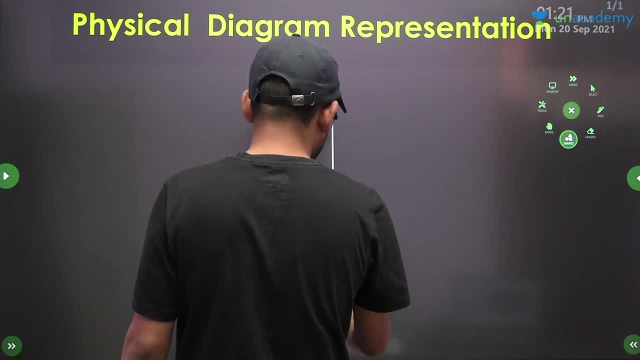 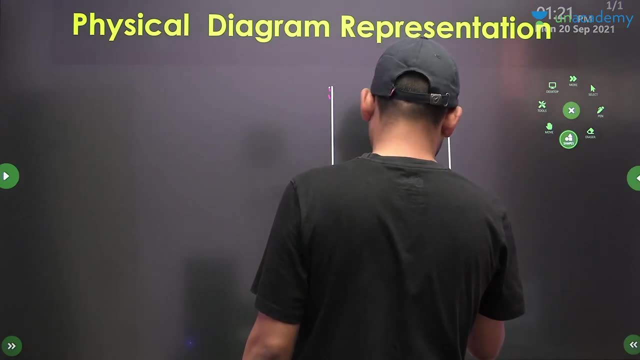 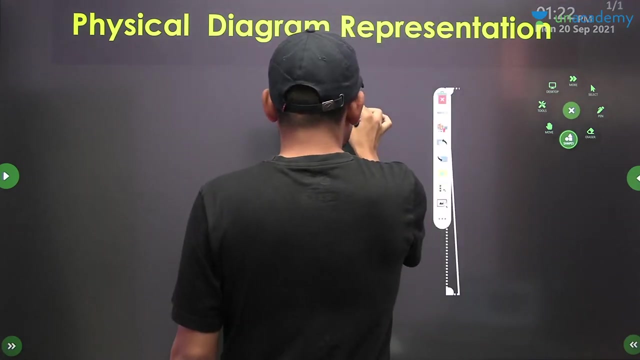 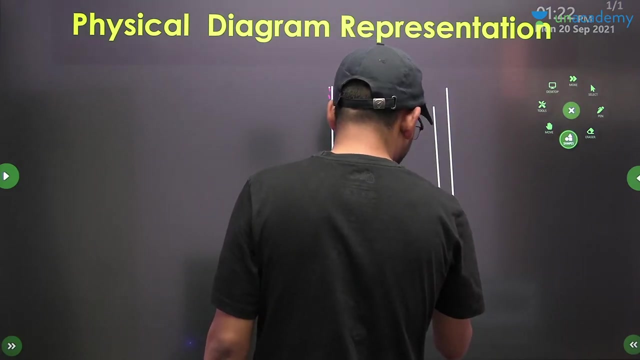 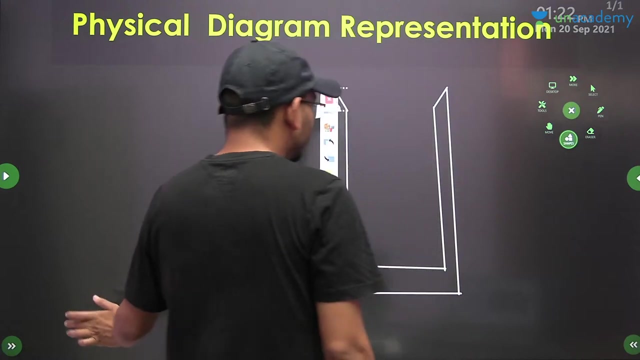 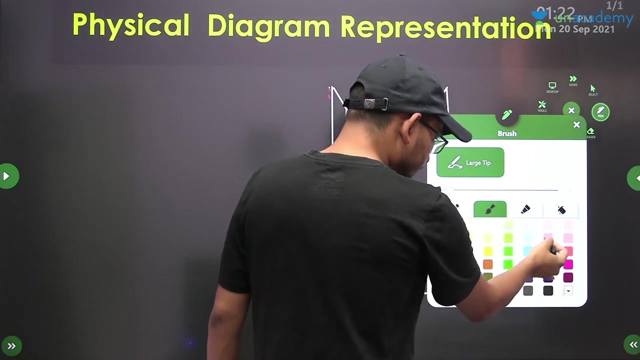 Make it big, Make it properly, Make it one page. Okay dijo, Make it bigger, Make it huge, Make it small, Make it ل. LOL. Make it big, Let's say: That's right, I'll stand. Make it a bigger, Make it big, Make it small. Okay, Under this, Whichever you want, 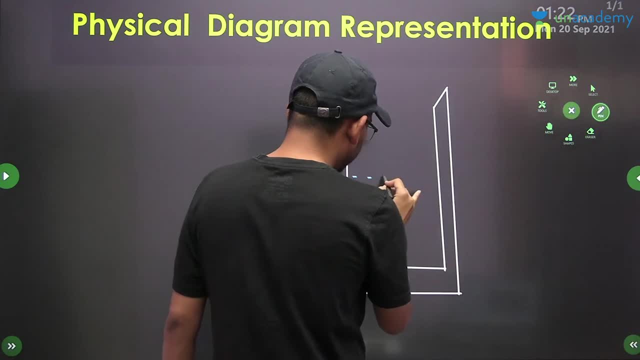 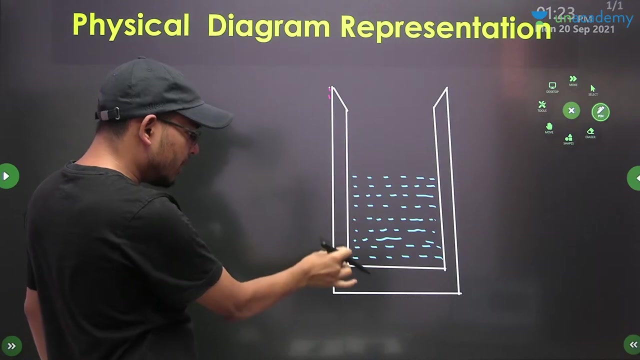 Using any liquid Ray In any liquid. it has a liquid filling in it. there can be any reaction in it. you can heat any substance, make it very well all people. this is your surrounding. it is jacketed in the surrounding and what is filled inside the water is filled. as you must have lived in the village, then you 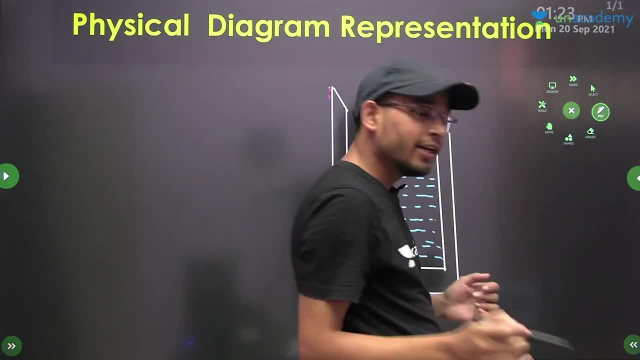 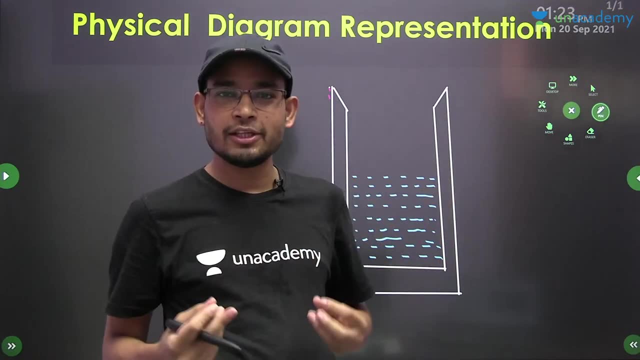 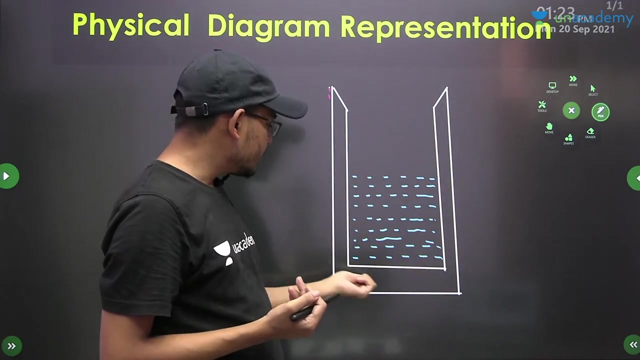 must have seen that there used to be ice in the old days. then what did they bring? they used to be covered in cloth. there used to be ice inside. that means you were given the actual ice and there was another ice outside. then it is jacketed in. which cooler. 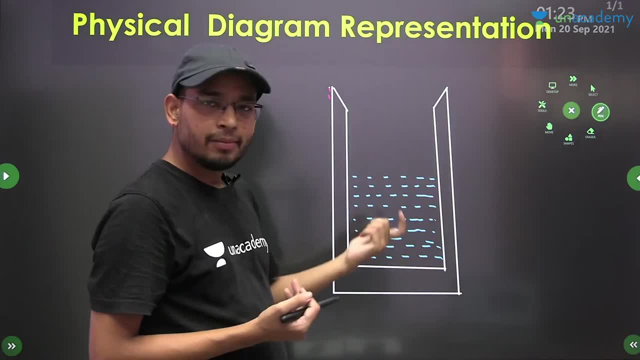 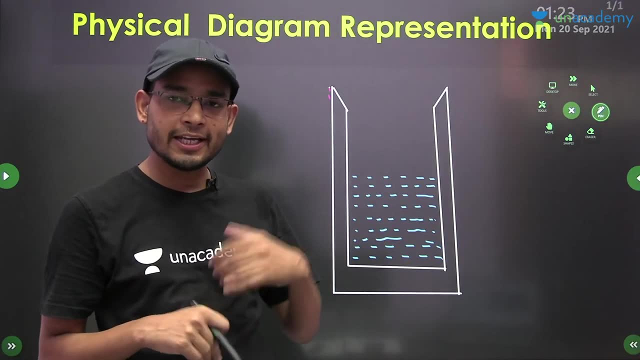 can be in which the surrounding is correct. if any steam can be, then with the help of which you can do the reaction inside this. if you are getting indothermic, then you will want to lower the temperature. if the thing is getting thermic, then the temperature will. 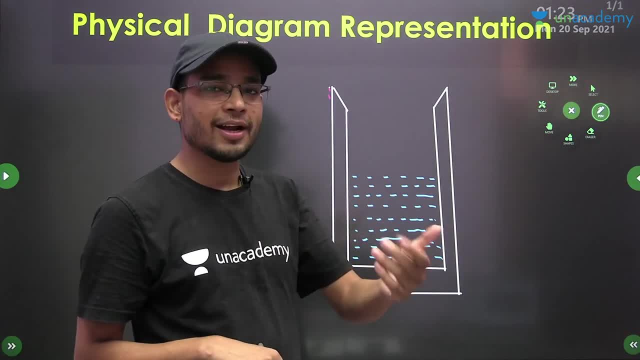 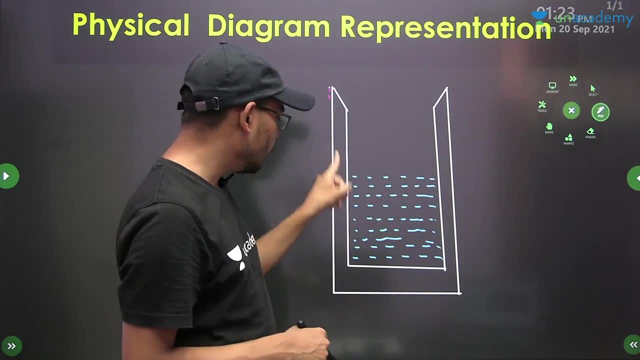 decrease, then the temperature will also increase. so water will also decrease and it will. If you want to increase the temperature, you can do it in the desired condition with the help of the coolant. What is there in it? Coolant. I will write it here. 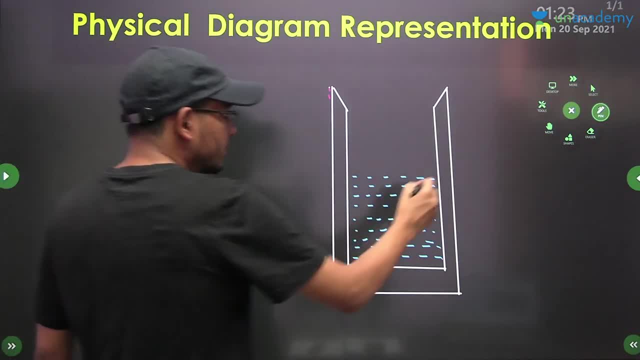 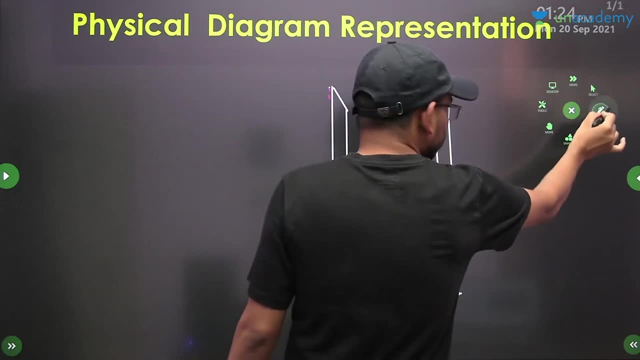 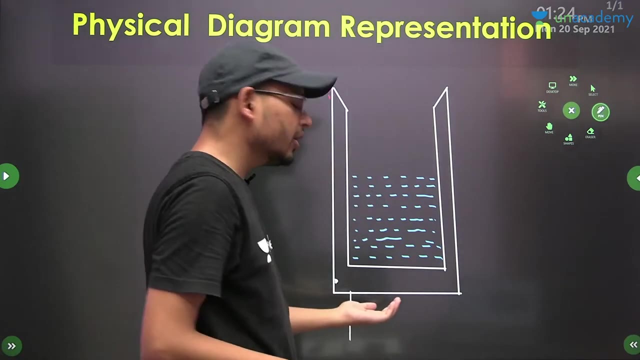 This is your coolant. I will put it from here. I will put it from here because there will be a lot of things here. I am putting the coolant from here. It can go from here. Coolant can also go and steam can also go. 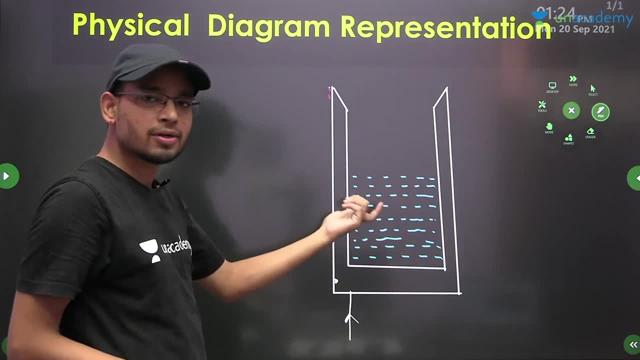 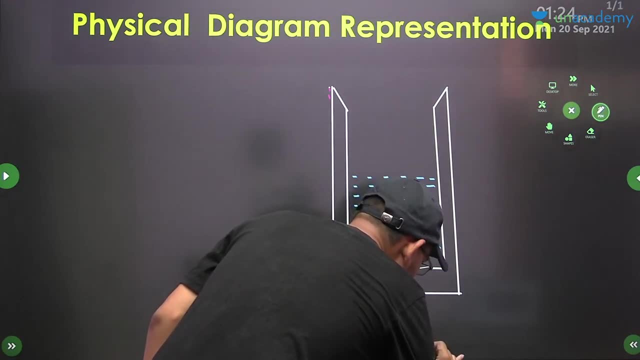 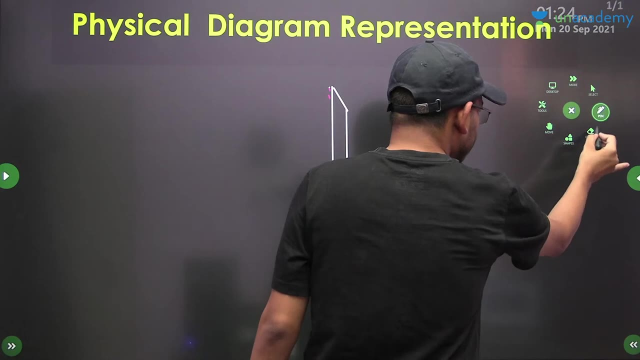 Steam can also go and coolant can also go. It will depend on your process. I will put steam, I am putting steam. Its flow rate is F and its temperature is TCI. Coolant can also be and steam can also be. I have taken coolant TCI. 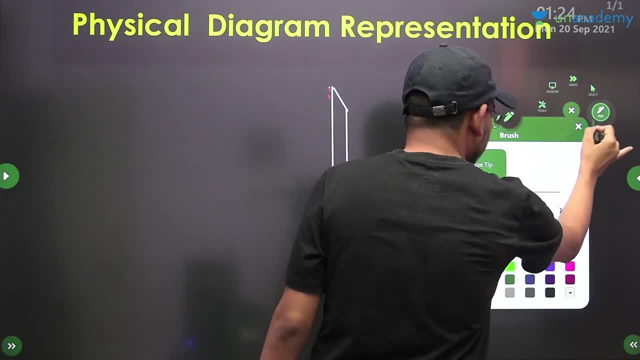 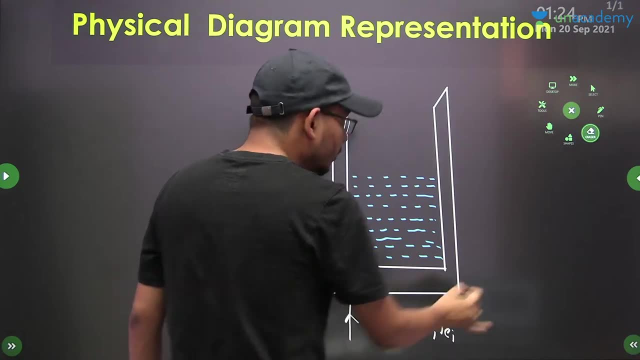 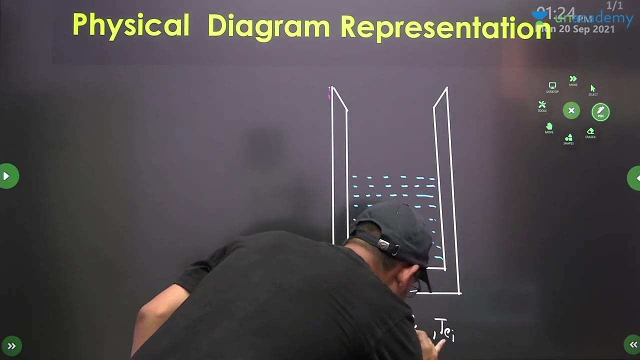 Write coolant here, Coolant flow rate. Write coolant here. Write coolant. It can be coolant and steam can also be. It will depend on the process. I will put coolant. I will put coolant. Its flow rate is FCI. Coolant's inlet flow rate is FCI. 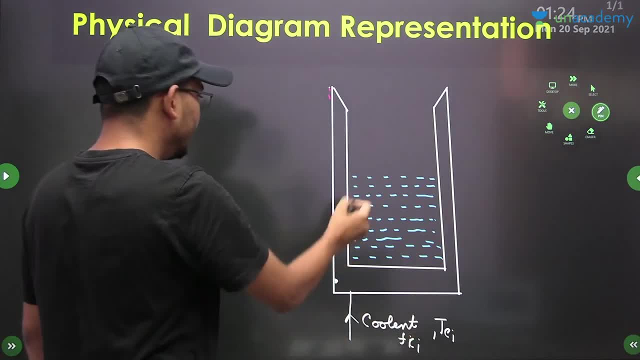 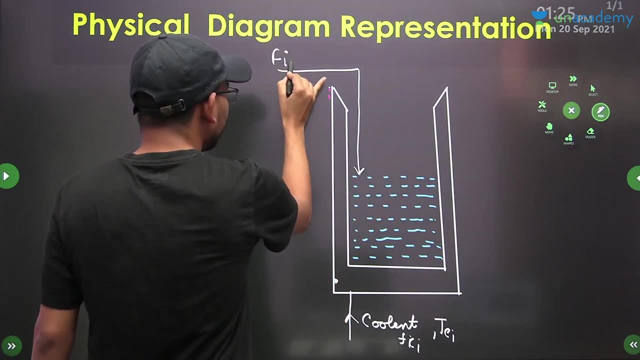 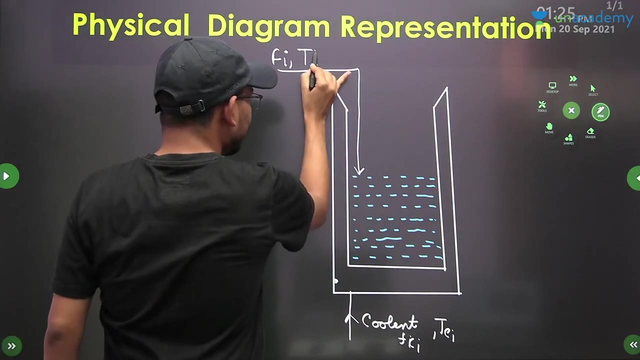 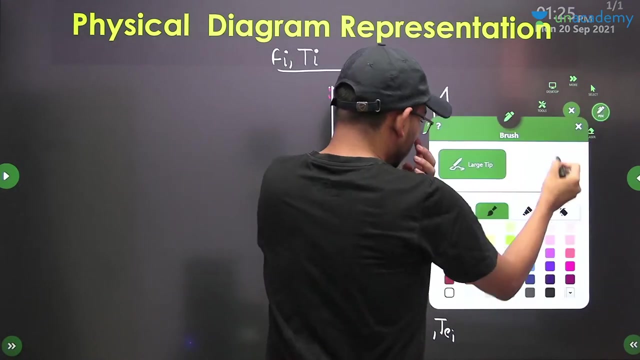 The temperature of coolant is TCI. This is our actual process. I will write it F of I. The inlet flow rate is TCI. This is the process. This is the process. This is the coolant. What is coolant? I will put coolant here. 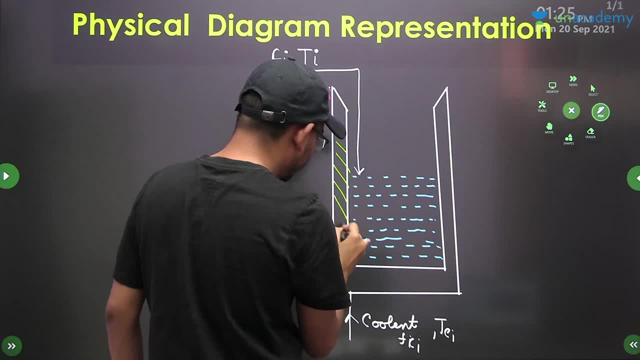 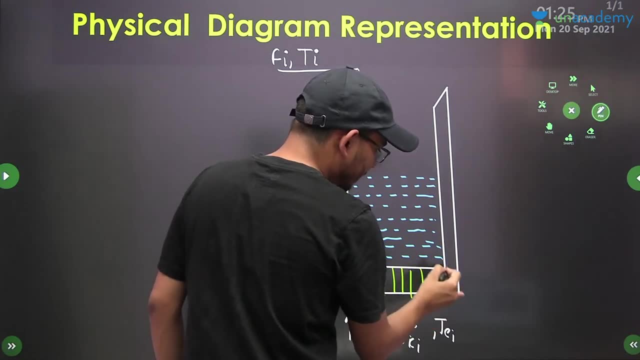 This is the coolant. This is the coolant. This is the coolant. Try to understand it carefully. I will take the comment later. Make the figure first. Make it while understanding. I will take the comment later. Everyone will make it while understanding. 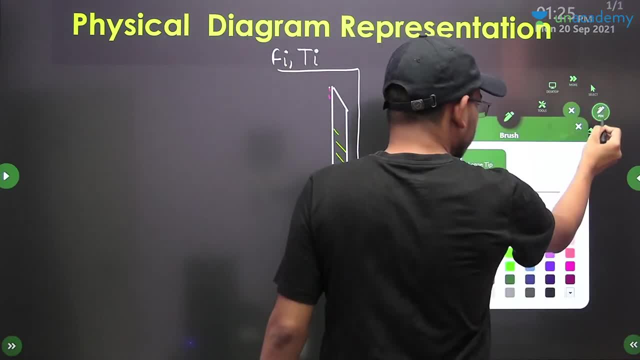 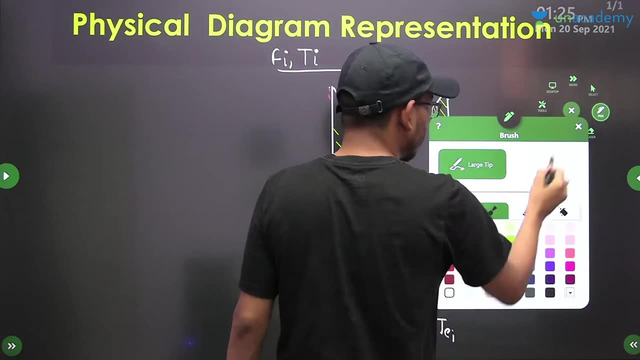 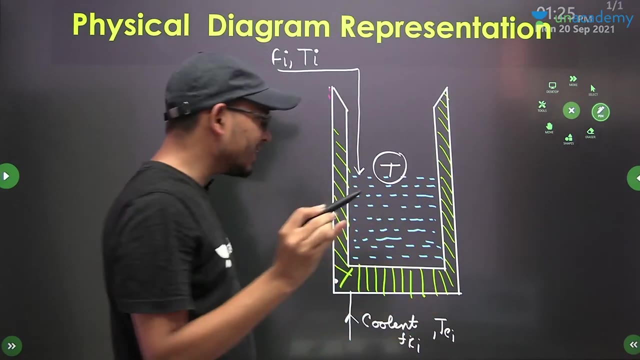 Everyone will make it while understanding Properly. If you understand the figure, then you will understand the whole process Right Now. see what is this. The temperature in this system is T, The temperature in the system is T And the fluid inlet was TCI. 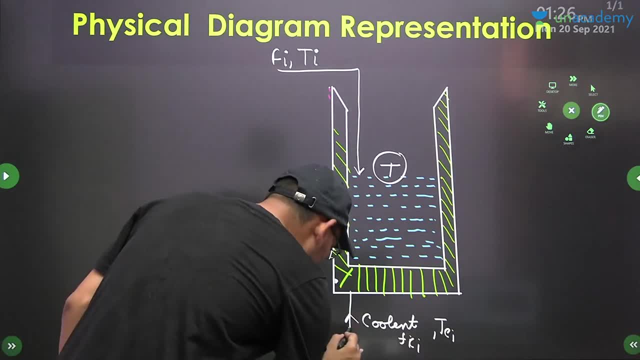 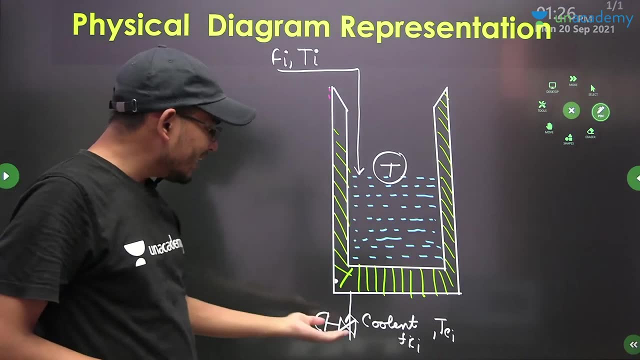 And the coolant was And the coolant was. Then I will say: here There was a valve and there was a valve. Further, this was a valve. Next we see this valve. The flow parting velocity of the coolant is FCI and that the 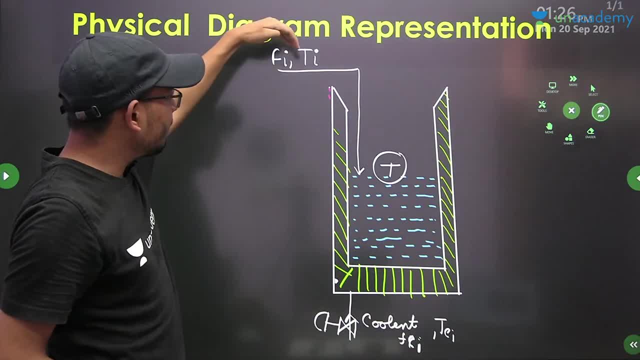 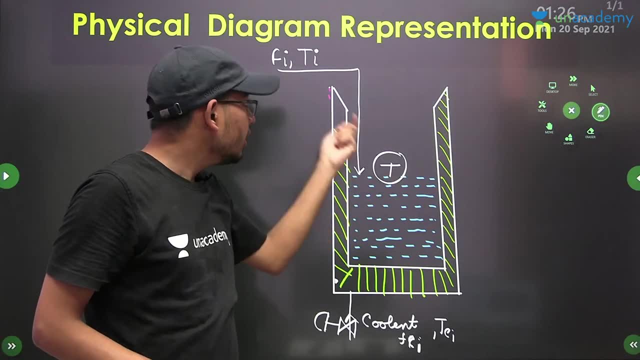 flow� velocity in the coolant is FCI And the temperature of the coolant is TCI. That our feed is getting. how much is the flow rate of the feed? FI And the temperature of feed is TCI. Now there will be something. 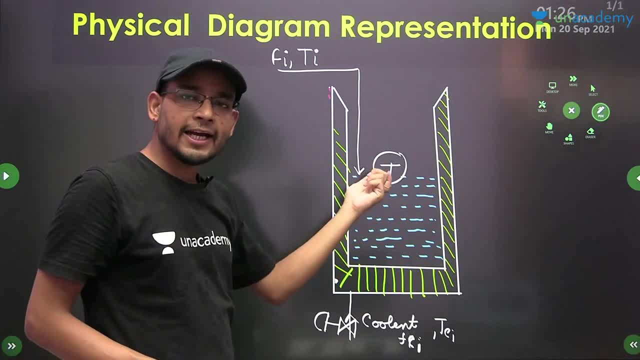 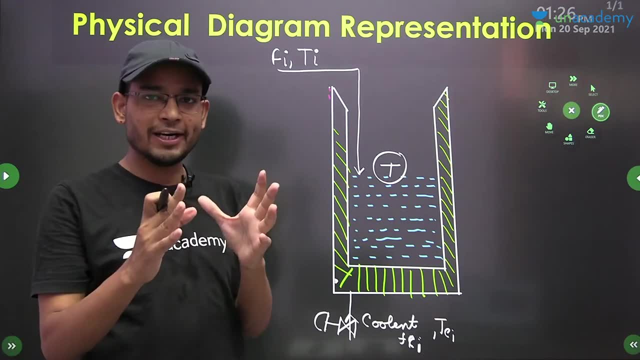 about the cylinder. so This system inside of this تمperature T. Now what is your objective? To maintain this temperature with the desired value, The set point that you have given. you want the temperature of this system to be maintained at 45 degrees centigrade. 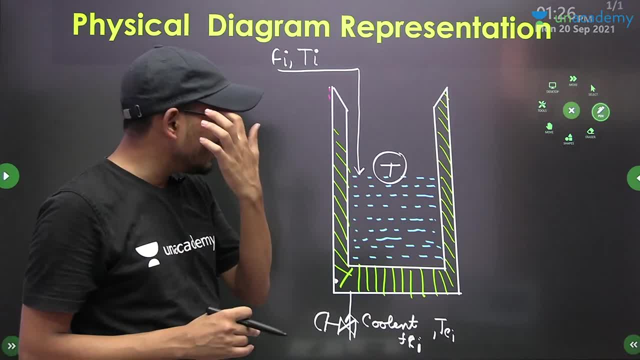 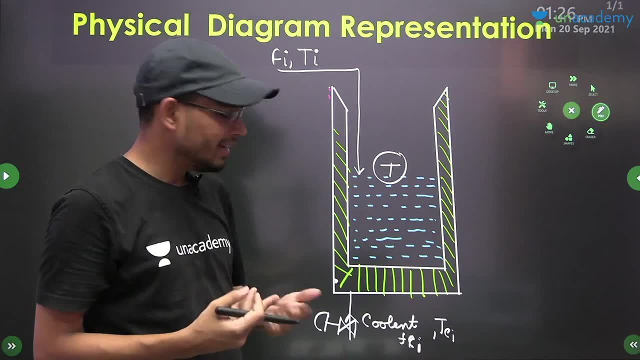 You want it to be maintained at 45 degrees centigrade. So to maintain 45 degrees centigrade, what will you do After a certain time? what will you do? You will measure it. If a process is running in your running, then what will you do? 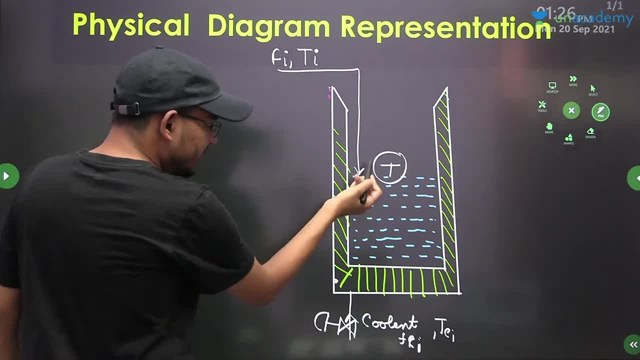 You will measure it. So you will measure it, which means you will put a measuring element in it. Which measuring element will you put? The one measuring the temperature And the one measuring the temperature? where will it go In the controller? 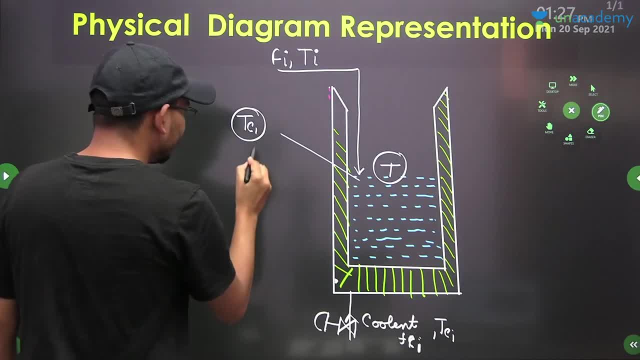 I will write it as TCI, TCI, TC1.. And how will this controller match its value With the set point TSP, The set point of the temperature? suppose you gave 45 degrees centigrade and it measured T. 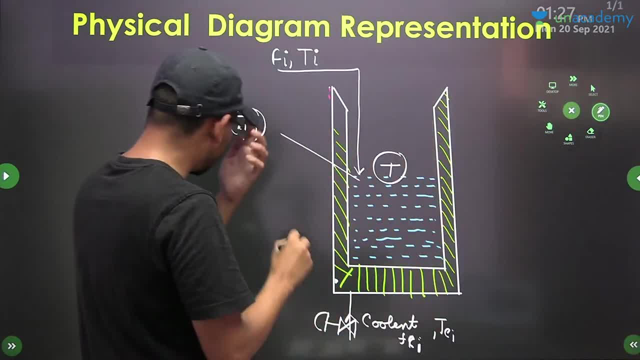 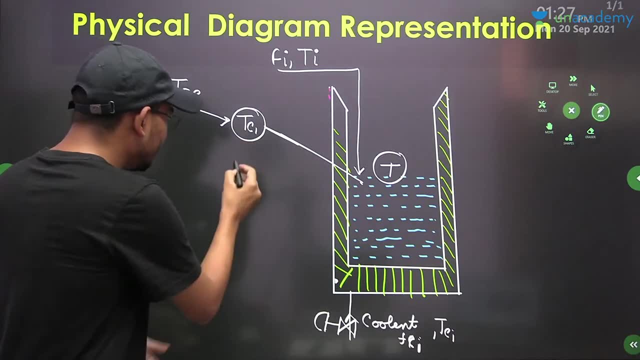 Where will it go In the controller? It will go in the controller. Then what will the controller do? It will produce the error. Where will it go In the controller Now? what will the controller do? The process that is going to come out from here. I have already told you this thing. 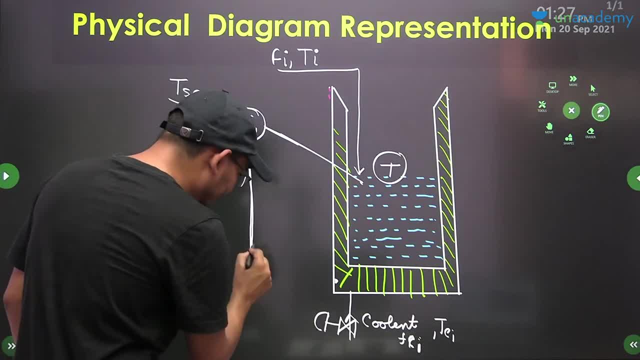 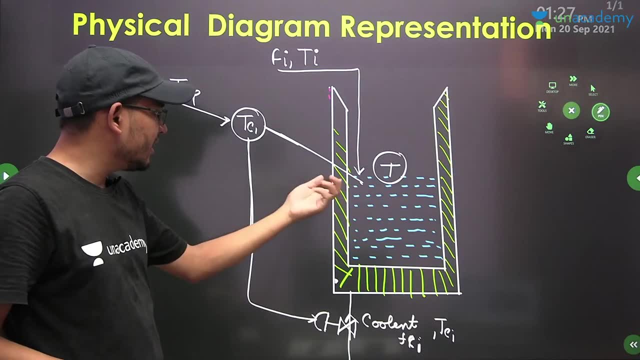 Where will it go In the final control element? What is the final control element? Your flow rate is coming. What will it do to the valve of the flow rate? It will come to the valve. It will read the valve that its temperature has increased. 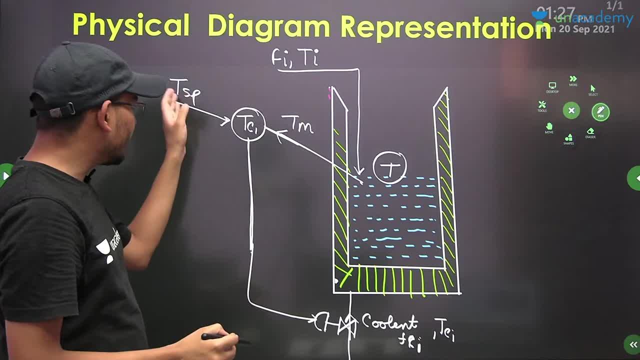 Your TEM will be going from here. This TEM will be going. This set will be going. This TEM is going. This TEM is going. So what will this TEM be doing? It will be looking at this TEM and it will becoming aware of your TEM. 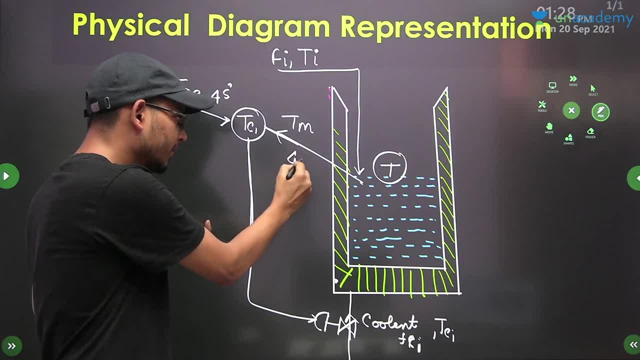 Suppose, for example, TEM's temperature is about 45 degrees centigrade. Let us say this TEM is 45 degrees centigrade and TEM has measured 40. So the error will go to its 5.. So now, what will this TEM do? 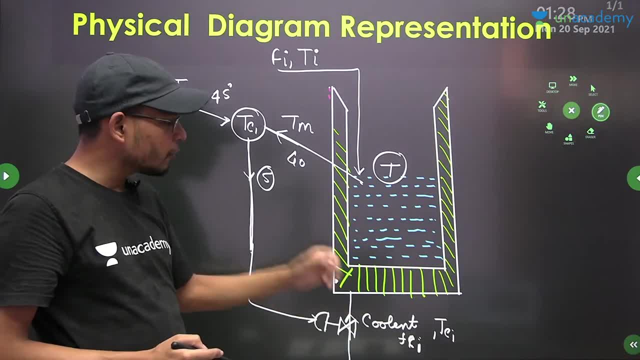 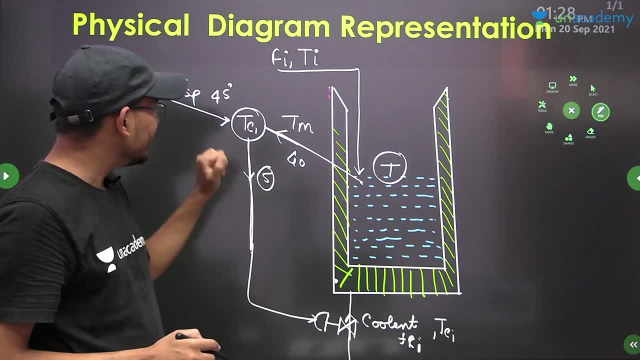 What will it do to the flow rate of the coolant? It will decrease it. It will decrease the flow rate of the coolant Right, So that your temperature is maintained. Fine, What is TEM's temperature? It is 40. And what will we need? 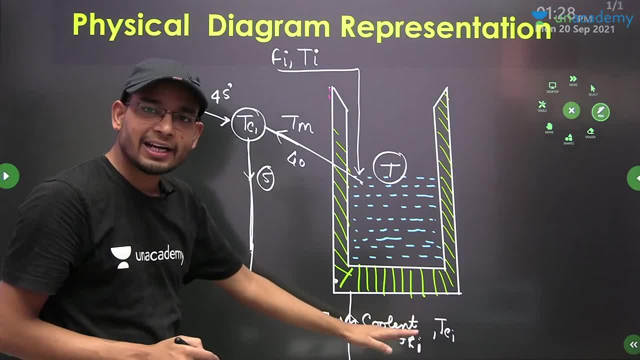 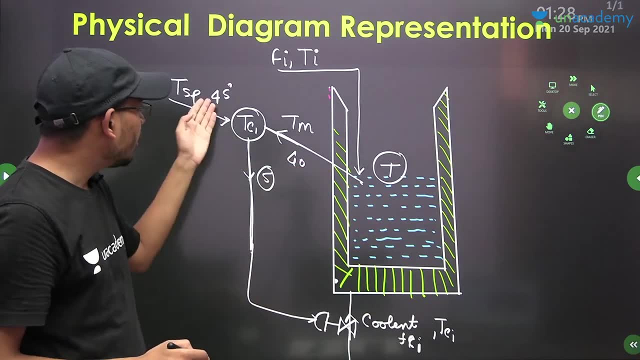 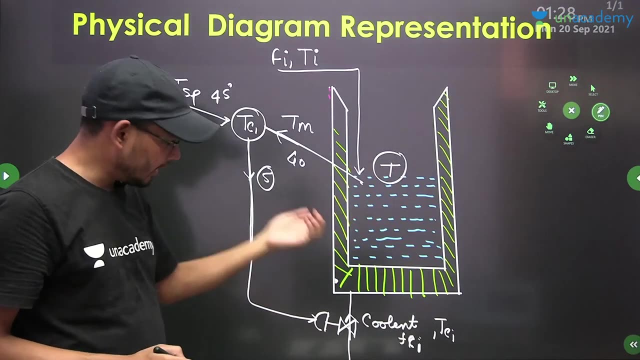 We need 45 and this is the flow rate of the coolant. So what will it do to the flow rate of the coolant? It will reduce the flow rate of the coolant because the coolant was going more. now there is an exothermic reaction in it, so the temperature is 40 and you have set up 45, so you will reduce the flow rate of the coolant so that its temperature increases. so you must be doing this work, what you must be doing. you must be doing this work right. 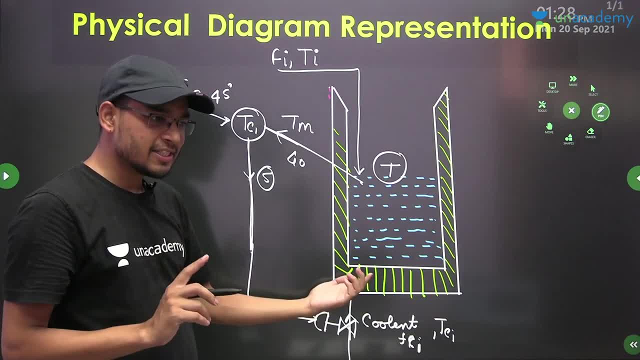 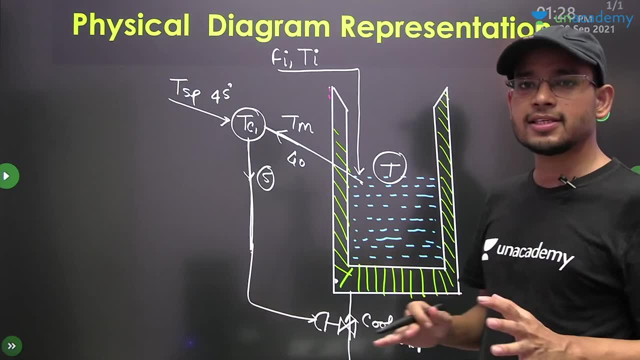 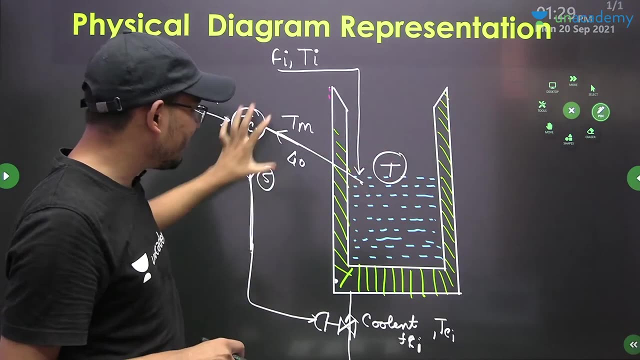 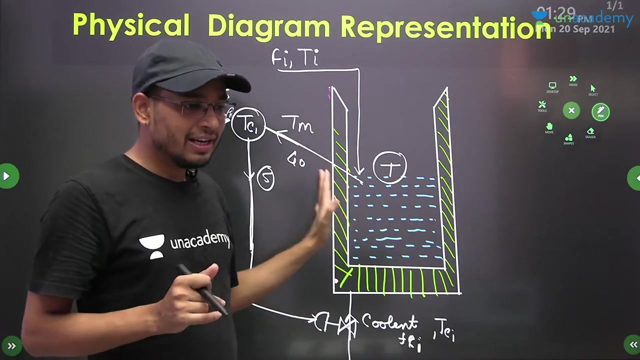 Okay, everyone understood this much. yes or no, everyone understood this much. this is your normal process. this is the normal process. okay, this is the normal strategy. everyone understood this much. now, I have not put your advance control strategy in it, what I have done now. this is your normal feedback diagram. okay, normal, but now where will the problem come? where will the problem come that you have to do this work? 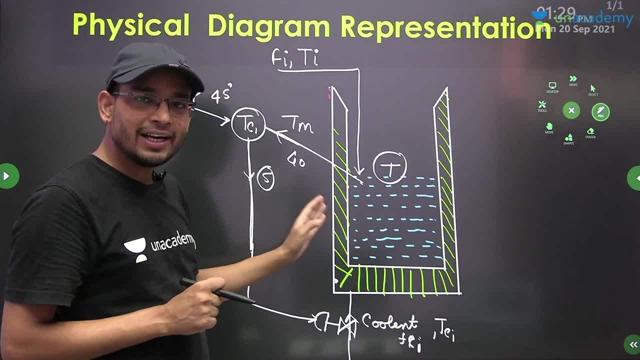 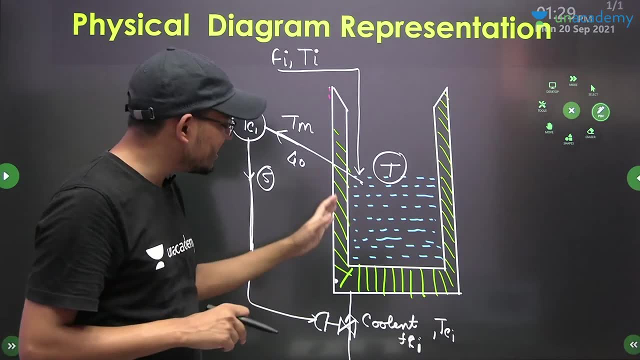 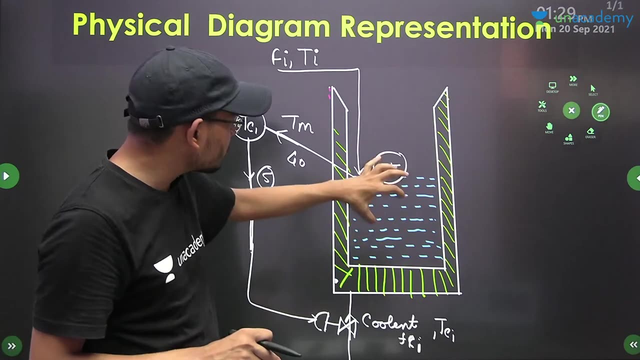 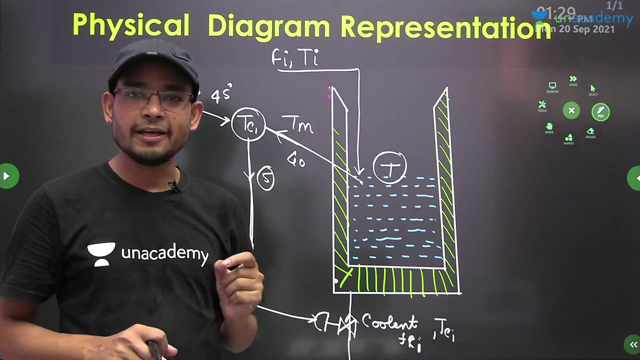 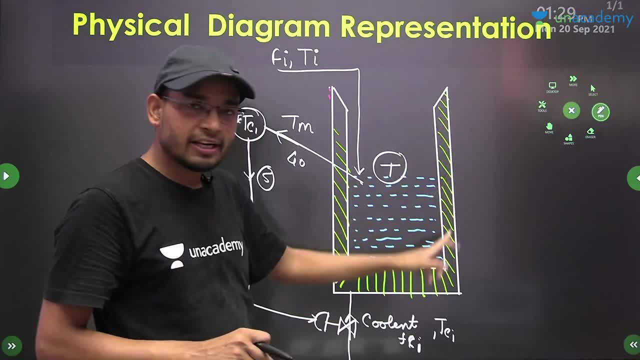 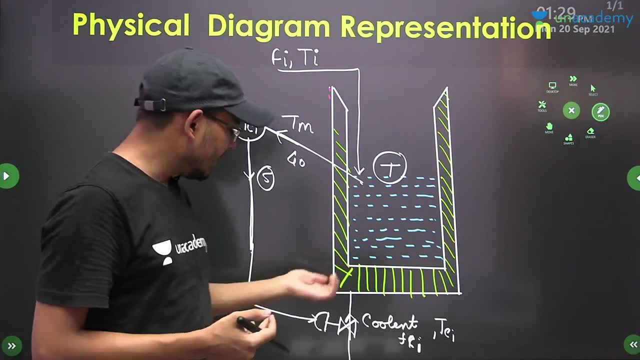 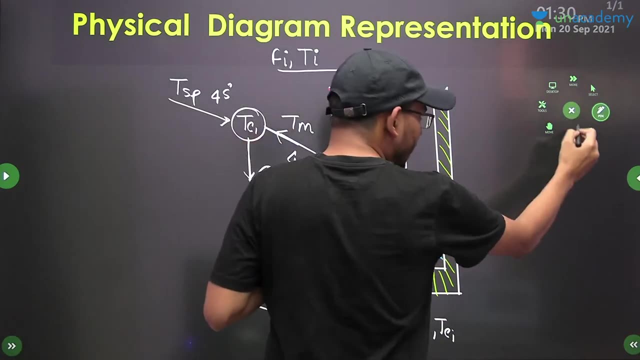 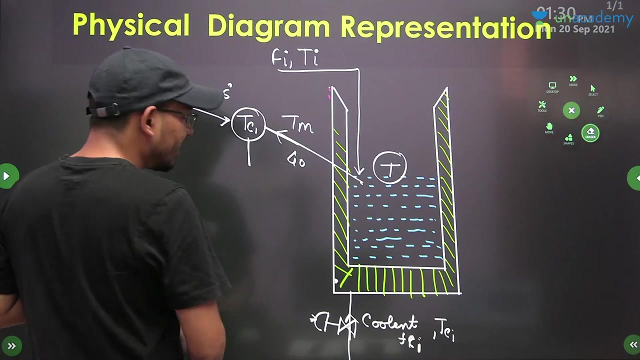 it. The coolant which is in the surrounding here also measures the temperature of this. so when we measure its temperature and apply it in this process, then we call it advanced control strategy. okay, so this is our normal one. this was normal, this was our feedback which we had made earlier. it was okay. now what do we do? we will go a little in advance mode. so what will I do? what will I do? I have made it just to explain to you now what will I do. I will also measure the temperature of the coolant. what will I do? I will also 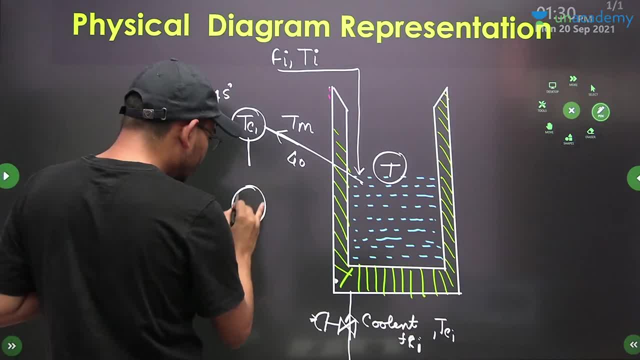 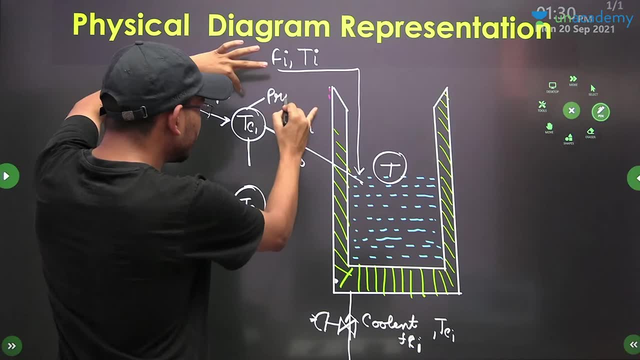 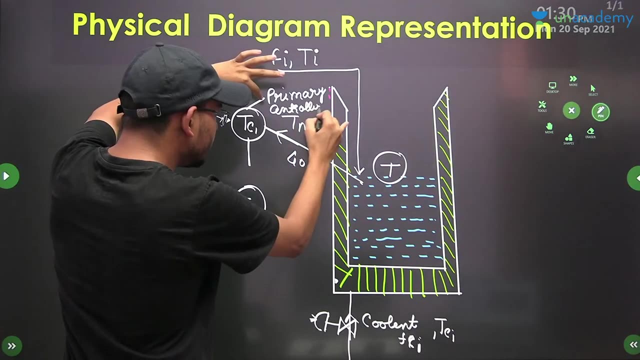 temperature measure. kalunga to ista matlab main ek aur controller lagaunga TC2, TC2. achcha, jo isko bolte hai primary controller. isko bolte hai primary controller, primary controller. isko bolte hai primary controller. jo primary controller ka jo output hoga. jo primary controller ka jo output hoga book. 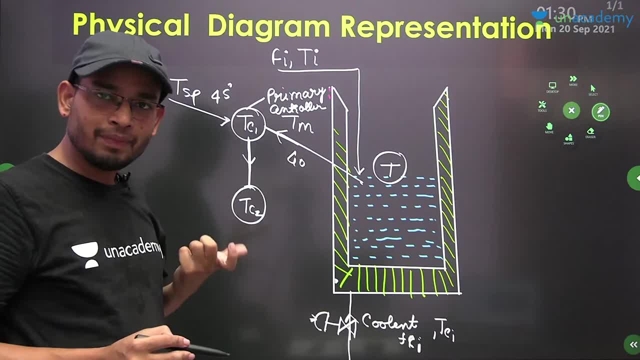 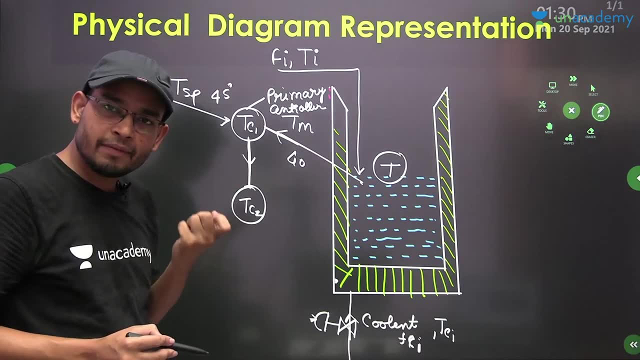 secondary controller ke liye input ka kaam karega. sar log, zara batao: jo primary controller ka output hoga, jo secondary controller hoga, uska input ka kaam karega. everyone are ok with this. everyone are ok with this secondary. 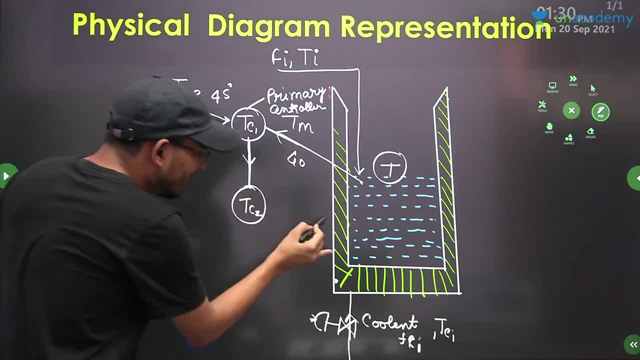 controller hoga. uska input ka kaam karega. to ye bolega ki bhaiya, ye input itna aaya aur ye coolant se kya karega? match karwa lega. ye aapka aara hai, ti ye aara hai. 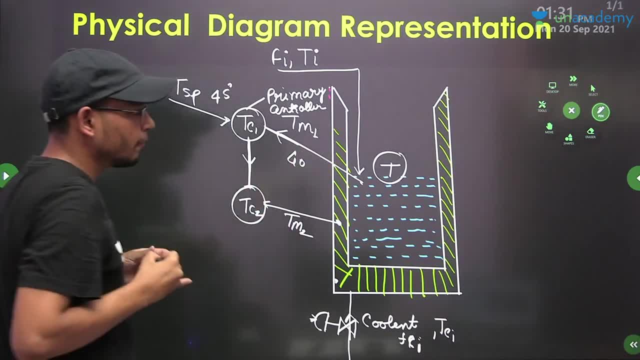 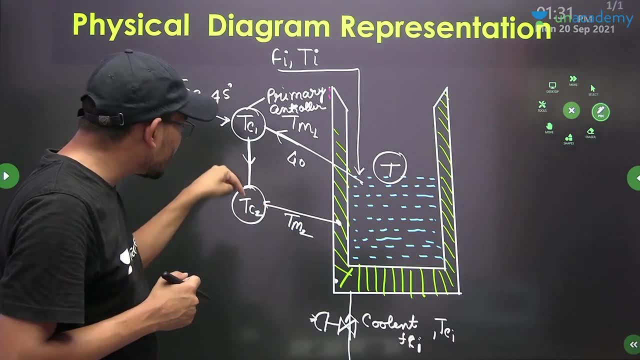 TM2 aur ye tha TM1. fine, thik hai. ye kya hai measuring device, ye coolant ka measure karega. ye poch jayega yahan pe aur yahan se input aarha. itna, ab, itna, jo error hogi, yehaan se任 produce karega. 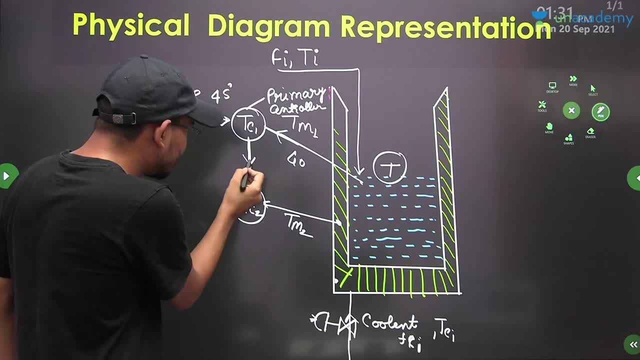 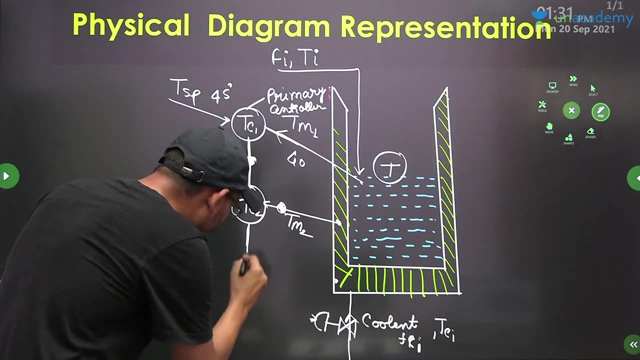 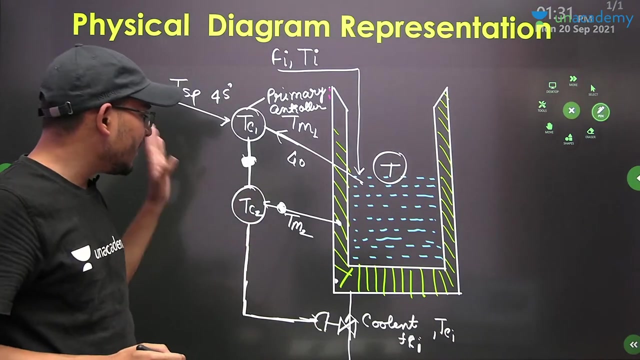 jo itni error. hogi itni jo error. worthless meeting tk valley. kisme jayegi controller ke ne Erfolg kaha ika dal yo Tata vega controller bhaji Usually TY and moale Elements to isko purple kholna hoga. and did he design based on track by its on will depend. 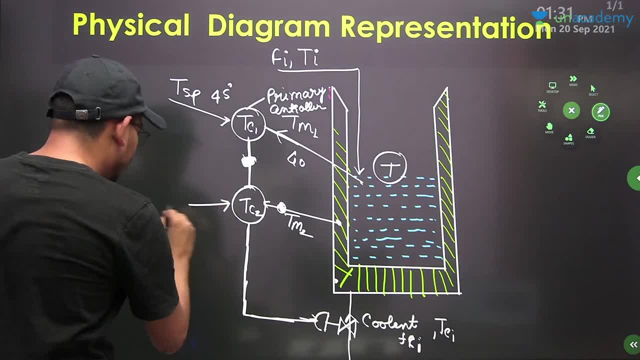 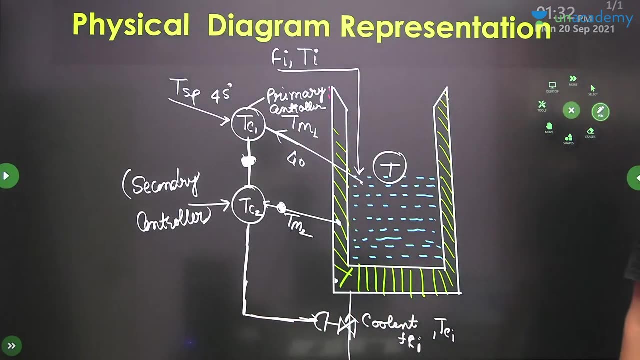 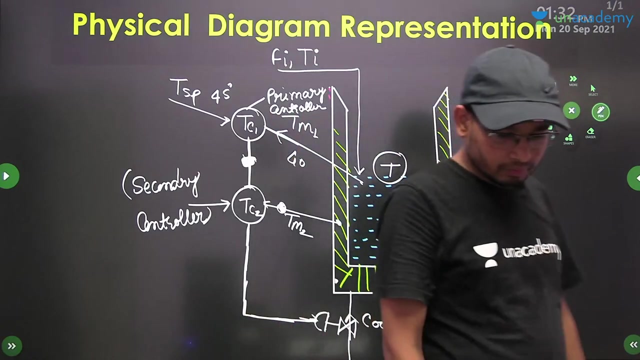 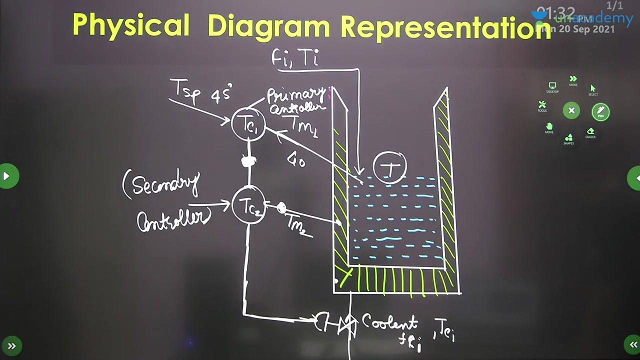 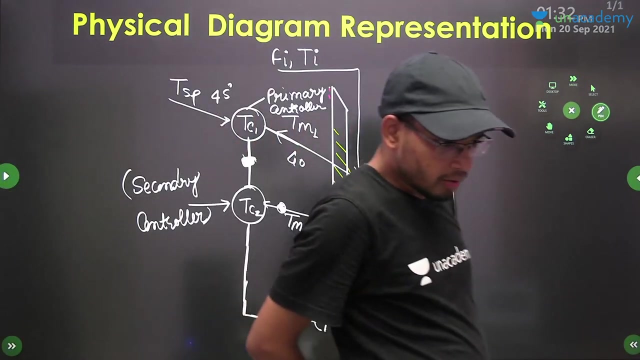 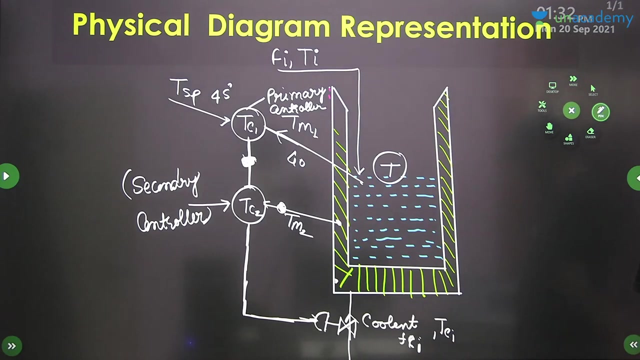 Whose Secondary controller? What is this called? Secondary controller? Secondary controller? This is called a secondary controller. First, make this much. This is called a secondary controller. Hmm, No, no. what is the set point of the secondary controller, Kunal? 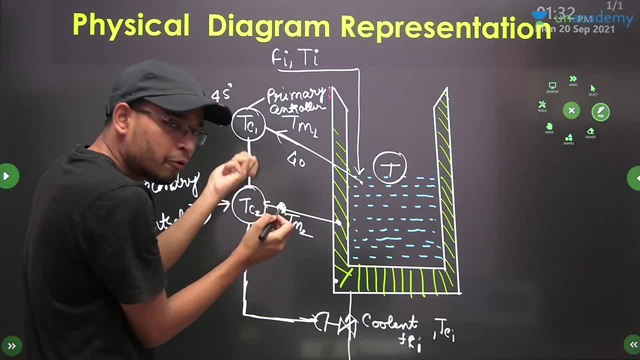 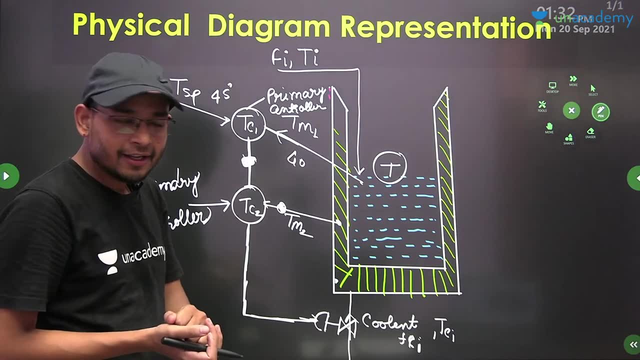 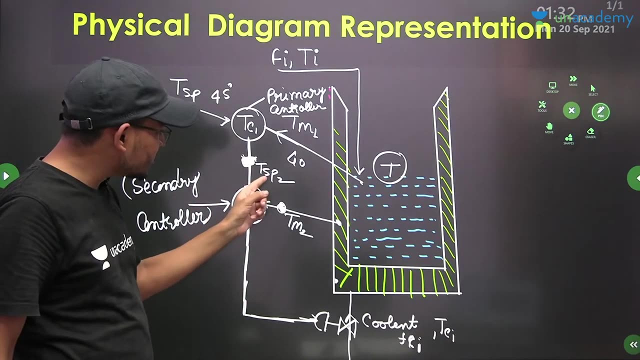 This is the secondary controller, The output coming from the primary controller of the secondary controller. This is the set point for the secondary controller. Okay, this is the. What should I write? TSP2.. Should I write this? Okay, what will happen? Whose TSP2 will happen? 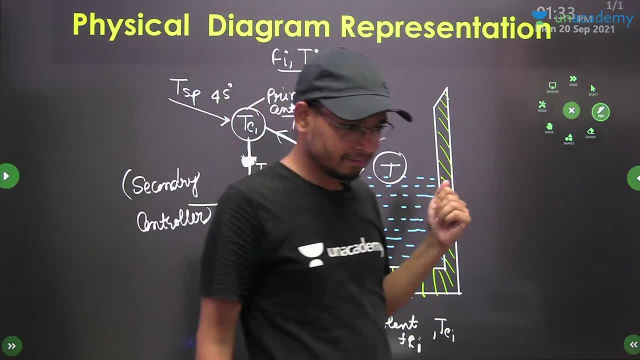 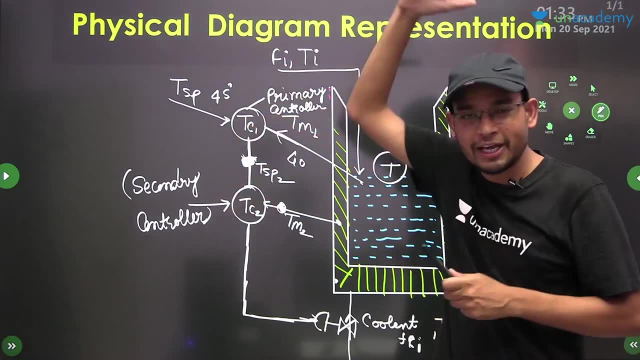 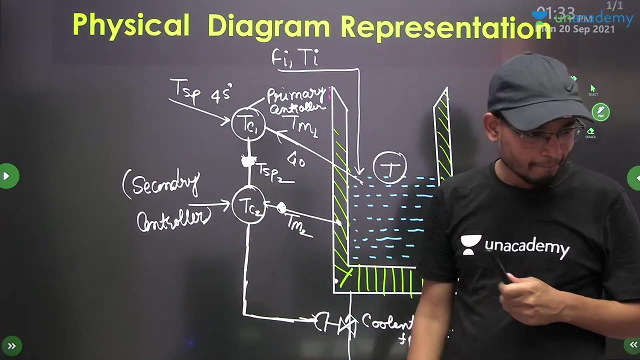 This is the set point for the secondary controller. Got it? What is this? What will be the output of the primary controller, of the secondary controller? What will happen? Its set point. Got it? So this is the set point. This is the set point. 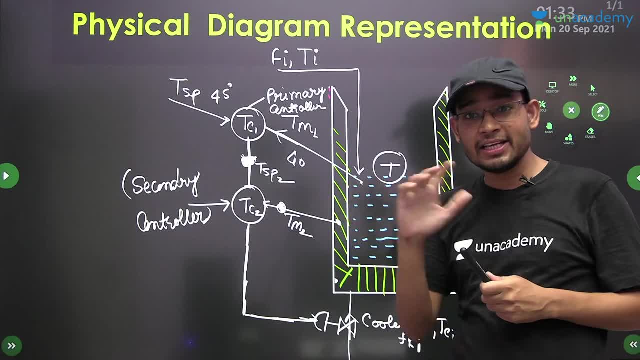 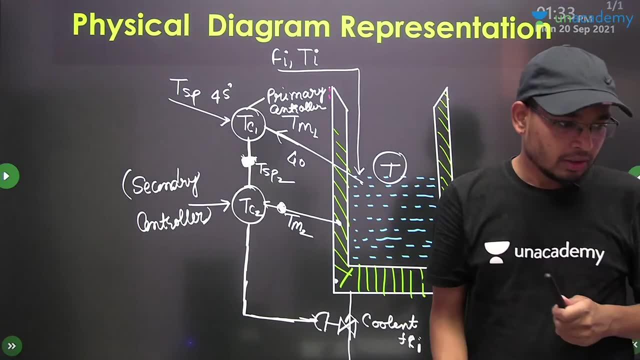 Everyone should understand this very carefully. This kind of thing does not come quickly in understanding. You have to understand each and every thing properly, Is it clear, Kunal? Yes, you can ask your doubt. Okay, so this is our RI Coolant. 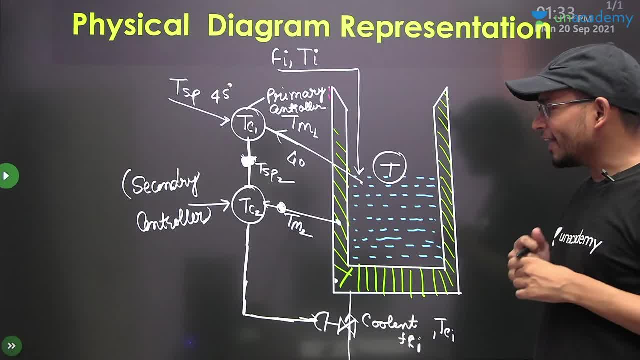 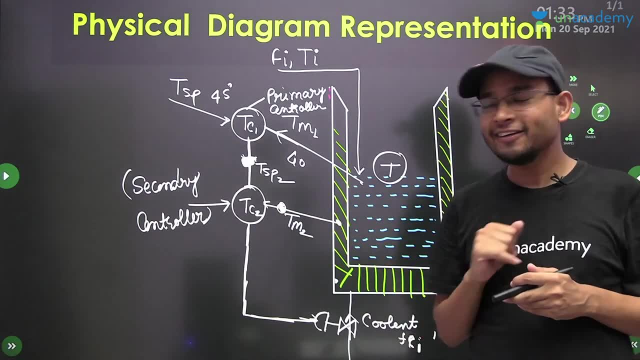 Now see what is the benefit of this. What is the benefit? That? now your system is advanced. Now it knows the temperature of the coolant as well. It also knows this much. For this, the work has become easier. Now see here What will change here. 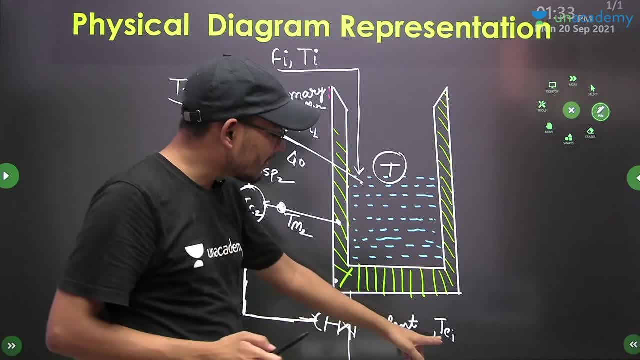 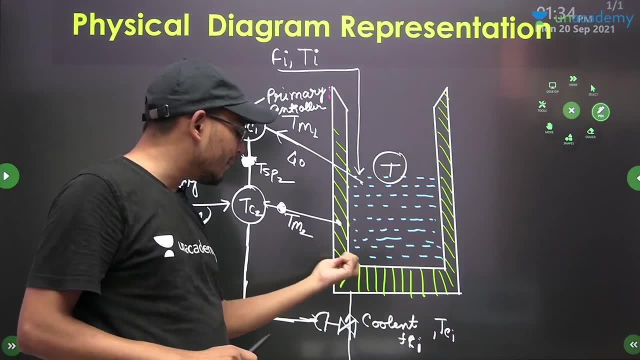 Here the change is the flow rate. Your temperature TCI never changes. What does it change? Flow rate, Okay, so now directly its flow rate, that you know its temperature, So you can easily get the flow rate to fluctuate. Okay, so what does it always change? 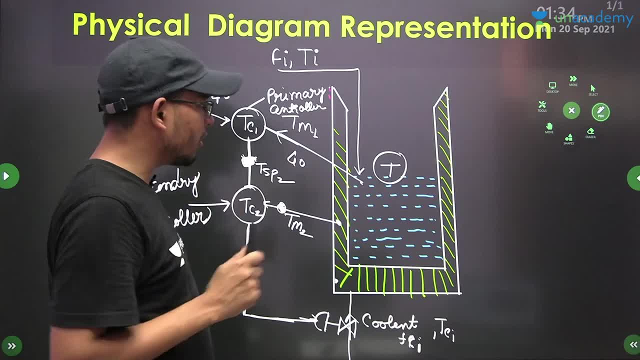 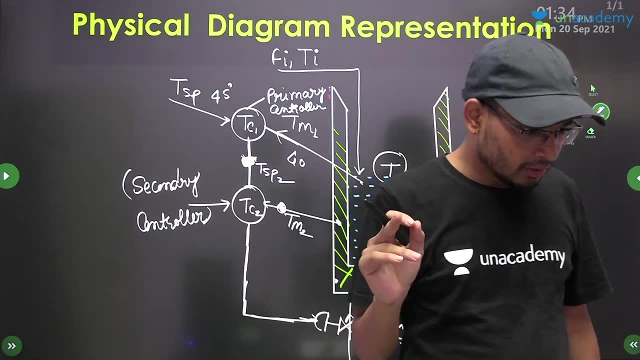 FCI. This is the Manipulated Variable. Okay, everyone now tell me What is the Manipulated Variable and what is the Measurable Variable. Everyone tell me What is the Measurable Variable and what is the Manipulated Variable. 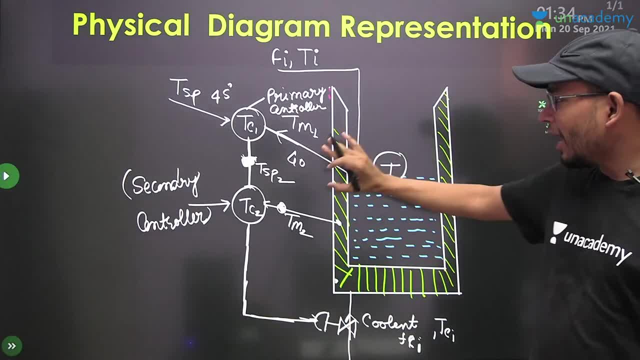 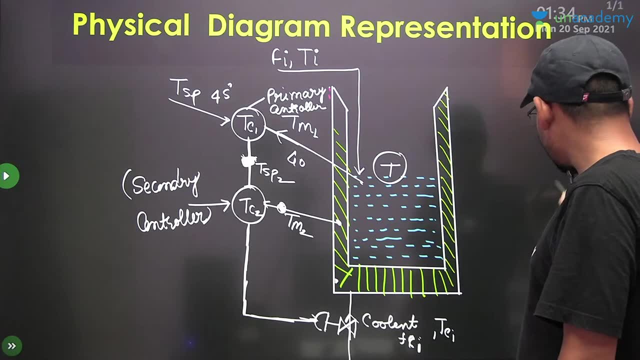 Hmm, I am telling you now, First of all, everyone, tell me What is the Measurable Variable and what is the Manipulated Variable. I will tell you absolutely. I will repeat the process from A to Z, Don't worry about that. 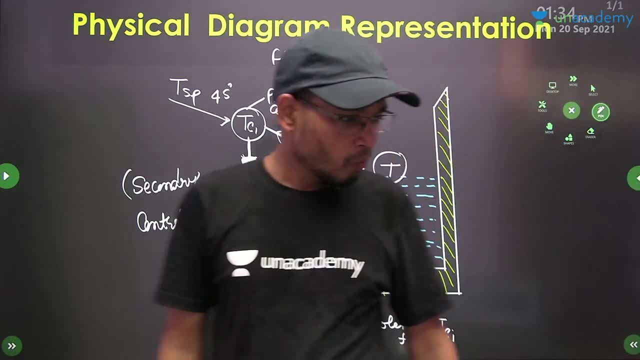 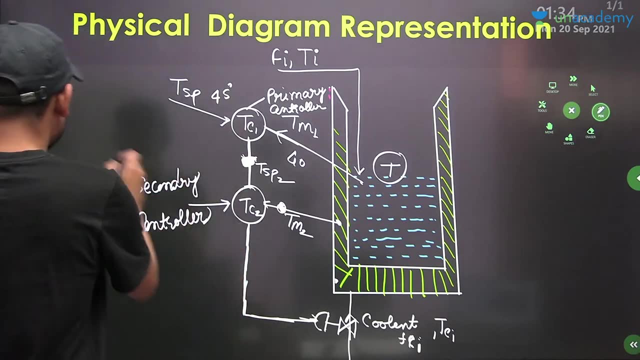 You will learn it. How many measurable variables are there? Two: How many measurable variables are there? Note number 1. This is the question of GATE 2005.. So in GATE 2005,, it was asked: how many measurable variables are there. 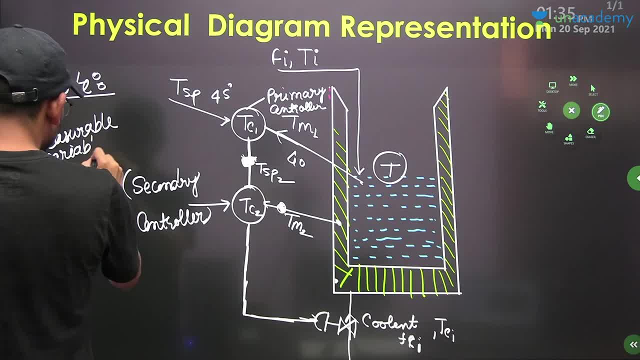 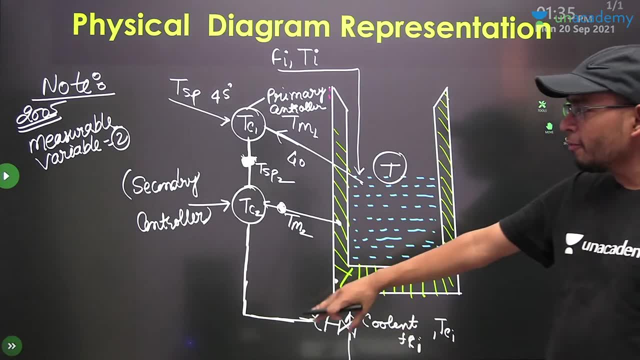 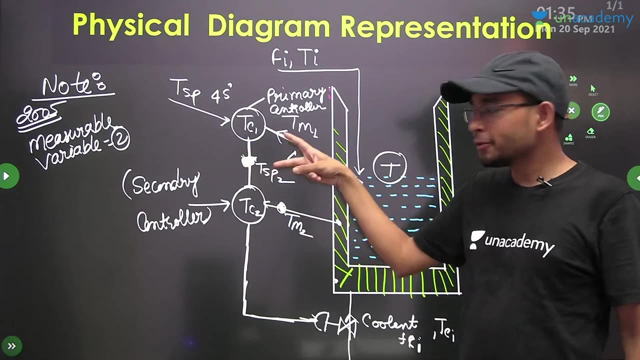 Measurable variables. Measurable variables equal to 2.. How many are the manipulated variables? Yes, How many manipulated variables? This is the measurable variable. Two: One is a measuring device. This is the two. This is the measurable variable. 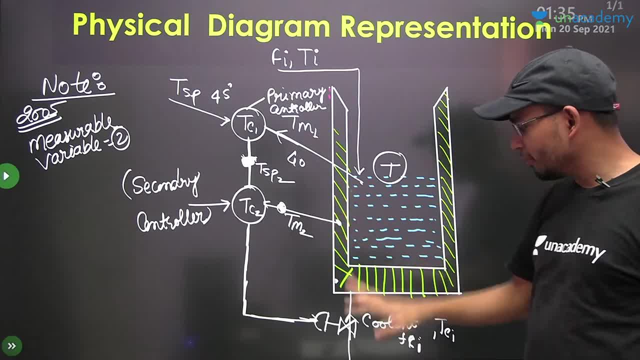 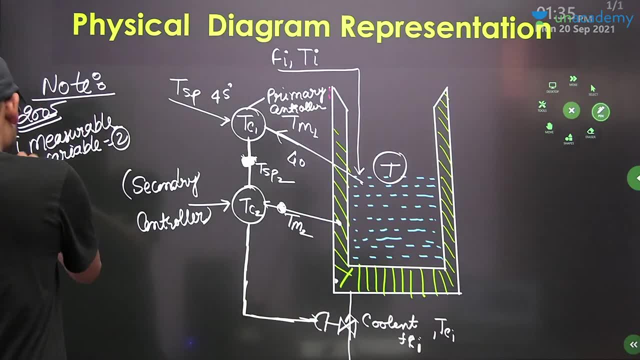 What are these two Measurable variables? Now I will ask how many are the manipulated variables? One is the measurable variable. Second, I will write how many are the manipulated variables. Manuplated variable. How many are the manipulated variables One? 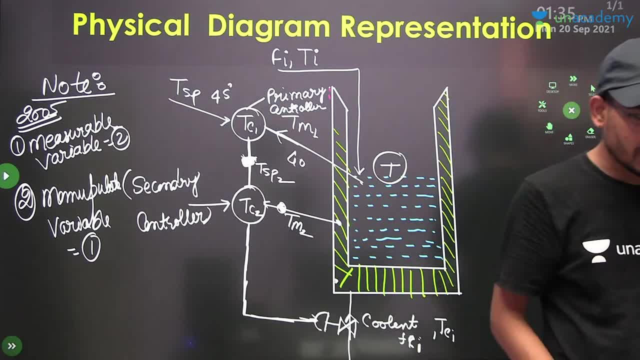 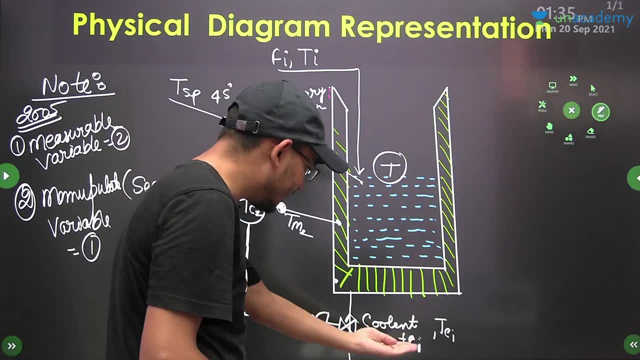 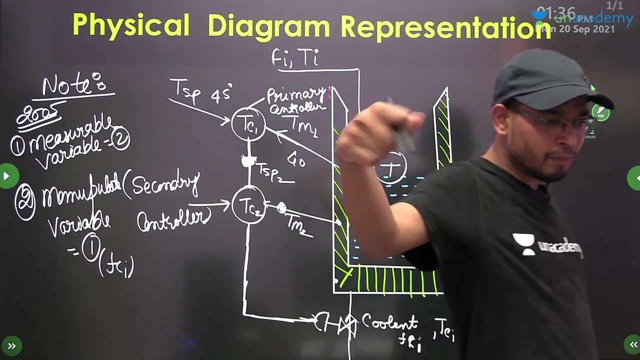 How many are the manipulated variables? One Who can be manipulated: FCI. FCI is the coolant flow rate. What is this FCI? What is this Manuplated variable? Very good Janhavi. Very good Janhavi. 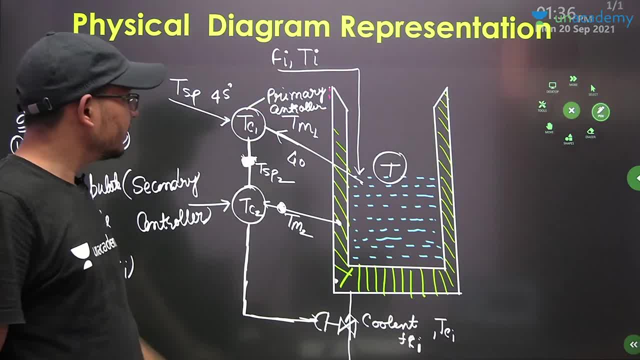 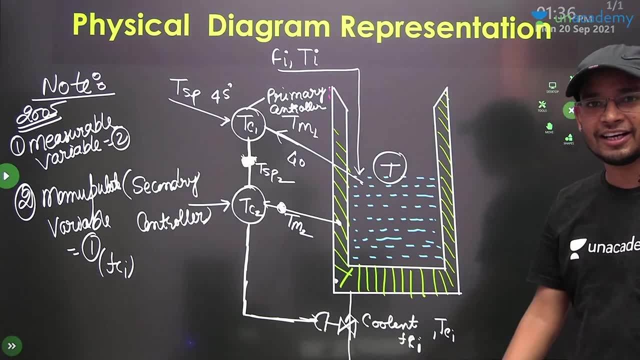 This one. No, no, no. This is not manipulated variable. This is the process flow rate. We will not manipulate this. If you manipulate this, then what will happen to your temperature? It will get disturbed In case if you manipulate this. 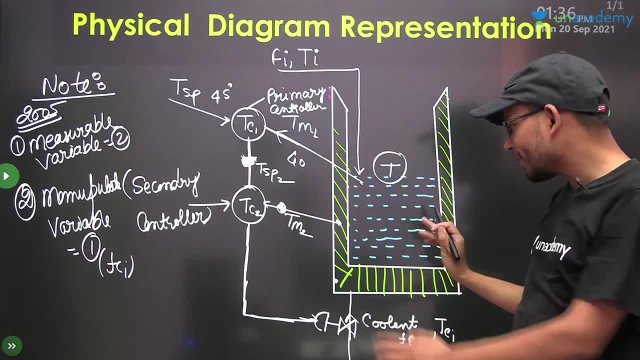 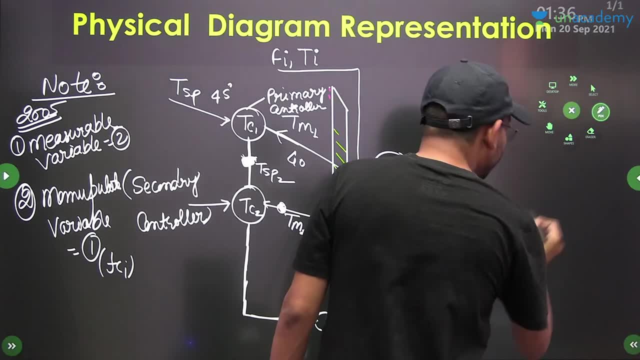 then what will happen to temperature? Input flow rate can be there. Fix it here. And what will happen to this Outlet flow rate will also be there. Where will this be going? See this, See this way: This is your flow rate fixed. 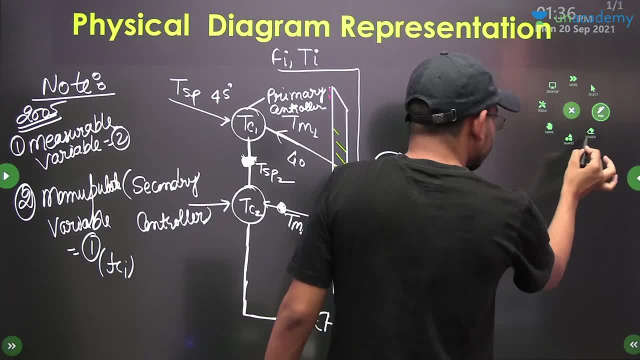 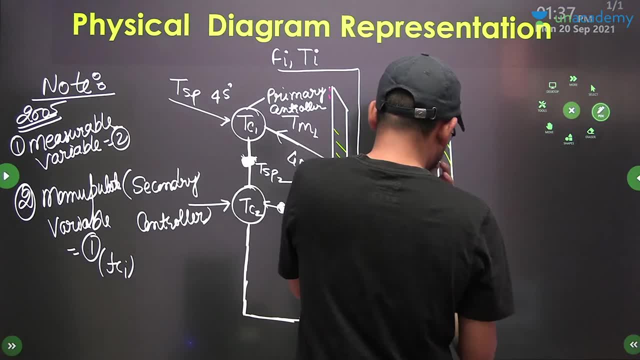 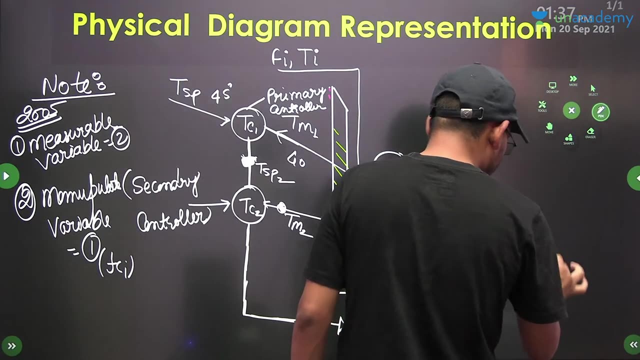 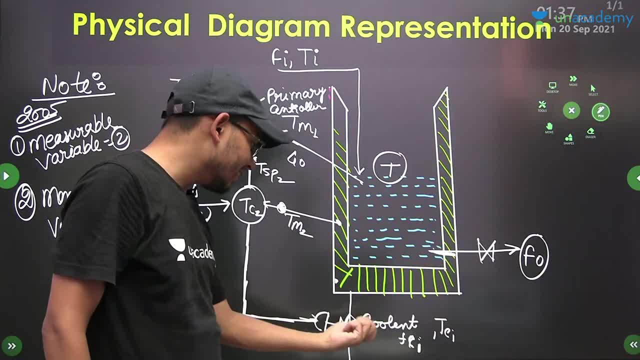 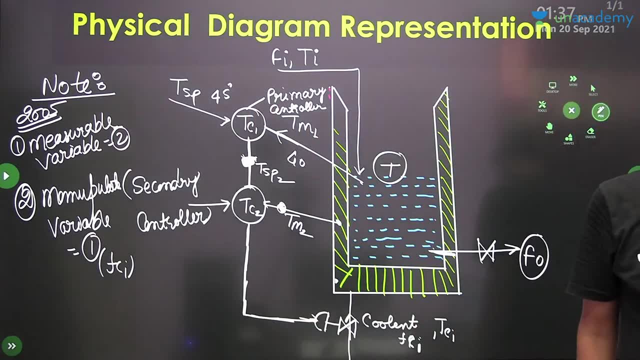 will be fixed in the reactor. It is going continuously. But what you have to do, You have to manipulate it from here. This is not manipulated variable. This is not manipulated variable. This is not manipulated variable. Who is always manipulated? The one whose coolant is going. 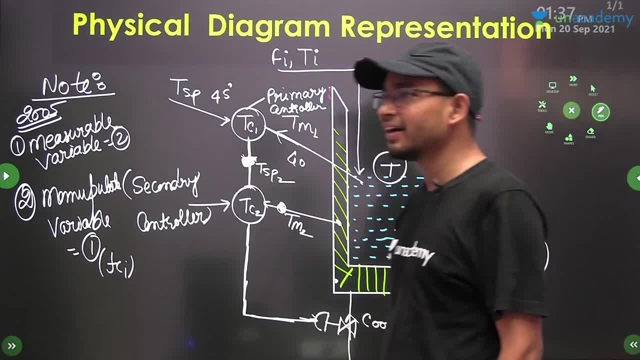 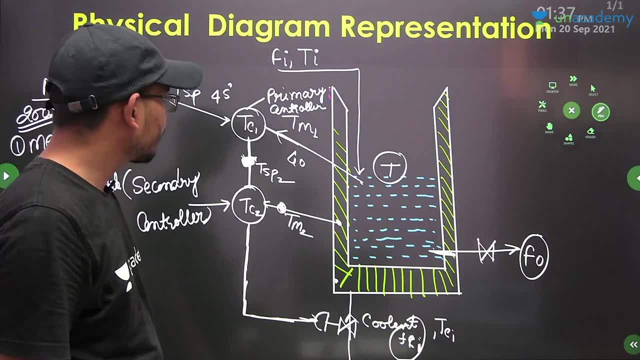 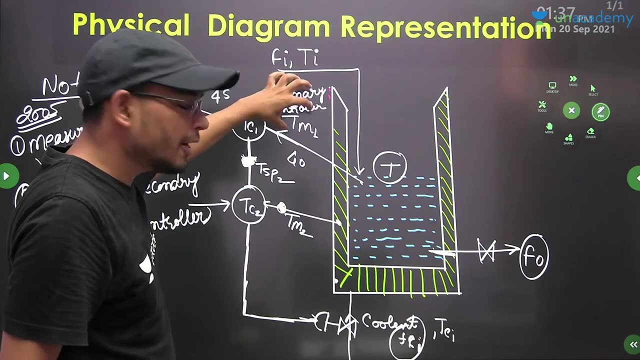 Coolant or steam is going. This is manipulated. Always keep in mind, Always keep in mind For one or two, two measured variable or one is the manipulated variable. Fine, The one which happens in the first is called primary controller. This is called secondary controller. 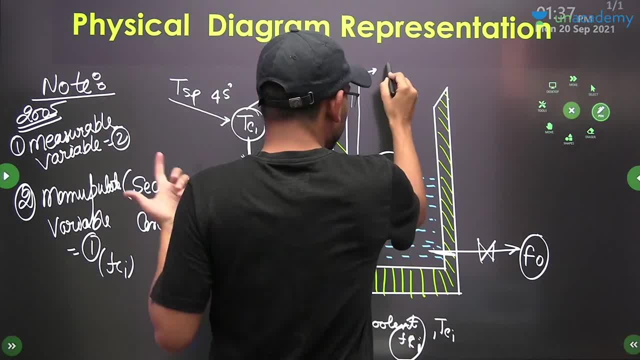 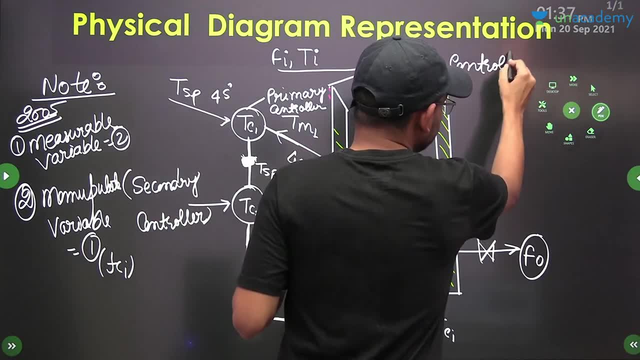 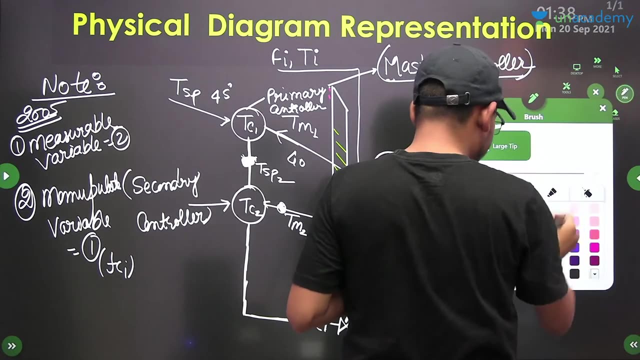 The next name called either. it is called as Master Controller, Principal Controller is also called Master controller. Tell me, why is it called Master Controller? How will you remember Master Controller? How will you remember Master Controller? Tell me, how will you remember What is the work of a master? 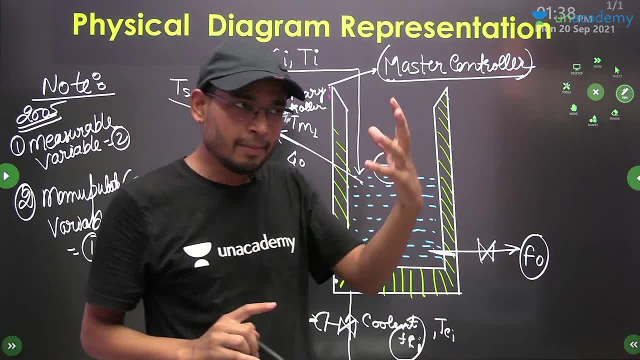 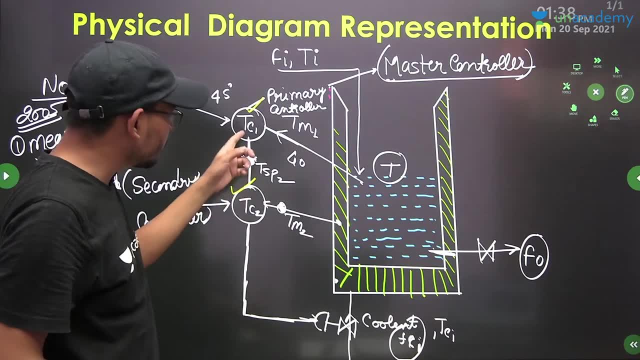 To give an order. What is the work of a master? To give an order. That, brother. I have to do this work. So what did he do? To whom did he give the order? To the secondary controller? Okay, He gave the order to the secondary controller. 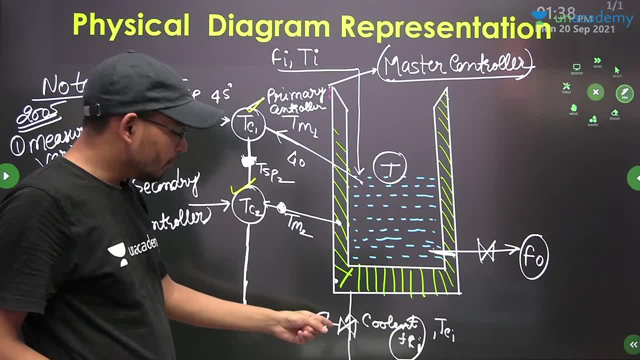 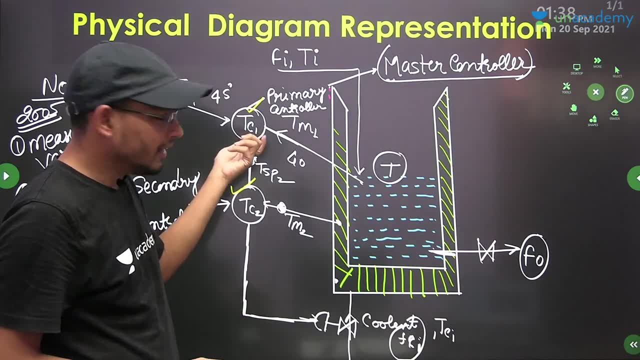 Now, according to which he has to run it. Okay, He will run according to that. What is this at the top? As you say, You don't say That your leader is this: Okay, He will give the order to his younger people. Then, what will he do? He will make the younger people work. 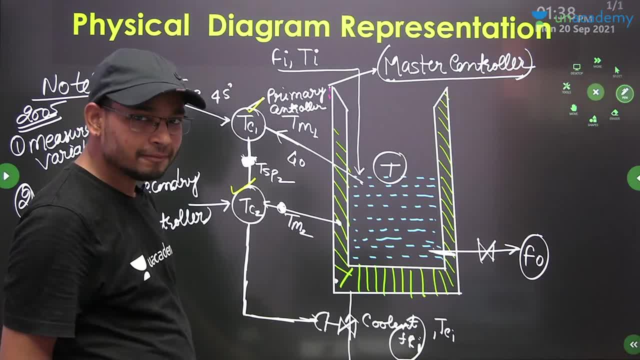 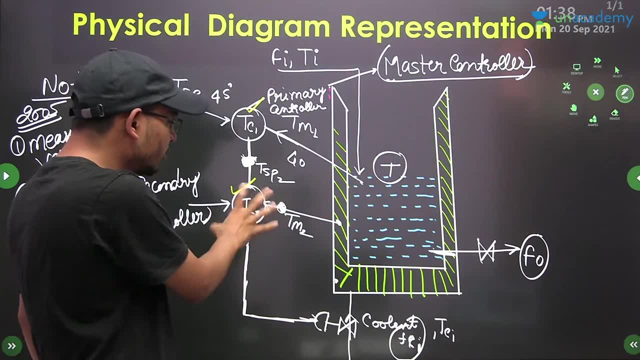 That your system will start working properly. Okay, So this is the thing. He felt that his main process Disturbed. Okay. So the first thing is: This is the secondary controller. It will work. Okay, It will not reach the primary controller. It will not reach the primary controller. It will adjust and change it. 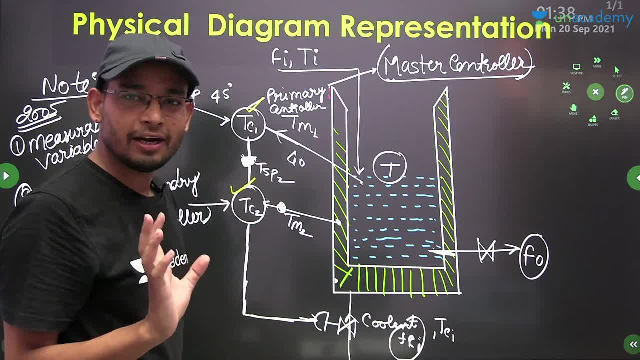 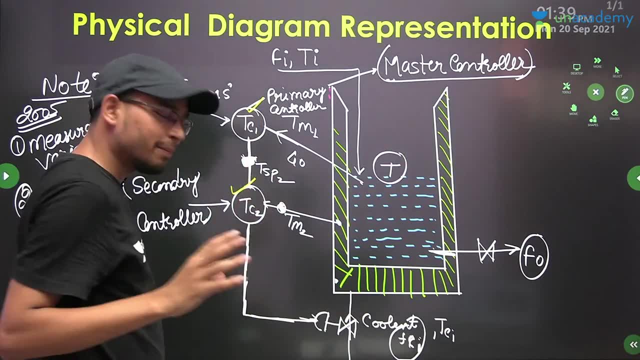 In case This process also started disturbing you. This process also started disturbing you. quickly, Then this will reach the principal. Then what will the principal say to the master? He will say: The master will disturb his students Or whoever will be The people below him. He will disturb them a little. 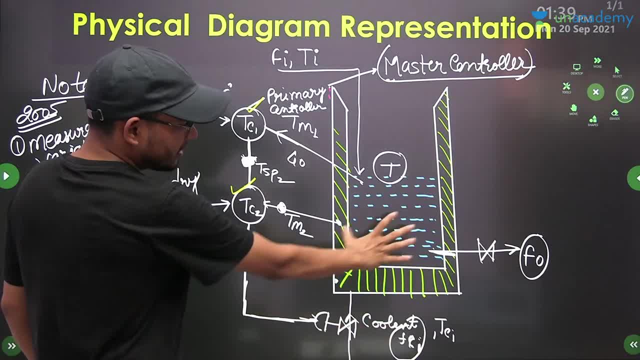 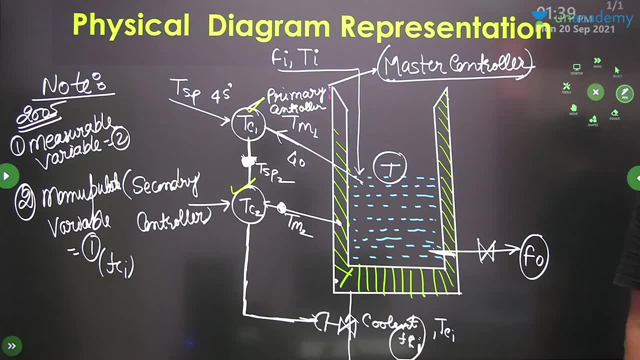 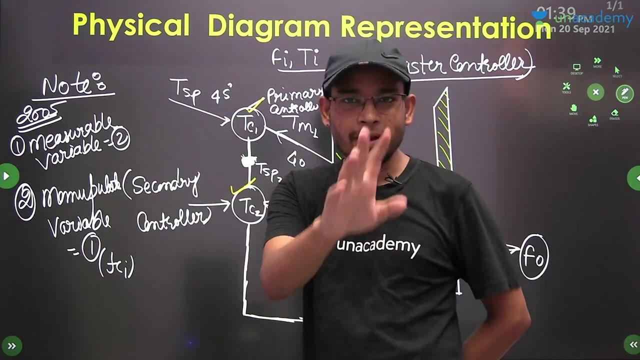 He will give them a little pain And these things will start running smoothly. Okay, So that's the thing. Understand in this way. Yes, The more controllers are installed, The more miserable Clear. So what is this? The primary controller? If you get it somewhere in your option, We call it a master controller. 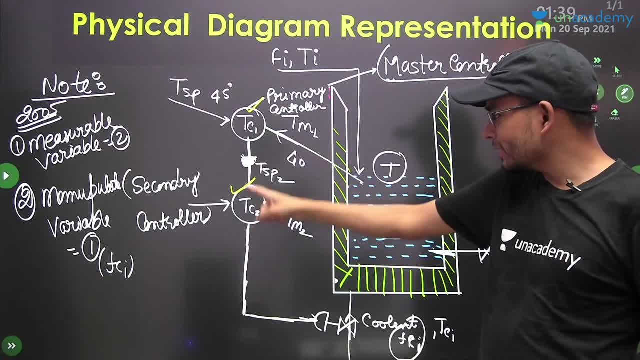 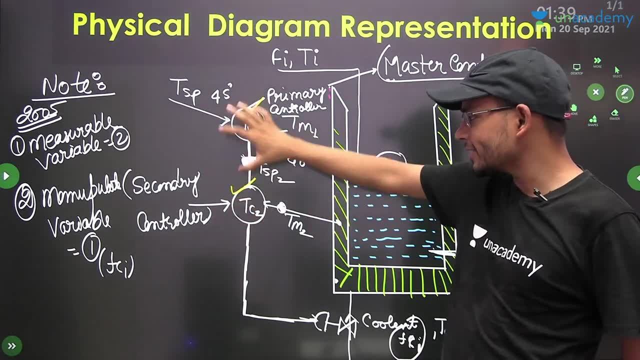 Okay. Why is the master? Because what does this say? It is called the master controller. What does this mean? This is giving the instruction of tc2. This is the secondary controller. This is what gives it Instructions And it works according to instructions. It will open or close. It will work according to the process. 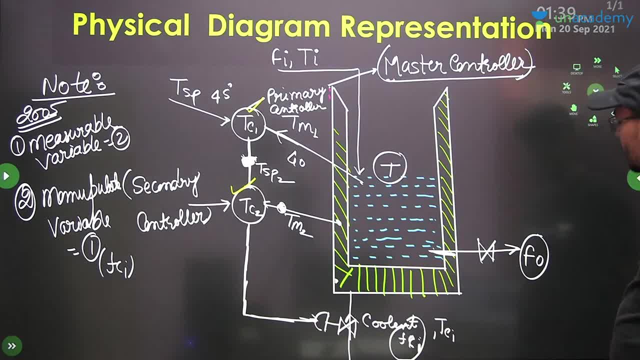 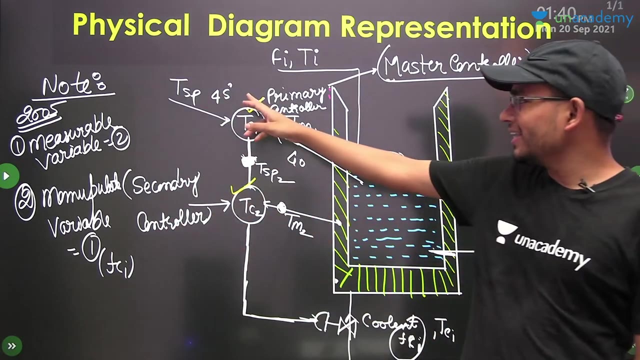 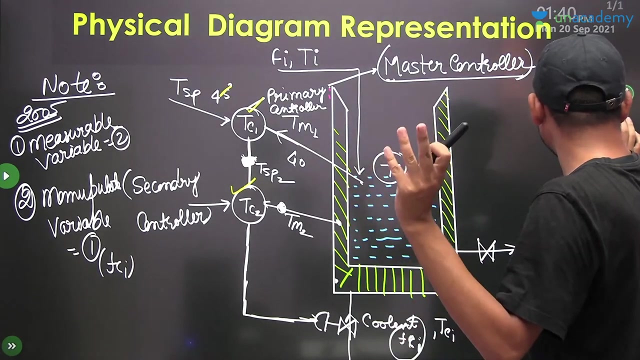 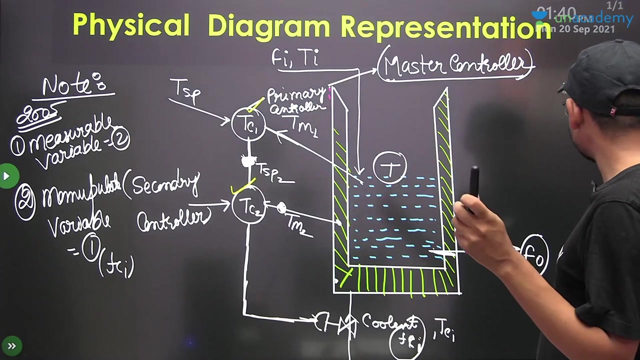 Okay. So first understand this process. Only then you will understand its block diagram. Understand the process first, All of you. This 45 degree is nothing. some people were asking: sir, 45 degree? this is nothing. I just told you like this, I just gave you an example: write it, write it, it's a good thing. even if you don't write, there is no problem. I just told you how it will work. 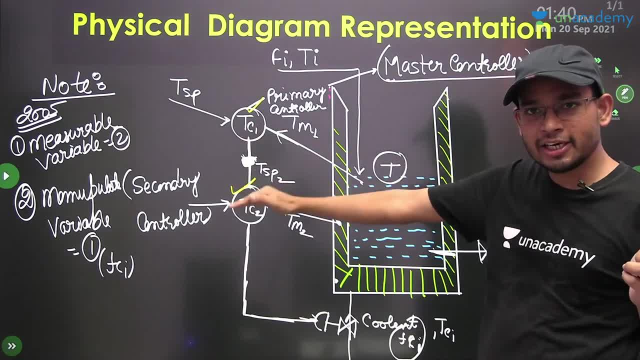 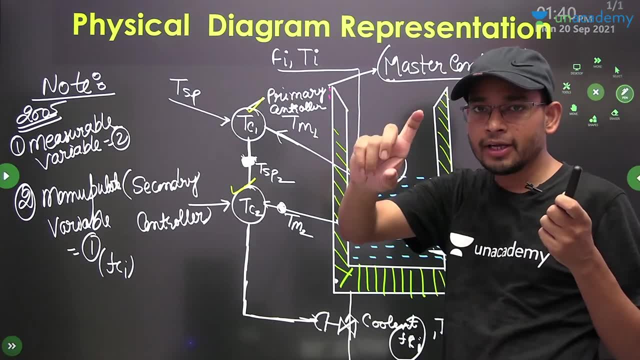 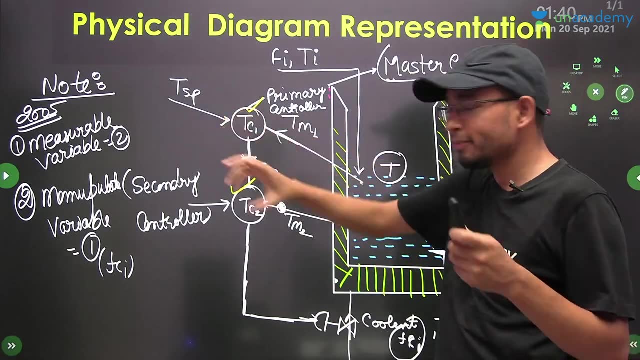 TC1 will provide the output signal increased. or what is the output signal of the controller? Output signal? this can also be in respect to the pressure. so the output signal will provide the output signal increased, so it will depend on its output. so what will it do with the measuring device and the setpoint? 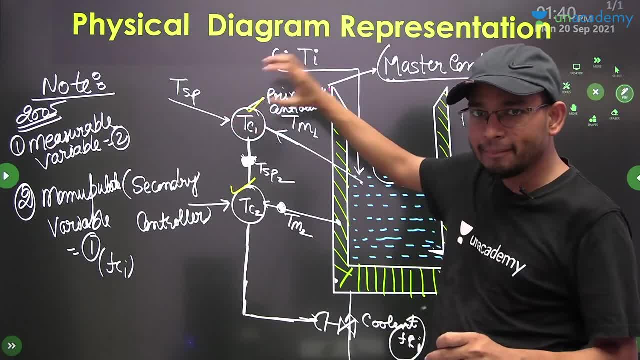 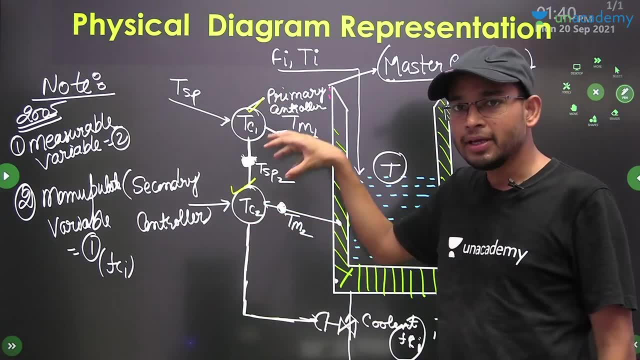 It will pick up the error. where will the error go? the error will go in the controller. the error of the controller will either be positive or negative. so, according to that, what will happen? the work of the secondary controller will be done. 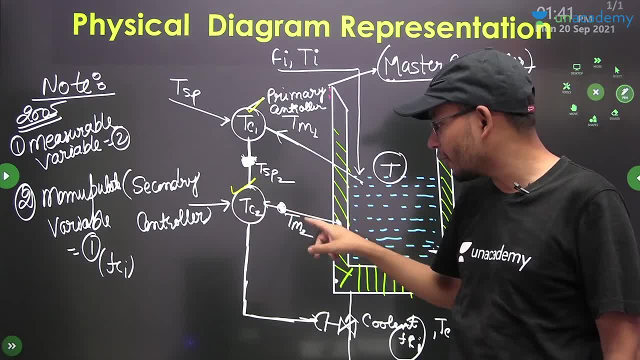 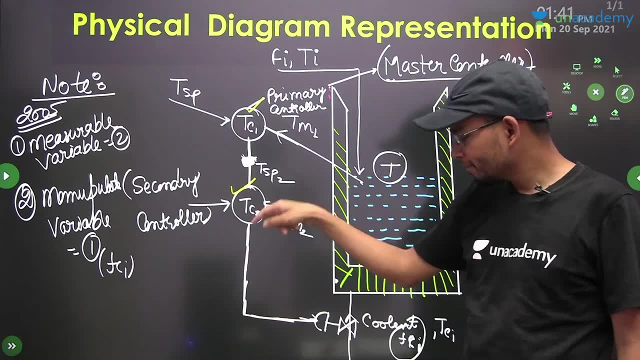 then what will be the input of the secondary controller? This setpoint which is coming, this one and this value which is coming, it will match this. then it will get this value from there. then it will go to your final controller element. sir, my doubt if coolant temperature is constant. 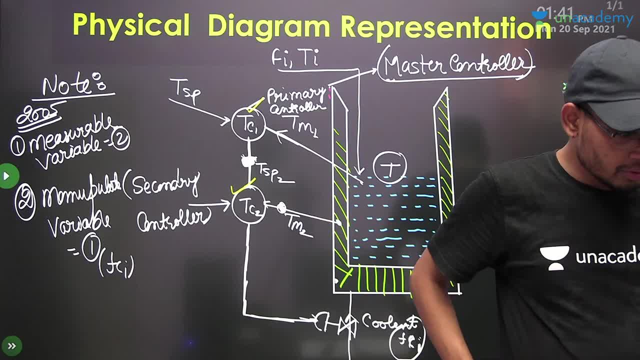 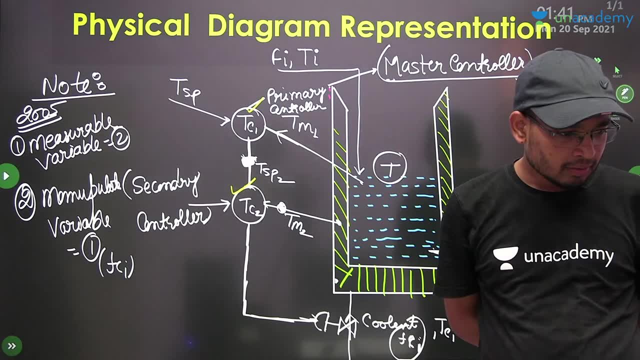 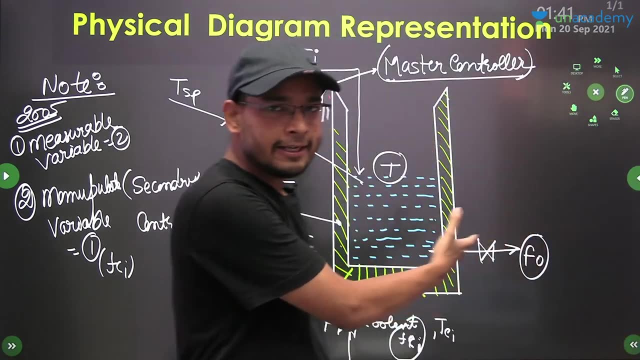 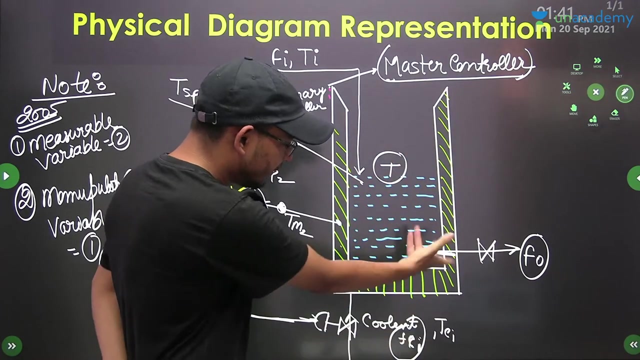 TM2 is equal to zero, then controller 2 no use. if coolant temperature is constant, coolant temperature is constant, then then if this temperature becomes constant, then you, then the meaning of its ejected will end. in case you have made this constant, then what is this? you fill it once. this does not happen. 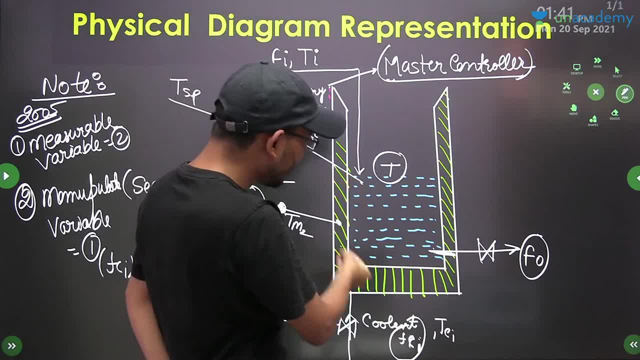 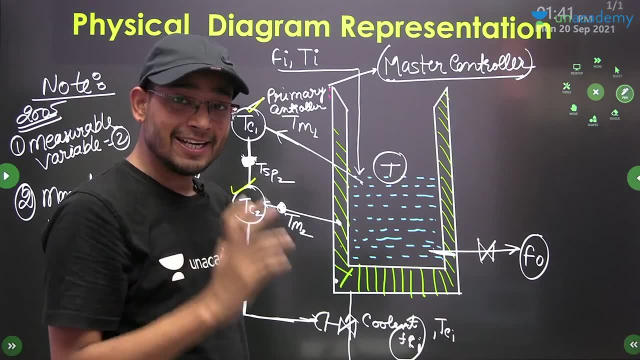 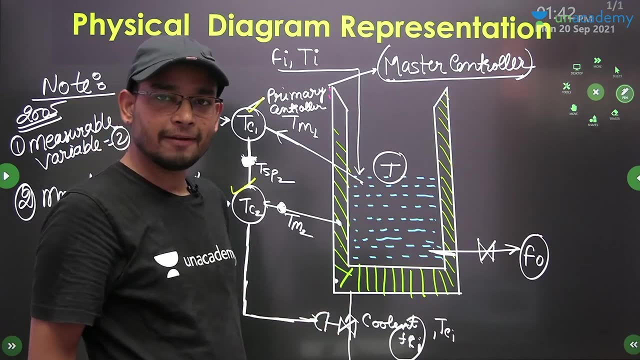 because the temperature of the reaction here will fluctuate. then automatically your temperature will fluctuate, right in case it happens at a steady state. at a steady state, okay, this temperature is fixed, then what will you do? the value that will come, then it will shake it. it will not do it after a long time. 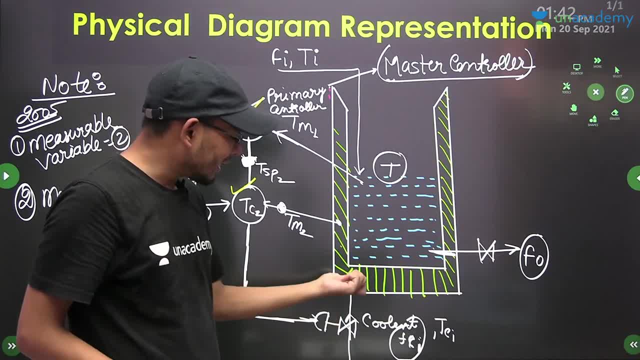 you are talking about a steady state. condition means, after a time, its temperature is fixed, its temperature is fixed. okay, then what will happen? then what will happen? it will work on its steady state, whatever error will come once it will set it. this temperature will also be fixed. this temperature will also be fixed. 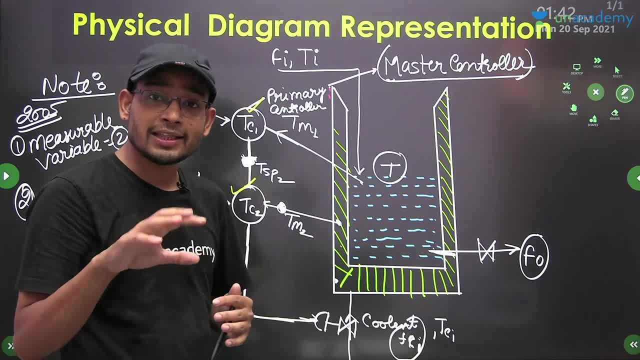 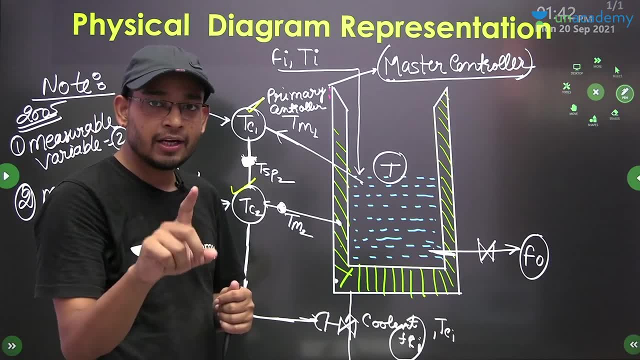 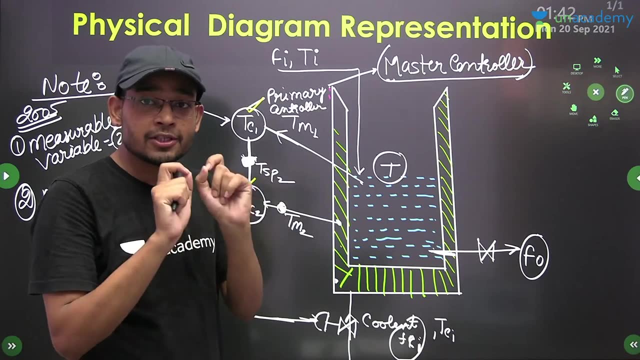 it will not fluctuate. when the controller's work happens, then your system gets disturbed. that's why the controller takes action. controller always work when your system gets disturbed. when your system gets disturbed, only then the work of controller happens. if your system is running smoothly, there is no problem. then what will happen? 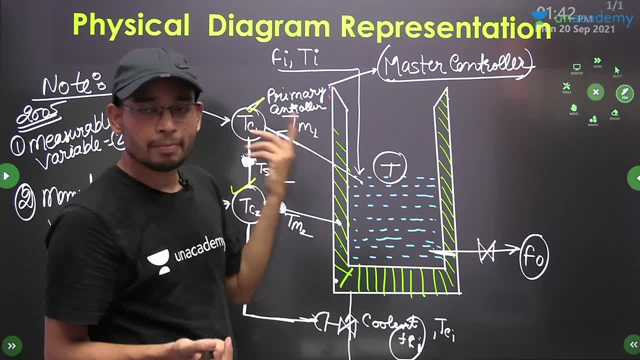 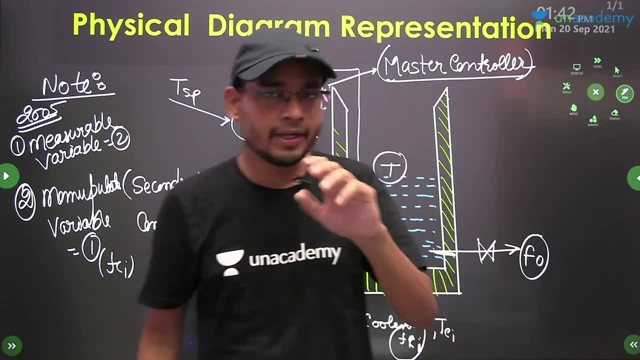 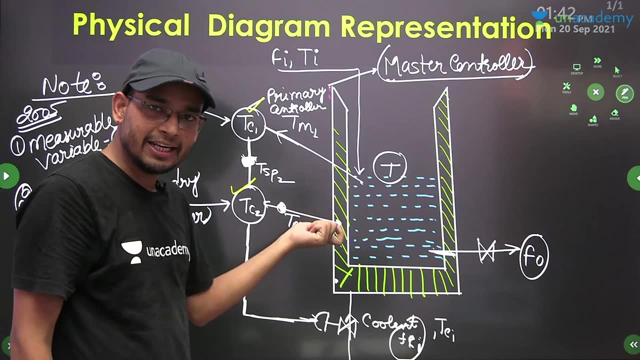 then controller will not take any action. action will not take. so what will happen? it means the process will go on, a steady state, clear: TM2 will not be zero. TM2 is not zero. TM2 having some value, TM2 having some value: 5 degree, 10 degree, 20 degree, TM2 will not be zero. 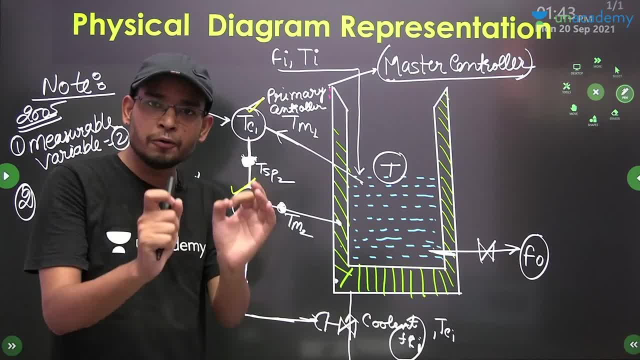 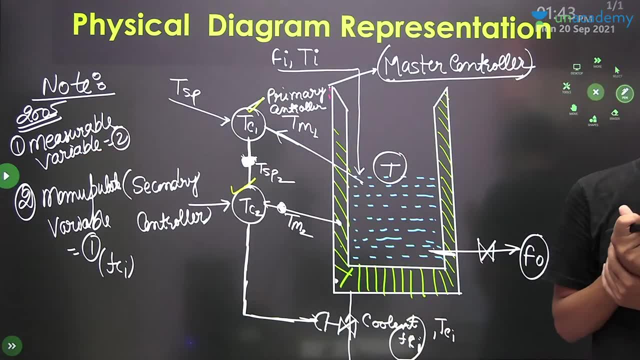 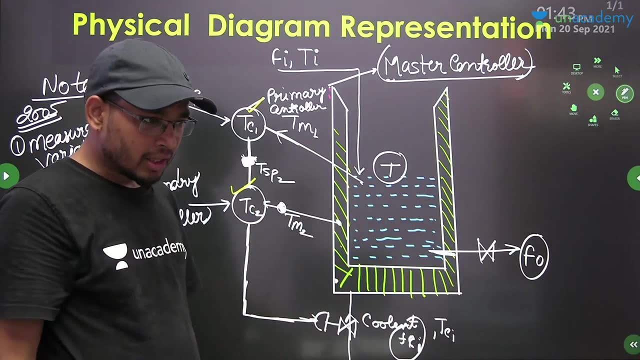 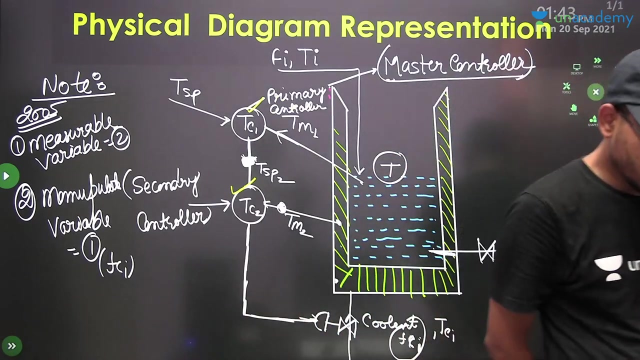 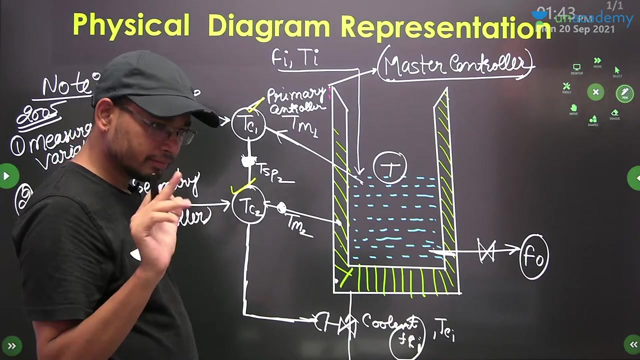 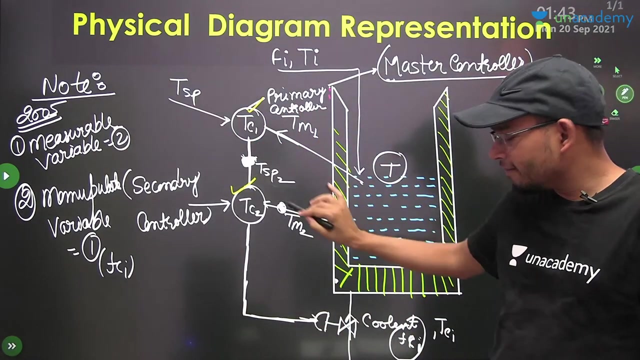 This will not be zero. There will be some value, but that value will be constant at steady state. Clear: TM2 will never be zero. This can never be zero. Okay, Okay, Clear. Your doubt is clear. Okay, There should be some deviation. Deviation will be constant. 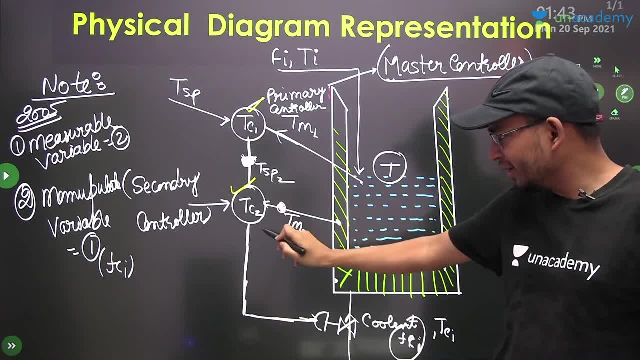 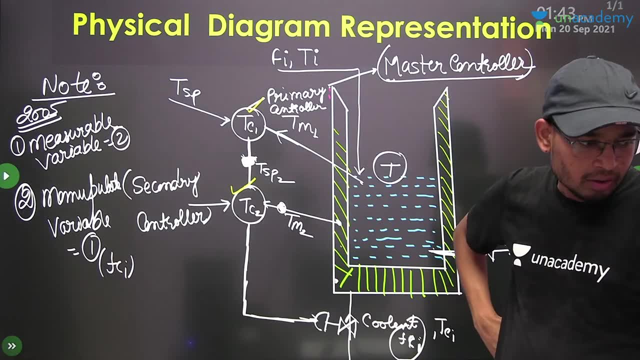 Here the value is 5, here the value is 10.. There should be deviation, but deviation is constant. Okay, Okay, Everyone understood it perfectly. I will say it once: yes, Everyone understood it properly. Okay, tell me one more thing. 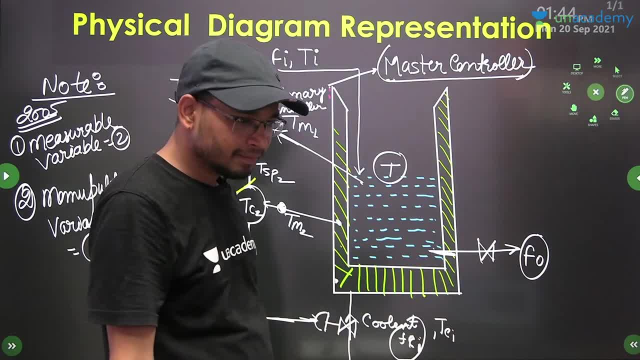 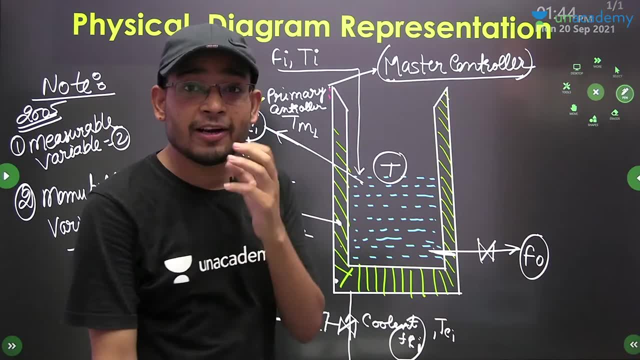 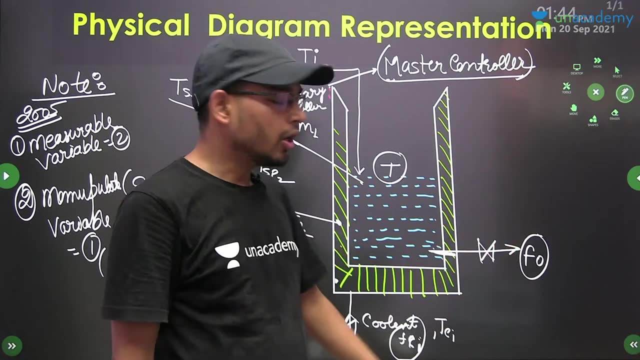 Will F0 be your manipulated variable or not? Will F0 be your manipulated variable or not? Who are manipulated variables? First, understand this. Understand the meaning of manipulated variable. Sir. tell me will it be or not, And why won't it be? 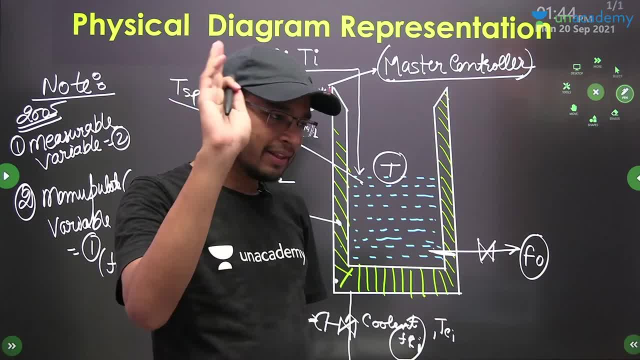 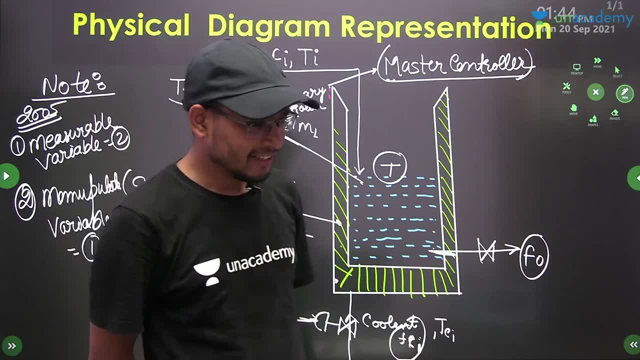 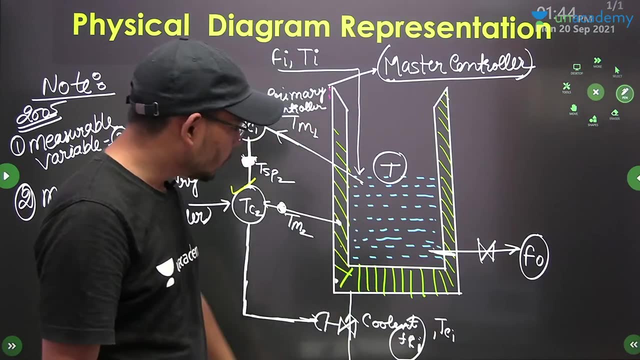 Explain this: Why won't it be? Okay, it won't be, But why won't it be? Why this is not manipulated variable? Why, Okay, you agreed that it won't be, But why won't it be? Tell me this reason. 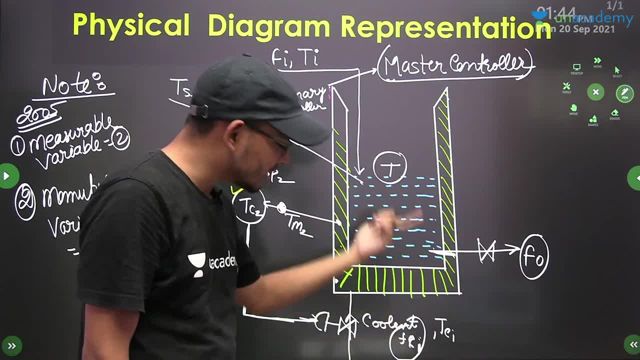 Suppose you have reached the interview of Bark. They made it and gave it to you. Now they will ask you: sir, you are changing the flow rate of this manipulated variable. You can change this also. right, You can change this also. 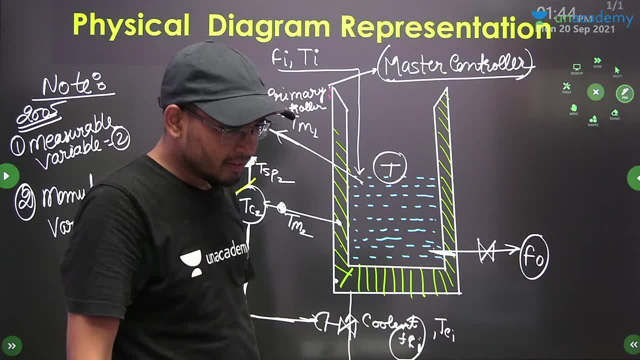 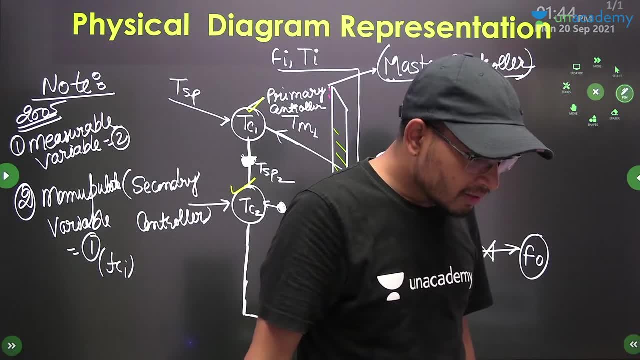 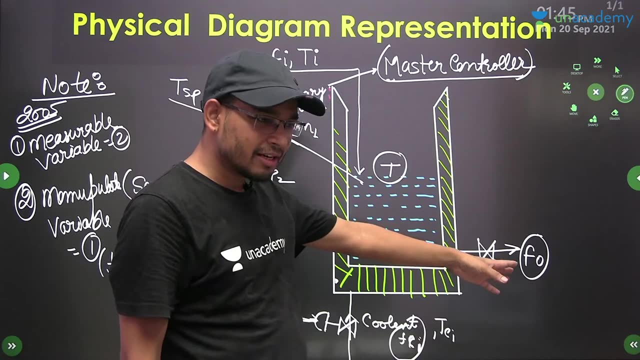 But why this is not maintained variable? Why this won't be changed in the temperature. You will increase or decrease this, but the temperature won't reduce to its flow rate. Will it change in the temperature? But you are not giving the exact answer. 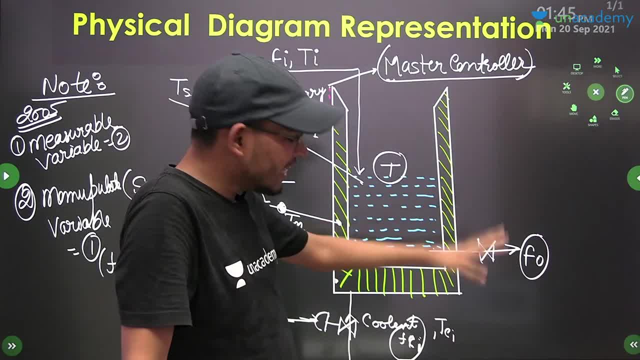 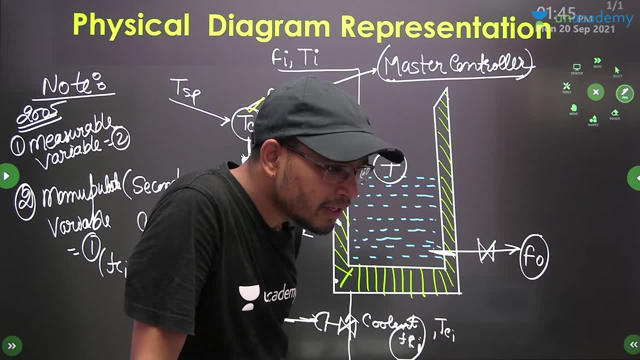 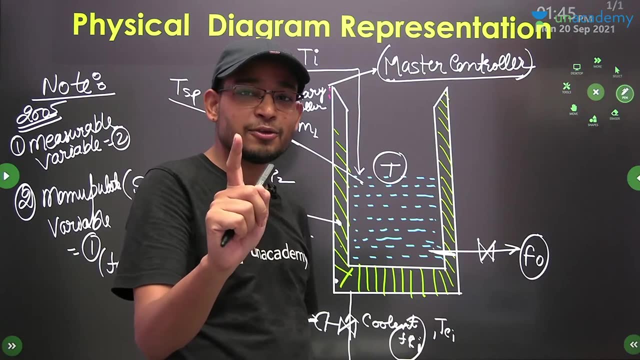 Will this change in the temperature, sir? Will this change in the temperature, sir? Yes, sir, Because every time the system gets disturbed, it will increase the follow. Listen carefully, understand the concept very carefully. don't ask anyone who is a leader in your class. understand it very well. 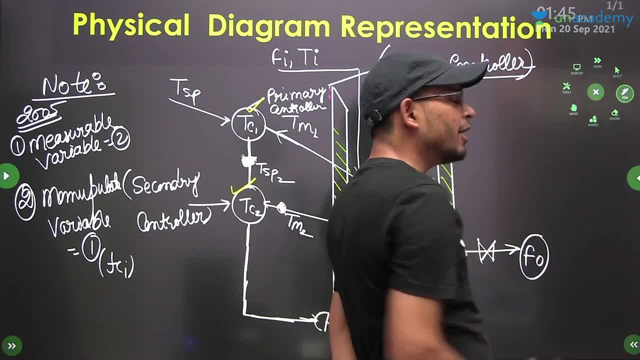 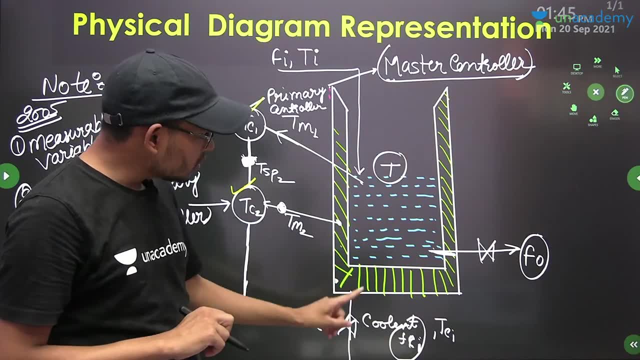 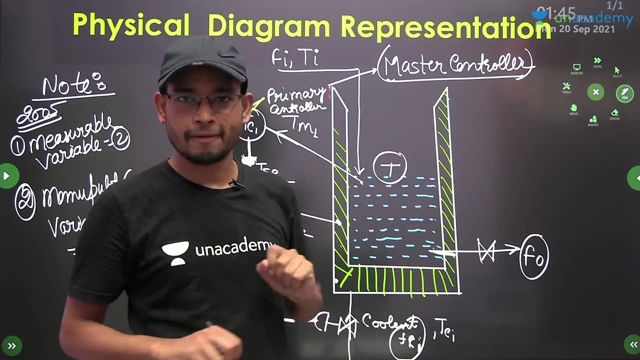 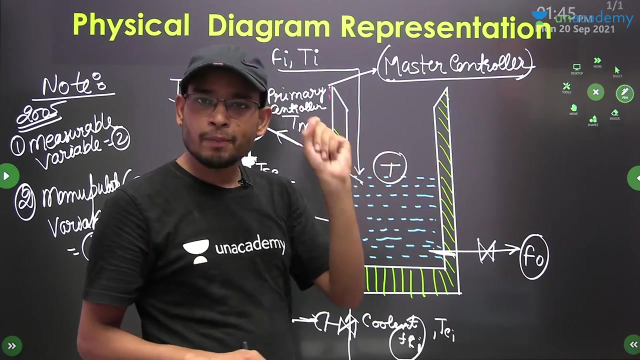 It means that we call the manipulated variable the variable which is directly attached to the controller, Those variables which are attaching directly with the controller. but this variable and this variable is not attached with the controller. It is not attached with the controller. that is why this will not be called a manipulated variable. 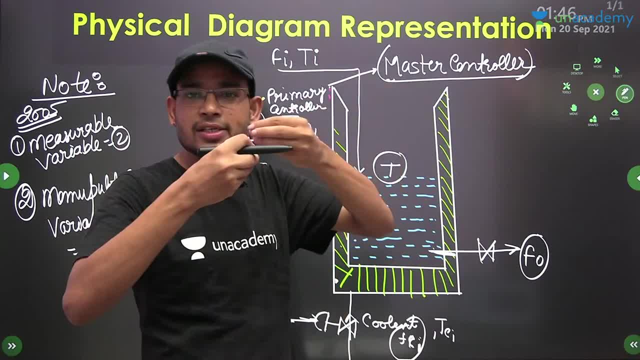 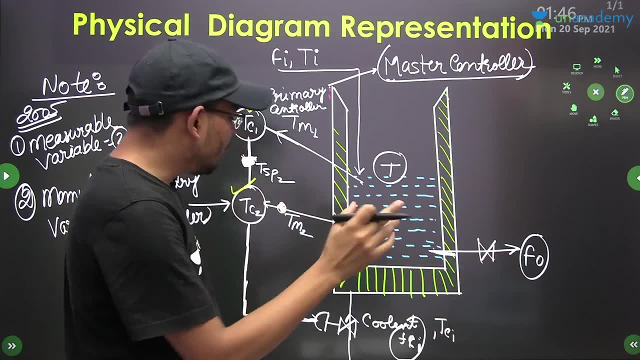 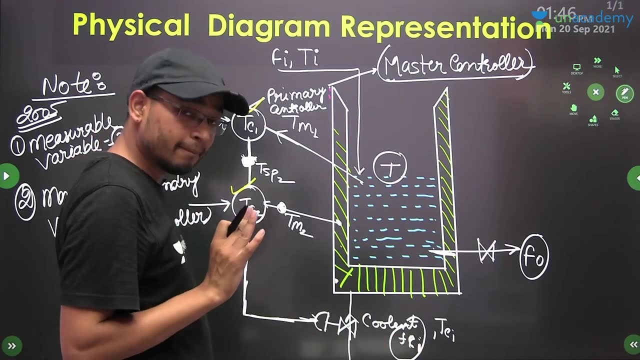 This will not be a manipulated variable because it has nothing to do with the controller. It will not open automatically. it will not be automatically closed. What is a manipulated variable? This? This variable is directly attached to the controller. What will the controller do automatically? 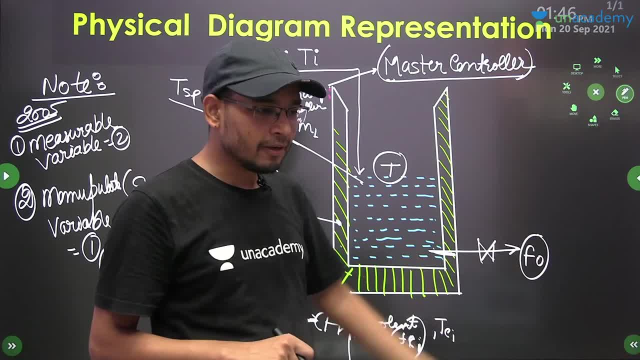 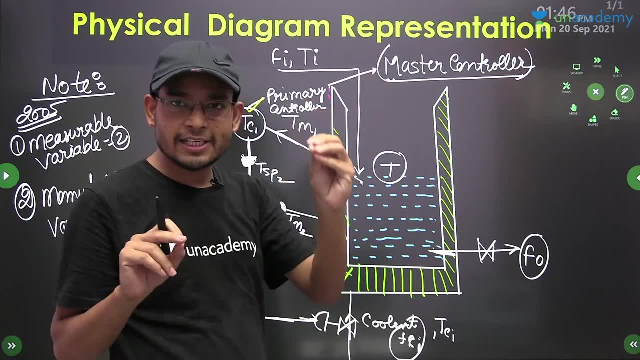 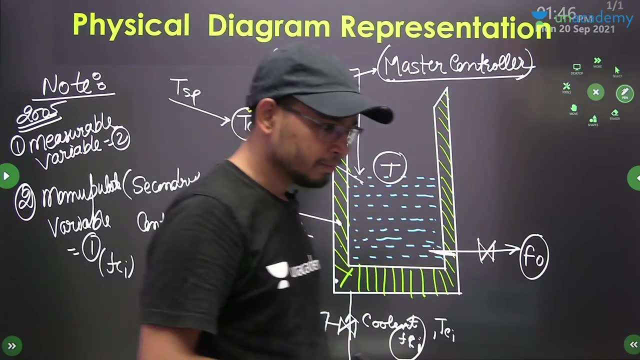 It will take its action. it will open automatically. it will not be closed. This is not directly attached with the controller. So those variables which are not attached with the directly controller, those variables will not be called a manipulated variable. Write this in your own language. 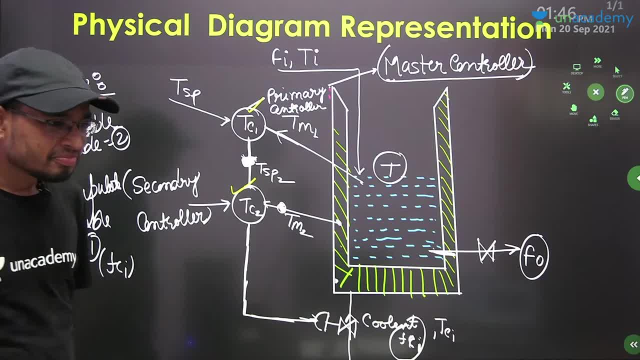 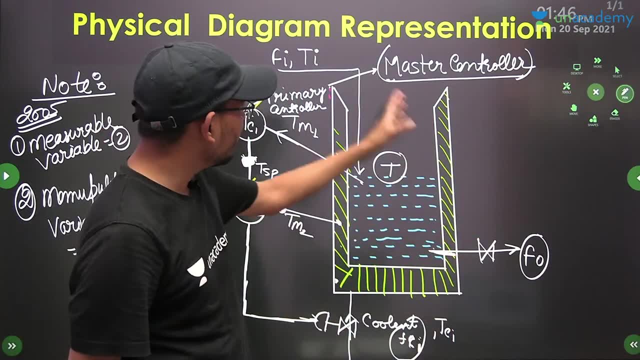 This answer was not right for anyone. This answer was not right for anyone. This answer was not given by anyone. This answer was not given by anyone. Hmm, Everyone understood the matter ahead: Why this is not a manipulated variable, Why this is not a manipulated variable. 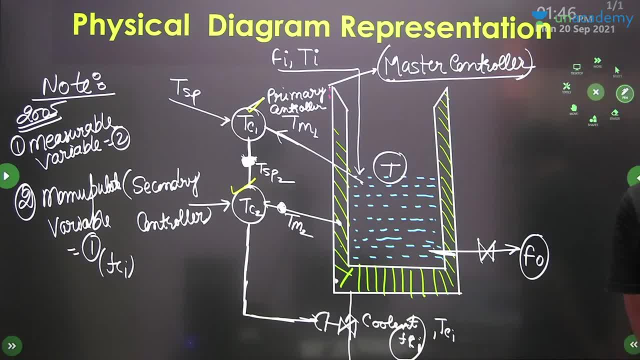 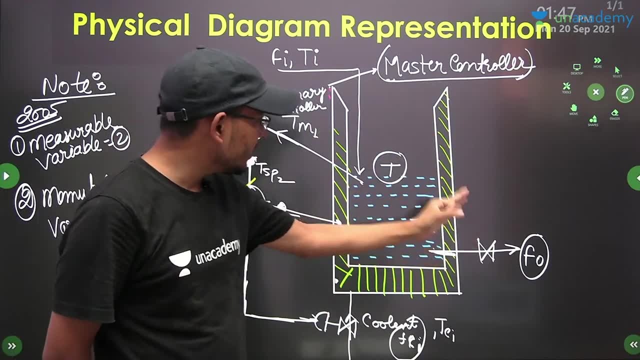 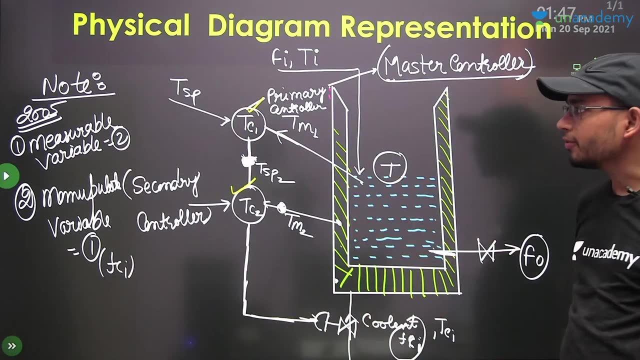 You will understand this after reading a lot of books Measuring it automatically. Yes, Okay, Everyone understood the matter ahead. So why this is not called a manipulated variable? This variable is not directly attached to the controller, so this is the concept. note it. it will be very useful in the interview. 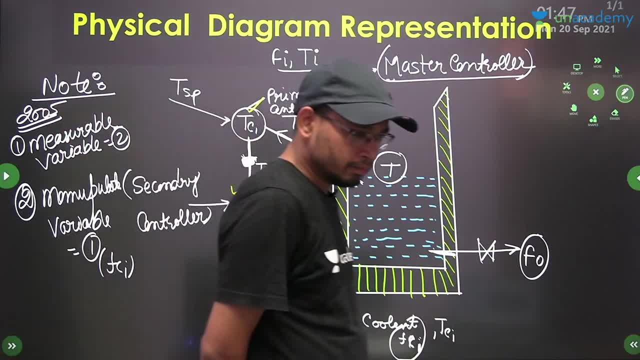 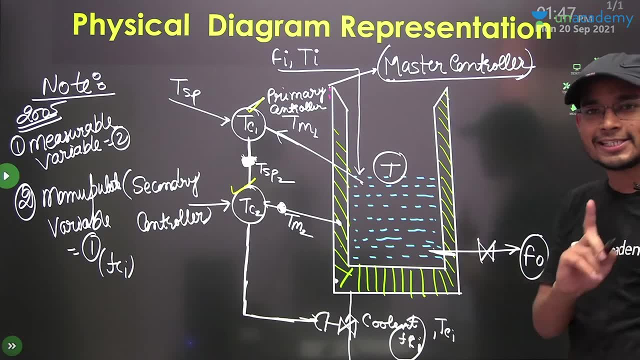 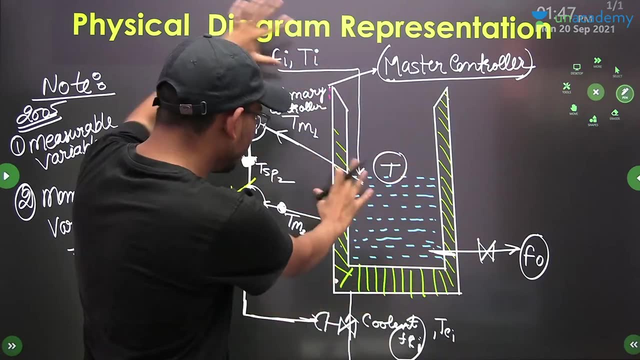 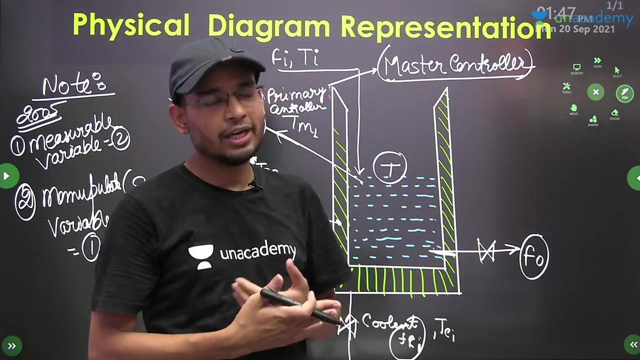 yes, in case, what will happen? this too will be attached to the controller. but this does not happen. this too will be attached to the controller. actually, this diagram is the actual diagram. this too will be attached to the controller. then this too will be a manipulated variable. 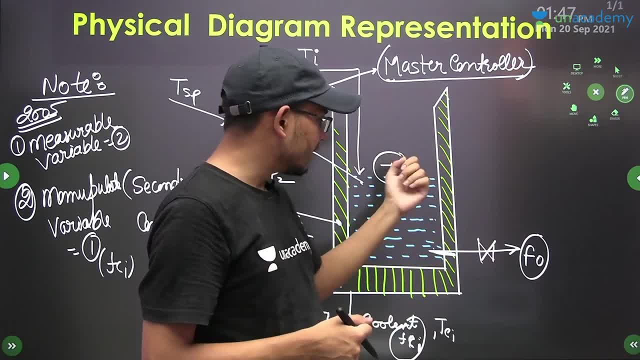 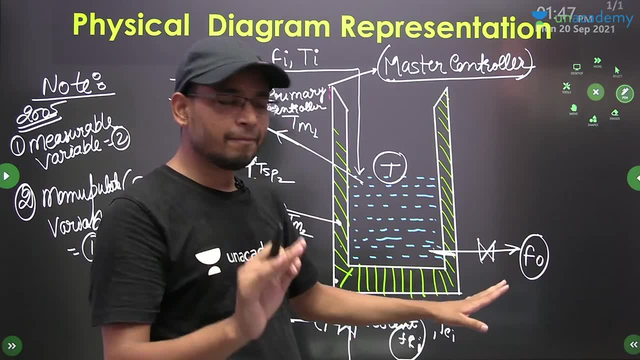 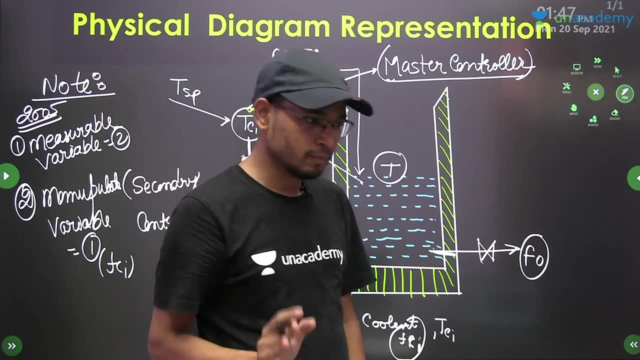 but this is not done. the controller never controls the flow rate. the controller always controls the flow rate of the coolant. in case this is also done, then the literature says that all the variables attached to the controller are directly manipulated variables. just understand this in one line. 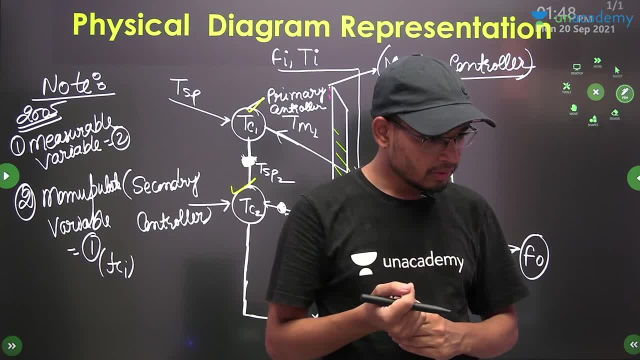 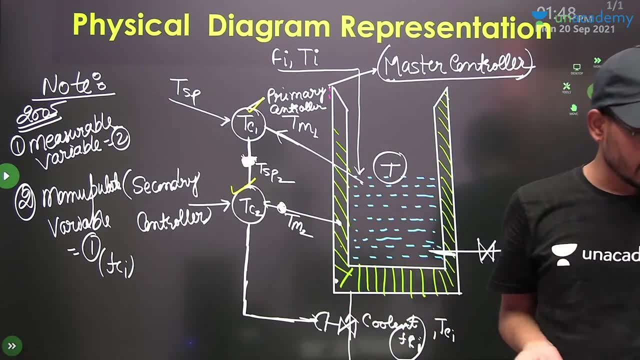 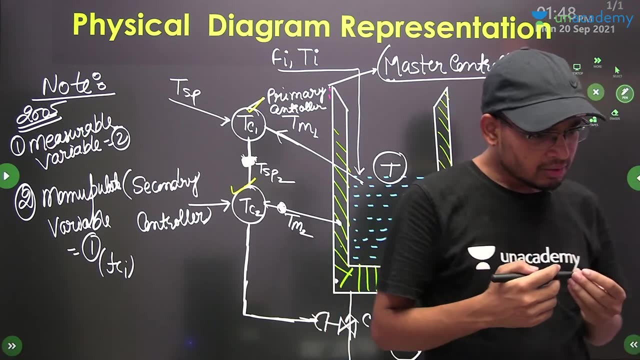 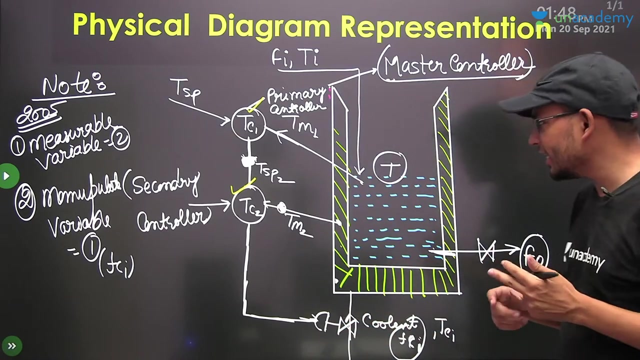 sir, what is directly attached can happen. yes, this is directly attached to the controller. this is a manipulated variable and it is not necessary that what is directly attached will be manipulated. these two things, no, no, no, you did talk about this. what does it mean? this is not attached. this is not attached to the controller. 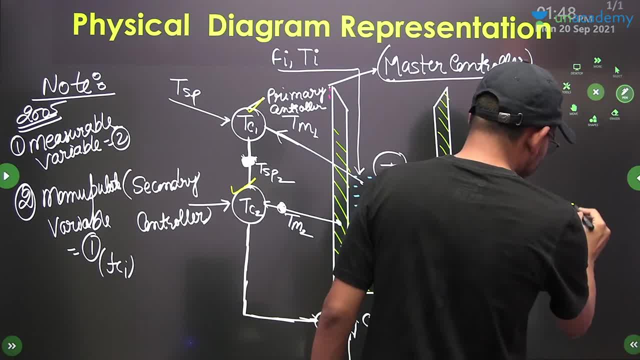 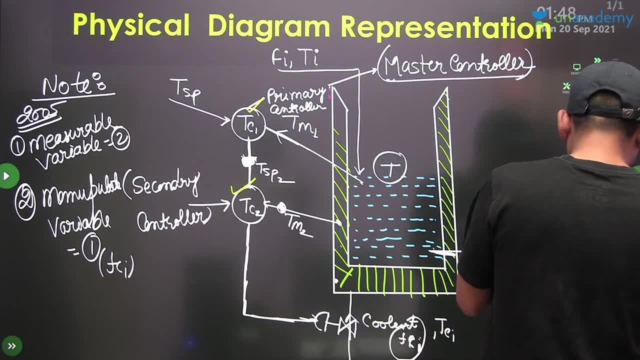 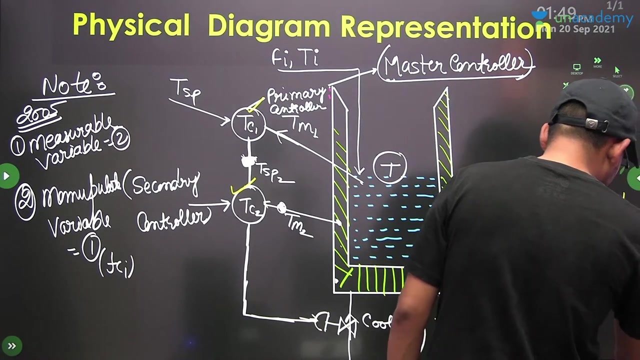 this is not attached to the controller. this is not attached. this is not. yes, write it again with: with controller. that is why this is: this is not manipulated variable. that is why this is: this is not manipulated variable. this is not manipulated variable. 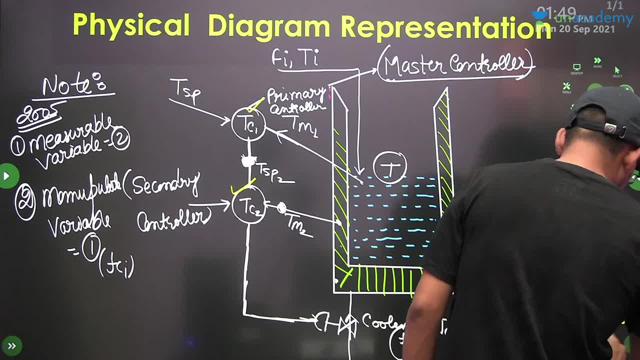 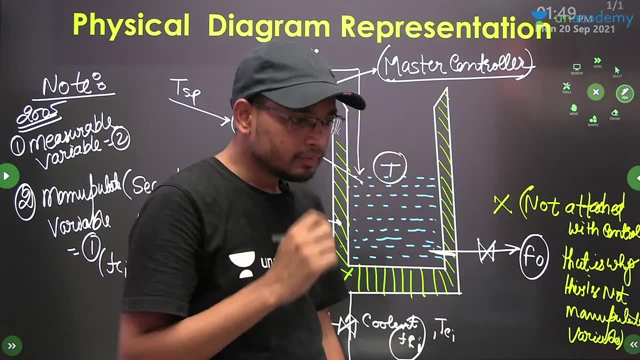 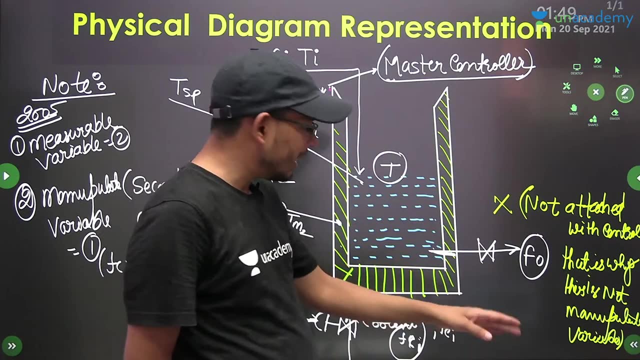 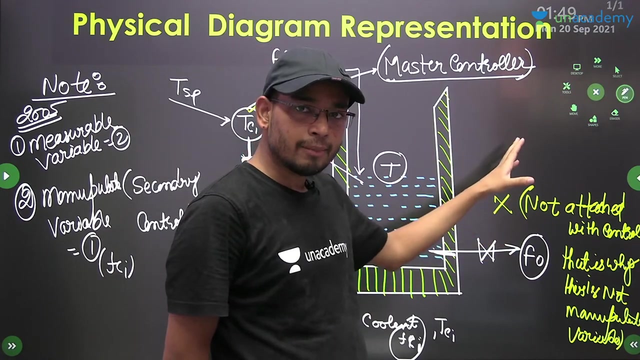 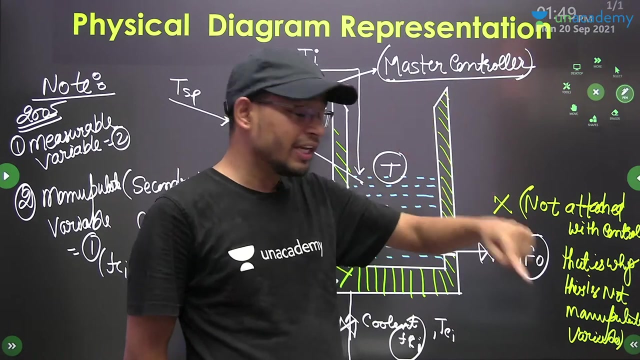 yes, F0 is there, because what happens there is that F0 is connected to your controller. okay, F0 will be connected to your controller. then it will become a manipulated variable, okay. okay, If this is not attached with the controller, It happens there because it is connected to the controller. 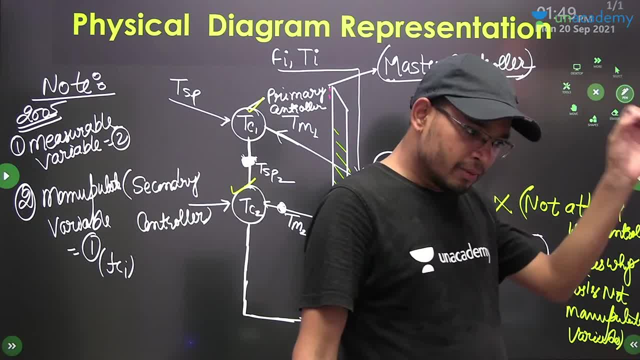 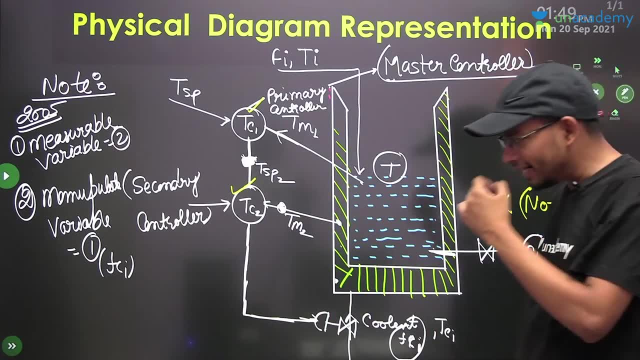 Sir, I totally understand. Yes, Veeran, Yes, Varinda Maheshwari, Absolutely correct, The one which is attached. we will call it simple Manipulated variable. This question is sometimes asked to you: Why this is not there and why this is not there. 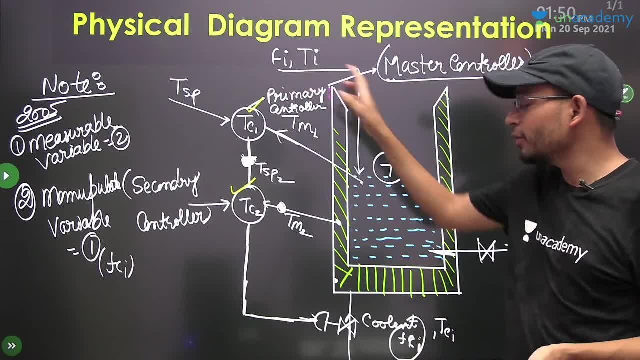 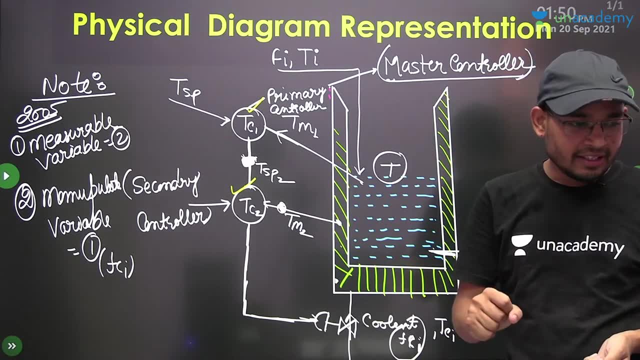 But we don't think, you know, We don't think why this is not there. We don't even get the answer to this question. We don't even get the answer to this question. This question is not written in any book in such an easy way. You will keep reading the book. 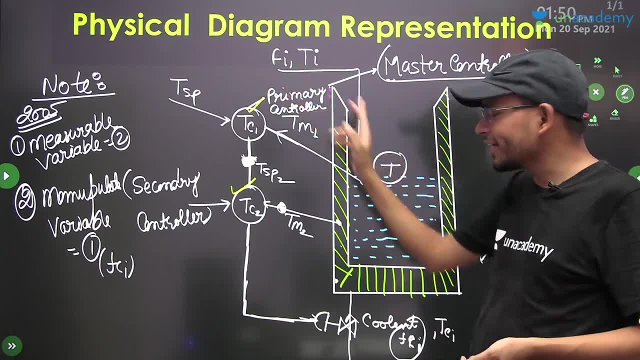 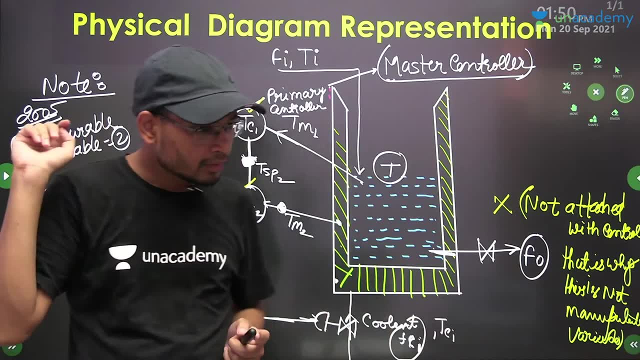 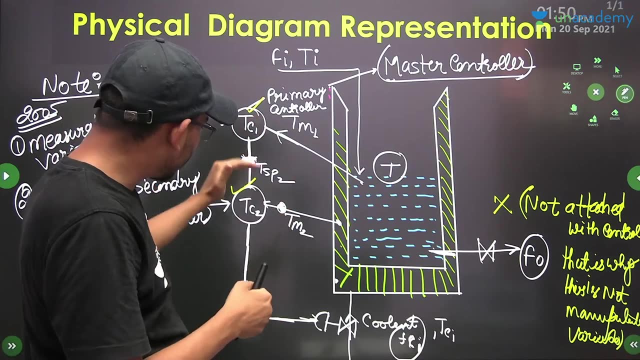 But you will read the entire theory from 3 to 4, But you will not get the clue to this. Okay, You will not get the clue to this. So, this physical representation, You must have understood properly, Each and everything. What is the primary controller? What is the secondary controller? 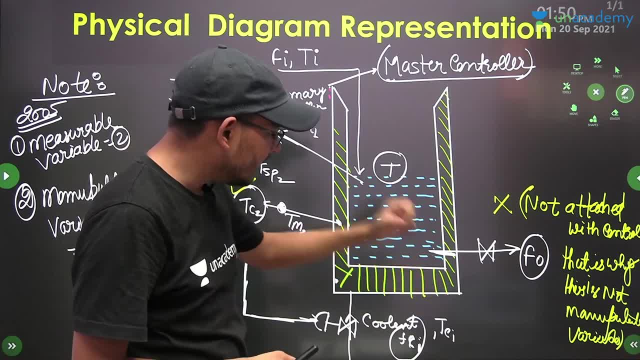 What is the error? How is the coolant working? What is the control? What is the temperature? What is the temperature? What is the FCI? What is the F0?? Everything is here. What is the manipulated variable? What is the measurable variable? 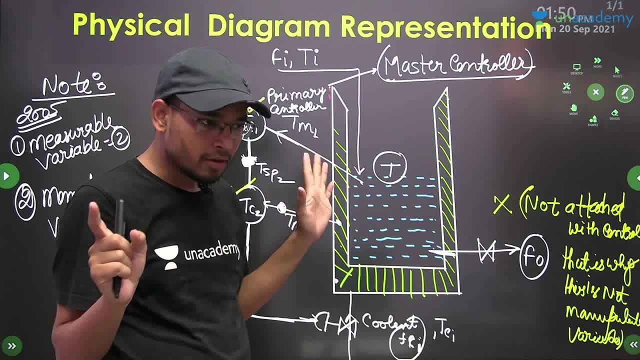 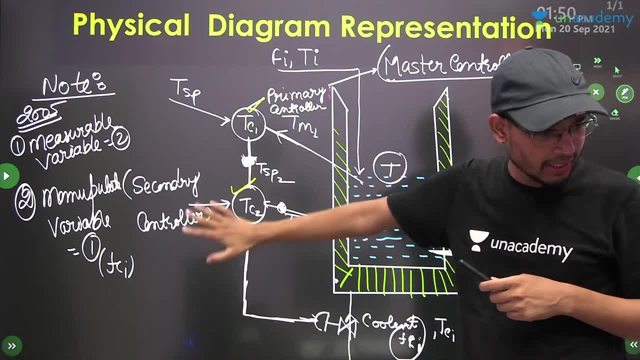 This much you have to understand from this diagram, Which I had to explain. Now come to its block diagram. Now we will put this. Everyone understood the whole thing. Okay, Now we will put the block diagram. Now we will talk about whose Block diagram. Come on, brother. 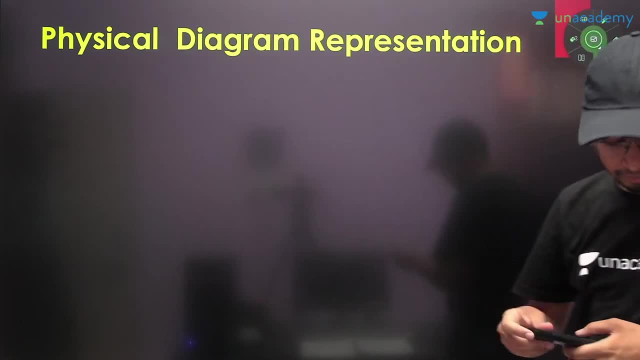 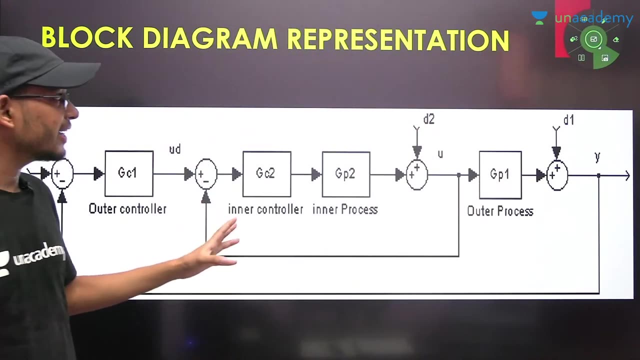 Let's talk about the block diagram. Let's put the block diagram. Let's put the block diagram. Now, everyone will put the heading Block diagram representation. Let's put the heading. Let's put the heading Block diagram representation. However, listen to it. Once you understand the thing- This too, you will understand. 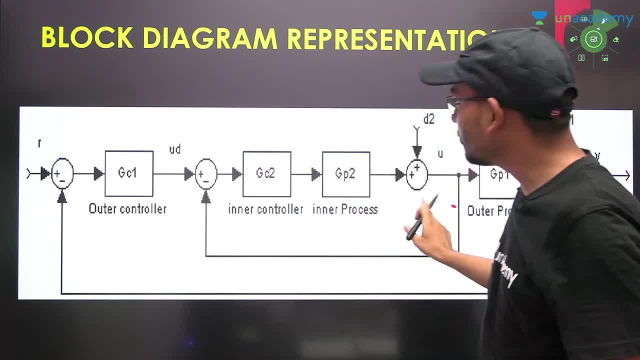 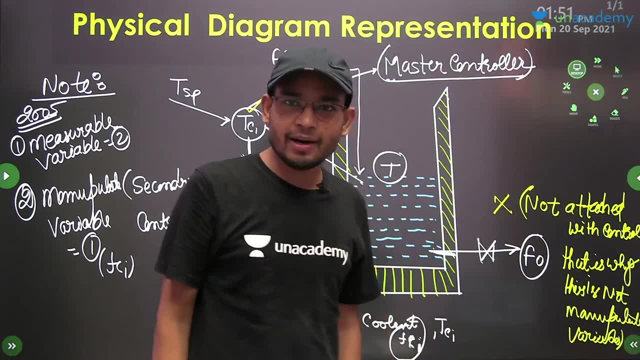 Tell you guys One minute. Let me show this, Then the work will be easy for you. Everyone say this Self. Will everyone make a block diagram of this? Will everyone make a block diagram of this? Everyone Think a little. Think a little. Will you make your own block diagram? 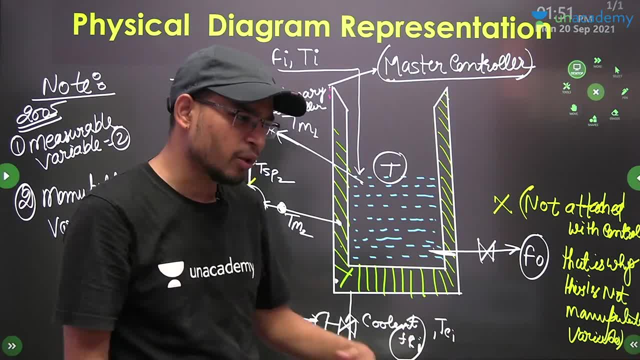 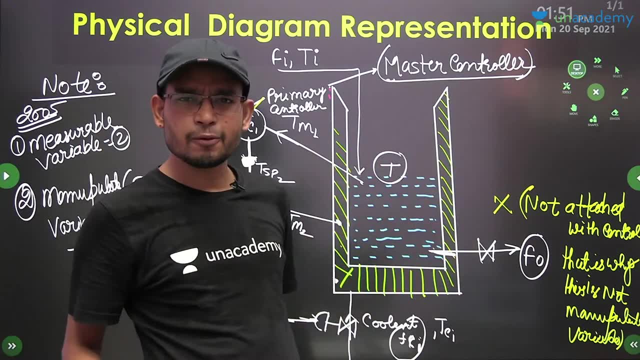 If you are asked to make your own block diagram, Will you make it? Just try it once roughly with your hands, Then it will be fun. Everyone try making with your hands, Then when I will tell you You will get clear Quickly. you have 1 minute time. 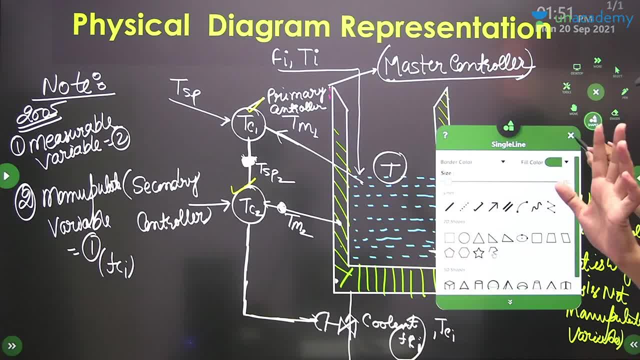 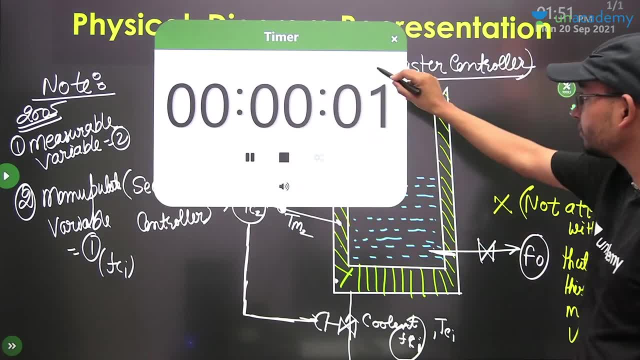 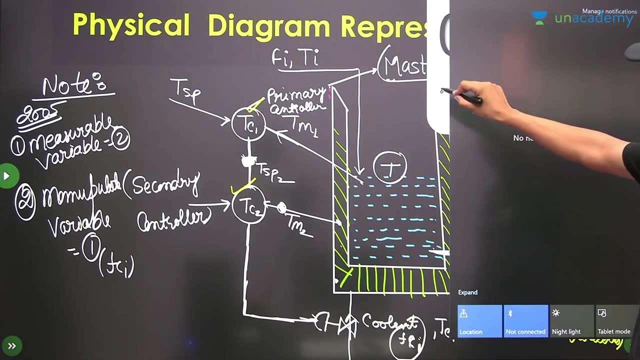 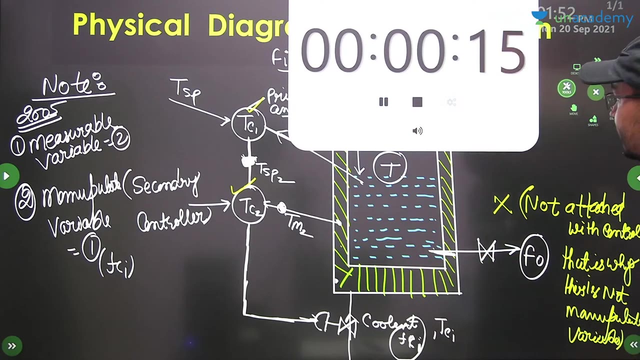 You have 1 minute time. Try making it with your rough hands. I am giving you a minute's time. try to make it. put it anywhere. you will have a figure. you will have a figure. what will you see from the board? 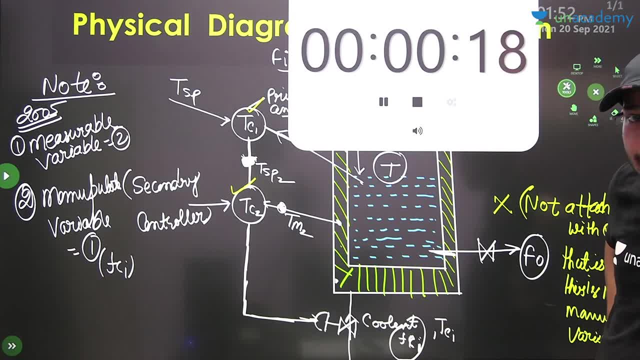 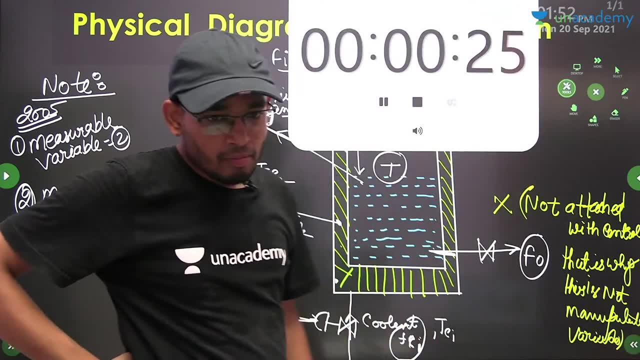 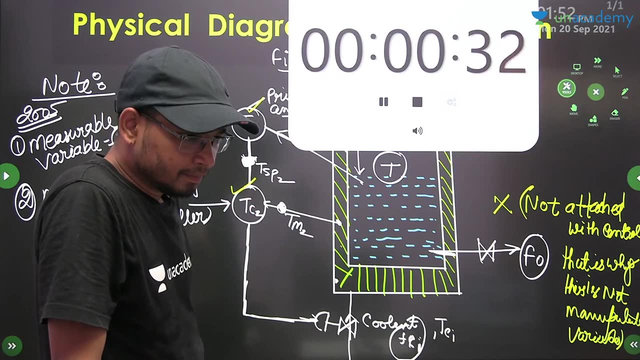 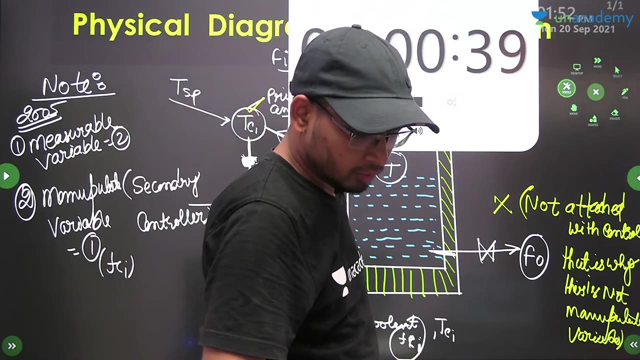 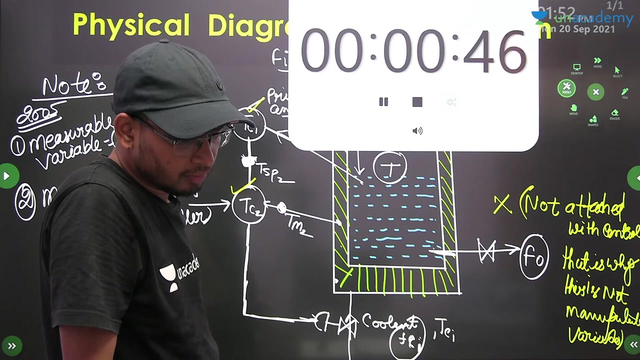 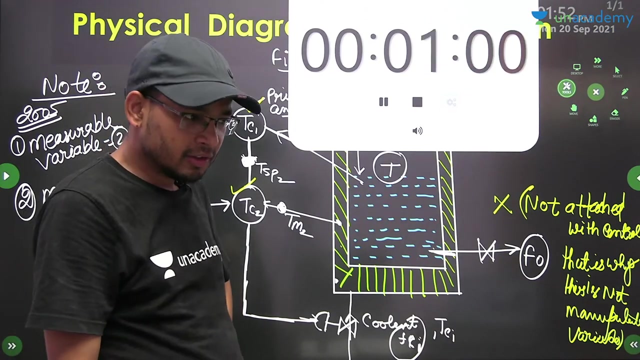 try it all. we have to make it in a minute, no matter how dirty you have to make it. make it quickly, then I will tell you, but then it will be more clear. done. do you need more time? do you want some more time? 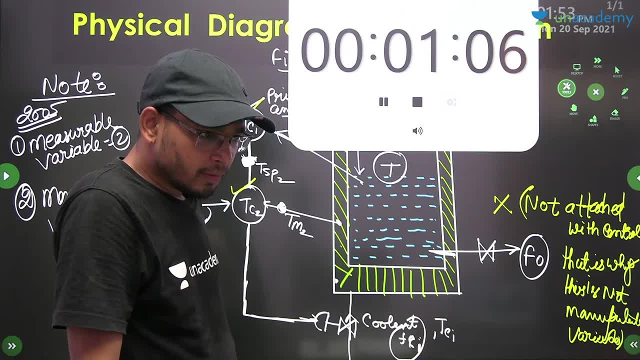 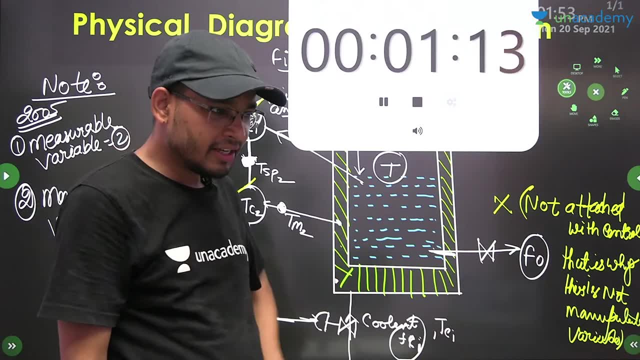 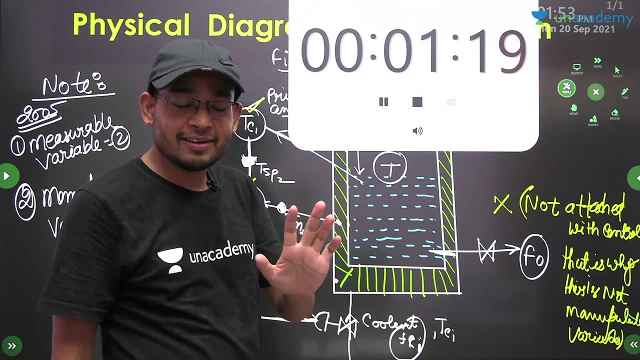 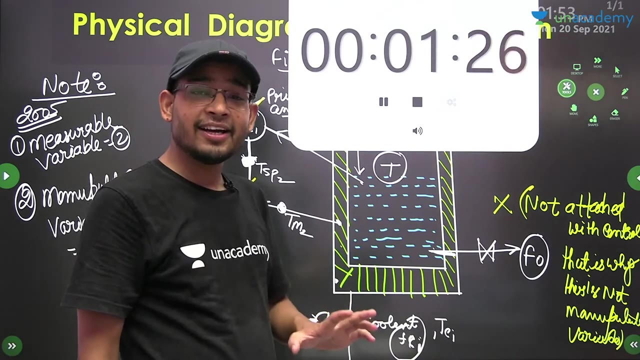 is it not being made? are you trying? are you trying? just try? if you try, something will happen tomorrow. what did CSK do? he tried. he did not give up. stay stubborn. the work is done. stay stubborn. if you stay stubborn, something or the other will become a run of your own. 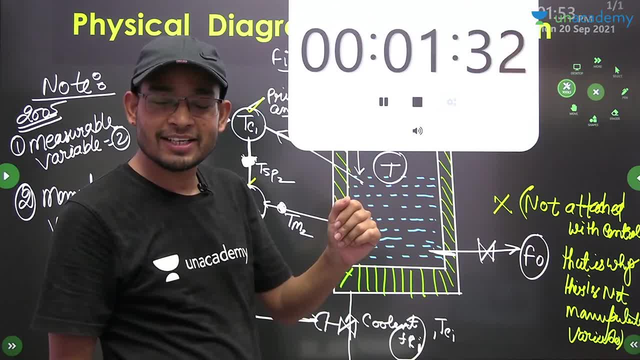 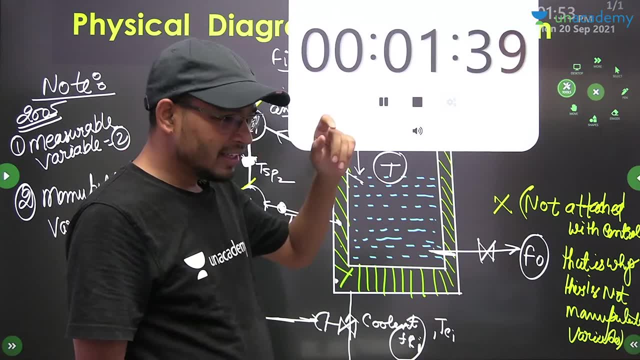 and if you do not stay stubborn in the beginning, then everything is over. the same happened with the Mumbai people. the Mumbai people could not stay stubborn. okay, if you stay stubborn, their work will be done. so it is more important to stay stubborn, Guru, okay. 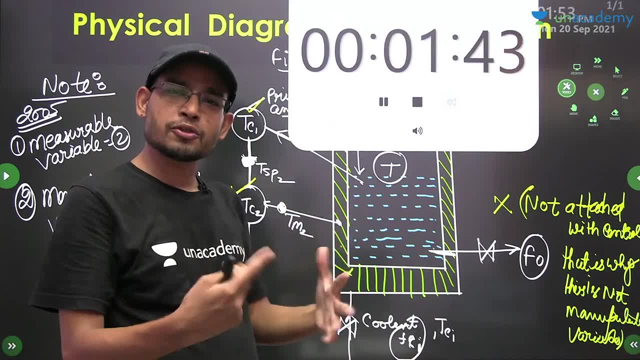 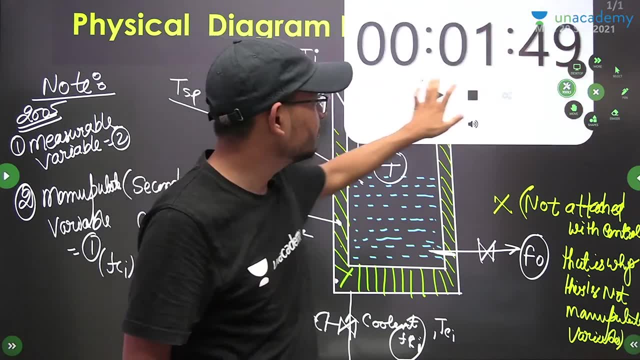 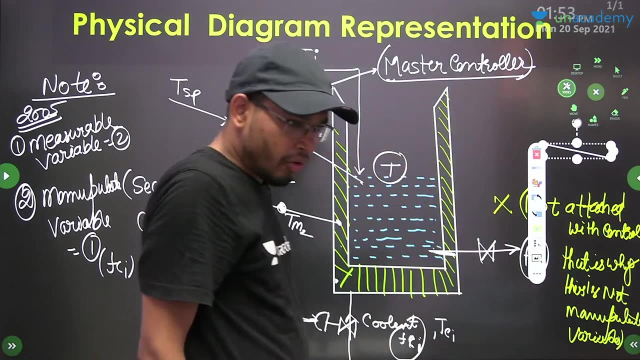 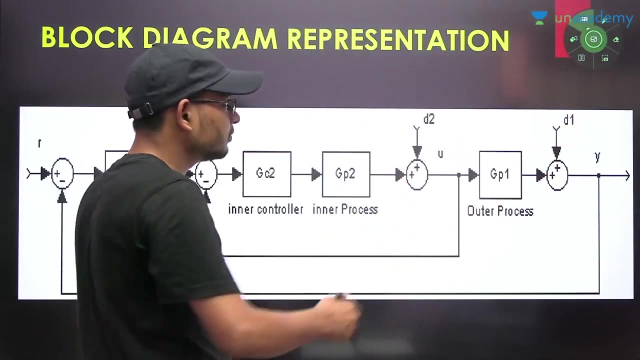 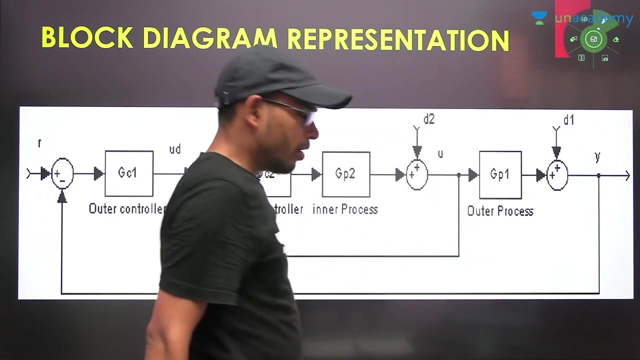 so try, try. something or the other will come out, something or the other will be made. come on, take your time, take your time, but the state, let's try and get what's done. okay, Prasad, done it's over. by the way, you are probablyケ. 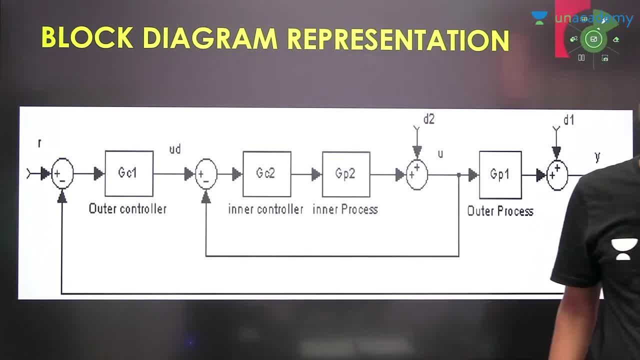 Both the members can make. it is itти? why has everyone got dead? you all will come out kind, gentleman. this is done. it's done. how did you make it? did you make it this way when i tried to explain- it'll explain it well, in this way- something that, in the way I made, something is made in this way. What to do is: did you make it this way? what did you make it know? have you made it like this? I told you: replace it in a sweet. I told you: yes, put it like this. I told you, yes, in this way, you made 엄청. la está esa. 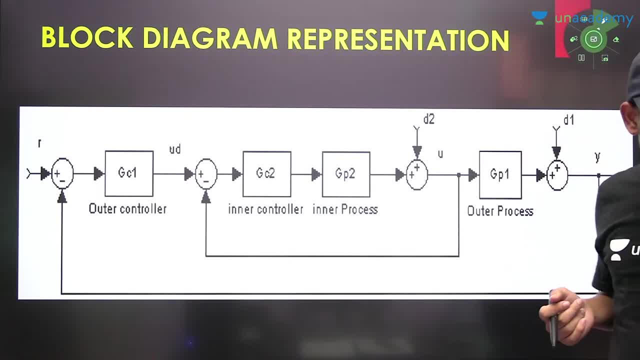 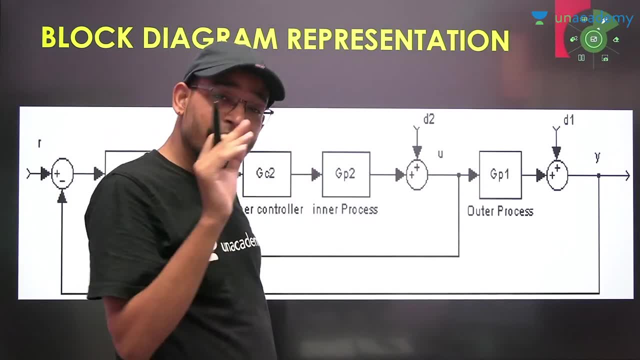 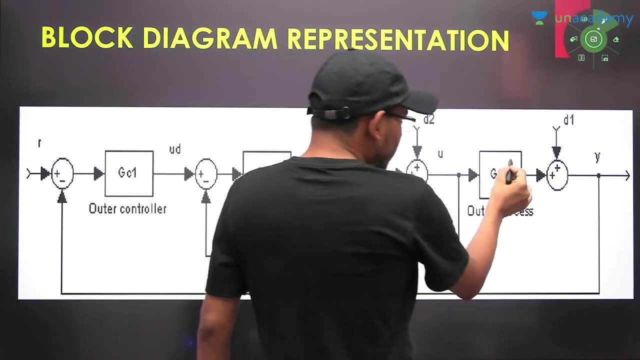 Everyone can see the figure properly. now see from where to start. this is not coming. So see the main process in which the temperature was T, in which the reaction was happening. what was your process? GP1.. This is the process 1, we will call it the actual process. 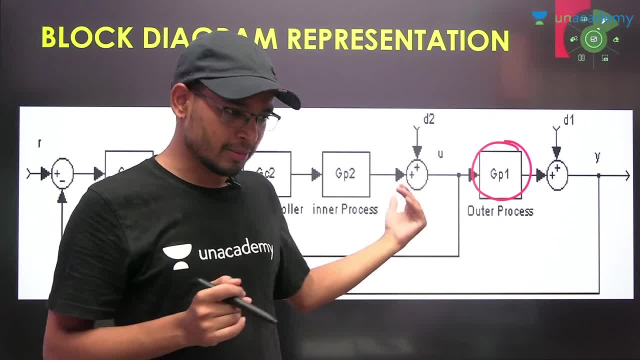 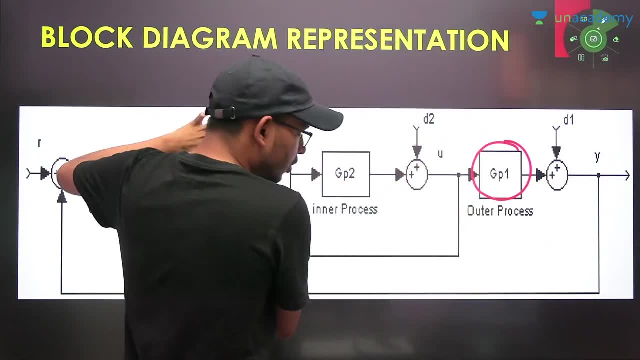 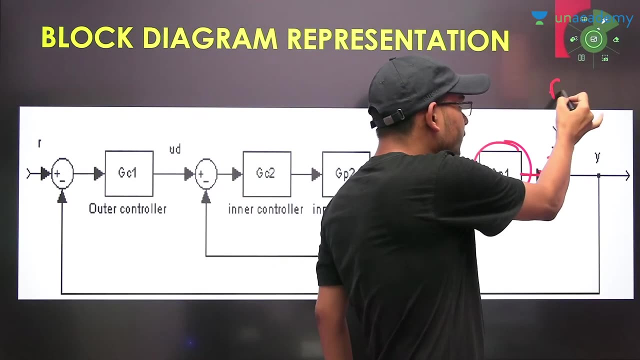 This is the GP1, now understand it very carefully. This was your process, GP1.. What happened to this process? Now forget all this. first start from here. GP1.. How much load were you disturbing in GP1?? This is your F1 flow rate. and what was T1?? 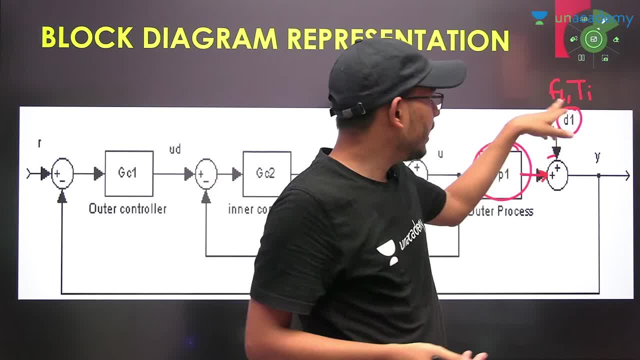 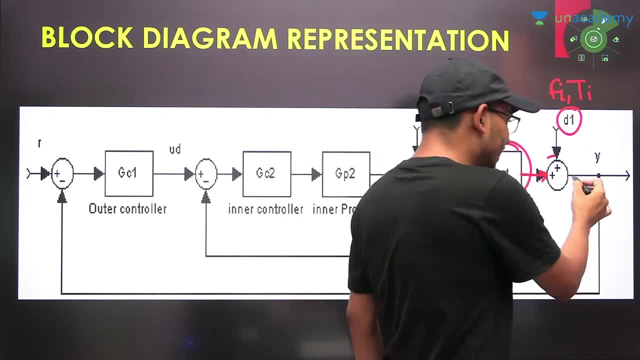 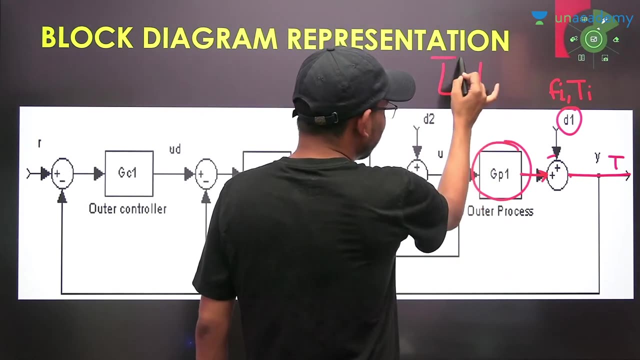 Ti. whatever flow rate was coming from above it, Fi and Ti. this was your load variable going on it And the output that was coming out of it. what was that? Your temperature T? Which reactor did I talk about? I just talked about this reactor. 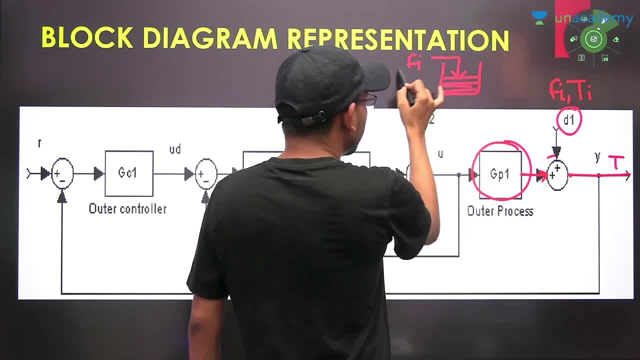 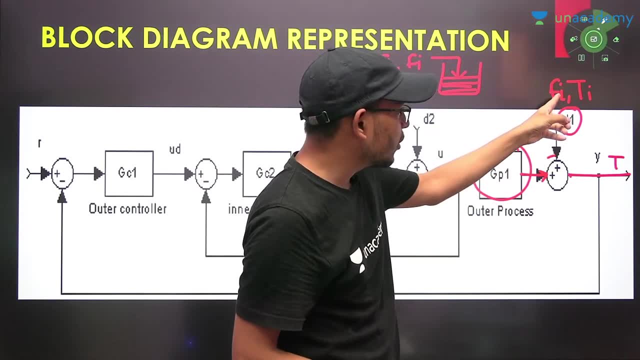 The load that was coming out of it. how much was coming out of it? Fi and Ti? This process is GP1.. What was your load in this process? D1.. What would be the value of this Fi and Ti? Now, what did you measure from here? Temperature. 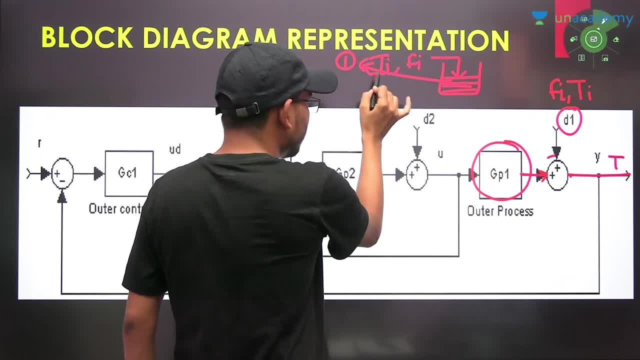 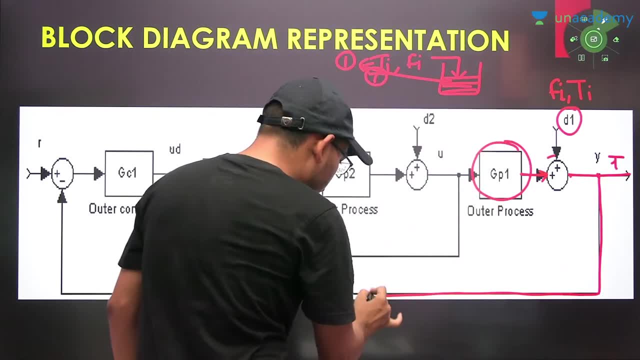 What did you measure? from here? Its temperature. From here, you measured the temperature. This temperature, This temperature was measured After measuring this temperature. where did you reach? Think where? I will say this, I will say this: Tm1.. 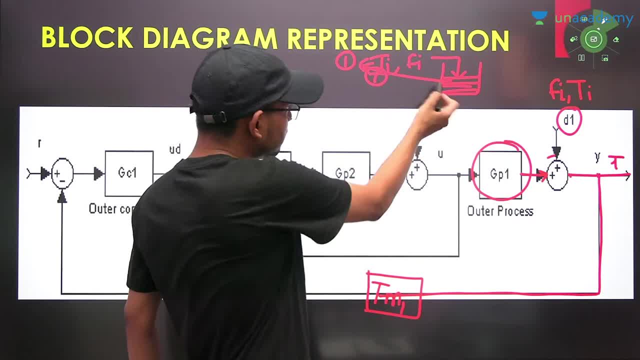 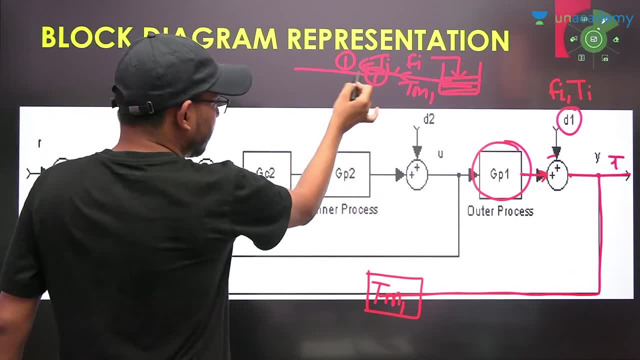 Okay, The first thing you measured. this is Tm1.. The water that was coming out of this Tm1.. Right, This is Tm1.. You measured: Where did you add this measure from the set point? What did you put there? 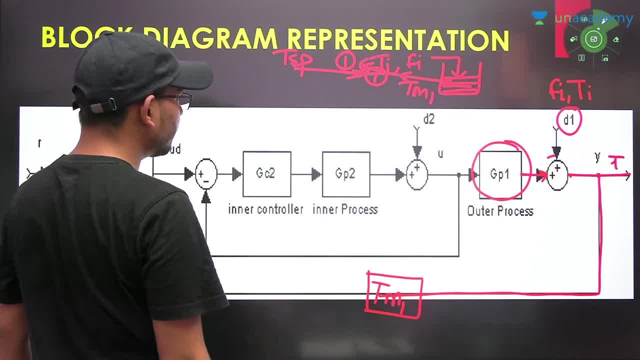 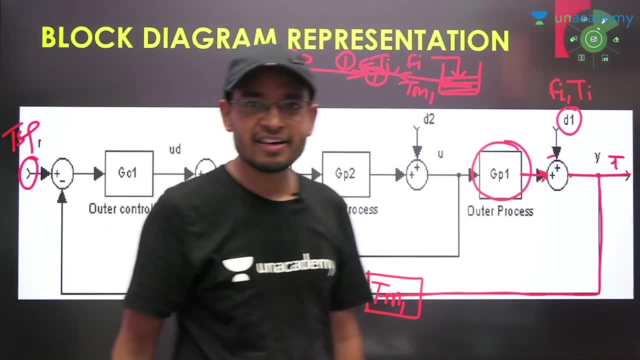 You had set the point right. Can everyone understand the figure You had set the point? To whom will this go? Set point: This will be Tsp. This will match with the set point And whatever its value is going to be minus Tm1.. 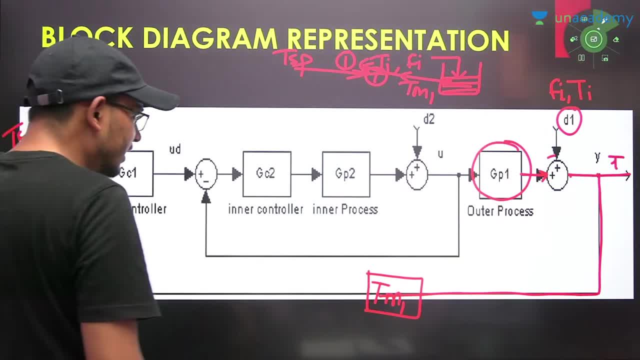 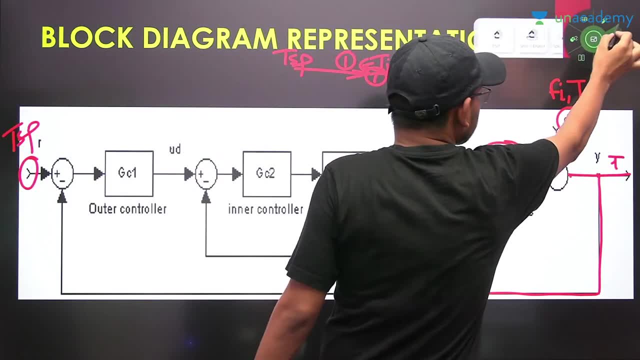 Okay, Whatever this value is going to be, don't write Tm1 from here, Because Tm1 is this. So don't write Tm1, write something else. Write Ym1.. Write anything else, Because Tm1 is this. 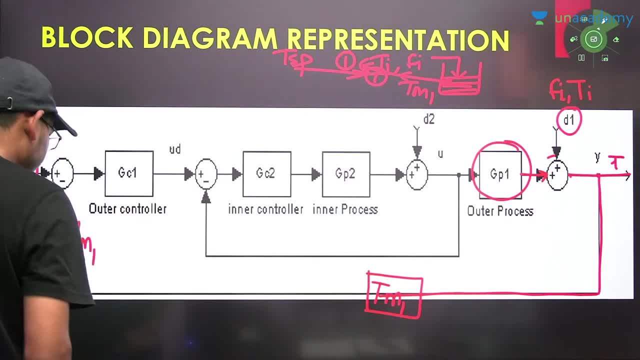 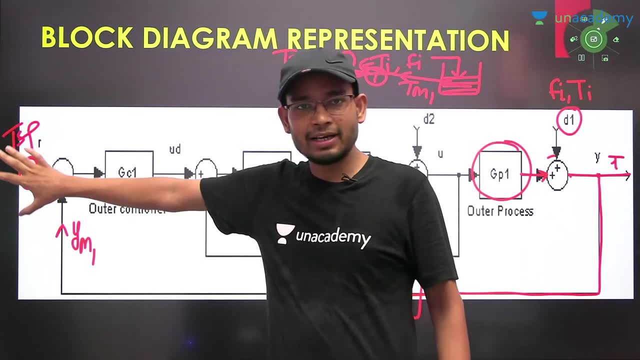 Okay, This value will be going, Suppose, Ym1.. Okay, This value will be going Ym1.. Then, from here, the response will match with whom With your set point. everyone can see that And that is the value of your measuring device. 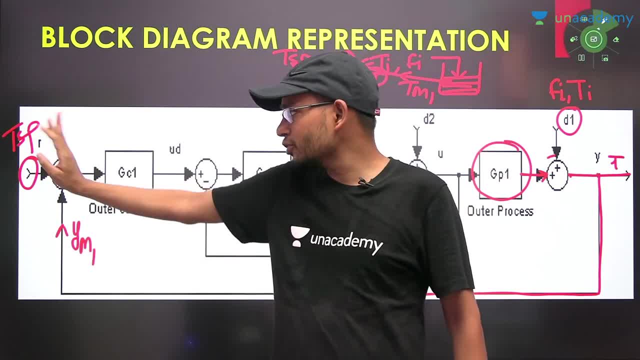 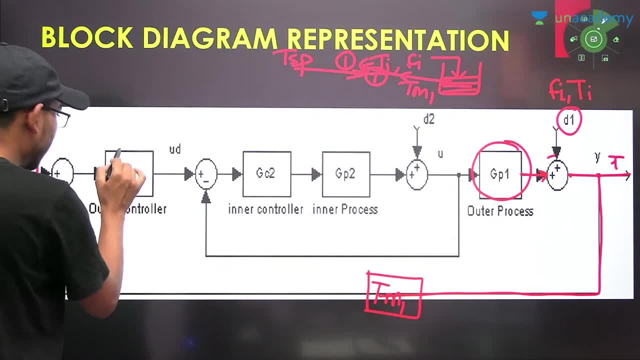 The measuring element which is going to produce the reading and the set point. to whom will that go, bro? Controllers- primary controller. This is the primary controller. This is the Gc1.. This is the Gc1.. This is the primary controller. 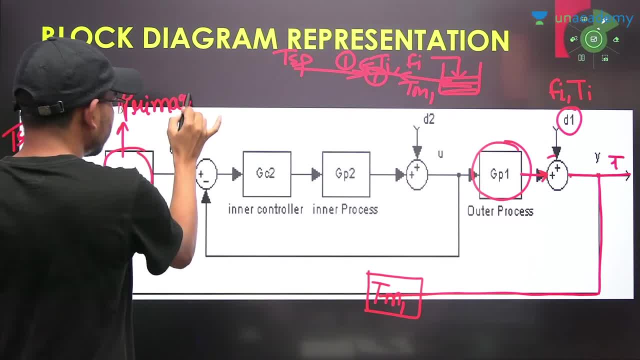 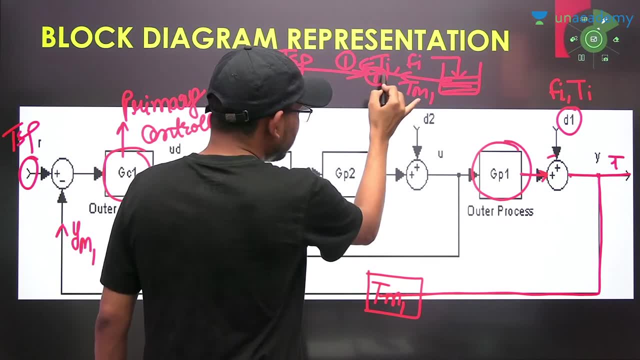 This is the primary controller. Everyone is able to understand the detail right? This will go to your primary controller from here. Where did it go? TC1.. It came to TC1.. This was the primary controller. Write TC1.. Write this TC1.. 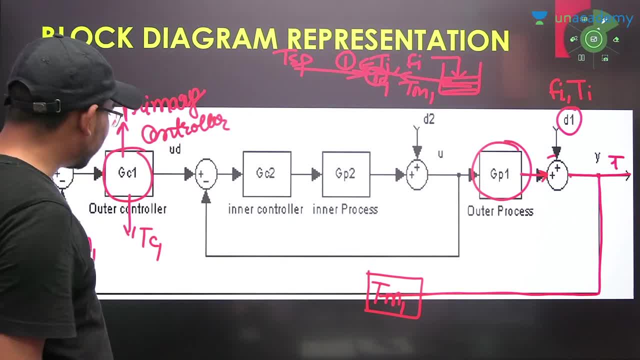 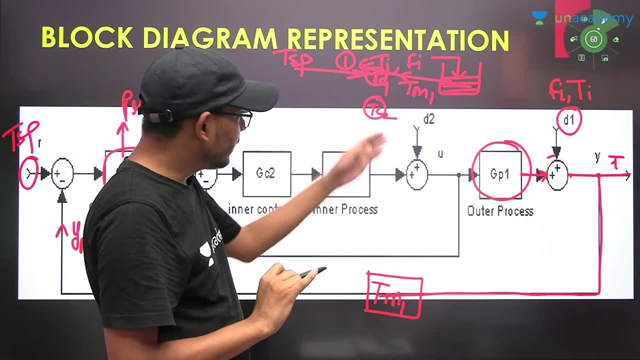 Did everyone understand? Now, what will TC1 do? The output of TC1 will go to TC2.. TC2.. Guru, do you understand everyone? Its output will go to TC2.. The output of the primary controller will go to TC2.. 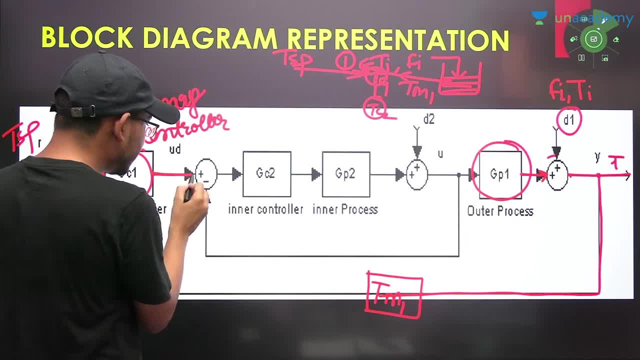 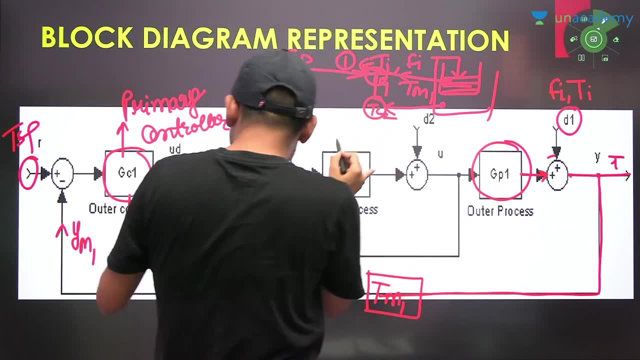 Now look carefully Now, before going to TC2, where will it go? There will be another coolant attached to it. The one who will measure the coolant and the input of the primary controller and the one who will measure with the coolant will be your TM2.. 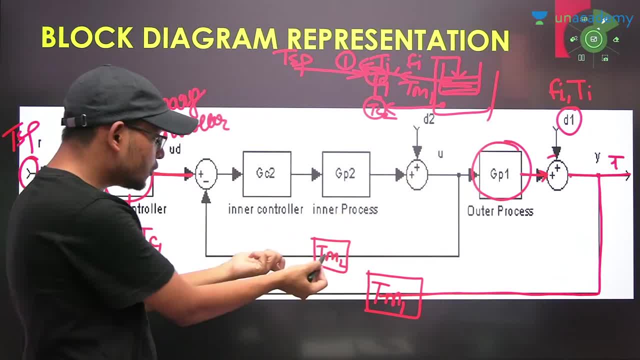 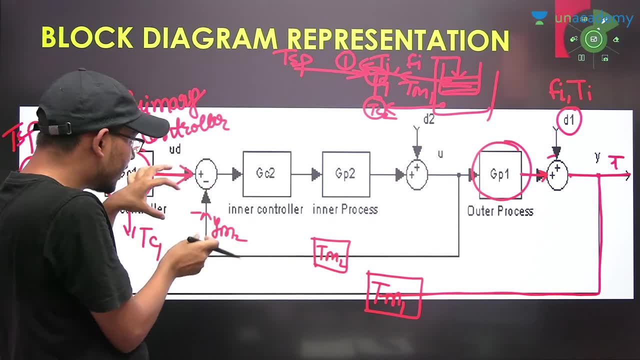 This is the inner loop value. This will be your TM2.. The TM2 that will be coming. I will write it as YM2.. This value will be coming and the input that will be going from the primary controller in which error will be going. 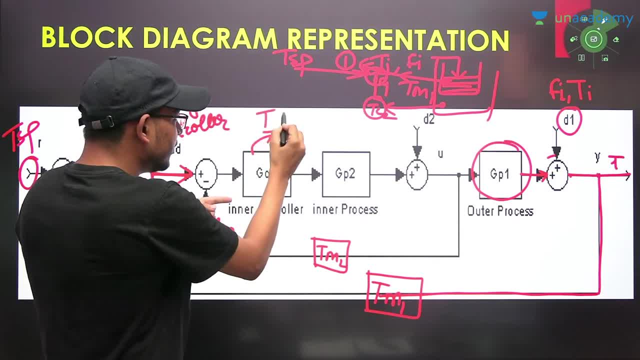 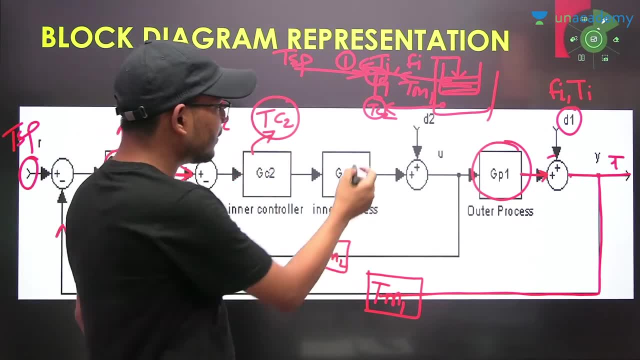 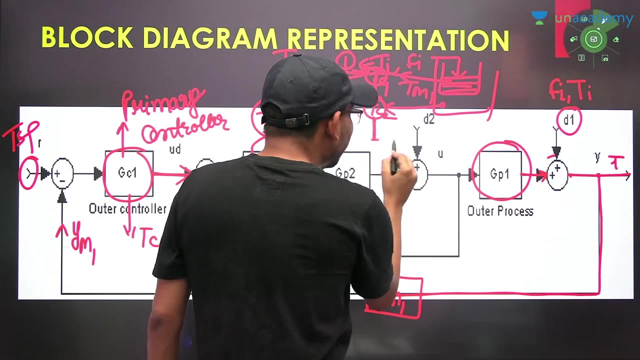 This error will be going in TC2.. This is your secondary controller. This is the secondary controller After the secondary controller. where will it go? Where will it go? Everyone tell me Where will it go. This is your coolant. Now the process is GP2.. 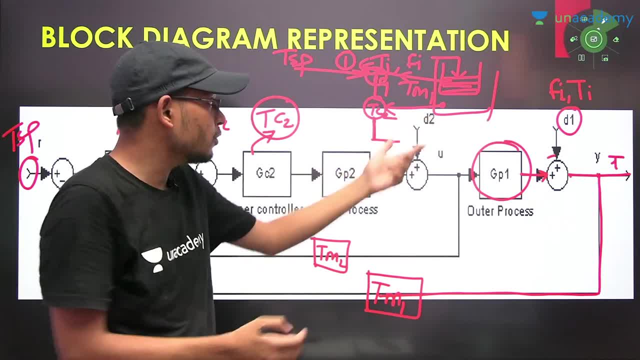 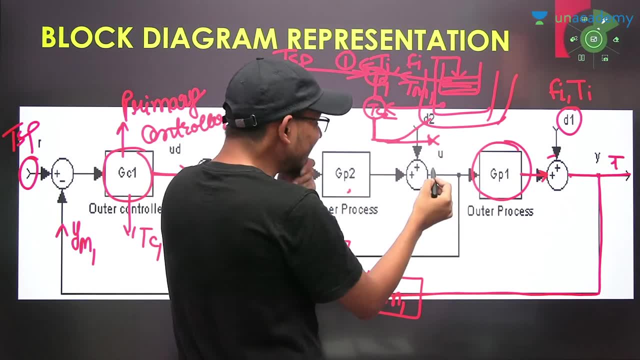 Where will your other process go In the process, The one that was your coolant? What will it do in this? Yes, Where will it go? Okay, Where will it go? This is GP2.. This process is GP2.. Now there is a load in GP2 too. 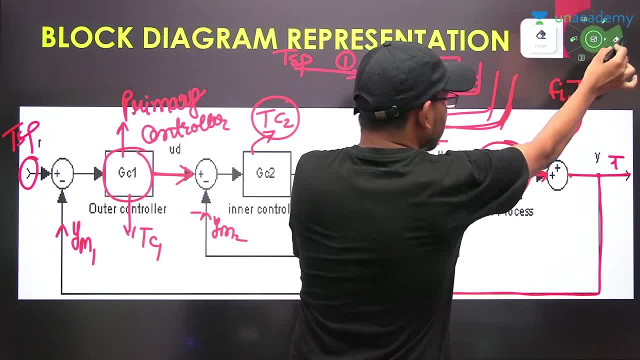 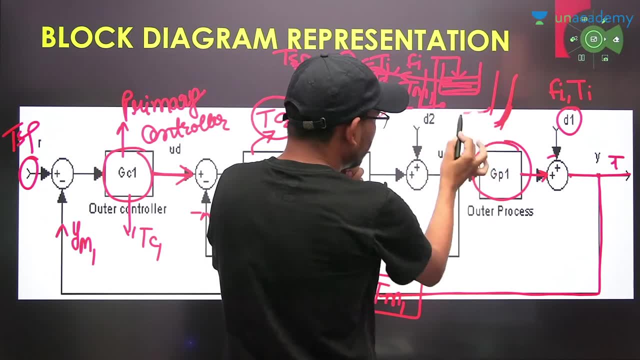 What is this D2?? See here, I am erasing it a little. I am erasing it a little. Let me explain to you. See what is written here. What is written here, This is D2.. What does D2 mean? 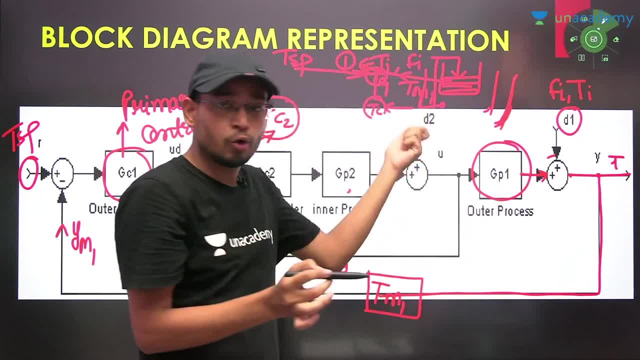 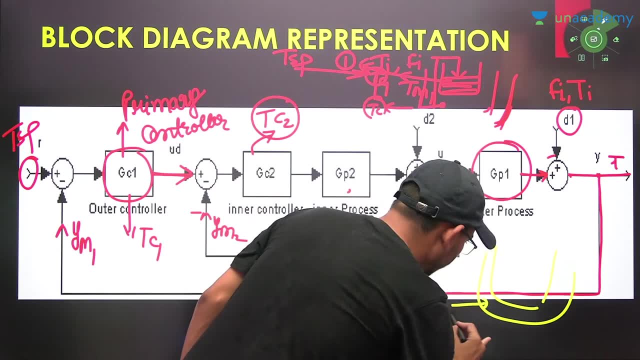 D2 means this: The coolant that you were putting in that is also loaded, The jacket that you had put in it. Suppose you had put this jacket. This is the process: GP2.. What did you see in this? You had given this load, right. 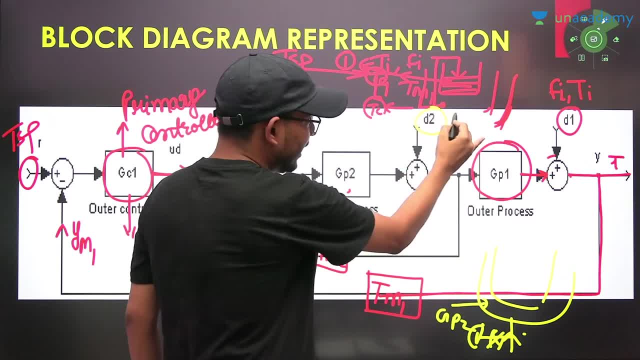 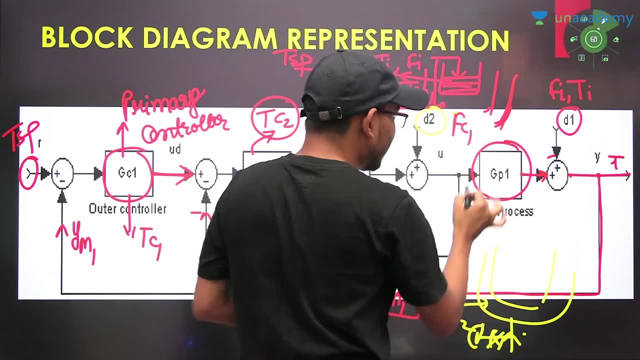 What did you give this? You had given this load. That is it. What is this? FCI Coolant flow rate And FCI Coolant flow rate and TCI Temperature. What was this? The input for the process? 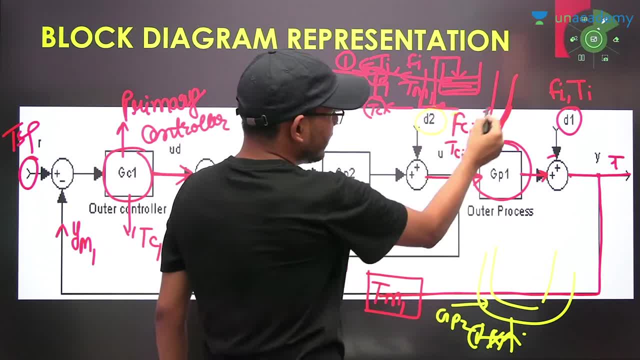 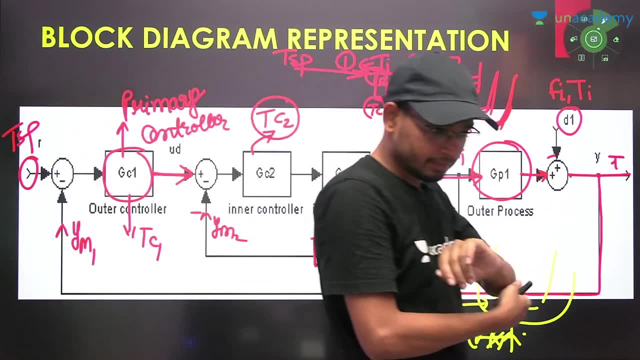 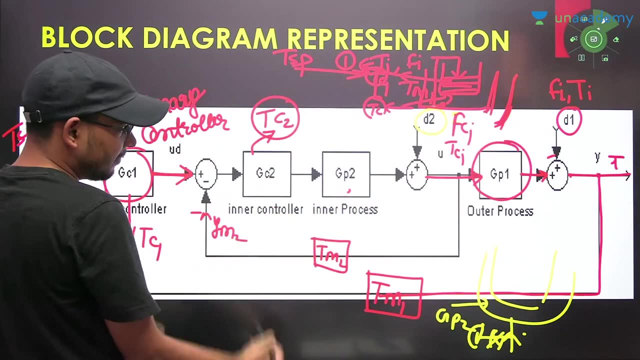 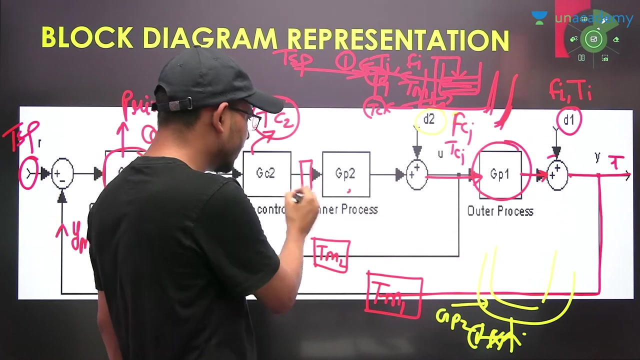 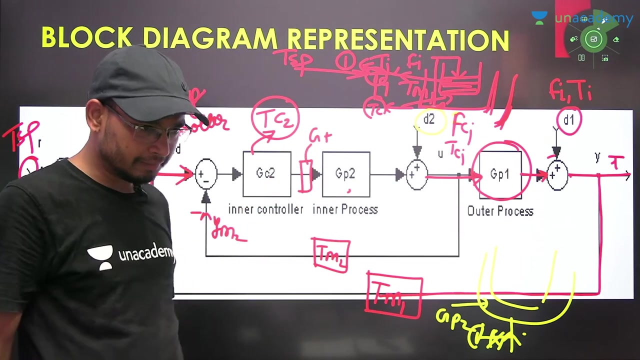 Now, where will this go In your first process? Okay, Where will this attach to you In the first process? So this is the first process. GF will come before this. it is not installed. where is GF? this GF will come before this. where will it come? where will it come? yes, GF will come after controller. GF will come here, but it has not been shown. GF will come here. ok, GF will come here. it has not been shown. before going to process 2, it is a little different. 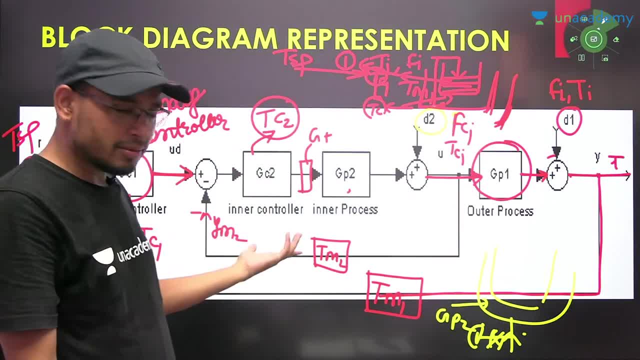 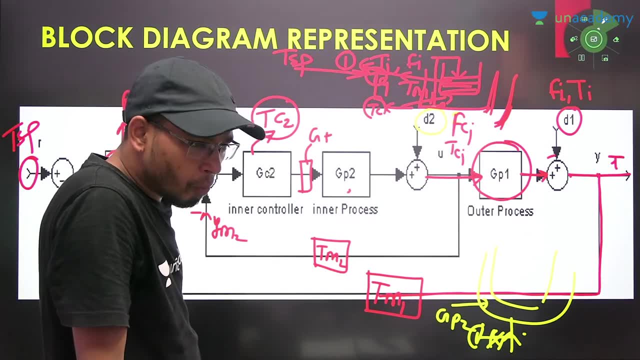 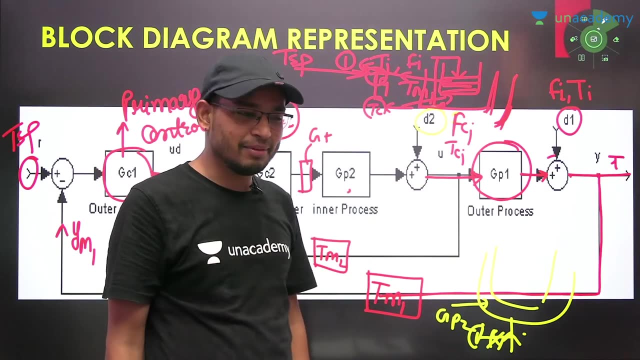 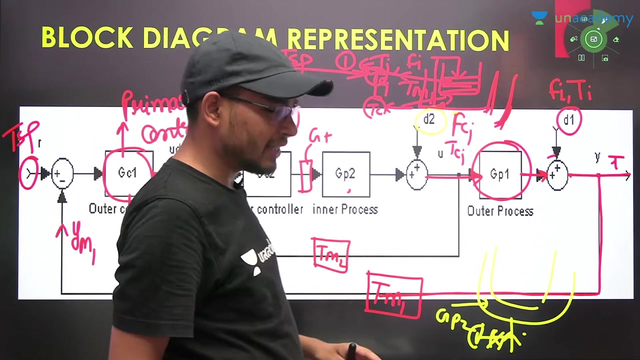 did everyone understand this or not? first tell me, are you getting this? I said: there is no figure in gate, you just have to understand. just understand. then also it is fine. if it does not come, then also it is fine. ok, G2, once once I will tell you completely again. should I tell you again once completely everyone. should I tell you again once completely. 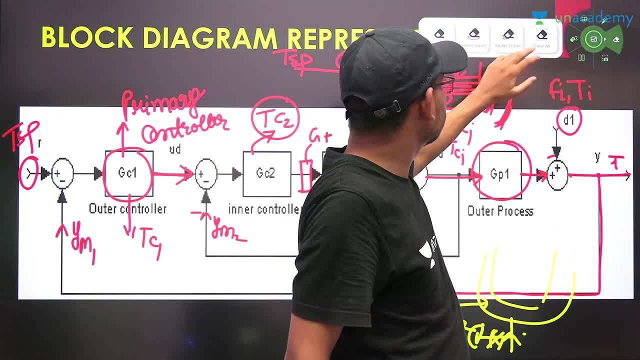 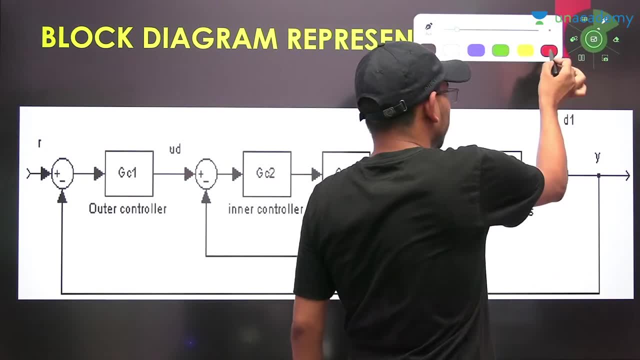 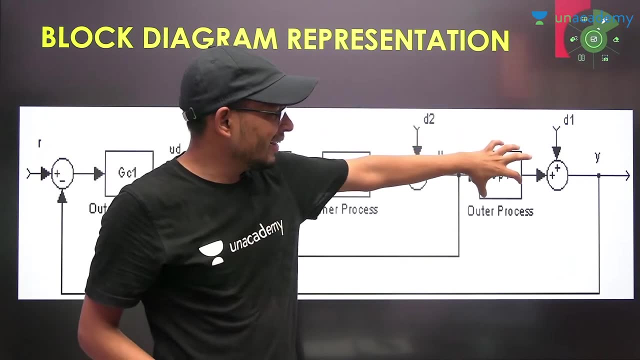 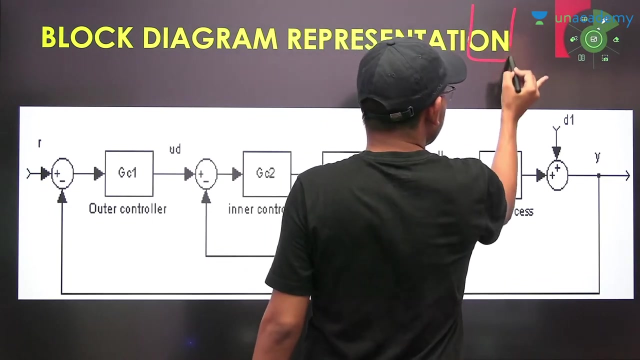 come on, I will tell you again. don't worry, I am erasing. I will tell you again. see, come on, I will tell you again. yes, sir, crystal clear. come on, I will tell you again. repeat, repeat. your GP1 was actually process. ok, your reactor was your reactor was ok. as I make this, this was your reactor. ok, this is your GP1,, this is GP1, ok, this was the process. 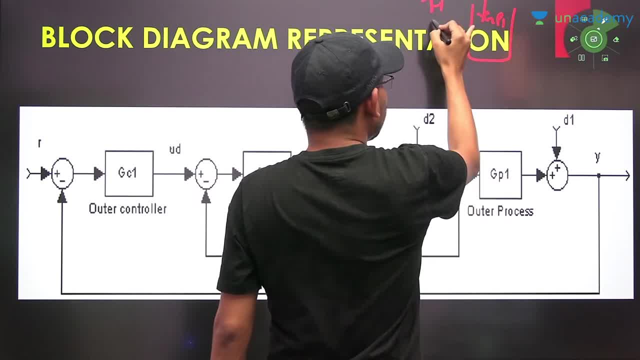 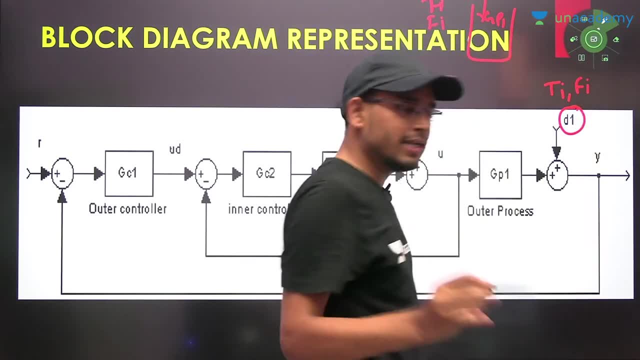 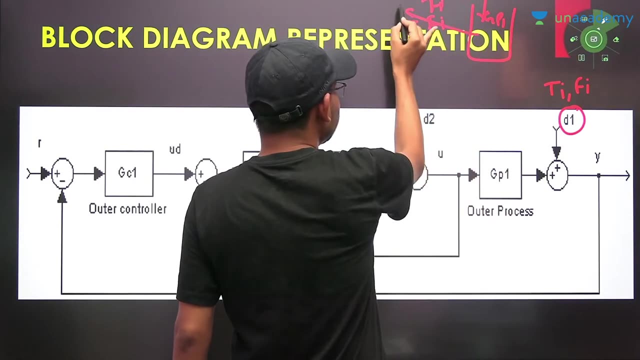 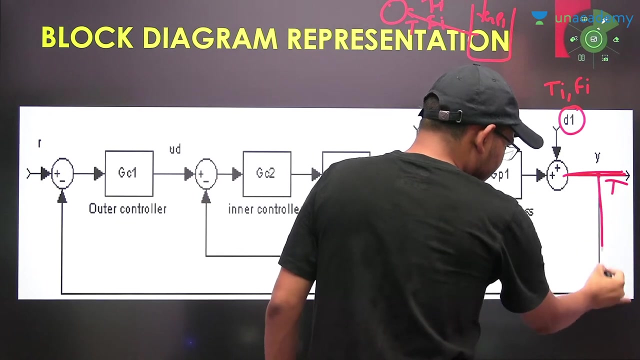 what was your load? this is TI and what was your FI? ok, this is your load. what is D1 load- TI, and what is FI? ok, this is your load in the process. now the output of this will be: this temperature device is attached. this will be the output, the temperature in which it will go. it will measure its temperature. it measured. I call it T. ok, this measure, with whose help will this temperature do? measuring device. this measuring device will be written TM1,. 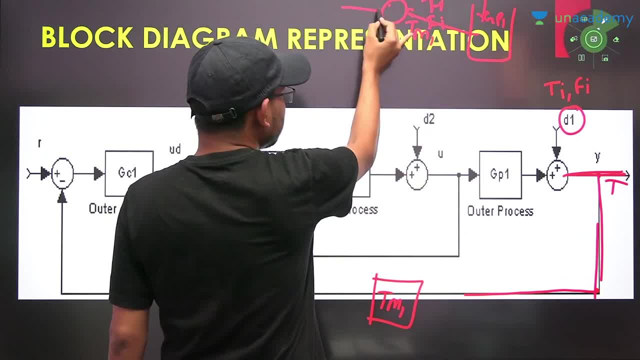 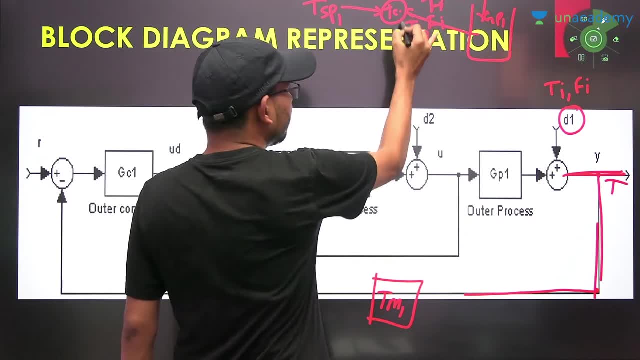 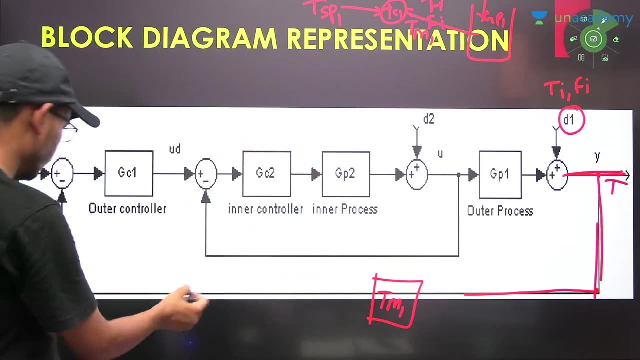 ok, this measured TM1, ok, temperature from where it matched it TSP. ok, consider TSP1, ok, and this controller came TC1,. this is the controller. ok, in this controller, how much error will come? TSP1 minus TM1, ok, so much error went in this. see, this came. this controller was GC GC1, in this, how much error came? TSP minus TM1,. so much error. I will call this E1,. 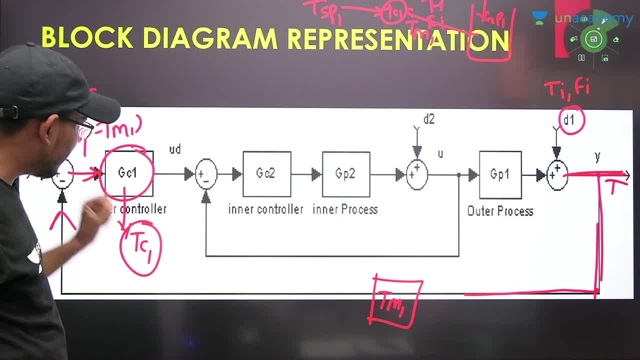 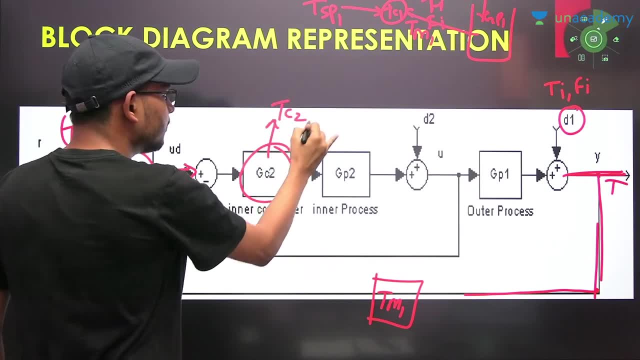 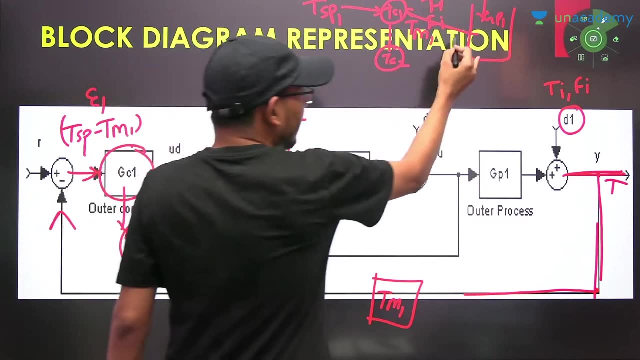 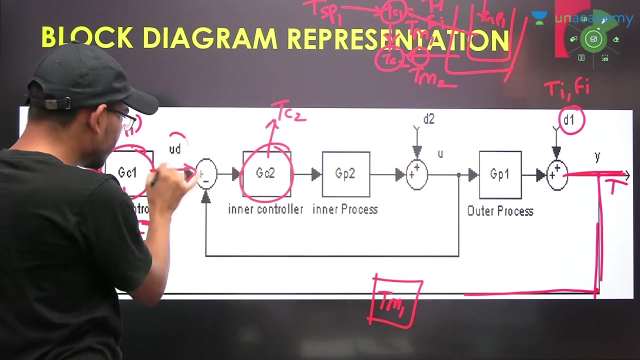 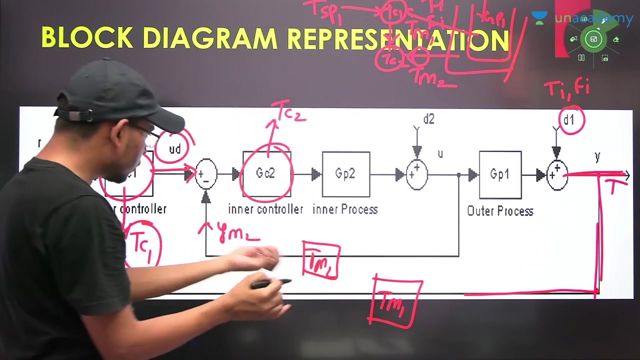 This is our primary controller. Now the output of the primary controller will be the input of the secondary controller, TC2.. The input of the secondary controller TC2, will match with the coolant. The output of the coolant will match with the input of the TC2.. 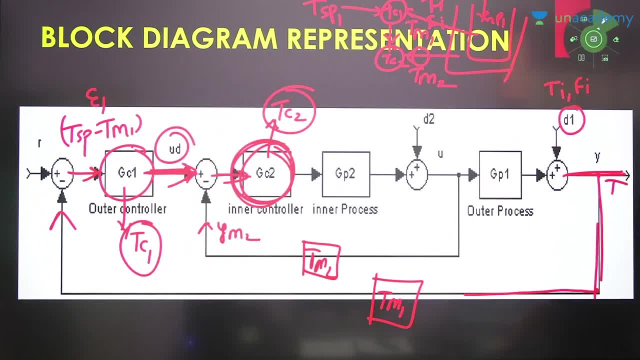 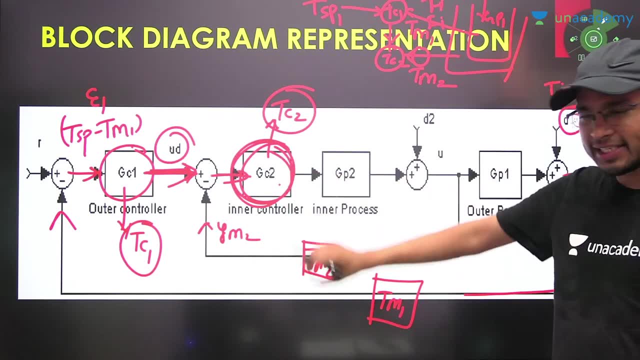 Did you understand? The input of the secondary controller TC2 will match with the input of the TC2.. Did you understand? I will read further. Will you quickly comment and tell A little fast? Understand that you have come to this point. 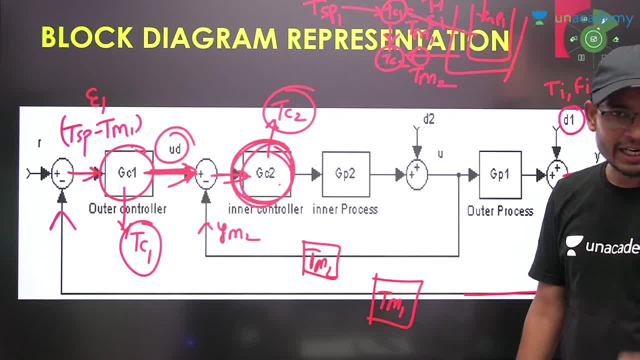 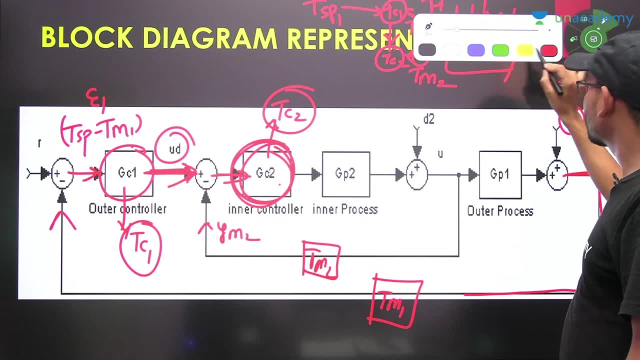 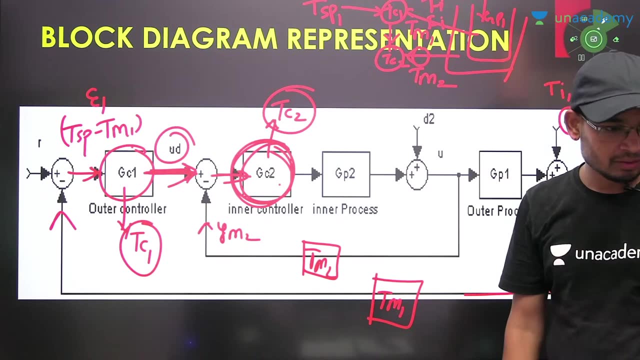 All of you have reached the secondary controller. All of you have reached the secondary controller, Yes or no? All of you have reached the secondary controller. Yes. If you are not coming, then ask. I am telling you in a very simple language. 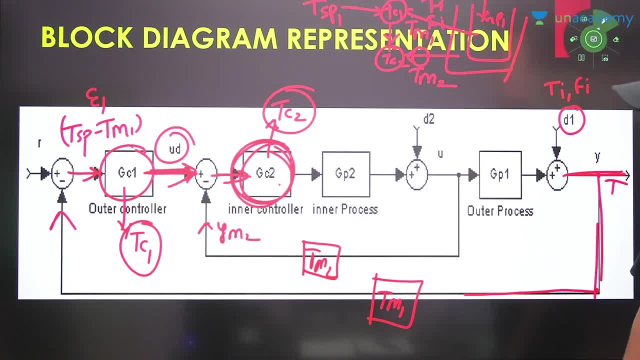 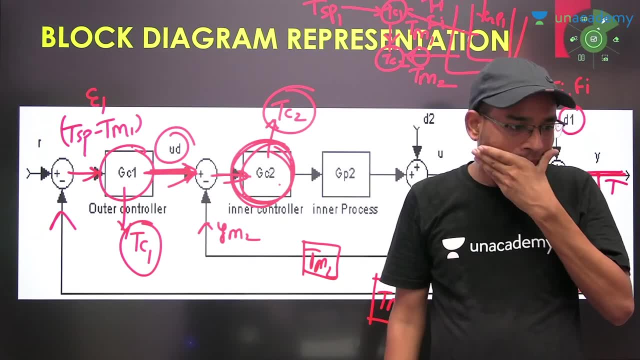 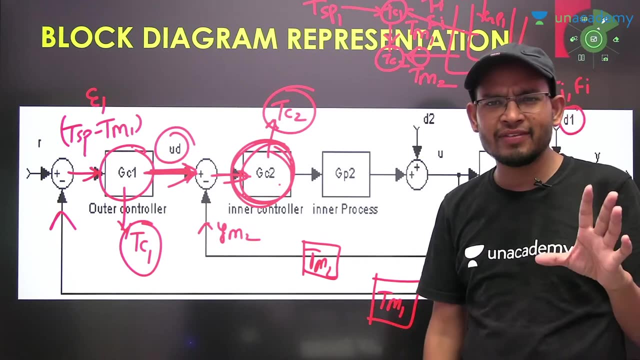 Did you reach the secondary controller? Yes, Okay, You reached the secondary controller. right, You reached this point. Okay. Now look Here. TC2 will be attached Somewhere. you will see that the final control element has been attached. If the final control element value is 1, then it won't be attached. 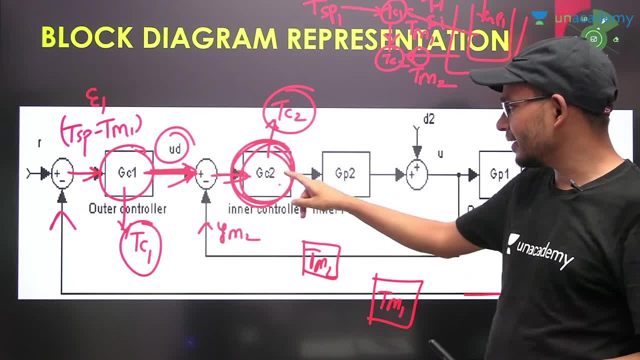 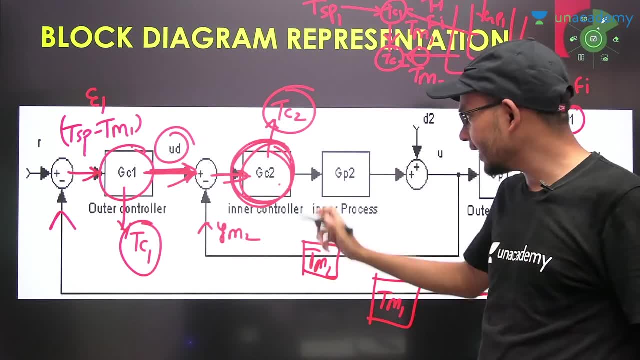 Along with that, the final control element between this one controller and process GP2.. So the final control element may be attached. If it is not attached, it does not make any difference. Okay, Where will it go in GP2.. In case you have to install it, then install it in the middle of it. 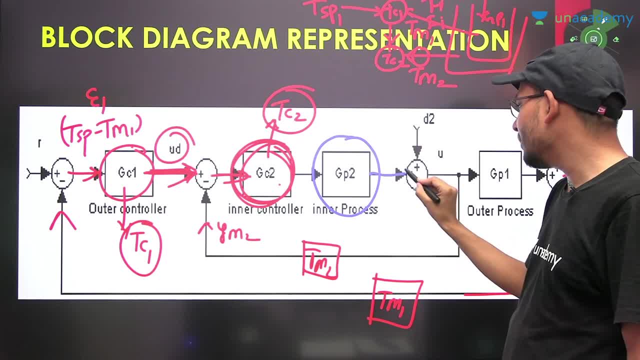 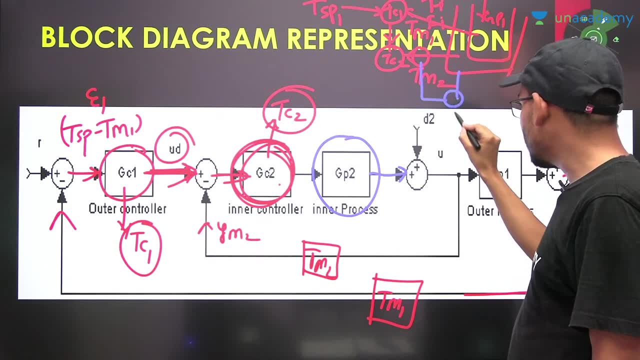 Where will this go? GP2.. Now, how much load will be there on the GP2?? How much load will be there on the one you have installed, The one going from here? How much load will be there on this? This is your FI and TCI. 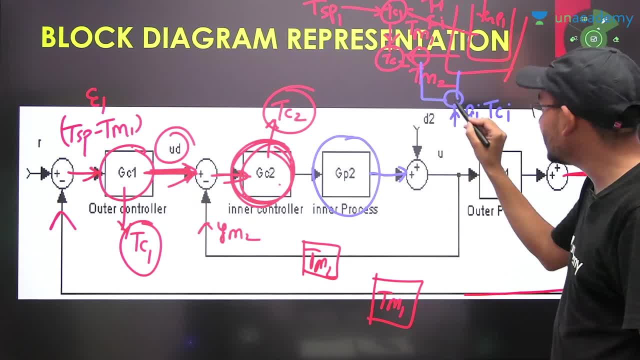 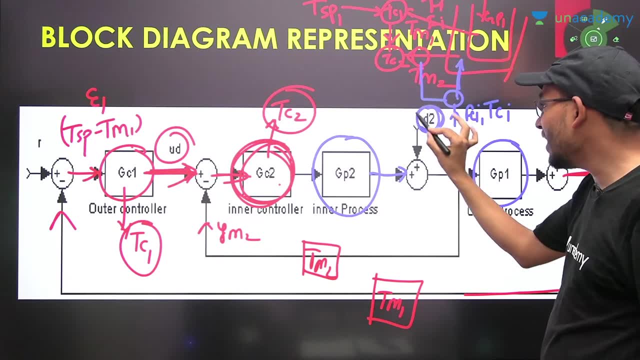 FI and TCI. How much is its load? FI and TCI? Then in which process will that whole process go? In GP1.. This is the process in GP1.. What is this? D2?? This is the load of the secondary loop. 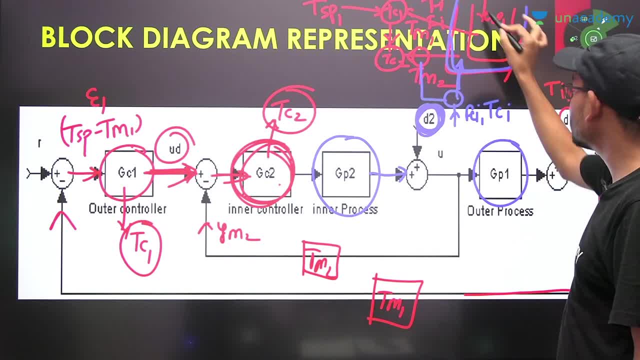 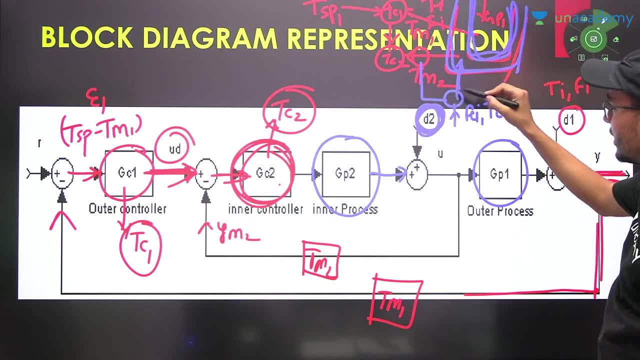 What is this? This loop is the secondary loop And this is the primary loop. The first one was the primary loop. What was the load of the primary loop- This one, FI and TCI- And what is the load of the secondary loop? 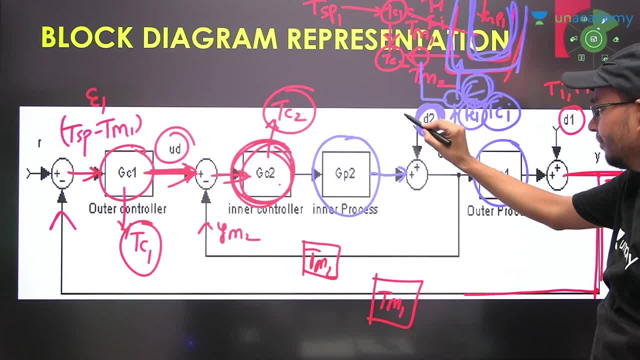 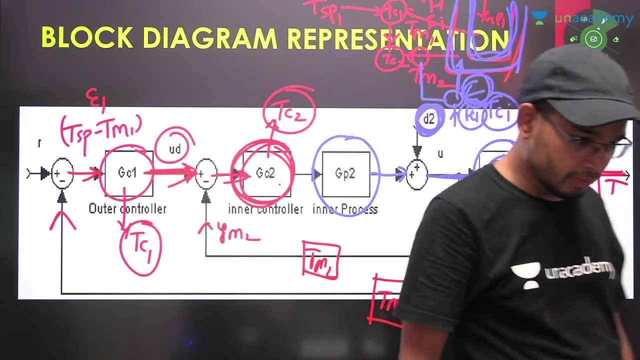 This is the load of the flow rate of the coolant and the temperature of the coolant. This is its load. Then in which process will it go? In this process In GP1.. So how much load will it take? FI and TCI. 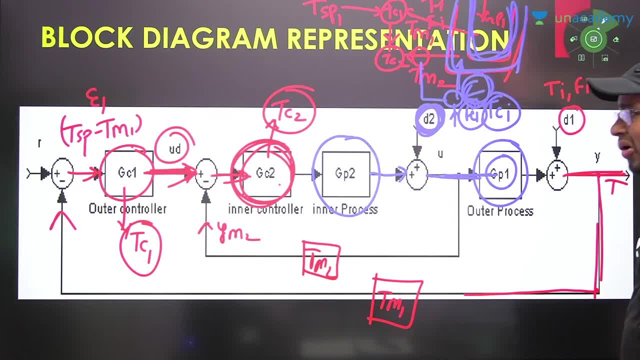 FI and TCI. How much load will it take? FI and TCI. Ok, So for every one this will take the total load of the secondary loop. How much load will that load take? 1. 1. 1.. 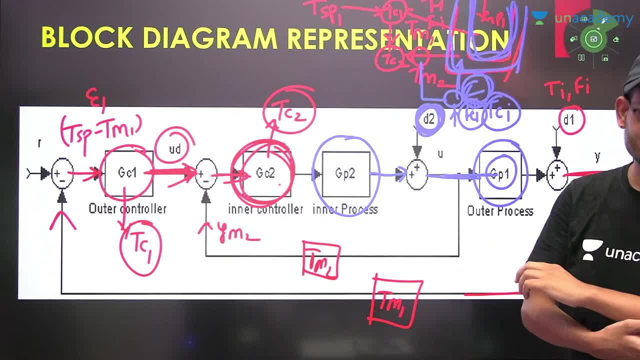 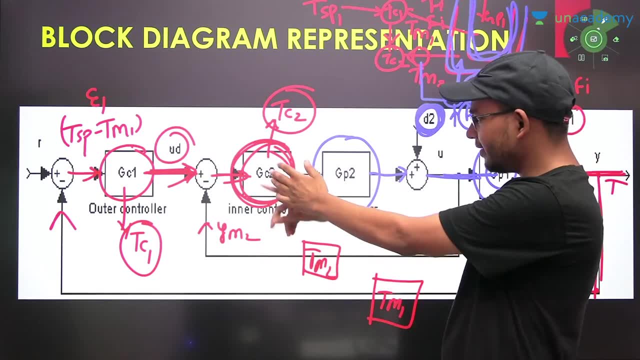 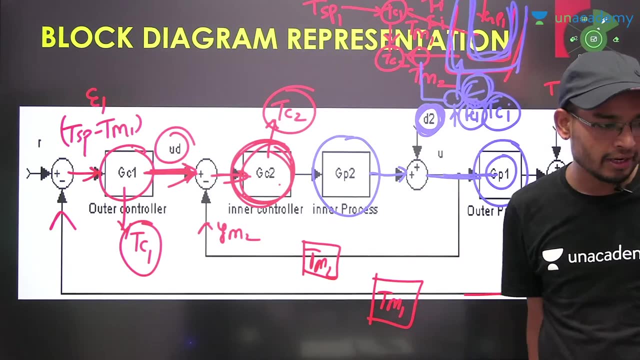 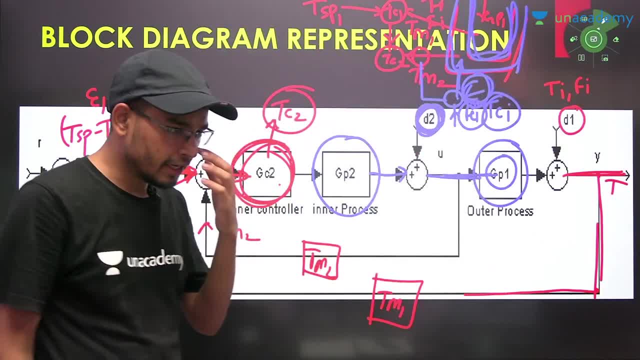 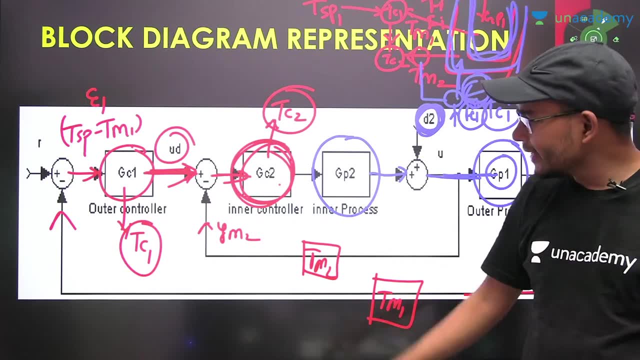 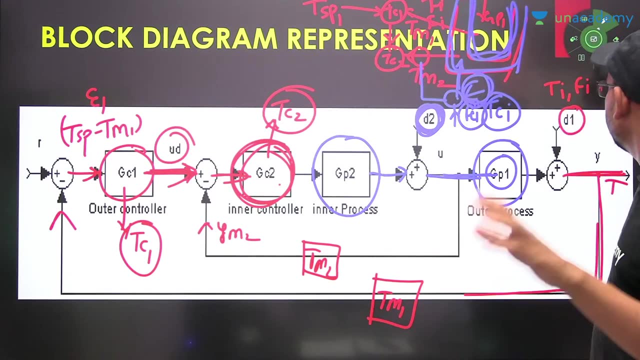 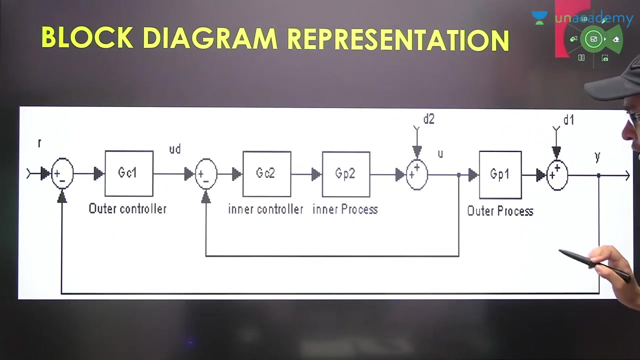 Write this much clearly, Write this much, Then see how fast it is, In case this work without you now first understand how fast it is. Listen carefully, See, Understand once. See how fast it is. Suppose you don't have this controller. 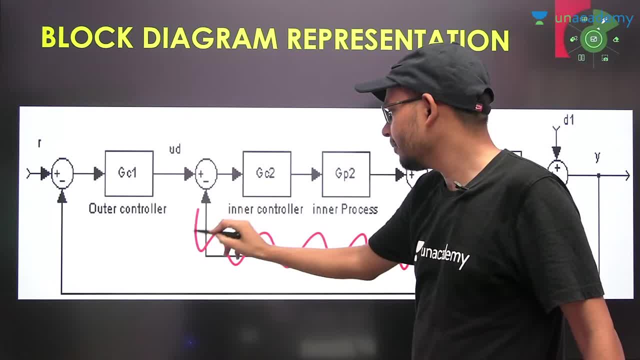 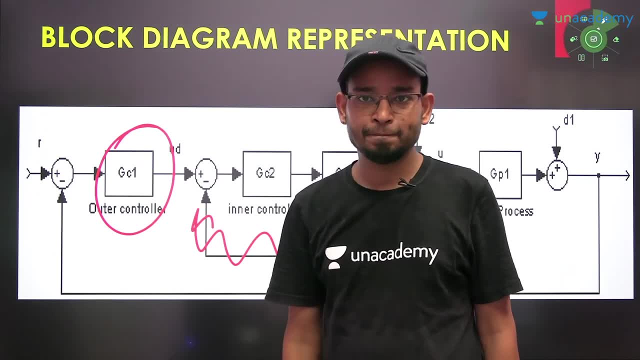 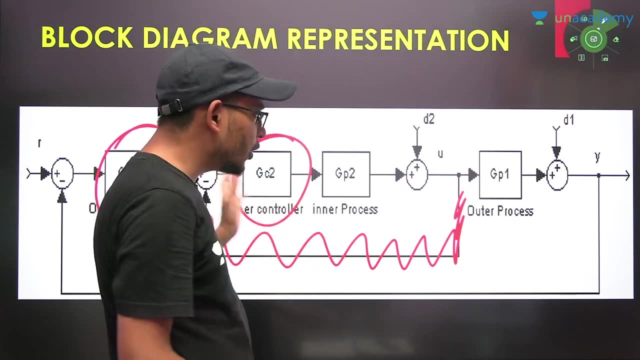 You don't have this controller. So what happens to the system? It gets more load. This primary controller gets a lot of load on it. Now you have installed one more controller, GC2.. So you have reduced the load of this, And what have you done to the process? 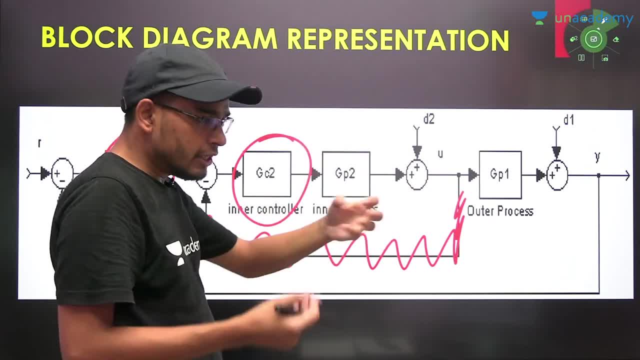 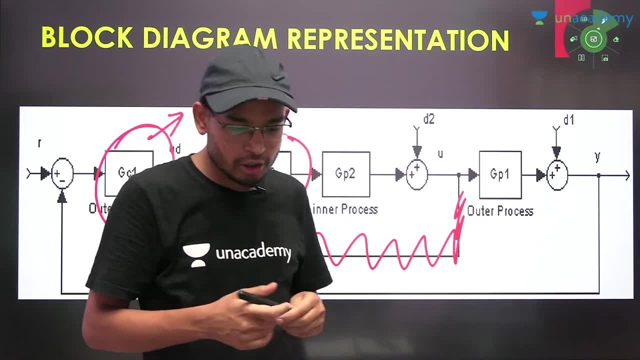 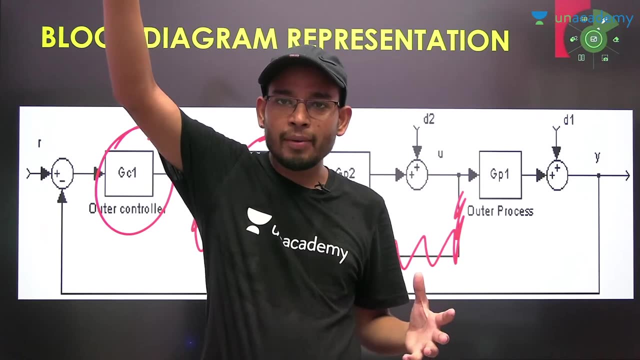 Now what happened to the process? It got fast. It immediately started to catch small errors. What does this mean? It started to solve the problem inside the loop. Suppose you build a building, So the one who sits at the top, in case he will do all the work. 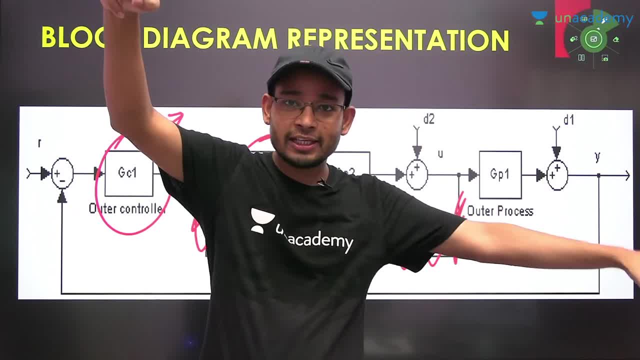 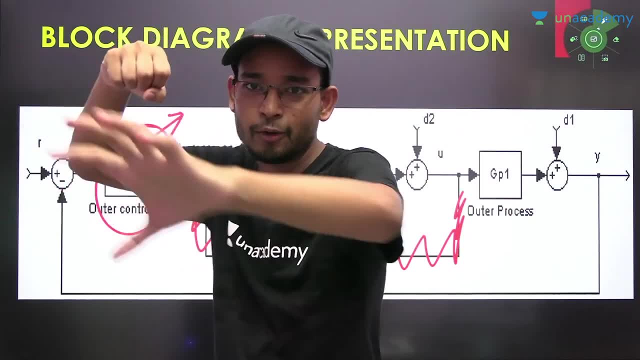 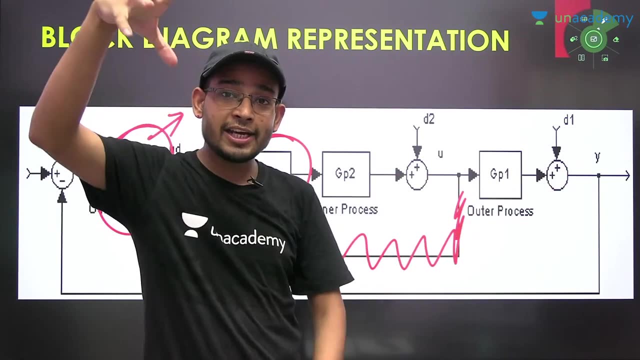 So it will take a lot of time to build a building. What does he do? He puts a distributor, He uses something, Then you will take care of this department. So what does this mean? Instruction is getting fast, In case he becomes a master. 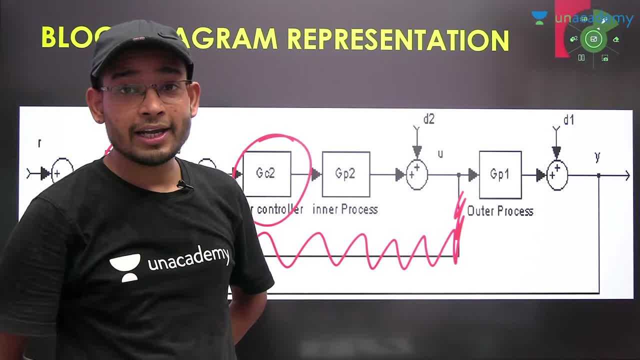 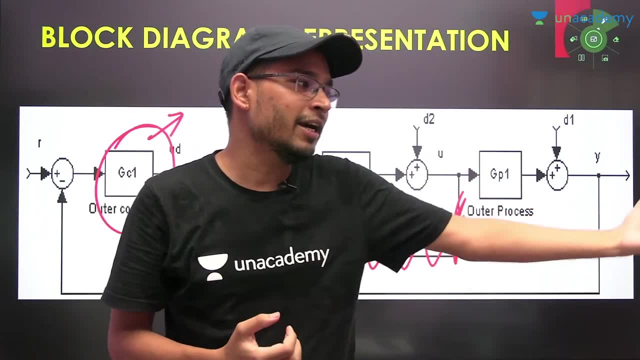 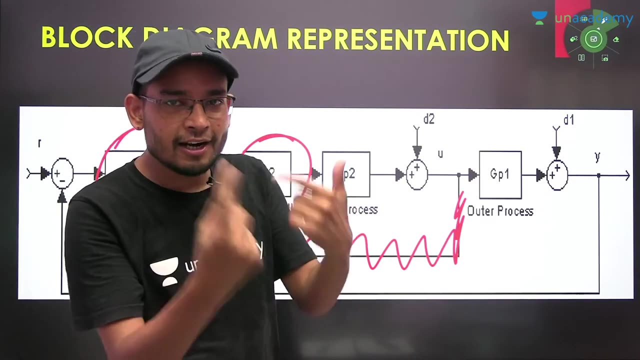 And he decides that he will do everything slowly. What will be your work? It will be slow. So it has done something called secondary control. Your department is this: You take care of this and give us information, actually working on the inner loop. 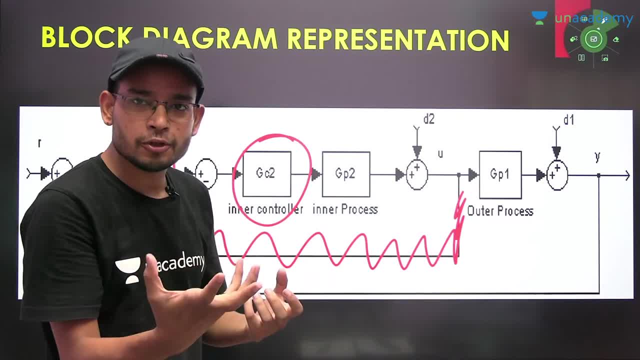 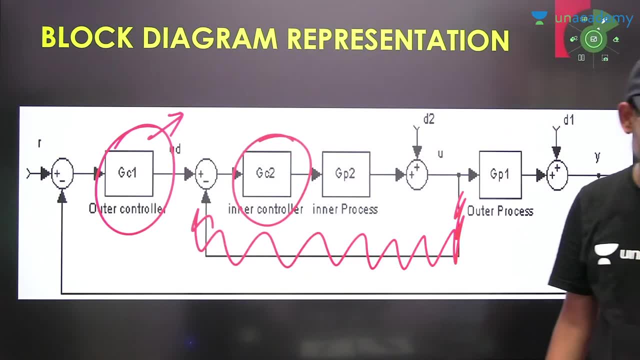 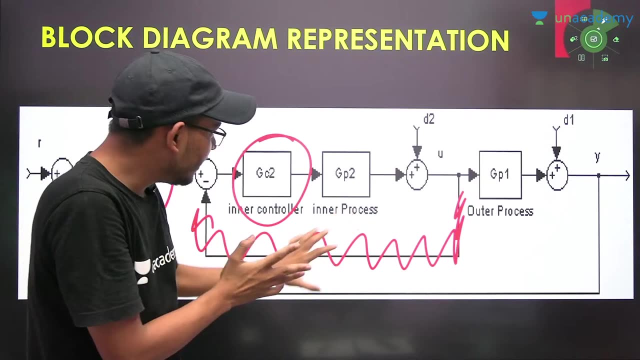 what is the inner loop doing? it is solving the inner loop and immediately it is giving that information to the client, to this client. are you getting it? that is the thing. the contractor, the building. what is the work of this? the work of the master controller is easy. 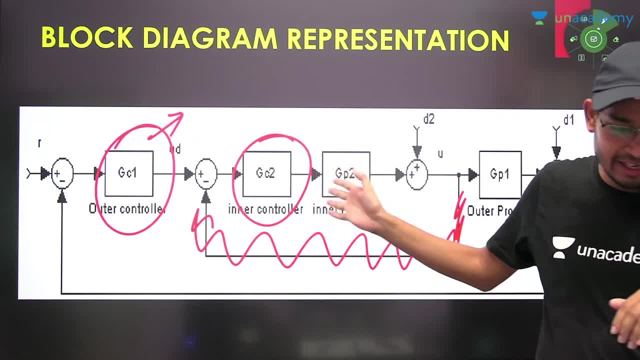 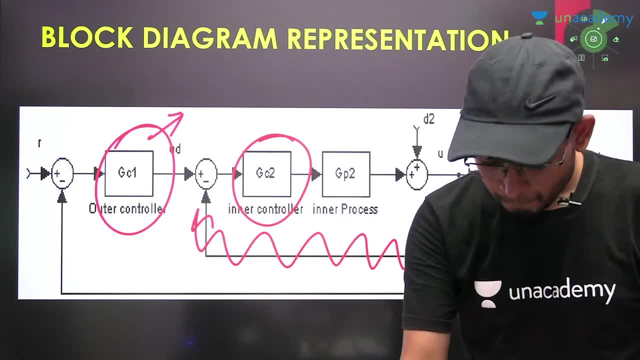 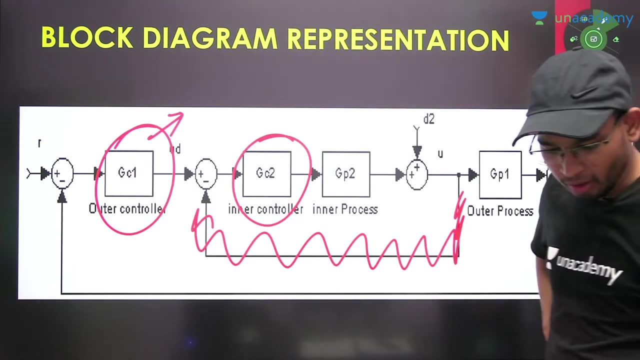 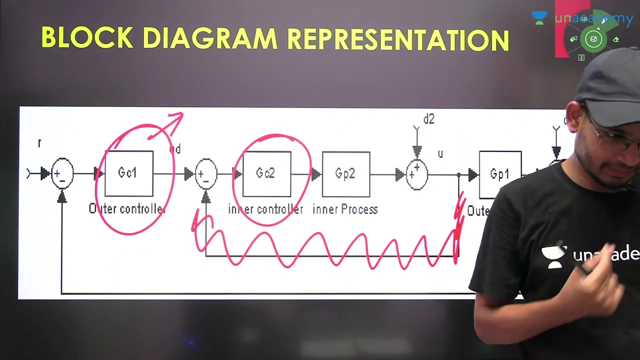 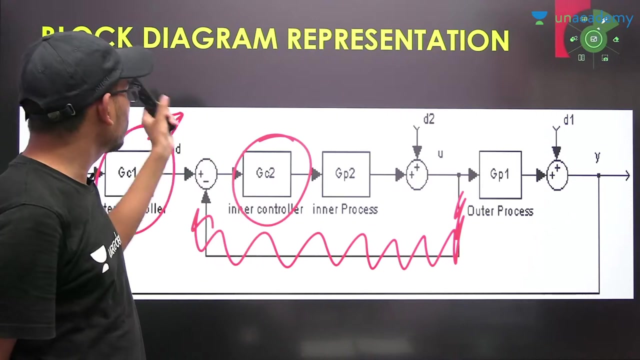 because it is solving the inner loop. that is the thing. what will happen. this is advanced control. it is fast, it is coming to everyone. all of you are getting it fine. ok, contractor, the building planner, the builder- clear, all of you have got the block diagram. 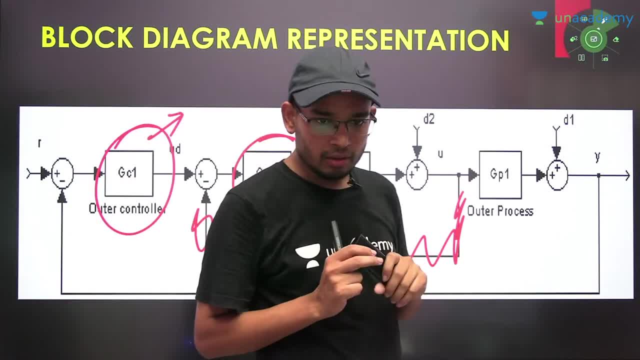 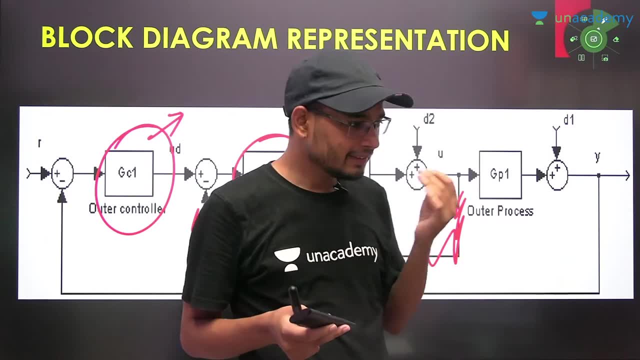 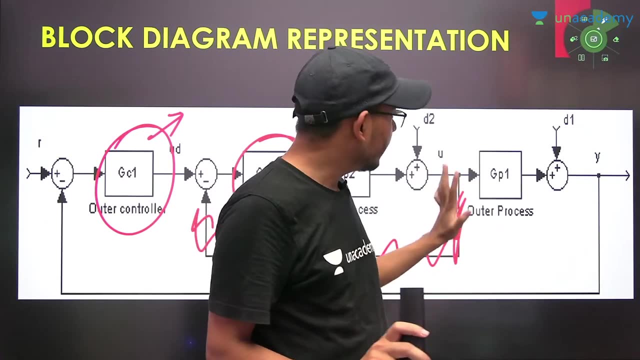 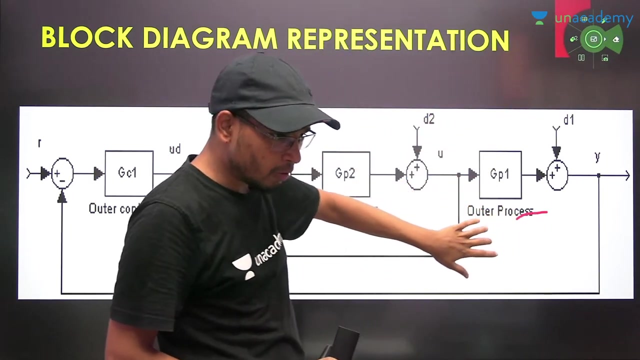 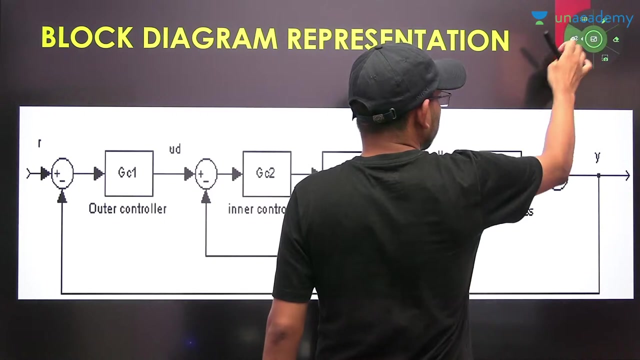 do you understand? block diagram is clear. say it, Yes, so it is the same thing. the block diagram came in a perfect way to understand. take clear, come on now. I move ahead. now. I give a question. I give a question, everyone will do it, come on. 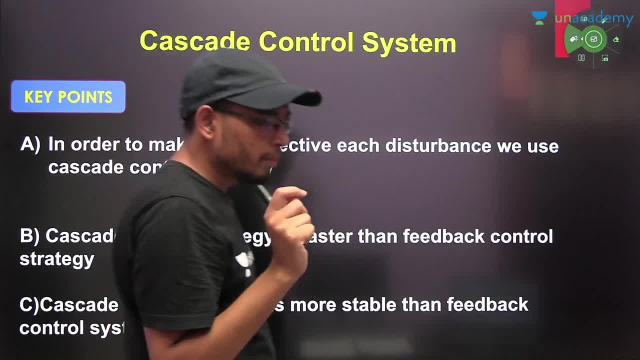 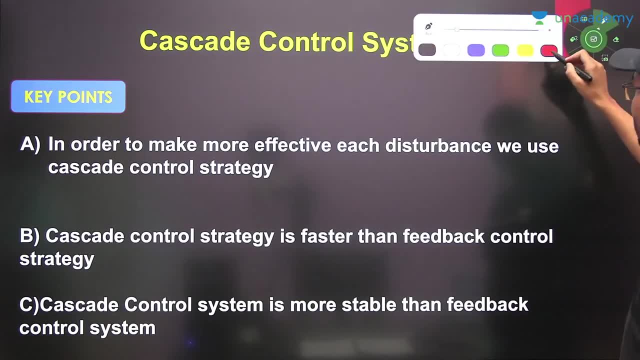 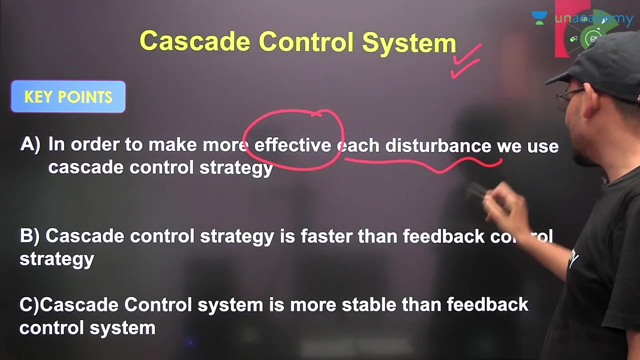 yes, write some key points in it. everyone read some key points. cascade diagram is beautiful. yes, see, everyone will write some points for the cascade control system. why will everyone write key points in the first copy? in order to make more effective, more effective for each disturbance. 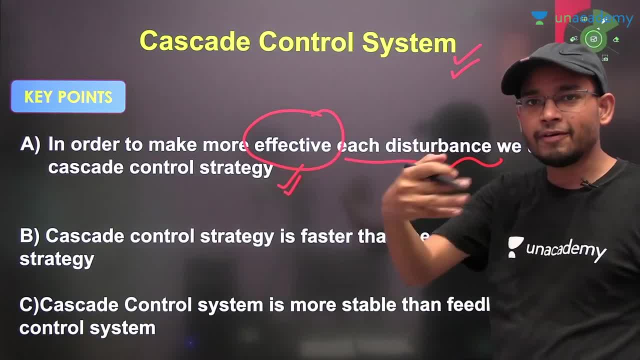 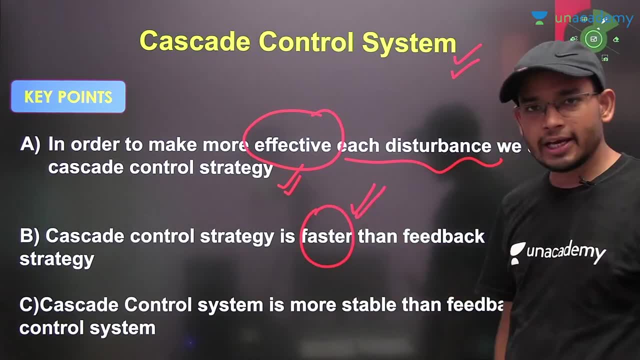 we use cascade control. why do we use it? because we make it more effective. okay, cascade control strategy. the faster than yes. obviously. what happens? it gets faster? okay, sometimes the question will come in one number. then you will do. cascade control system is more stable than feedback. then, 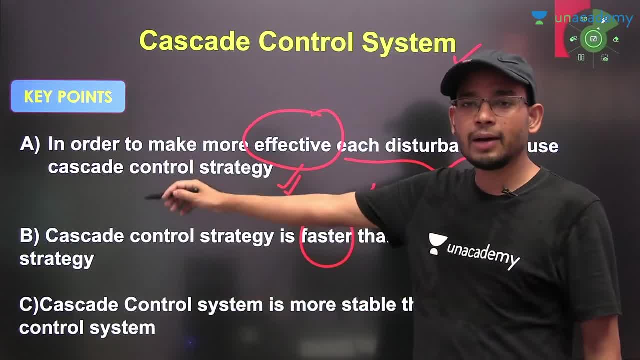 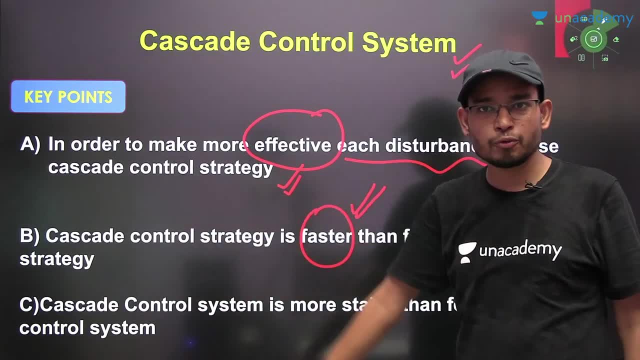 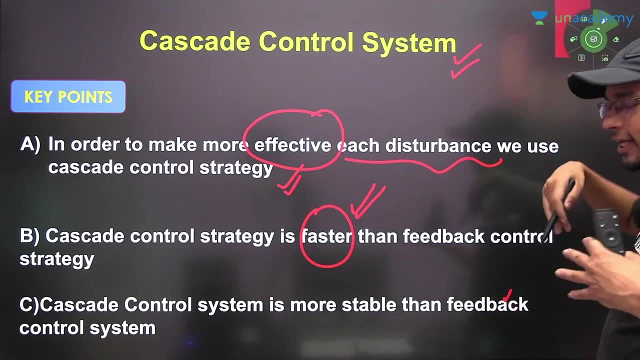 all three points will be written. okay, three points are important. it will be useful in your gate. you are going to give bark or nrl. you will ask such theoretical questions in the bark. write these three points quickly. right then? what happens with the cascading? what happens to our system? a fast? 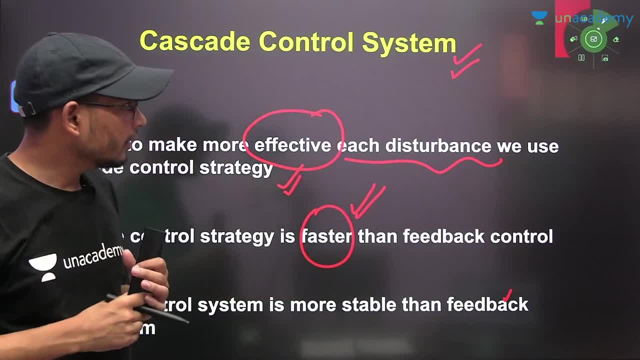 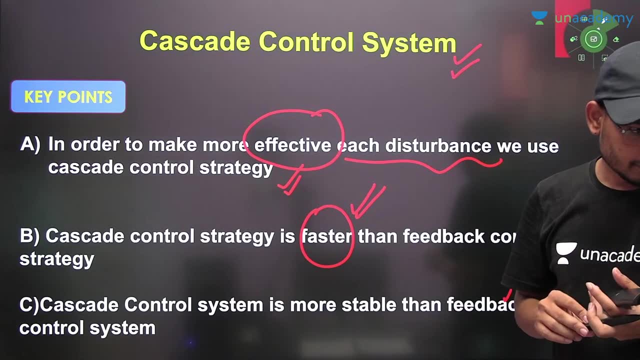 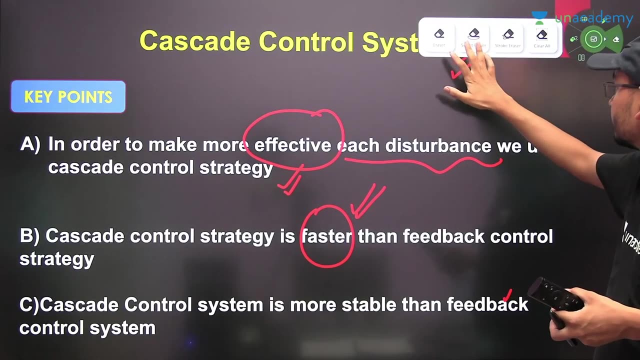 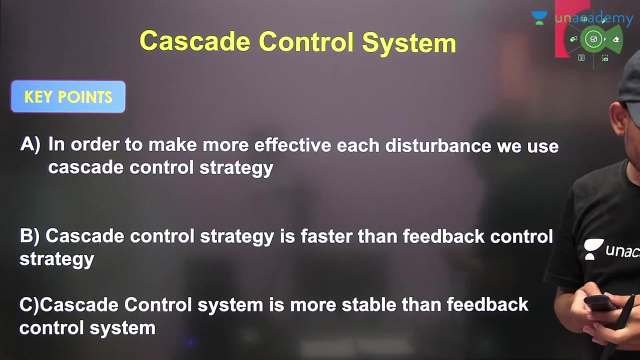 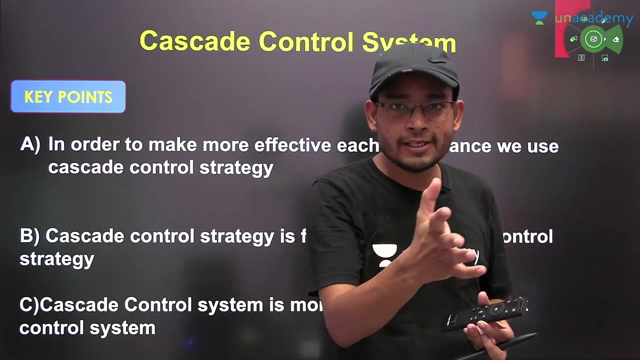 It works faster. It is more stable. It works faster. Write it quickly and then move on. Yes, feed forward is written. Feed forward is slow. Cascading is fast. Feed forward is. Cascading system is more stable than feed forward. 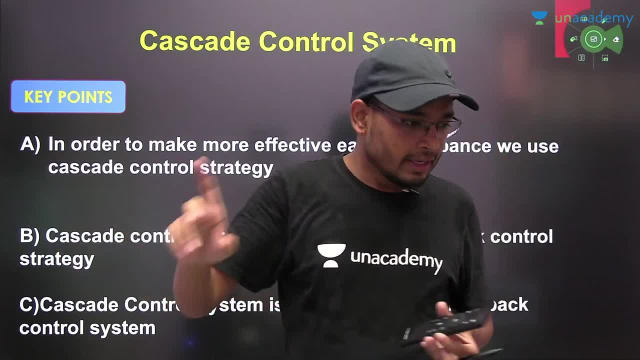 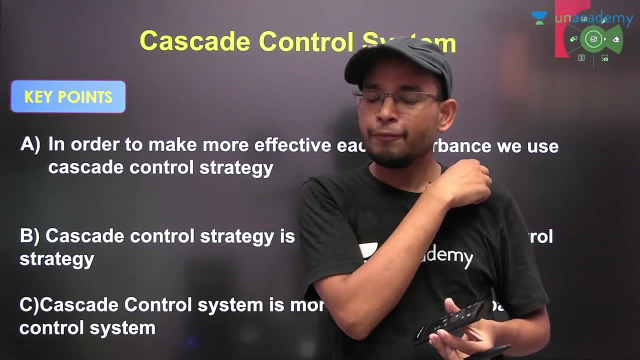 Are you talking about feed forward? We were comparing feed backward. Yes, feed forward is a different thing. You will compare feed forward and feed backward. You will not compare with this. What does feed forward mean? You will not compare with this. 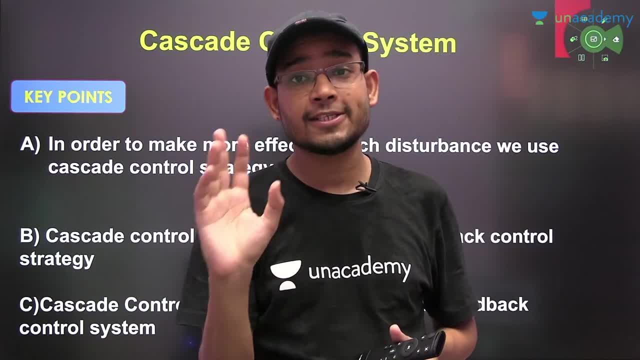 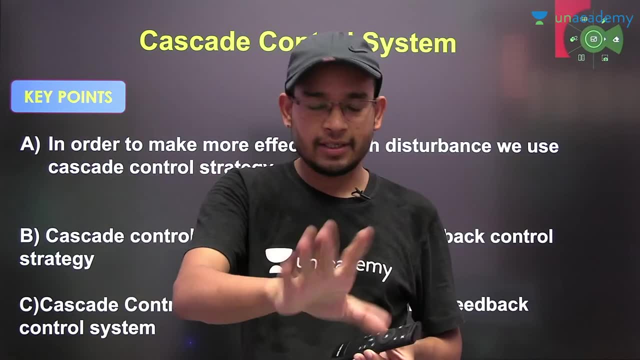 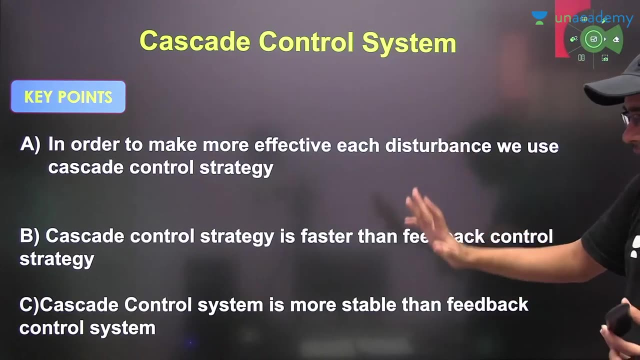 Cascading is the most fastest. Your cascading is the fastest. How will you compare feed forward with feed backward? You will not compare feed forward with this. We cannot compare from this. Everyone compares with a particular thing. You will not compare anyone with anyone. 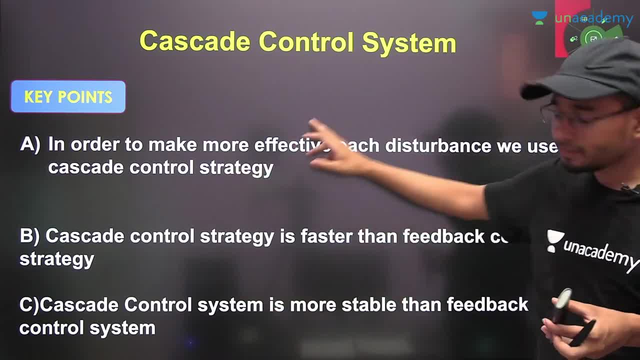 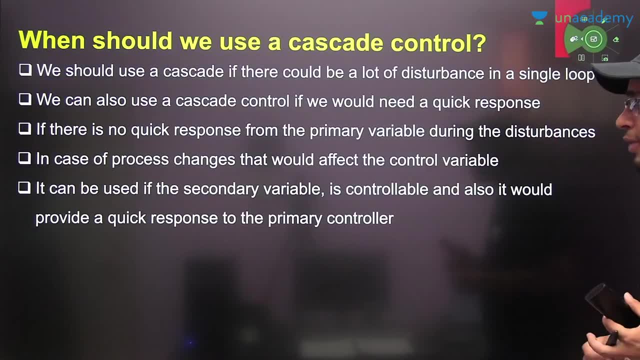 Done, Done. Have you written it? Done? Yes, Write some more points. This is quite theoretical. When should we use the cascade control? Write this. All of you will be useful. When should we use cascade control In case your system? 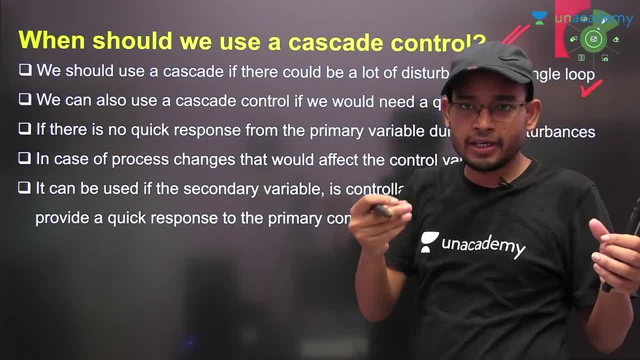 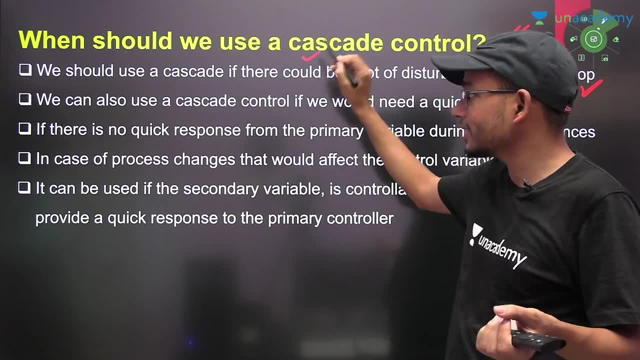 See, many things are coming. Disturbance is coming. What are you doing in your system? Many things are coming in the inner loop. Disturbance is coming. Then what do we do? We use cascade. Now you need quick response. 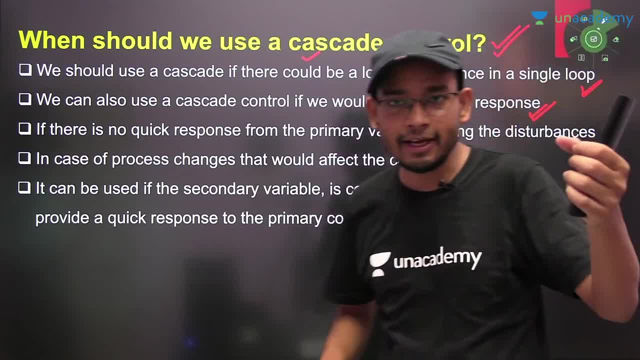 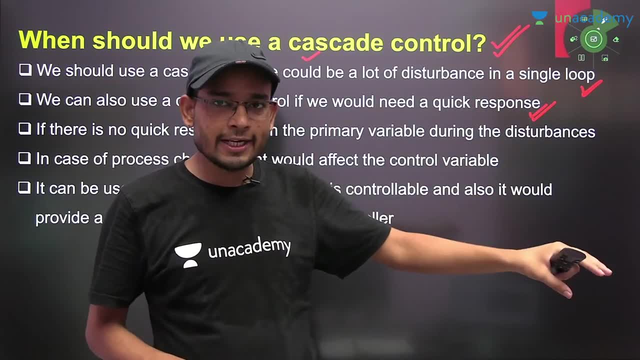 This means you need fast response. As I told you in the example, A person of the top level, In case he has installed many controllers. He has done cascading. By doing cascading, your response becomes fast, It starts working properly. 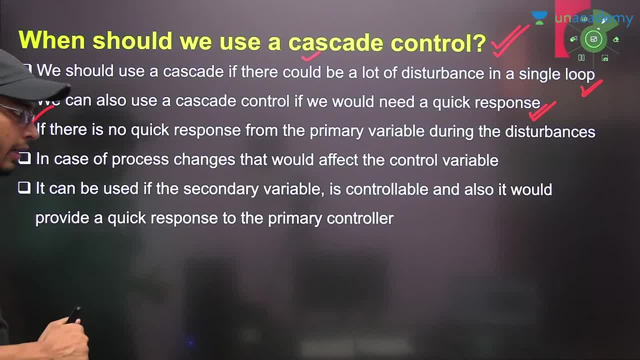 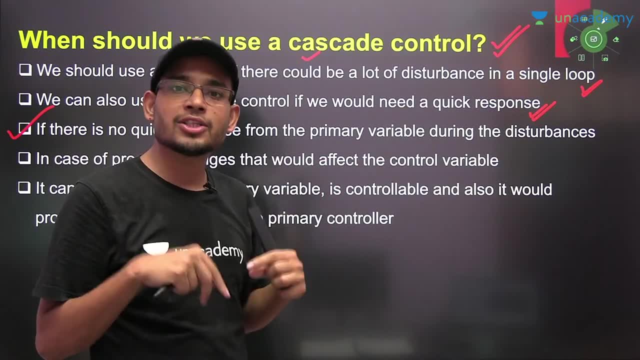 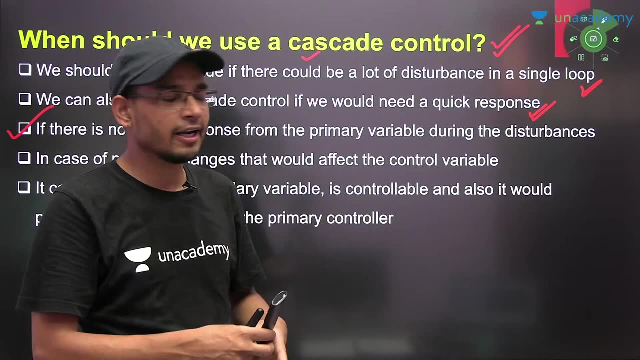 What is the third? Yes, Yes, Now the primary variable, The primary loop. What will happen? There will be a lot of load on it. There will be a lot of load on it. So it will not work quickly. The response will not start to be fast. 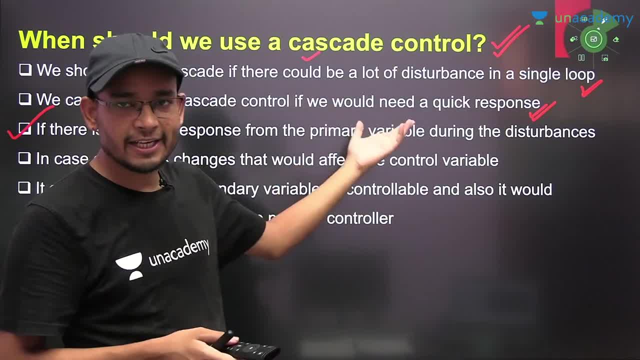 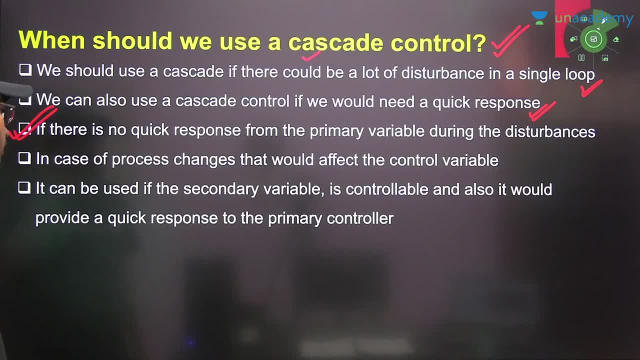 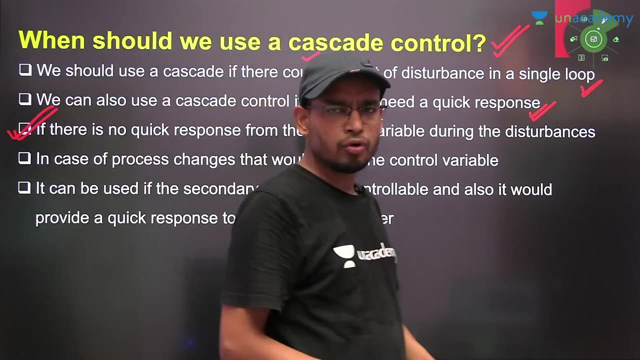 So what will you do at that time? You will do cascading, So that you can also make it fast. Third point: Yes, In case you have changed any process. You have changed any process And your system is affected. Your system is affected. 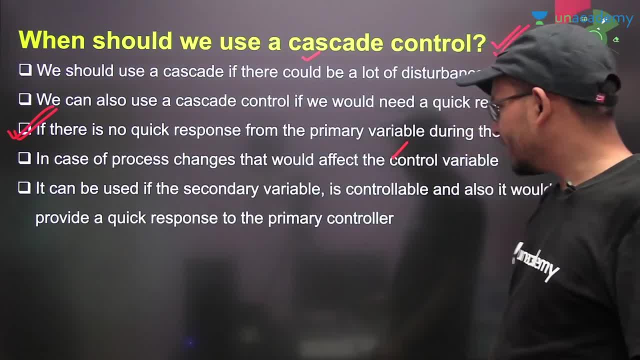 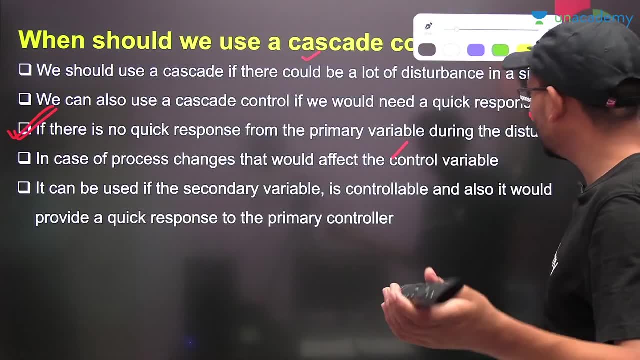 So what will you do? You will do cascading. Yes, You will write all these points. Your system will work, In which the main important is 1, 2, 3 is more important. This is theoretical. You know, It works for B Tech. 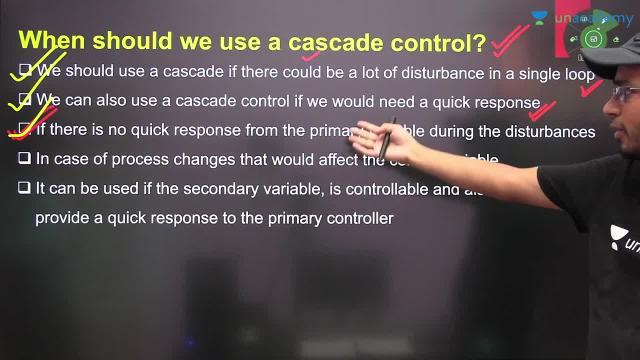 Who will be second and third year students. It will work for them And you can just have a feeling. Sometimes you are asked the question in interview. You can tell a little about them. Hmm, So when you use the control secondary variable, 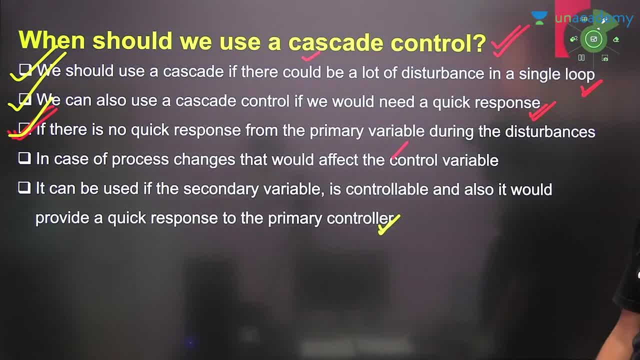 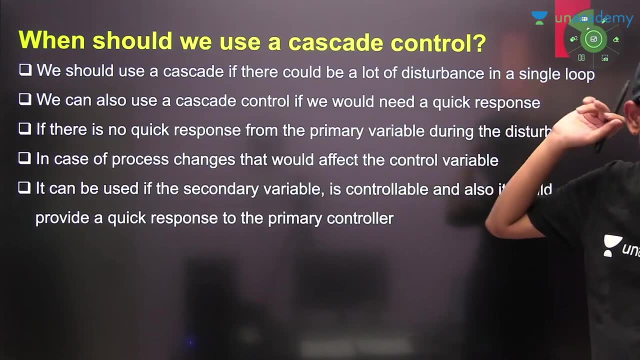 So your primary variable controller, What does it start to do? It starts to make a quick response. Okay, So this was when should we use the cascading control? Have you written it? You must have written it So quickly done. 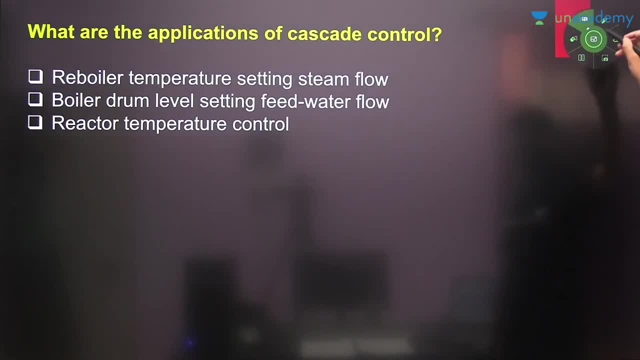 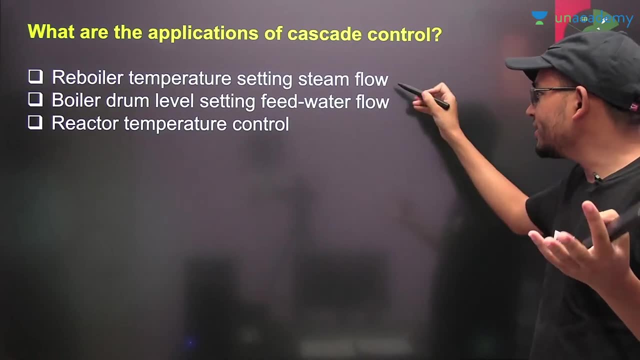 Done Very good. What are the applications? Write the application also quickly. What are the applications? Like your re-boiler, In the re-boiler you have to maintain the flow rate of the steam. Then you will use it. You will use it in the boiler drum. 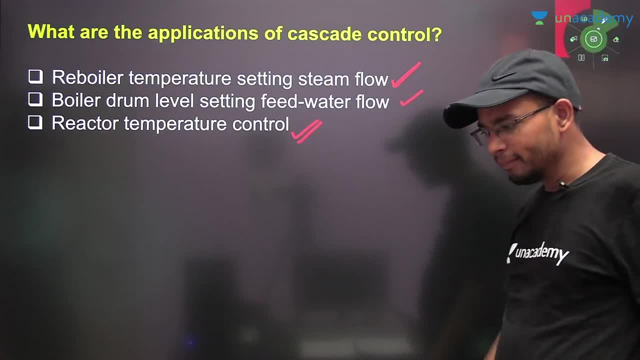 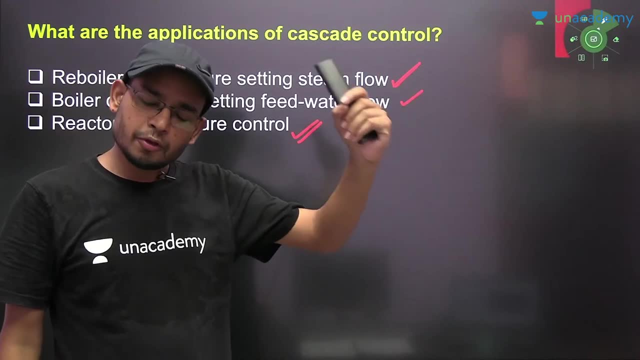 You will use it in the reactor temperature. All this is done in the distillation column. You do cascading in the distillation column also. Distillation column is done, Your heat exchanger is done, So what will you use there also? 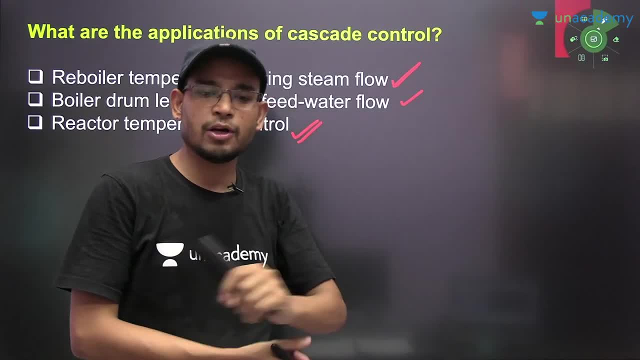 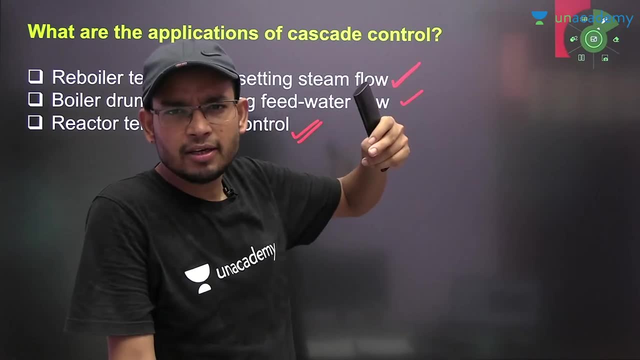 Cascading. If you get a chance, then I will explain it to you with one more example. I have just explained it with liquid level tank and this, If you get a chance, then I will explain it to you with distillation and heat exchanger also. 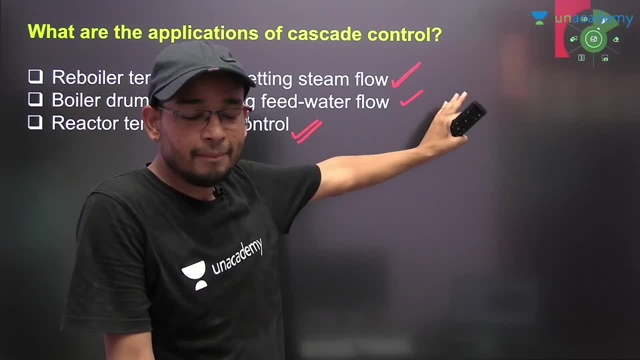 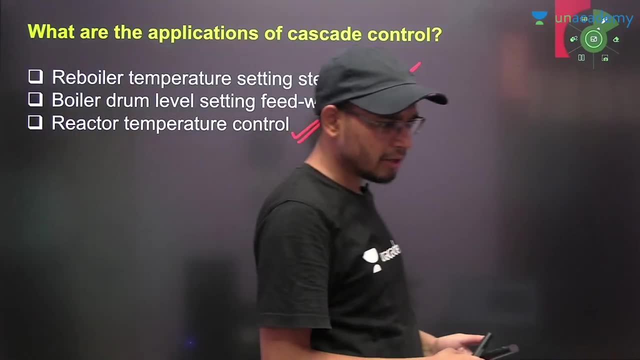 How does the role of cascading come from distillation And how to use heat exchanger. How does the role of cascading come from distillation? I will also talk about this in the future. First write the application properly. Distillation column is used everywhere. 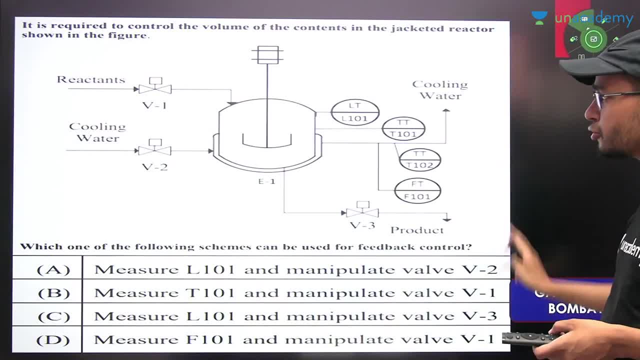 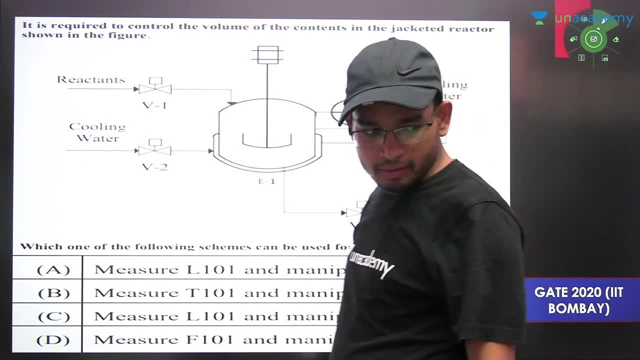 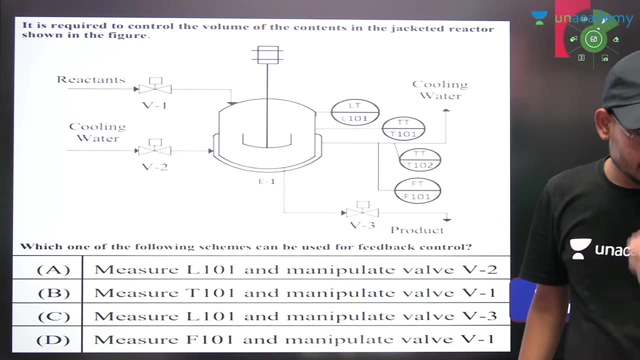 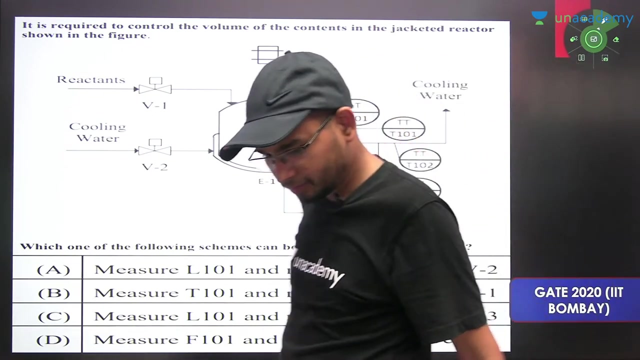 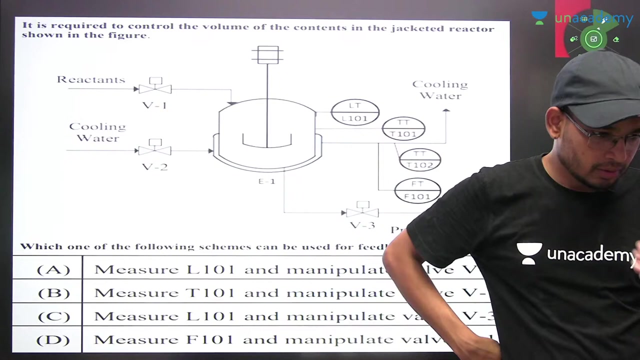 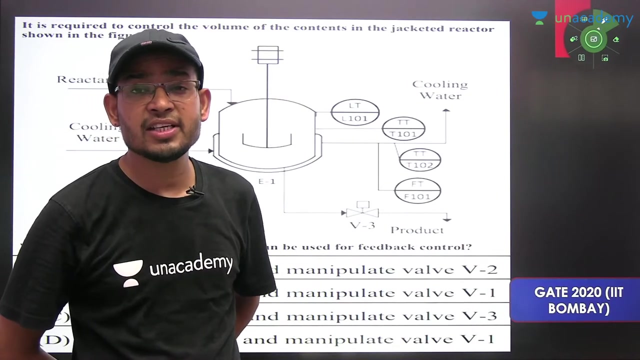 Now let's do some questions. First, do this. Someone asked me to do this question. Let's do this properly: Done, Done, Done. All of you do this In a nice way. PYQ practice for IPC. Not only PYQ, I have also asked questions for the textbook IPC. 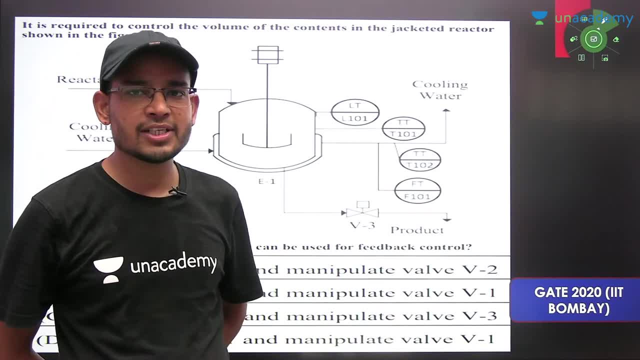 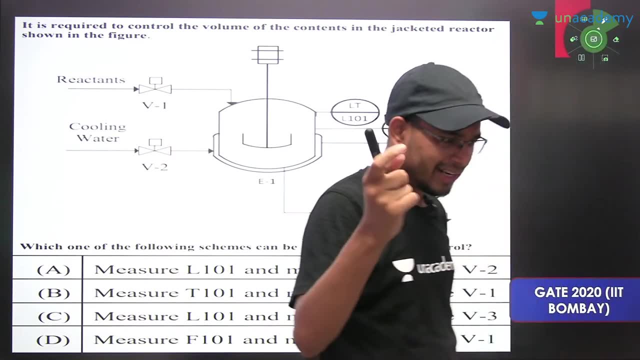 I have taken questions for the textbook session. You can go to my profile. You will get there. Okay, I will also talk about the plan for tomorrow. I will also talk about what is the plan from tomorrow. Yes, it is 2021.. 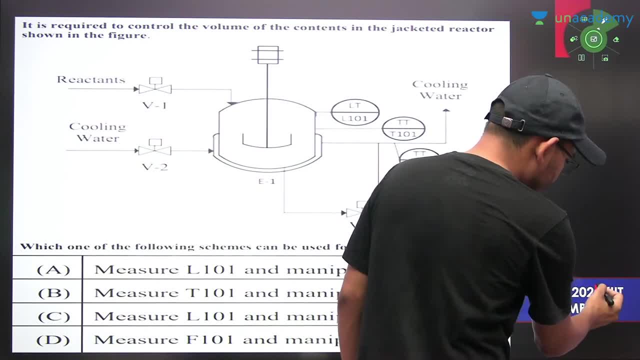 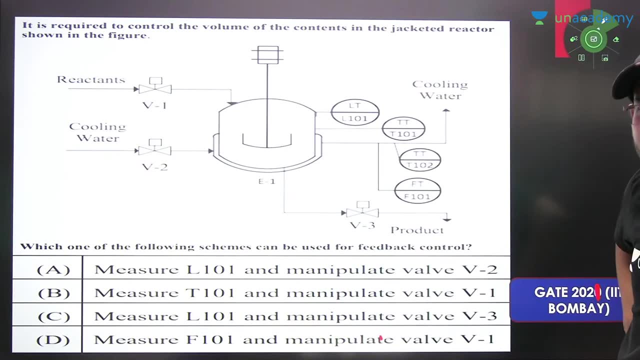 Yes, yes, it is 2021.. It is 2021.. Come on, All of you try this. This time. it has been asked. This is the latest. What is the main point of this question? All of you first tell this. 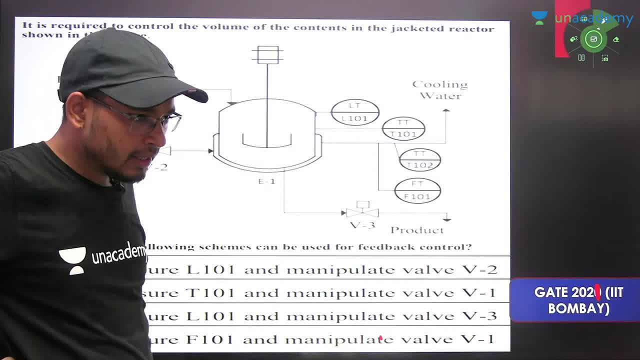 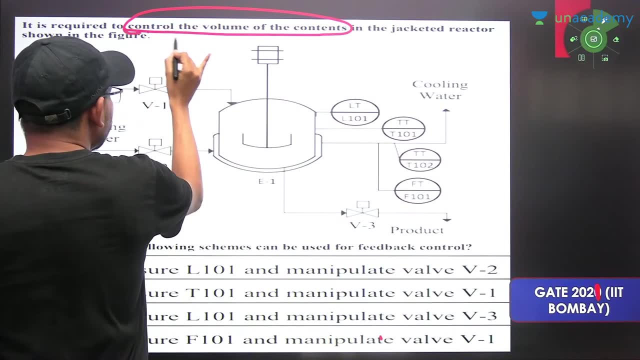 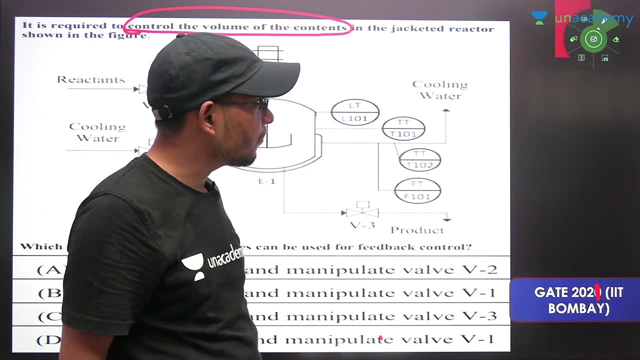 What is the main clue of this question? What is the main clue? Control the volume of the contents. Okay, What you have to do is to control the volume. You have to control the volume. All of you try it. See if you are able to make it. 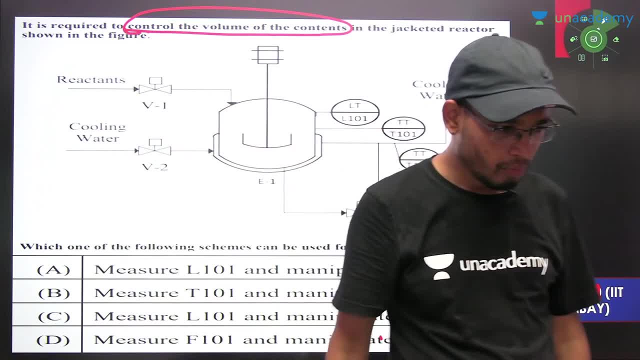 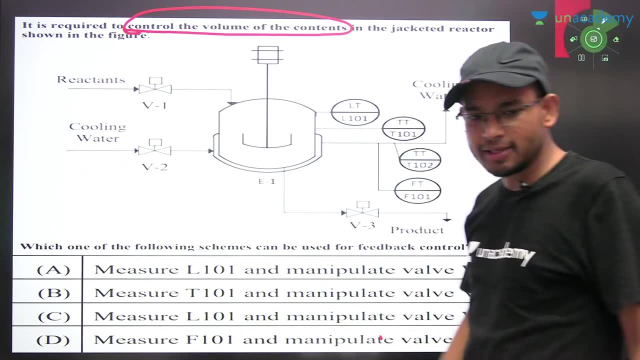 Are you able to make it? See all of you quickly. The answer will be: What should come first? First, think a little yourself, Think for yourself. That's when it will be done. Otherwise, I will get it done and go. 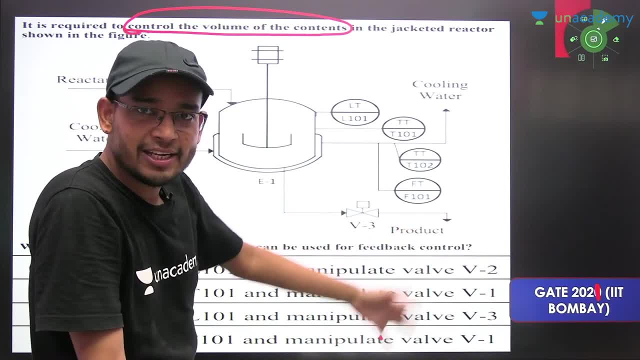 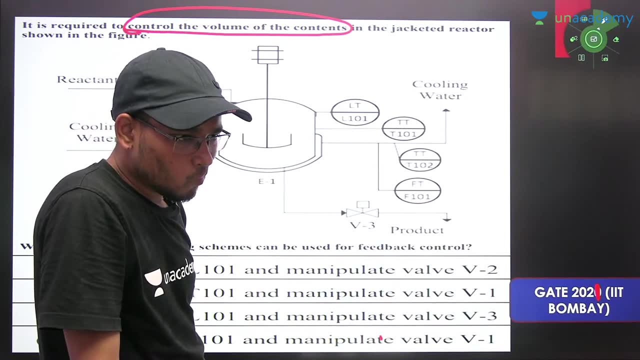 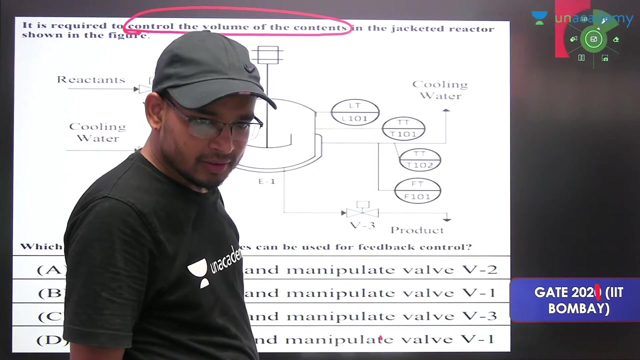 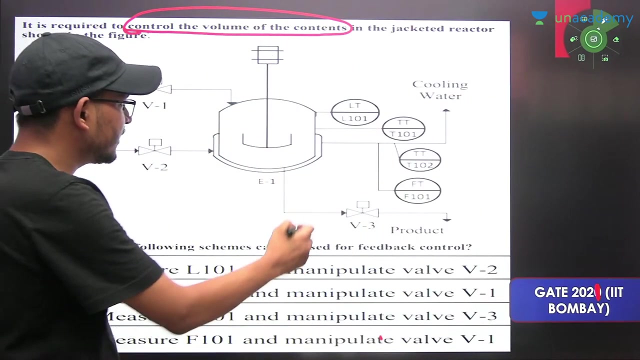 Think for yourself a little. This time. it has been asked. I have given you a hint. See, Come on, Let's do it. Reduce the brightness a little. By the way, it must be visible. Reduce the brightness, Come on, I will write it here. 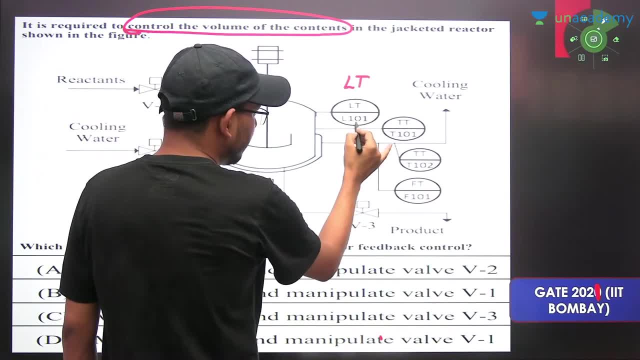 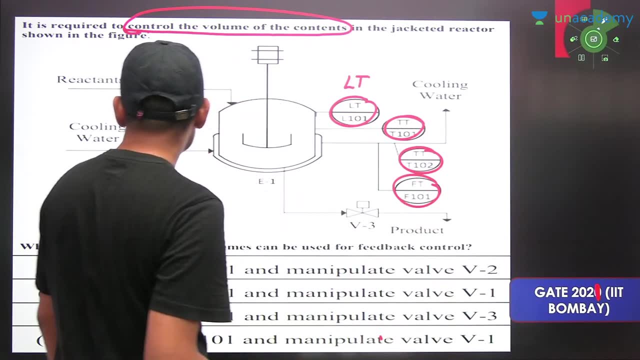 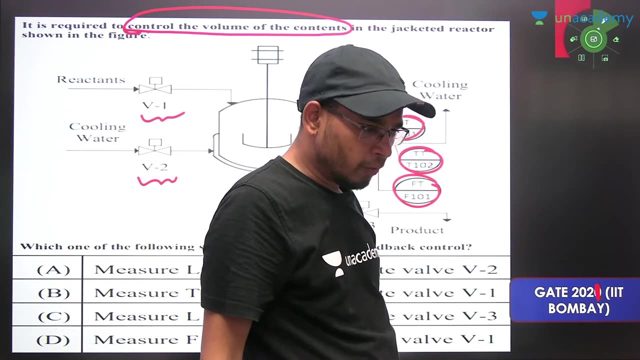 This is your LTE level 101.. This is the temperature controller. This is the temperature. again, This is for the flow. This is your V2.. This is your V1.. This is visible. Come on, See what we have to do. 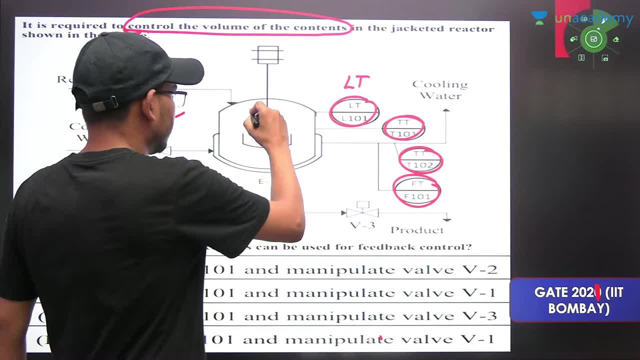 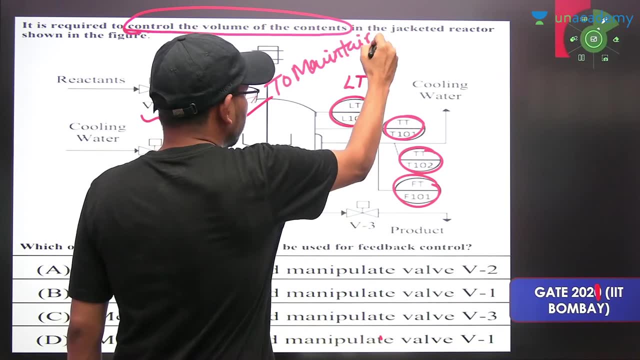 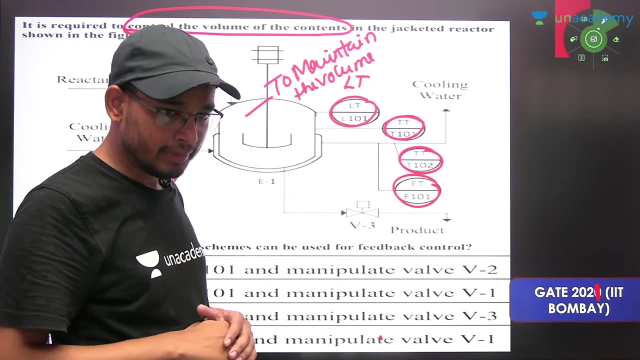 This system has to maintain the volume inside it. To maintain the volume. Maintain the volume, Want to maintain the volume, First thing that is important. What are you going to think about in this? What to do? Maintain the volume? How will we maintain the volume? 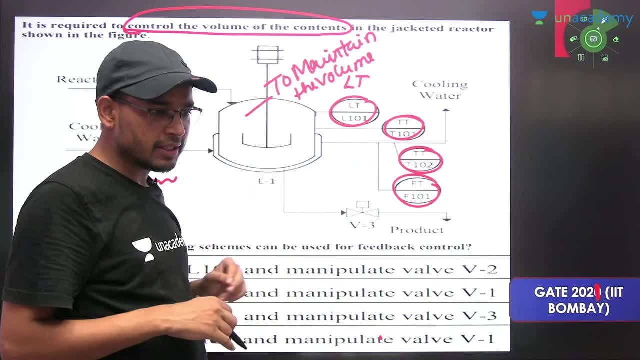 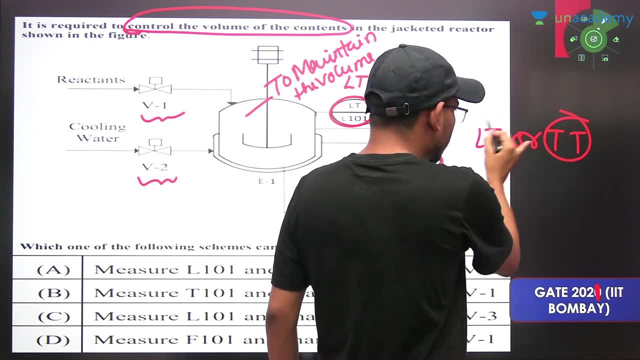 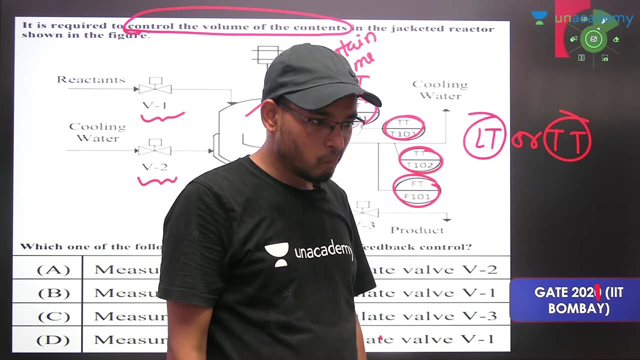 Tell me this. By level transmitter or temperature transmitter? Tell everyone. By LTE or TT, By LATE OR TT? Tell everyone. will you measure it with ELAT or TT? tell me, will you measure it with ELAT or TT. 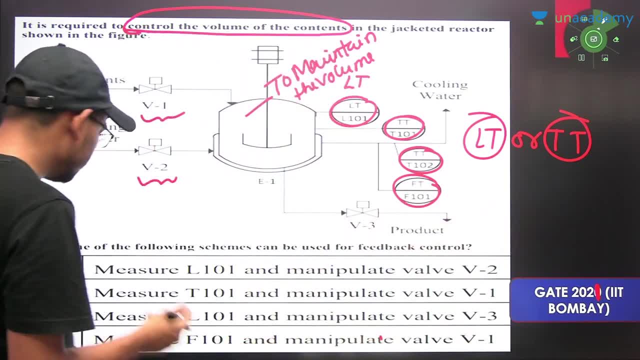 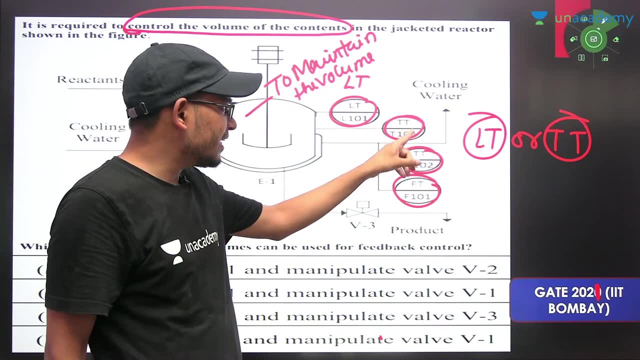 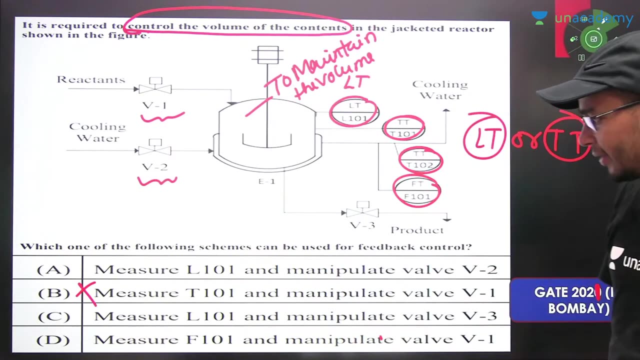 you don't have to measure the temperature. so finish the TT part, finish the B part as it is, because the temperature is 101, the temperature 101 has no meaning because we have to maintain the level, we have to maintain the volume, so you have to measure the level. 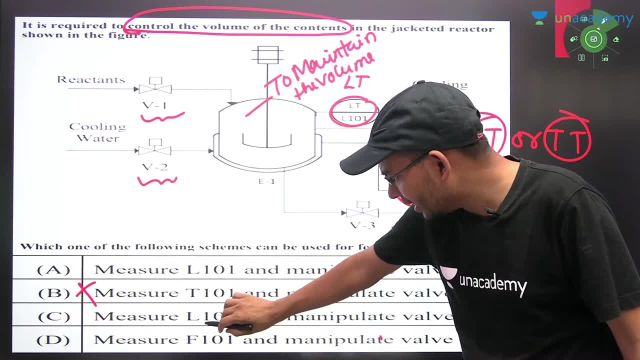 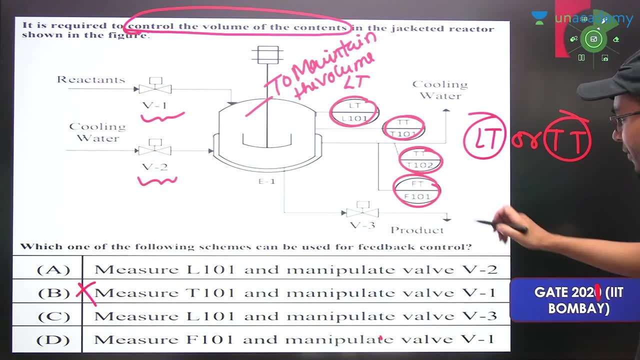 okay, now EL101 and EL101, and this is F101, F101- okay, what is F101?? first understand the fourth option, what is written in D part, F101. so tell me what is the flow rate of coolant? will we measure it to maintain the volume? 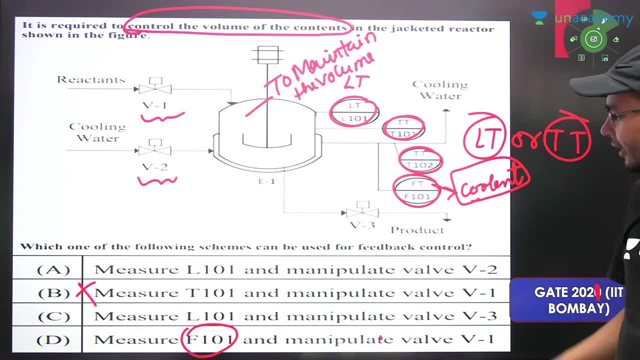 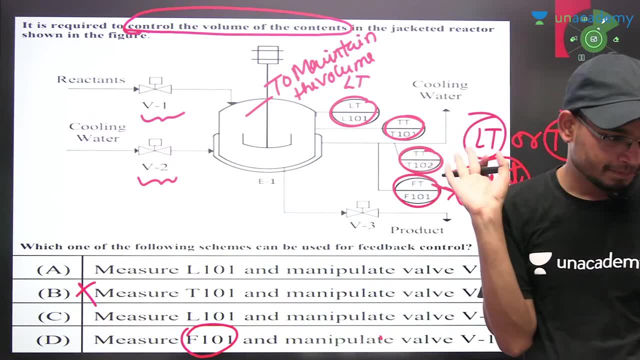 will we manipulate it? will we maintain it? because? because what is this? this is the flow rate of coolant. so the flow rate of coolant? there won't be any effect in its volume. tell me who is this? the flow rate of coolant FT. FT means the flow rate of the coolant. 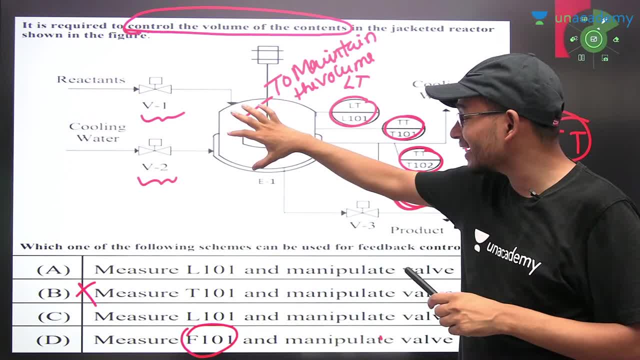 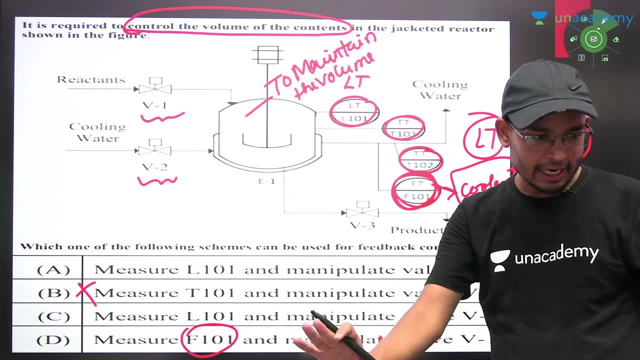 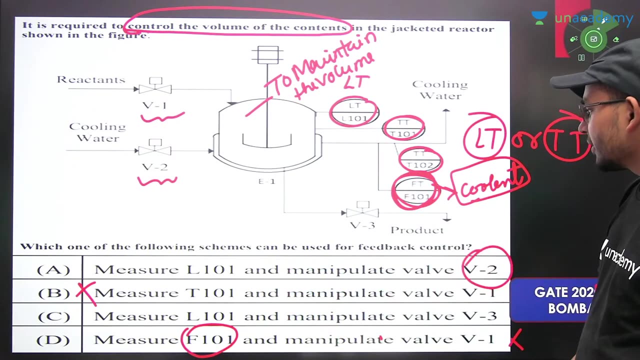 so we don't have to maintain the volume of coolant. who has to maintain the volume of the reactor? so this is wrong. D part, D part is wrong. okay, all of you do wrong first. now come measure the L101 and manipulate the B2 ball, all of you tell me. 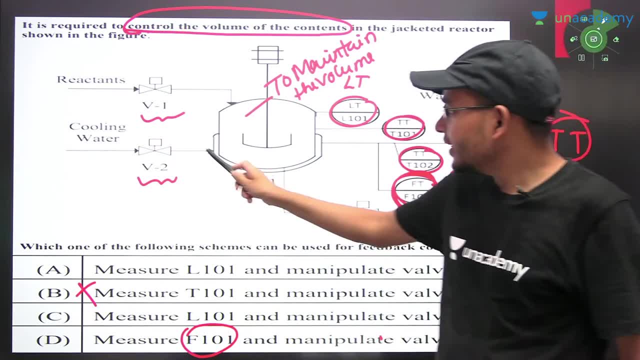 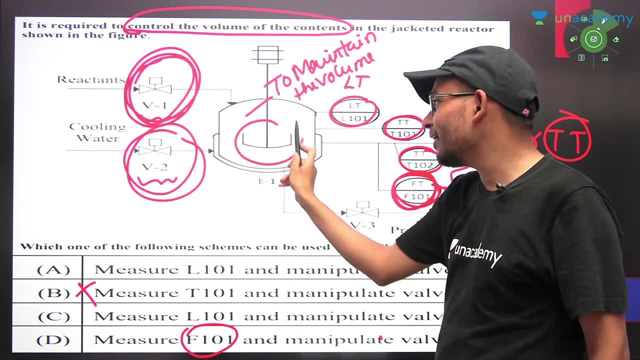 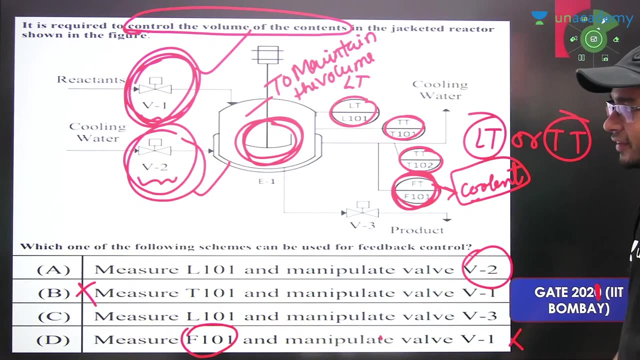 what is B2 ball? yes again, will we manipulate the water of coolant or will we manipulate this one brother to maintain the volume inside it? all of you tell me, will we manipulate B1 or B2?? all of you tell me, will we manipulate B1 or B2?? 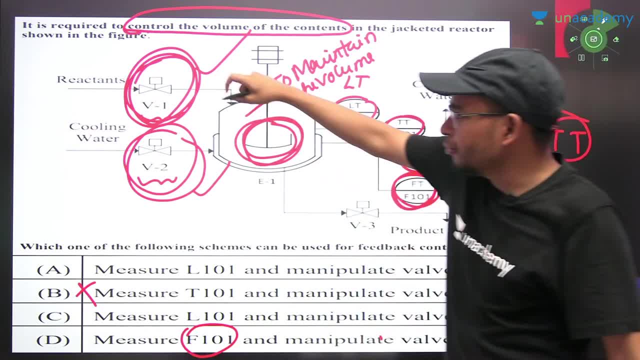 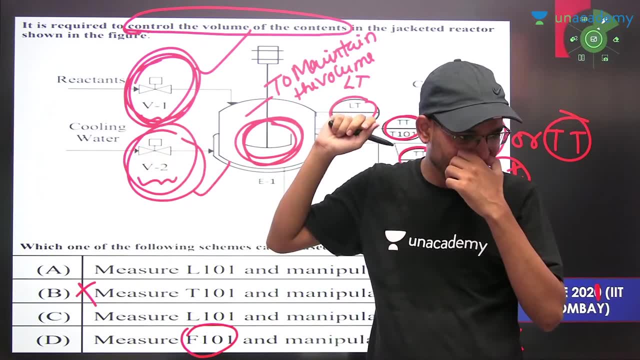 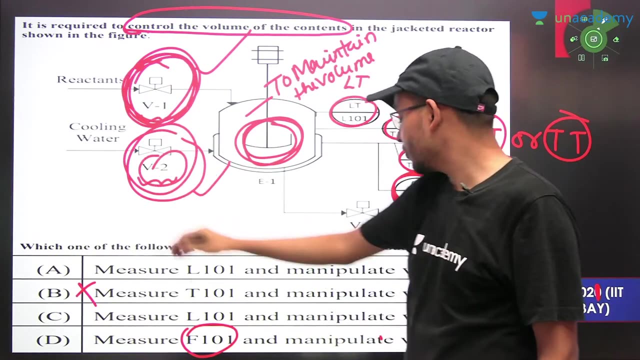 tell me. you can manipulate the ball manually, but not in the manipulated variable. it is a manipulated valve. you can open and close the valve. all of you will do B1. you will do B1 because this is a direct reactant and who owns this? we won't do B2. 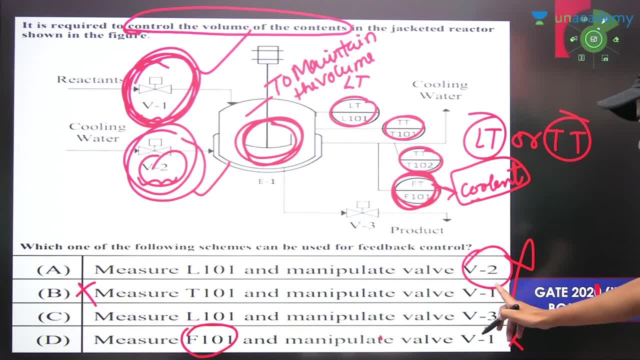 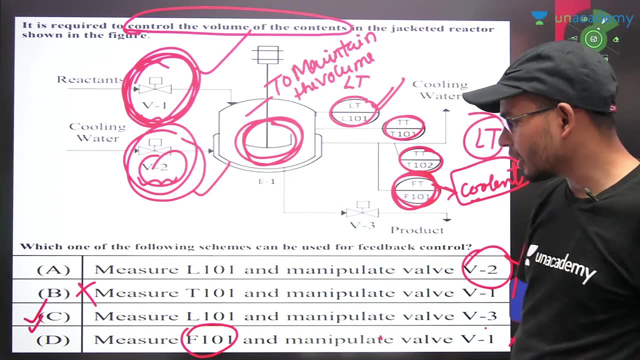 so first cancel the B2 ball. so A part is wrong, A part is wrong, B part is wrong, D part is wrong. what is left? C you do wrong. now make the C right. check the C right. L101, what is L101?? you should know the level, then only you will be able to control the volume. 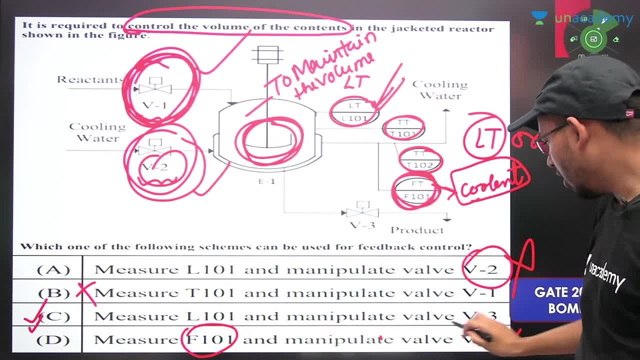 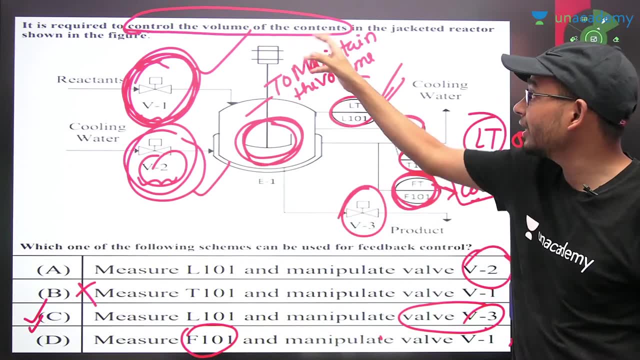 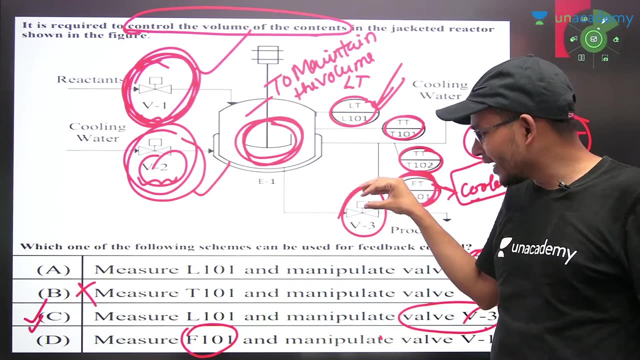 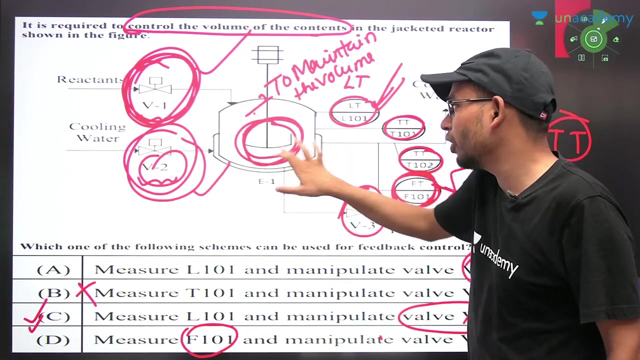 and the manipulated valve is V3. by manipulating V3, you will be able to control the volume and maintain the volume. by reducing V2, the volume will be disturbed. this means, with the help of V3, you will be able to maintain the volume. so the answer will be C part. 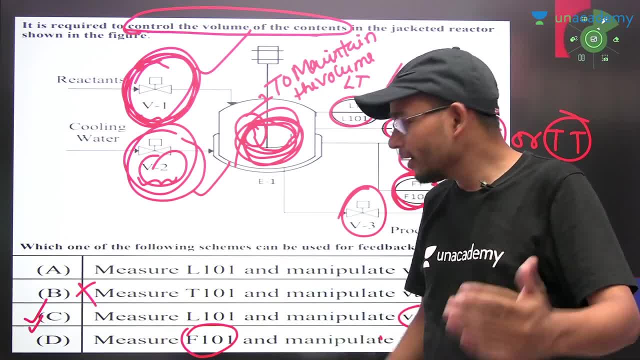 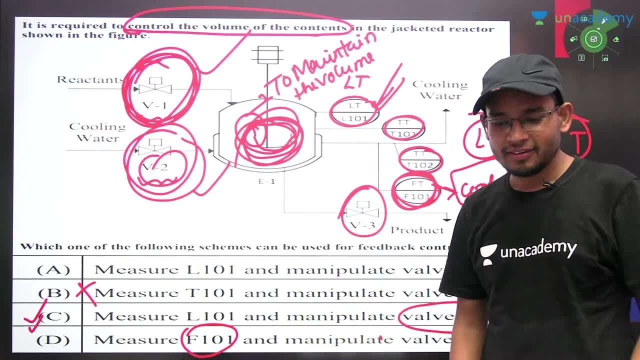 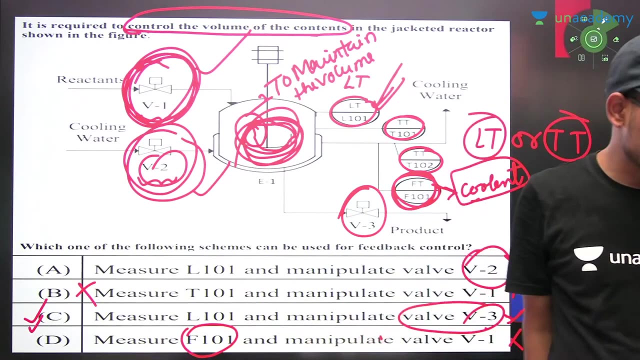 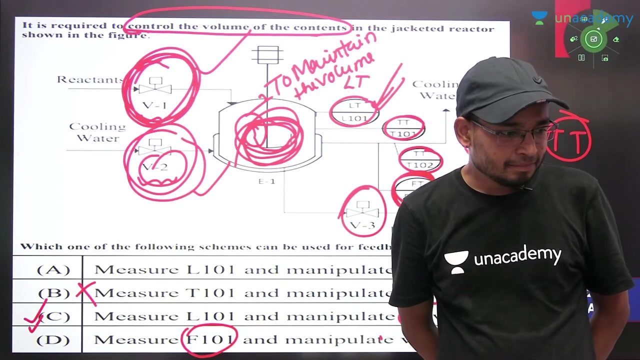 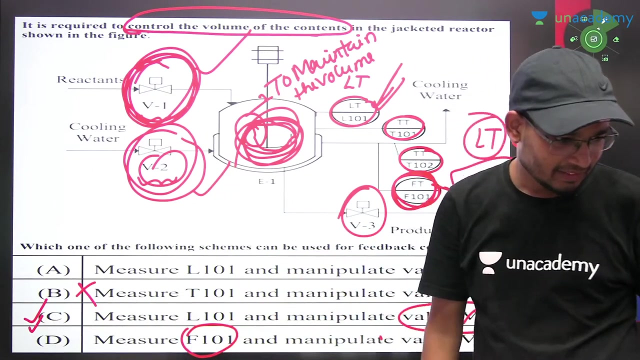 everyone understood C part and did you understand the 3 wrong options? it is important to understand. if it was coolant, then we would have talked according to it, then we would have seen the coolant. it should be clear that why it is wrong. it is a theoretical question. 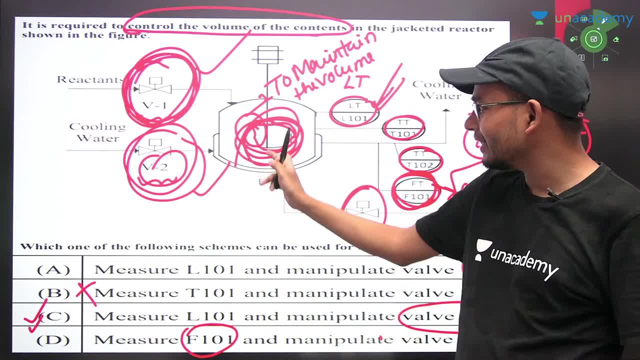 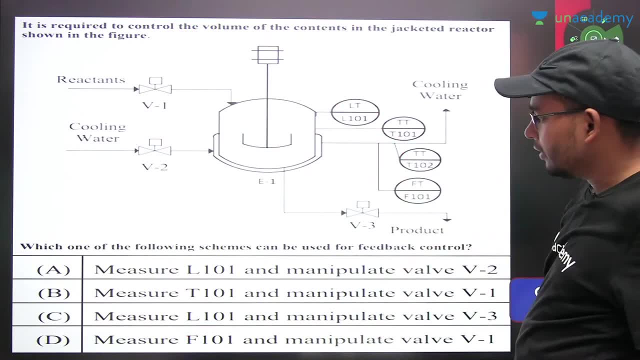 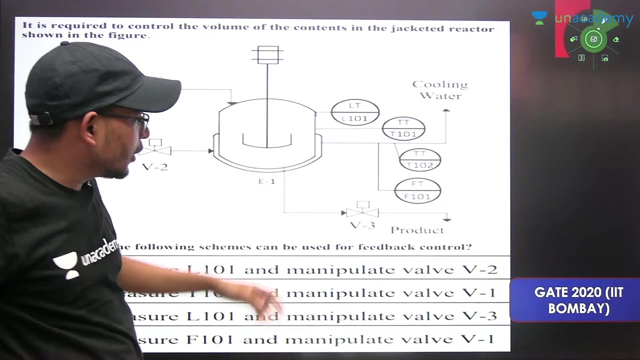 yes, we should understand why it is wrong, so always pay attention to the wrong part. if it was coolant, then what would we have done for coolant? let's talk about coolant. if it was coolant, then what would we have done? if it was coolant, then what would we have done? 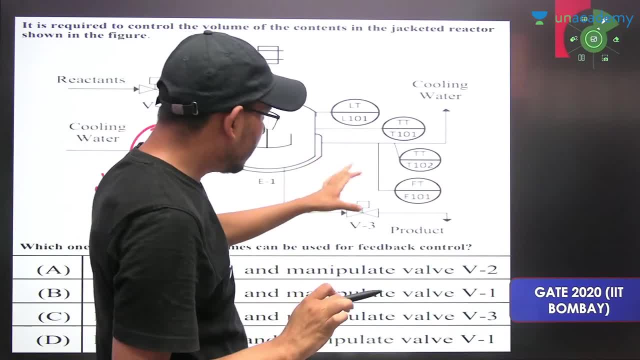 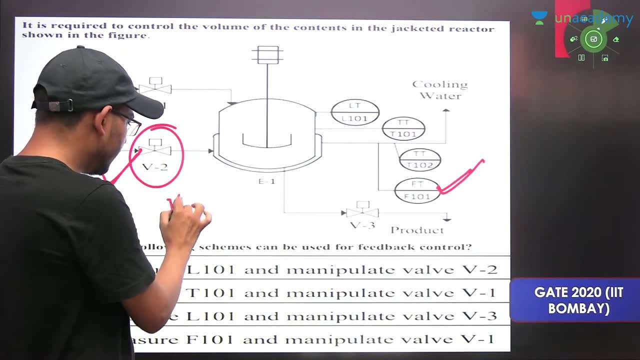 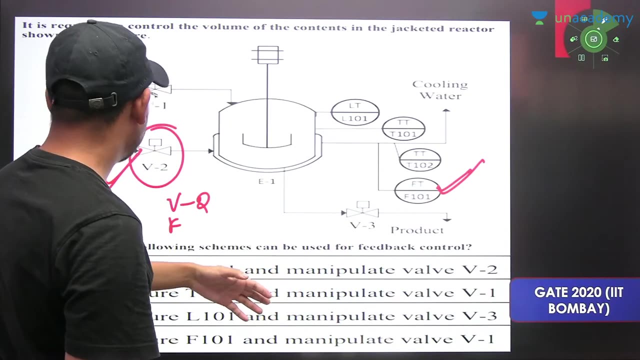 its flow rate would have been V2, in case the coolant would have to work this one and this temperature and this flow rate, FT. so FT and V2, V2 and FT- what is this? F101 and V1, V1? yes, there is no option in this. 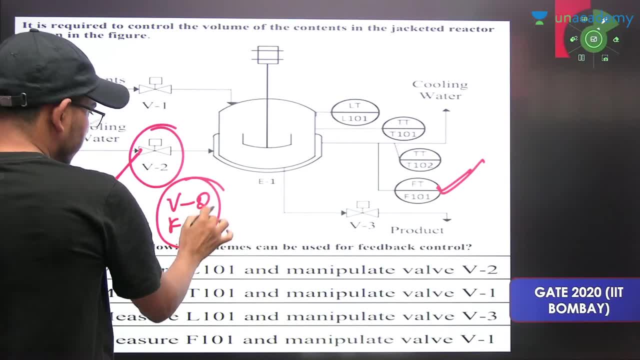 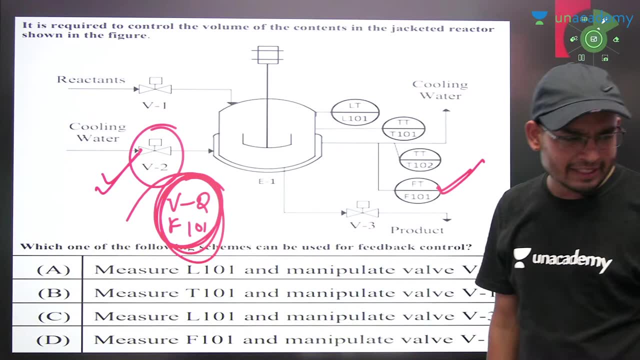 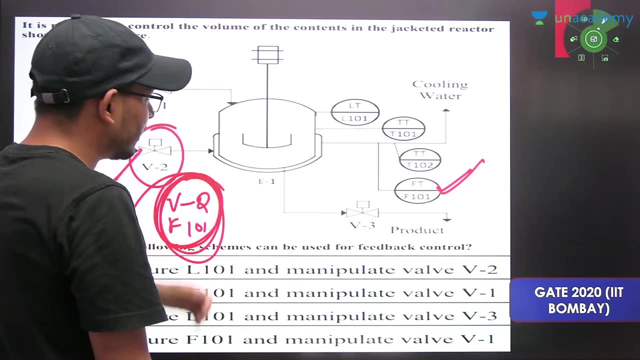 so this is V2 and F101. in case of coolant, you have to maintain this one. if it was temperature, then let's talk about that too. let's talk about that too. okay, let's talk about that too. they have to maintain the temperature. so what happens? 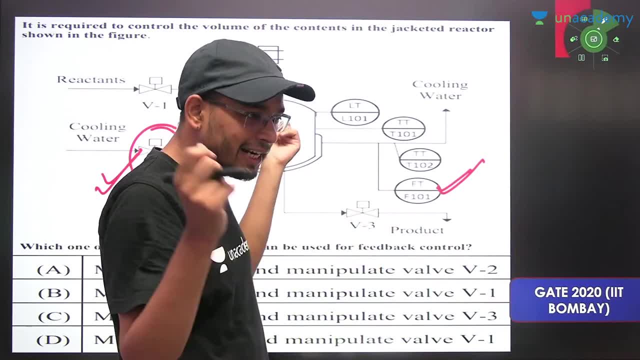 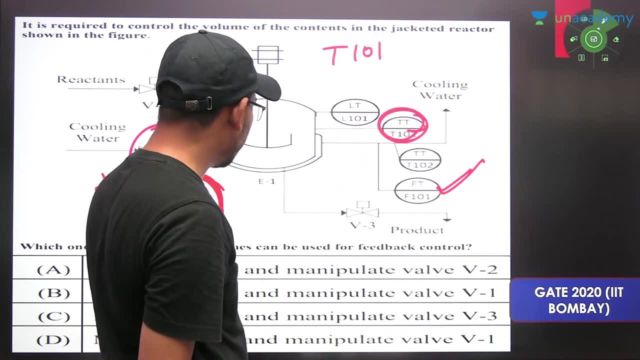 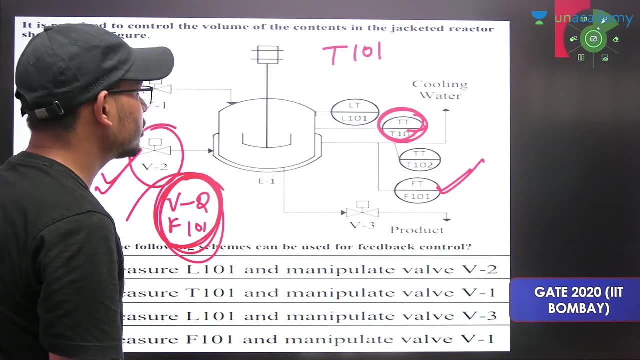 see, the temperature is 2. now you have to maintain the temperature in the reactor. so what you have to do is T101, understood T101? and what else is there to maintain the temperature? yes, for temperature, everything comes. for temperature, everything will come, you know. for temperature, V2 will also come. 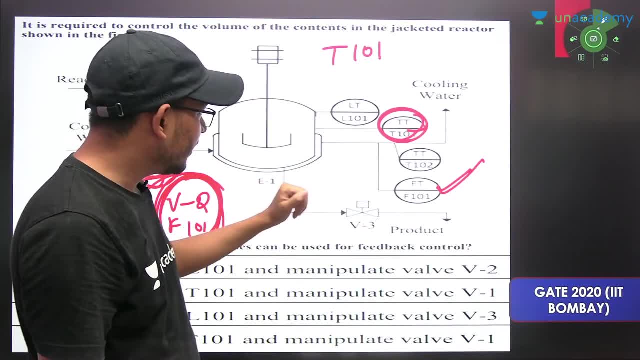 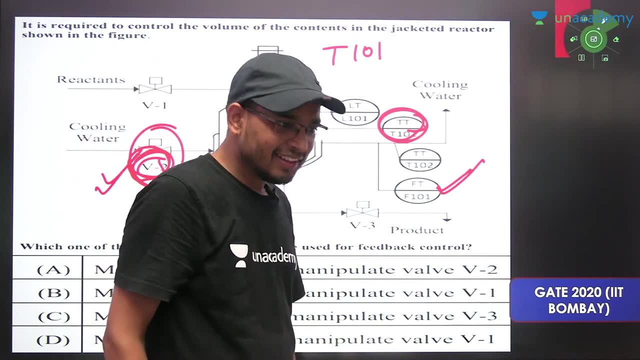 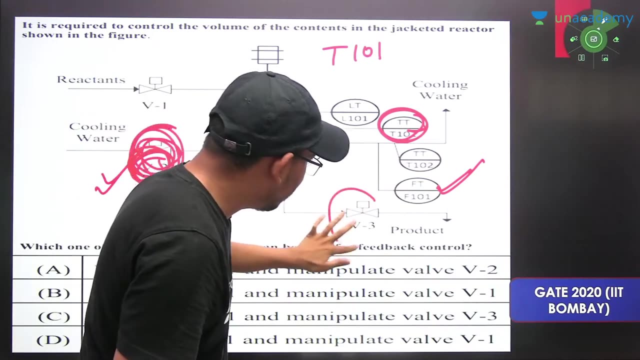 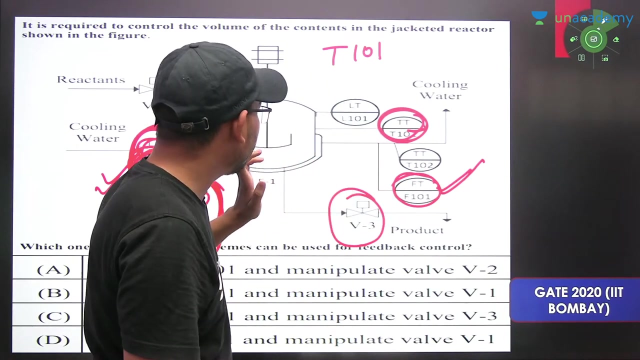 because, according to V2, you will also have the temperature of this. okay, everything will come for temperature. everything will come right because the flow rate of coolant will change. then it will come right. you have affected this V3, then also it will change. okay, the flow rate of the output you took out will also be affected. 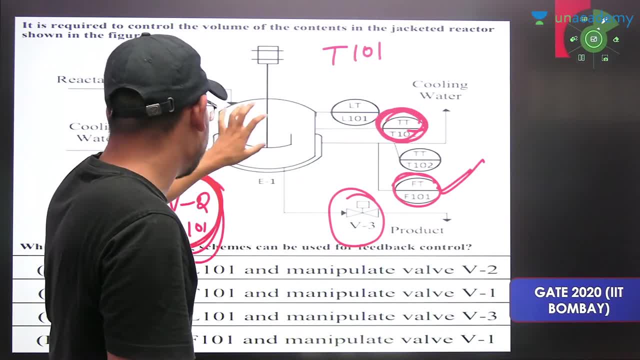 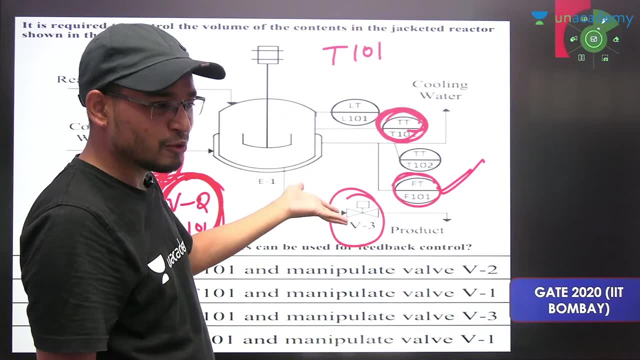 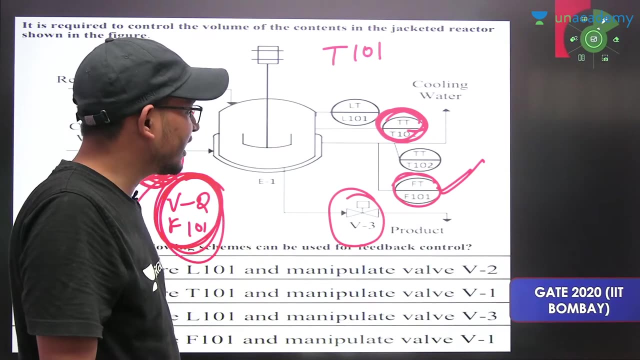 okay, this will also work for you. yes, for temperature. because of this, also, the temperature will change. okay, because of this, they have given so much brain. you are asked about the volume. it is a game for temperature. okay, it is a game for temperature. yes, many possibilities for temperature. 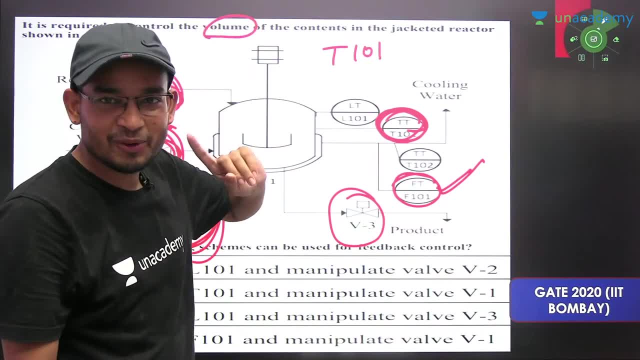 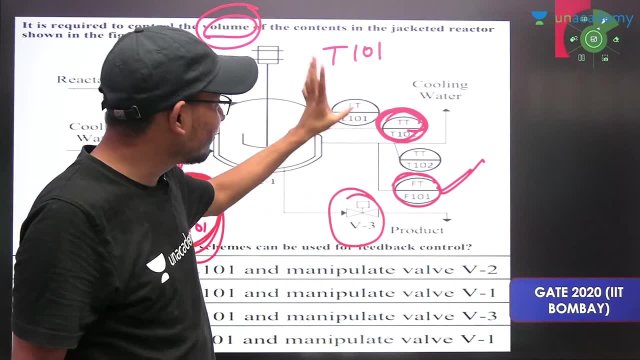 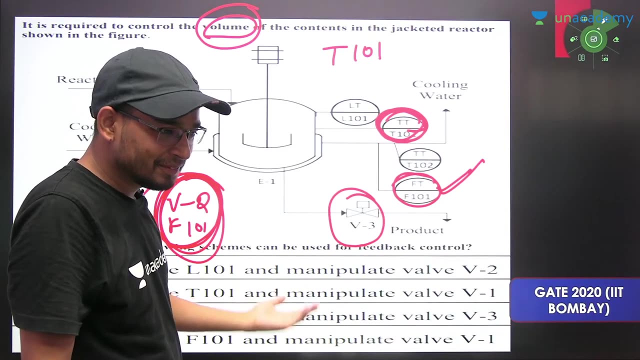 that is why they are giving only volume. they are very smart people. okay, they are very smart. they said: no, brother, we don't have to study so much in Jamele. tell us the volume directly, okay. so you must be getting the point. you have to understand. you must be getting the point. 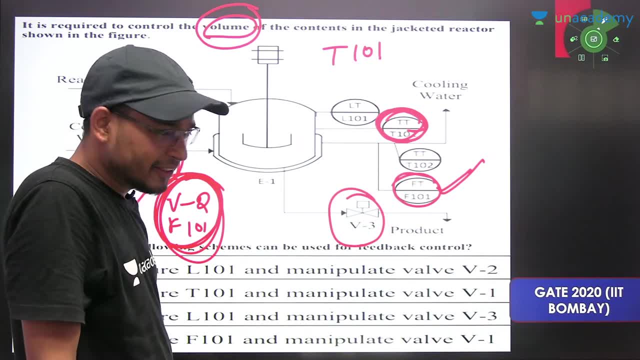 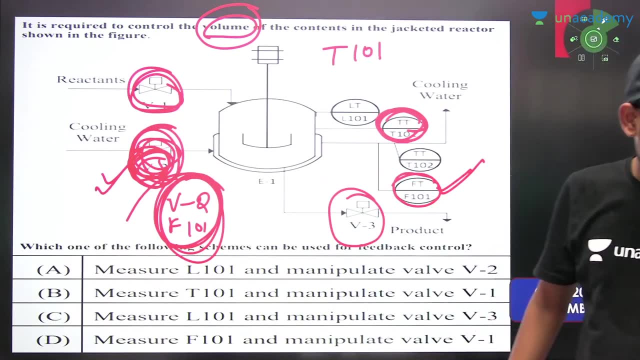 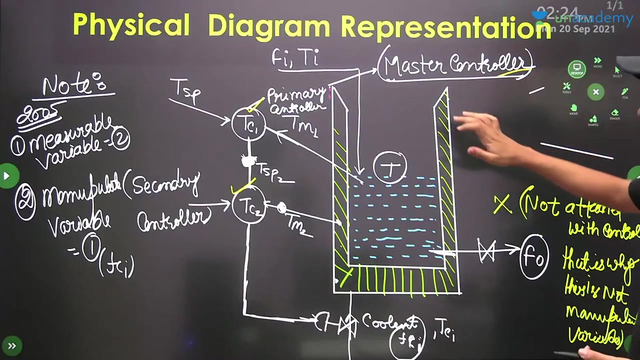 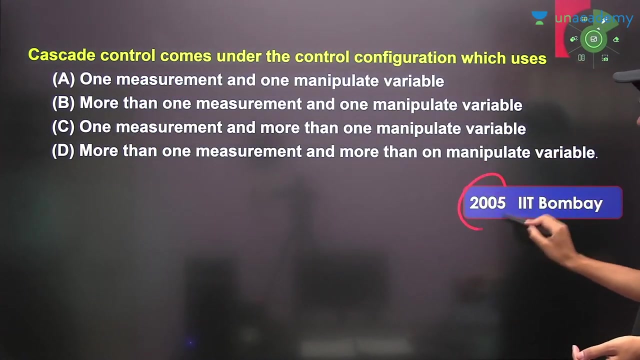 are you getting or not? so you will do it this way, this way done, sir. so this was clear, let's go. one question was asked in 2005. do it quickly. all in 2005 it was asked by IIT Mumbai. these were the 2-3 questions of cascade. 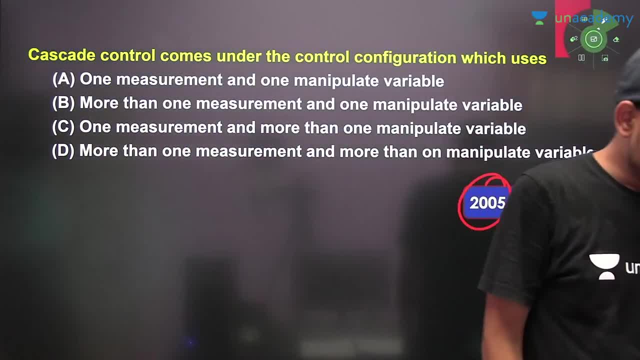 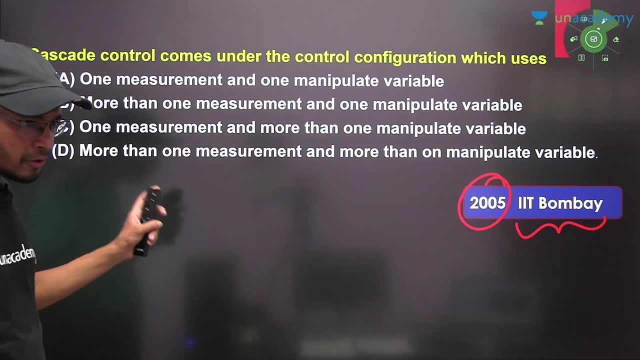 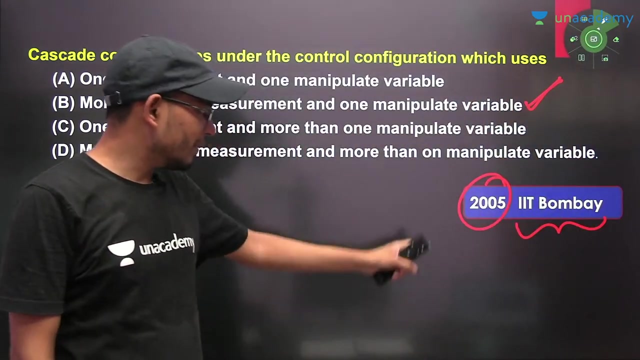 I am getting all of them done. all of you do this cascade control system. all of you will make this with love. see what is coming. more than one measurement, one manipulated B part will be coming. okay, B part will be coming in 2005. it is asked: in 2005. 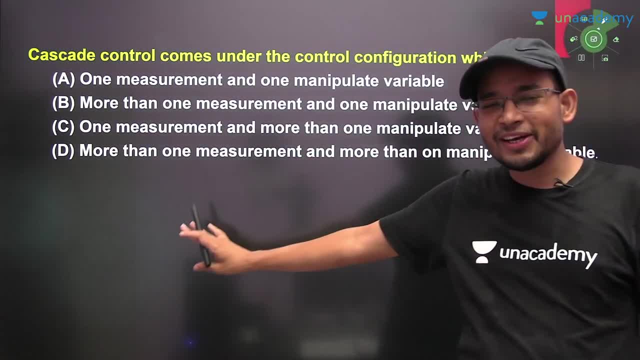 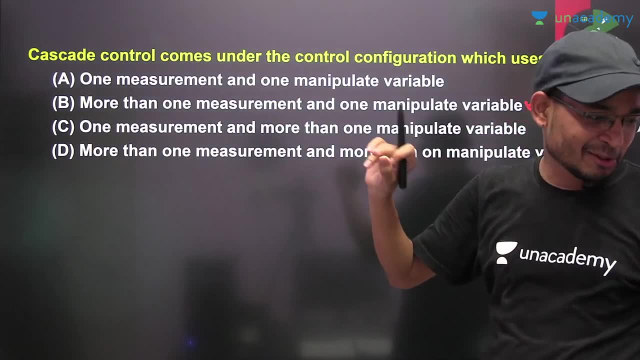 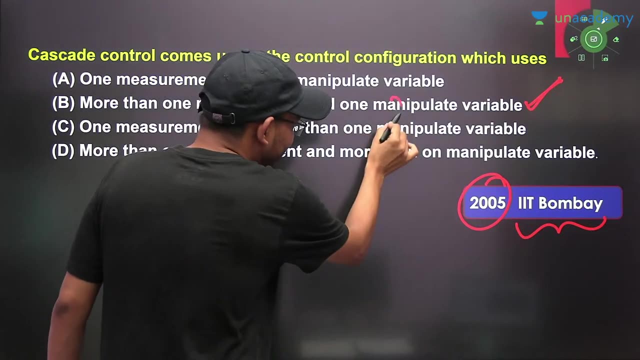 you know, incase theory is not clear to you, then this too, my friend had an answer. he knew nothing about theory, he had remembered PYQ. so he said: Manish, tell us how to remember this. we have to remember this. manipulated means A and what is written here. 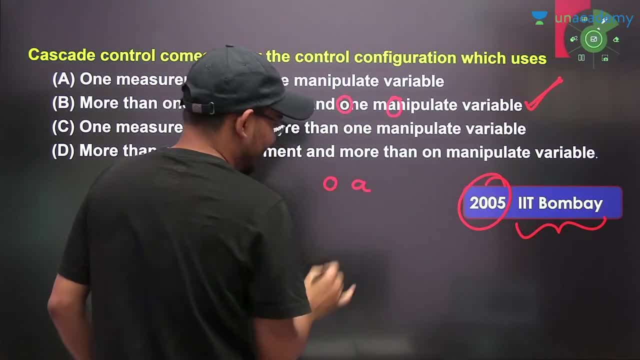 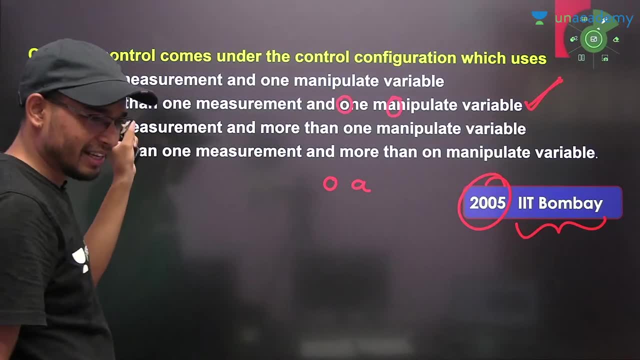 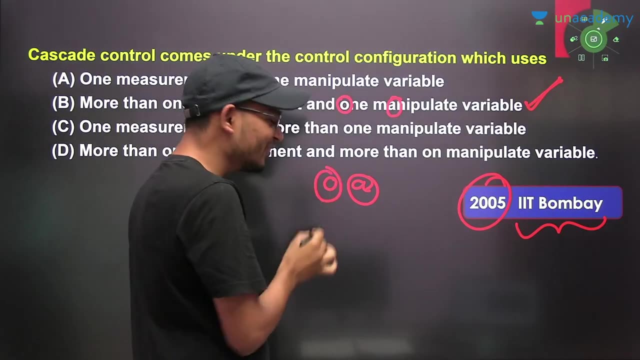 O, O and A are similar. O and A are similar, so A will be manipulated and E is two. it will be more than 1. what will be 1? Manipulated, because A comes in Manipulated and O comes in 1. so remember it like this. 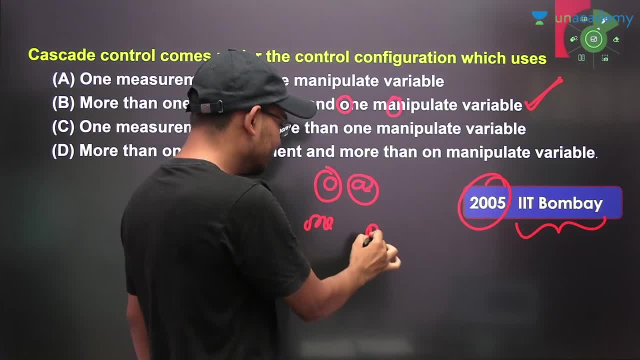 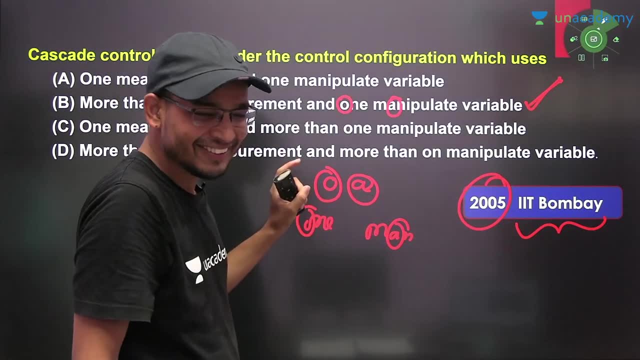 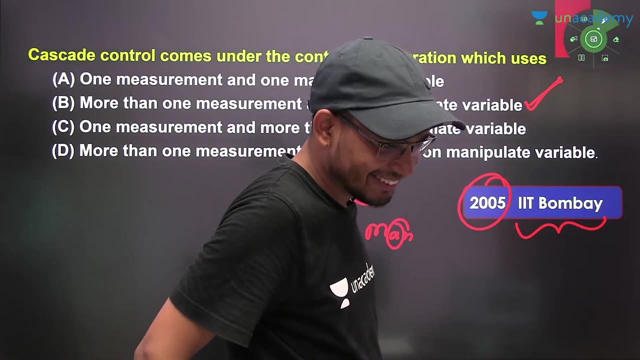 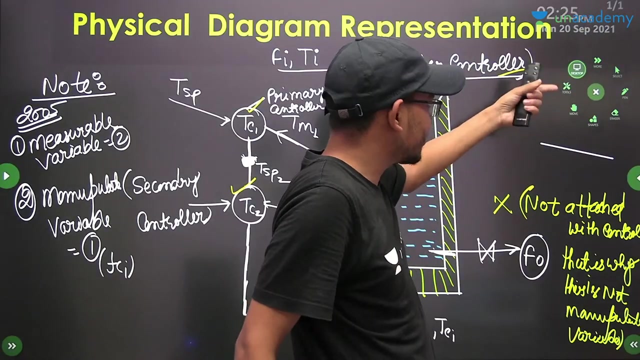 1 O N E, and it means Manipulated. so A is compared to O, so remember it like this. so remember it like this, so don't remember it. you have to understand. so in this way. if the concept is not clear, then only one compulsion is made. 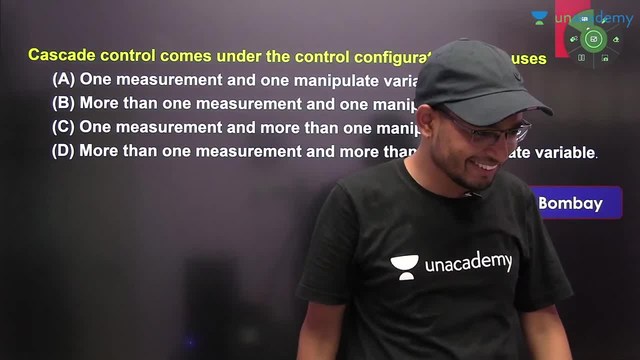 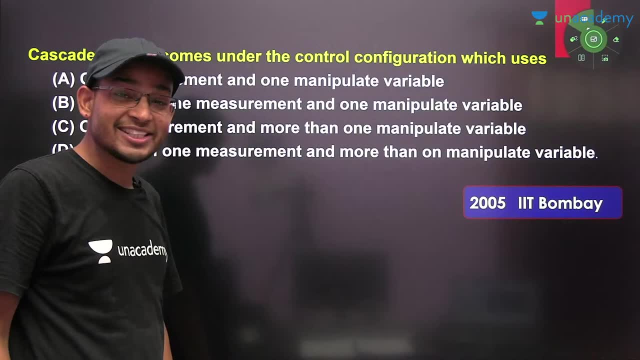 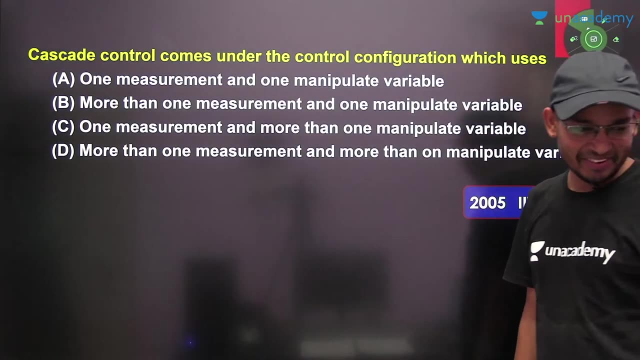 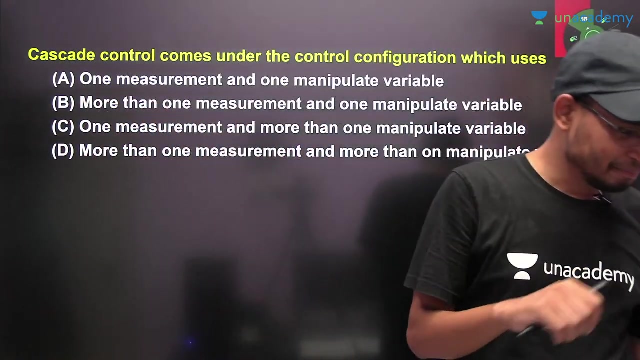 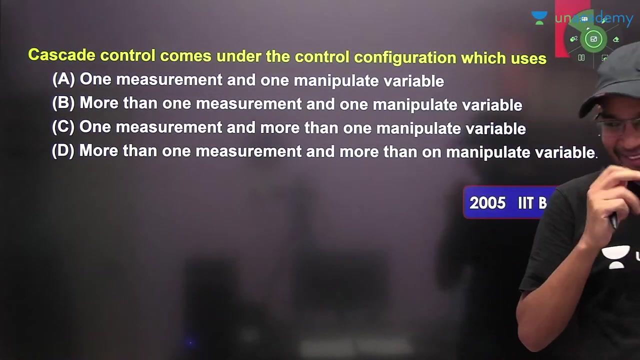 remember it, ok. he told me the concept amazing. ok, so don't remember it. you will understand the physical diagram and do it yourself. ok, if you understand the physical diagram, then you will do it easily. don't remember it, ok, because you don't know the physical diagram. 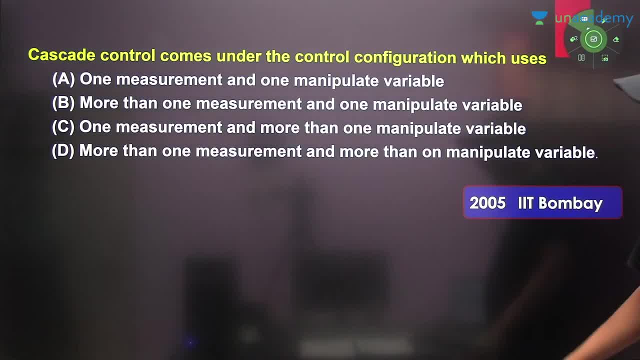 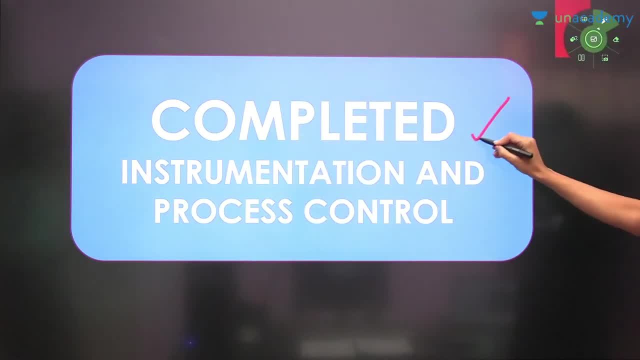 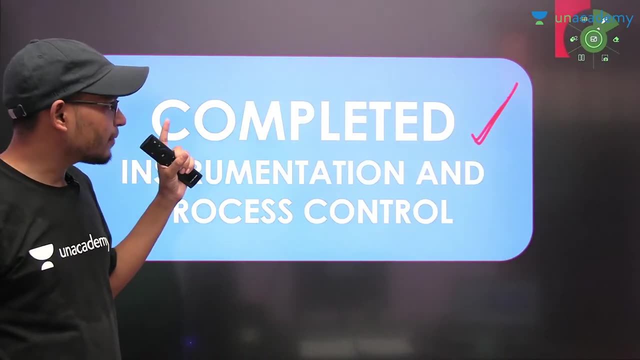 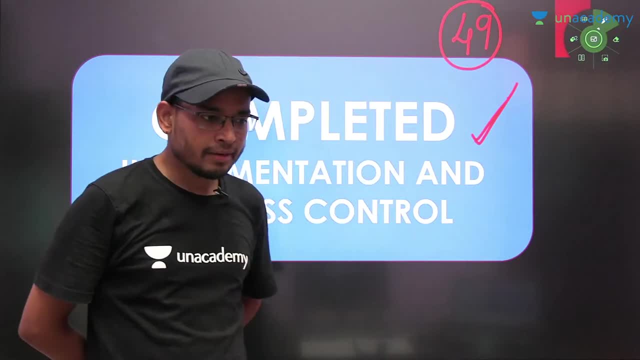 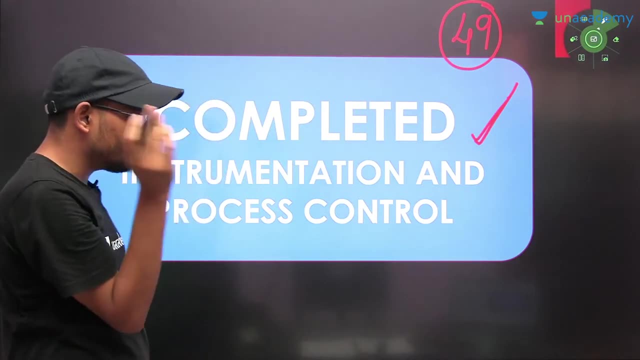 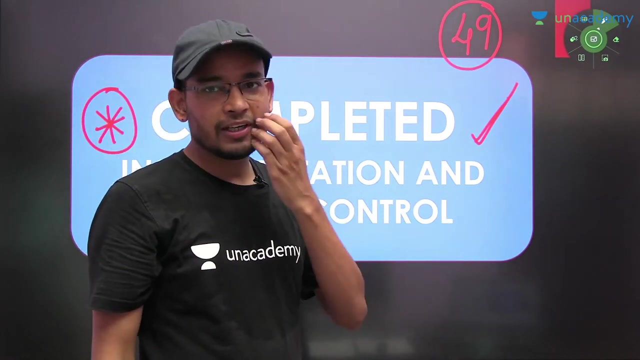 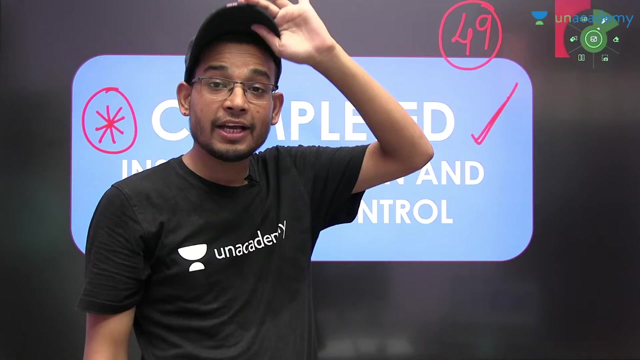 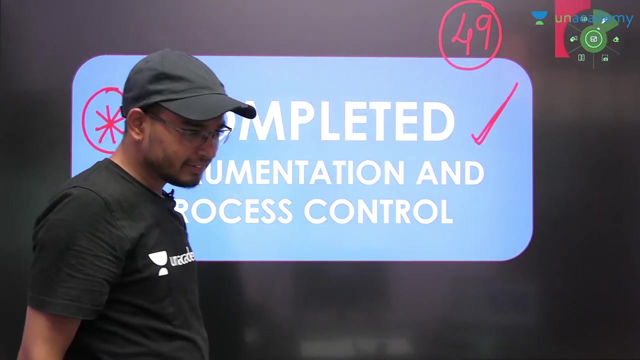 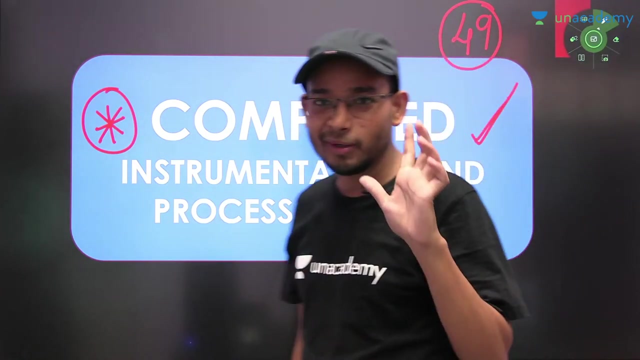 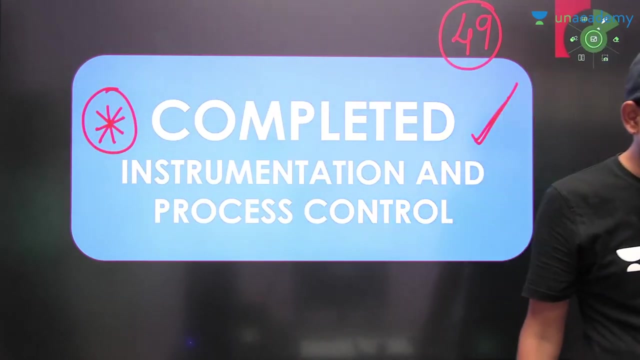 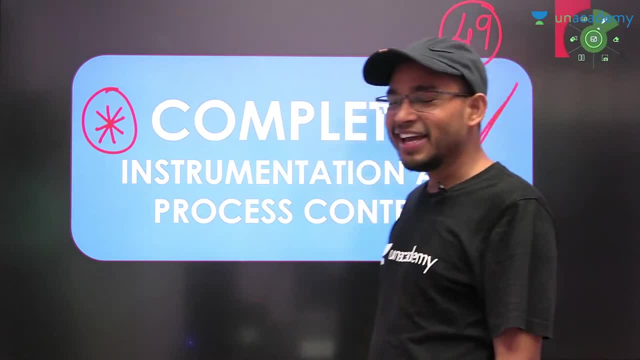 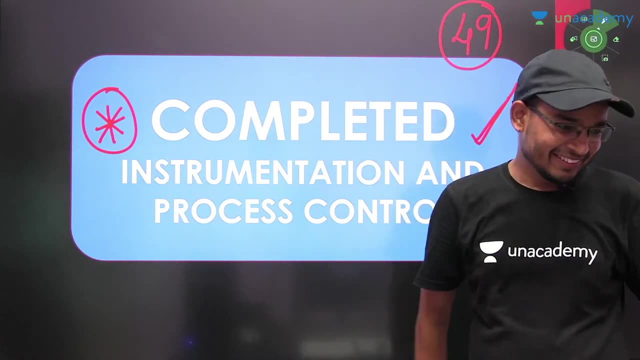 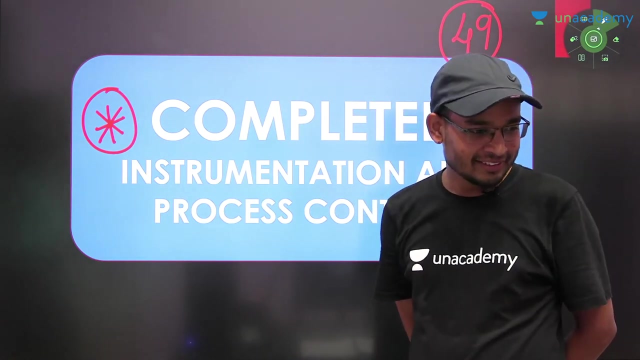 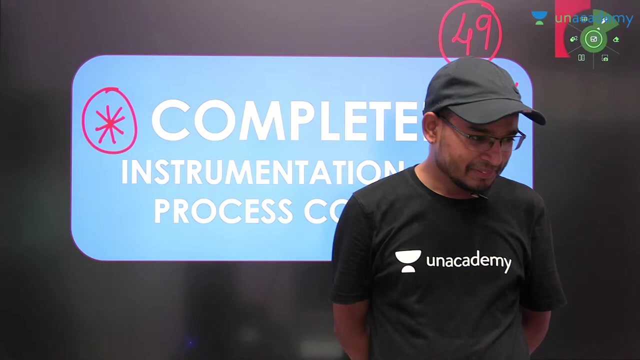 Yes, don't be scared, It is important, Otherwise you will be in a state like MI, Right, So this was your instrumentation and process control. Oh, this is Juhendra, Thank you, Enjoy, Enjoy. I have given you the whole playlist. 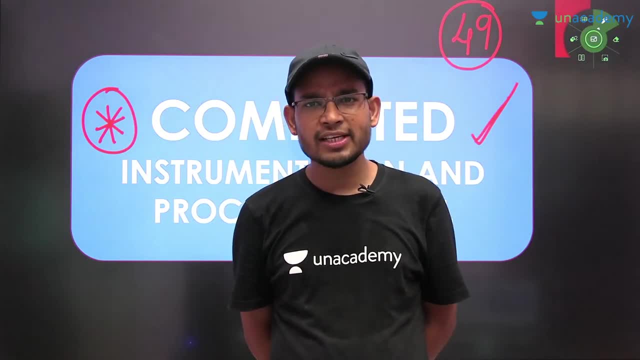 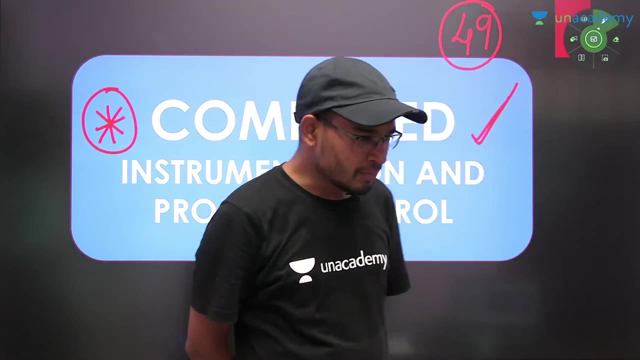 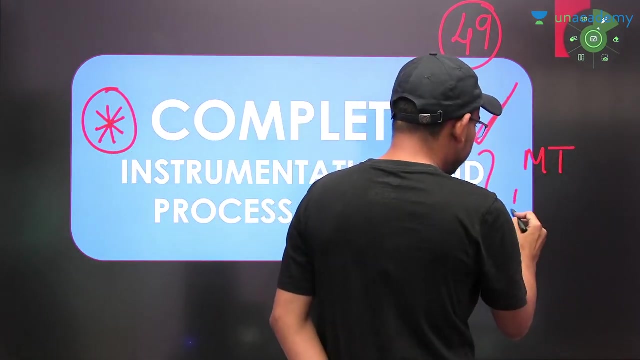 of all the sessions. It is a proper playlist. You can send it to your juniors, Those who also want to join. So I have completed two subjects in this way. Your MT- Both are big subjects, MT and IPC- Right, You have. 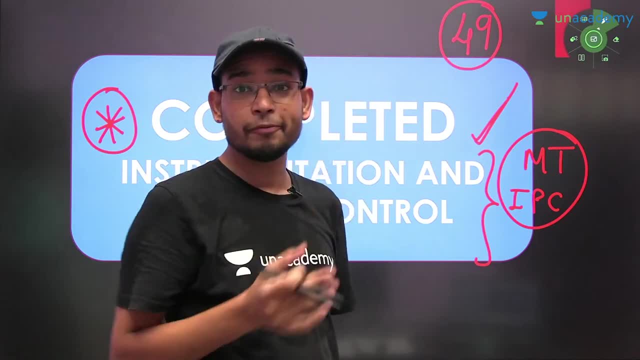 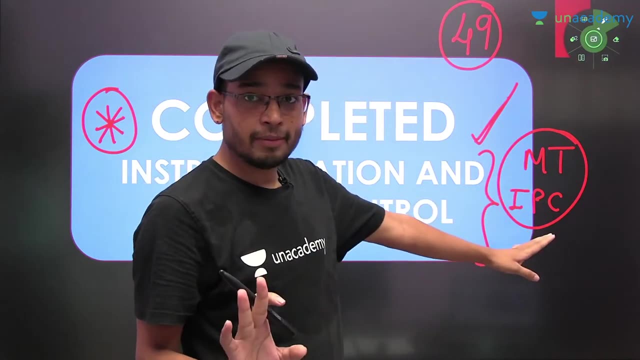 done them properly, In this proper way. I have also taken two lectures. I have taken 49 lectures on YouTube. There are many classes on special. I am telling you about theoretical. There are 54 or 56 lectures on MT. There are 49 here. 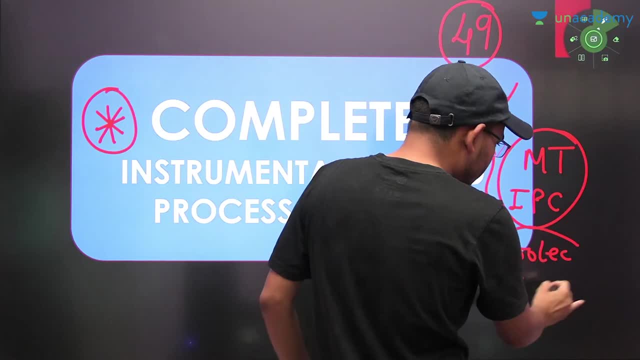 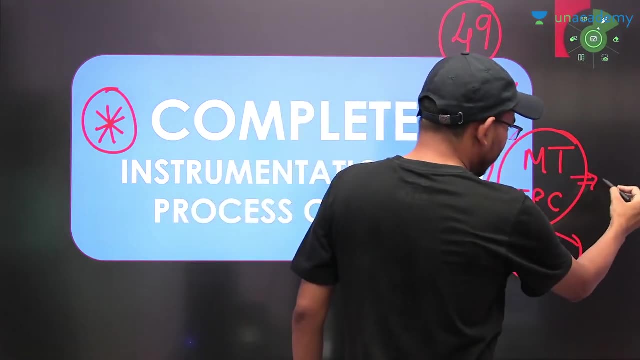 So you can see these 100 lectures- I have covered both in 100 lectures In YouTube- And see the numerical part on special Right And it will give you marks around to 23 to 25.. It will give you at least this number. 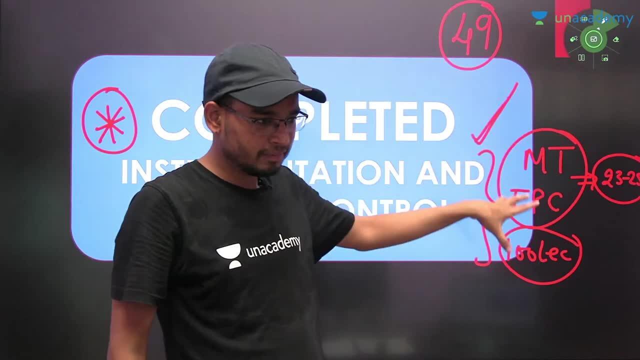 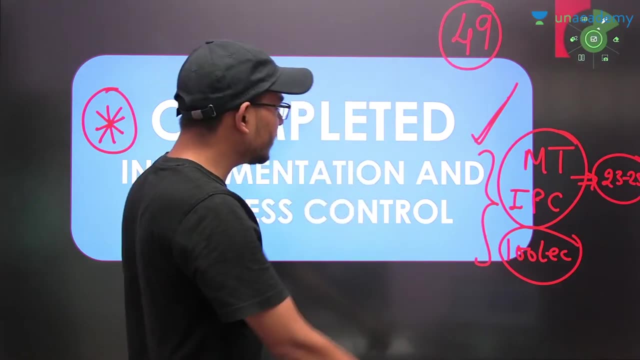 23 to 25.. These two subjects, In case you have done them properly, Right, I have also done 70 to 80% of your numericals in PYQ. I am telling you in the lecture: 70 to 80%. 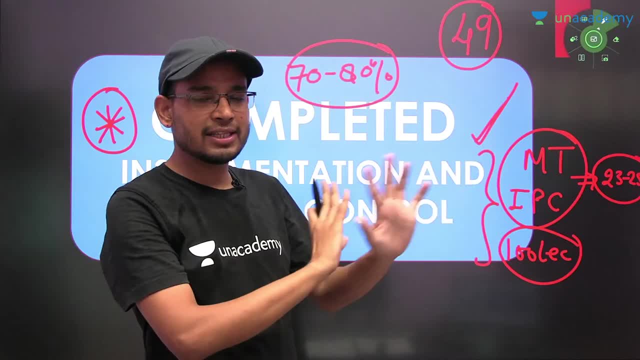 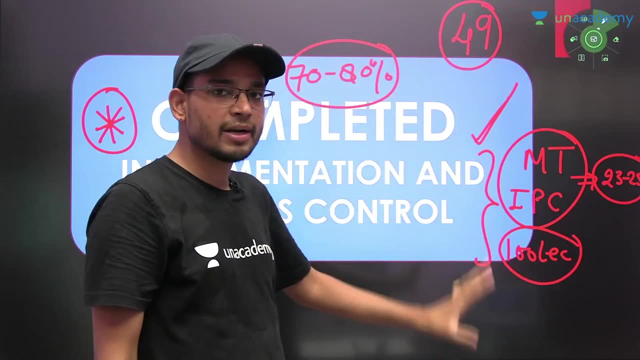 of your numericals have been done, Because if any topic is going on, then I do 3 to 4 numericals daily. Right, You must be watching. You will get numericals in every session. So 70 to 80% of your PYQ must have been completed. 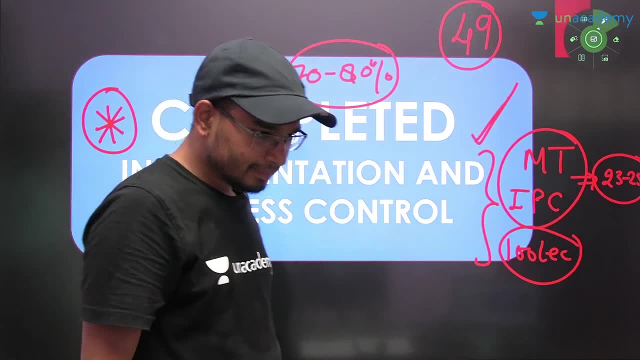 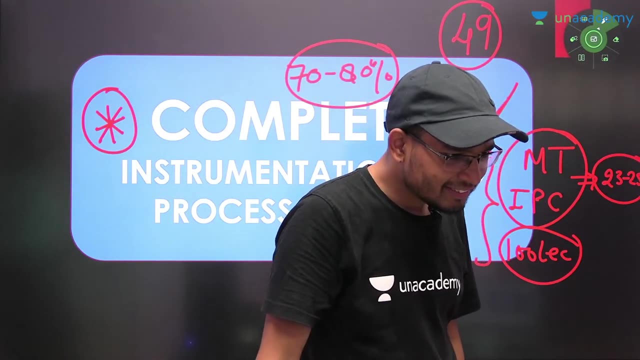 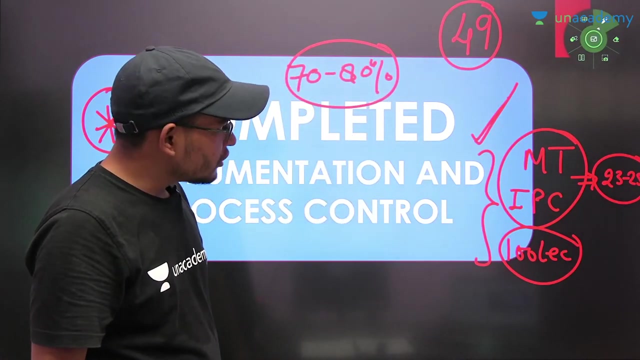 Right, Some PYQ will be left. We will finish it later. Yes, So this was your support. I cannot comment about solution THERBO because team discussion is going on, But, yes, I am bringing some of your sessions. 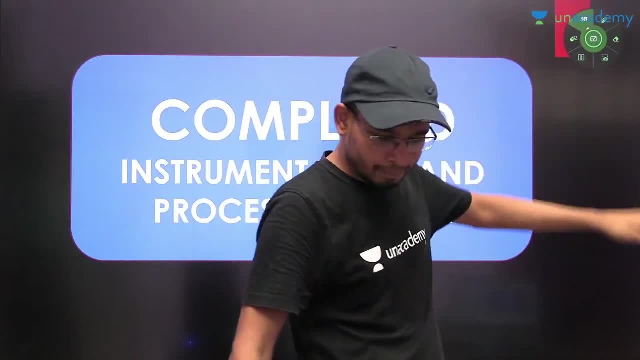 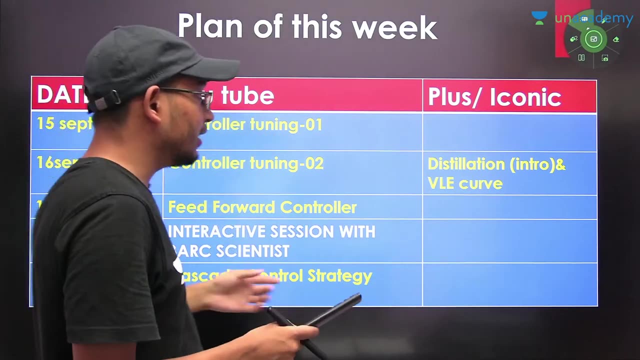 I am bringing some of the sessions. I will mention them later. I am bringing some sessions. I will mention them later. I told you that your cascade will be completed by 20th September. so today is 20th September and your reference. 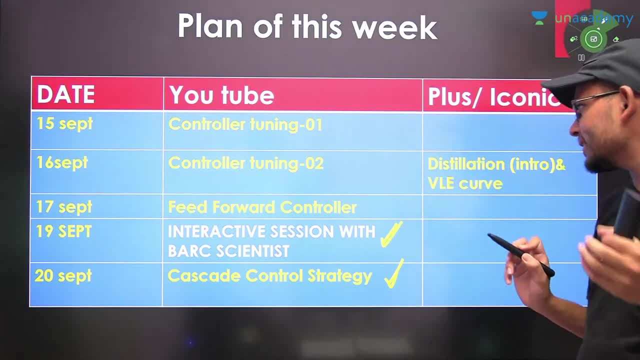 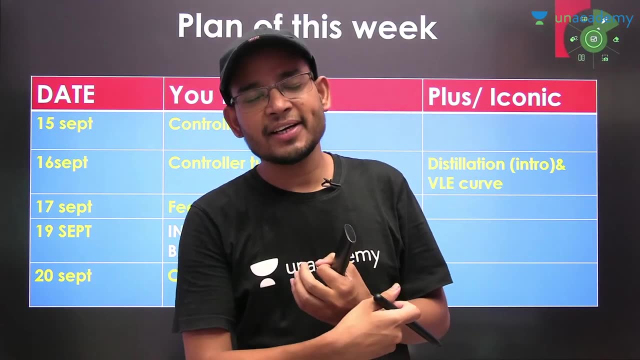 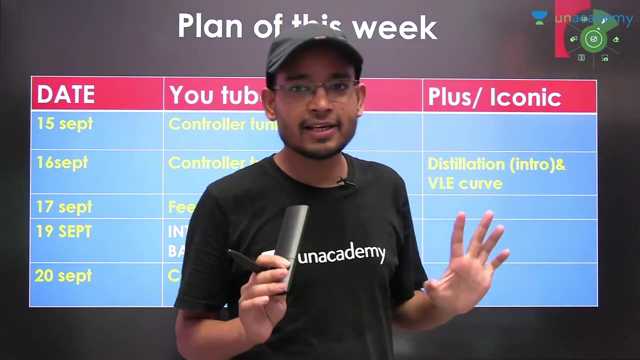 Yes, yesterday you had a session with Bark Scientist. now your session will be from tomorrow. tell everyone, Do you want to practice some good numericals in IPC? Tell everyone, Do you want to practice some numericals? I will keep the session from tomorrow. 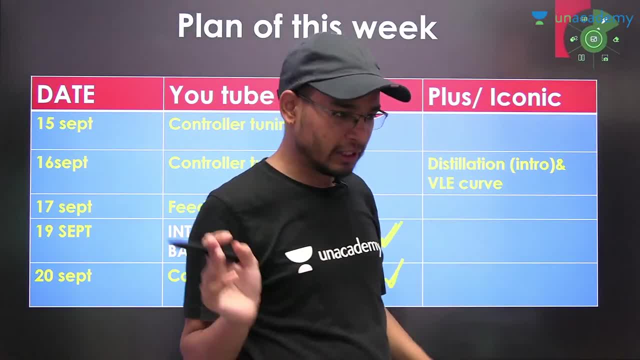 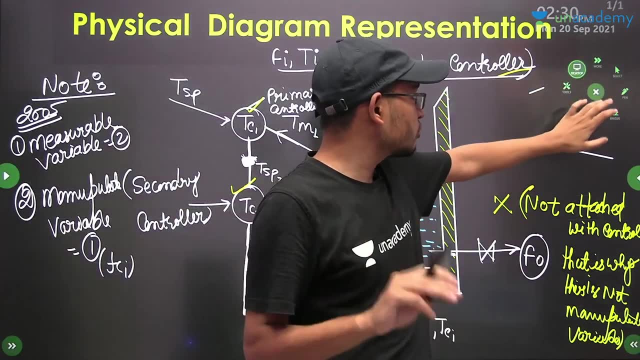 Not on YouTube, it will be on the app. our numericals are a bit fast on the app. Everyone will want it, but good numericals will be there. Numericals will not be good. it will not happen that you have done 50 questions in a session. it will not happen. 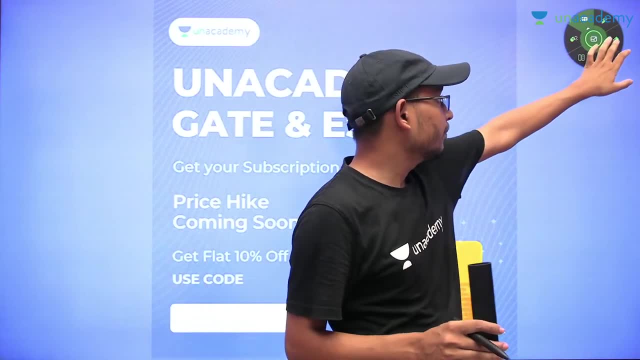 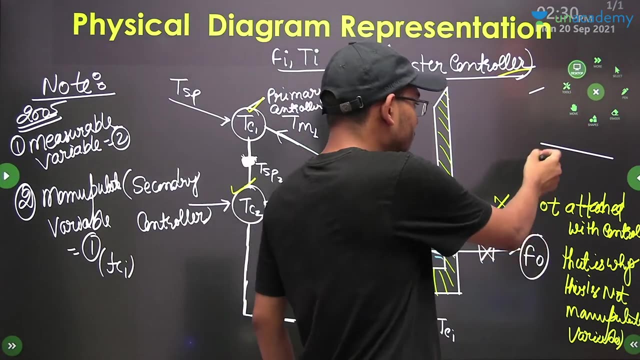 Numericals will be good for you, so I will just tell you here: Numericals will be good if you attend the whole numerical part, then you will learn a lot. This is the guarantee. you will learn a lot, so I will tell you here. 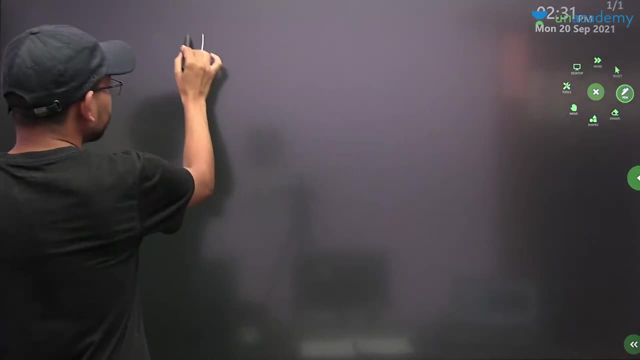 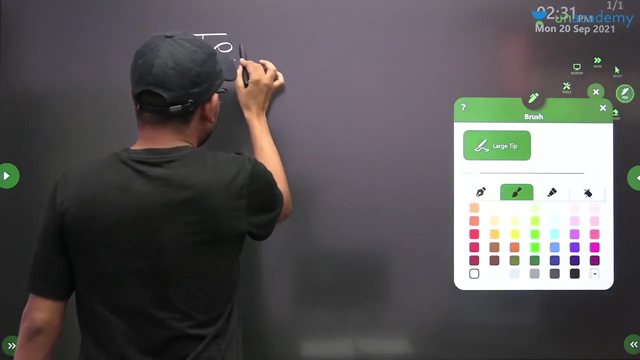 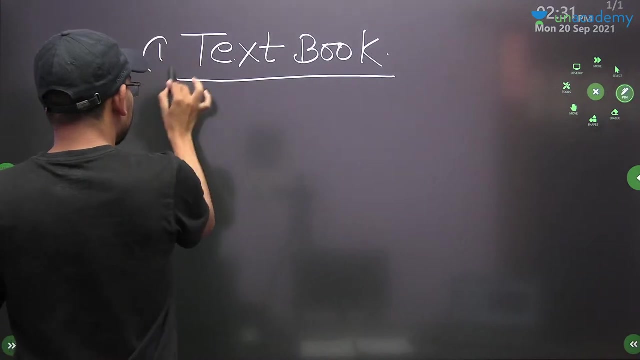 Yes, it is possible that you will also get numericals in your textbook. Okay, I will tell you from here. Right, so it can be your textbook. These can also be numericals of the textbook. Okay, plus number 2,. good questions will be given by your PYQ. 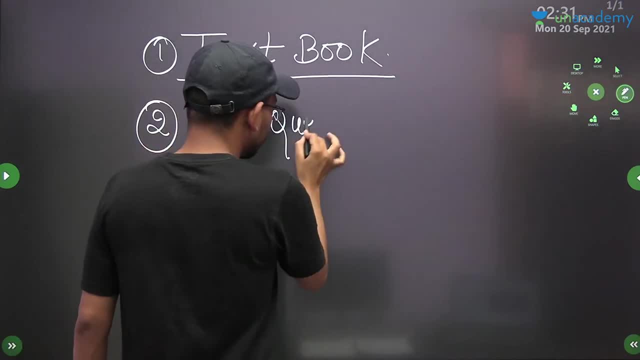 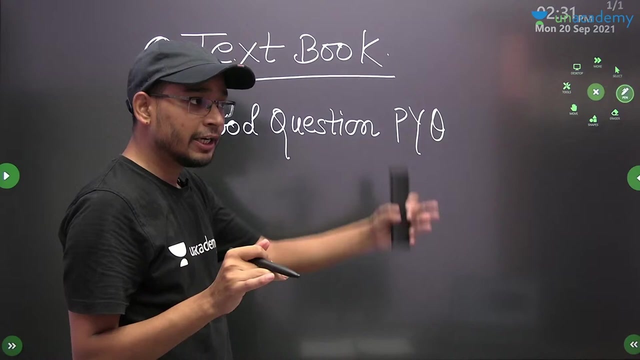 Good questions. Good questions will be given by your PYQ. Okay, whatever I feel that I have to do this PYQ, then I will do it. Third one: your questions will be from some of your internet resources Which have come in the literature. okay, 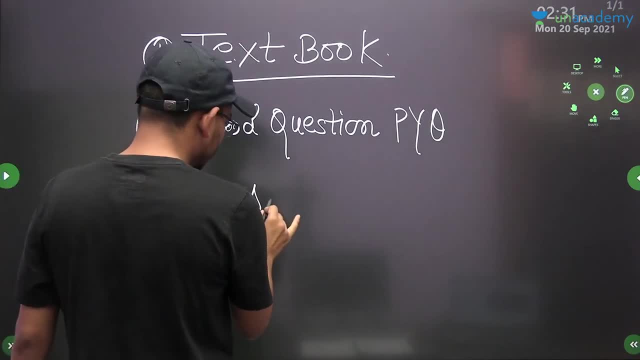 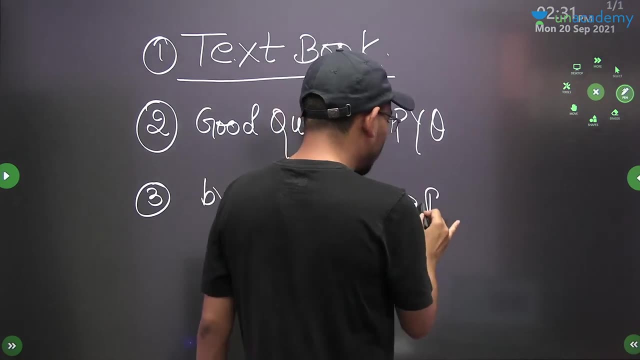 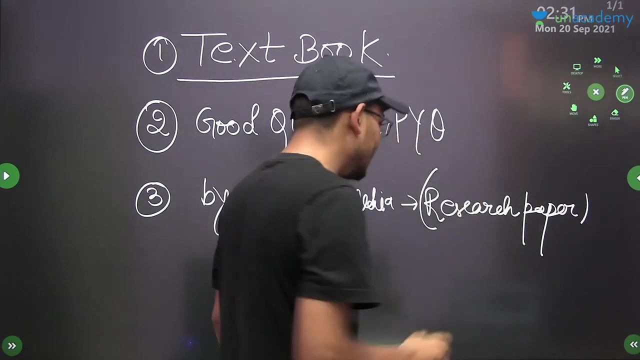 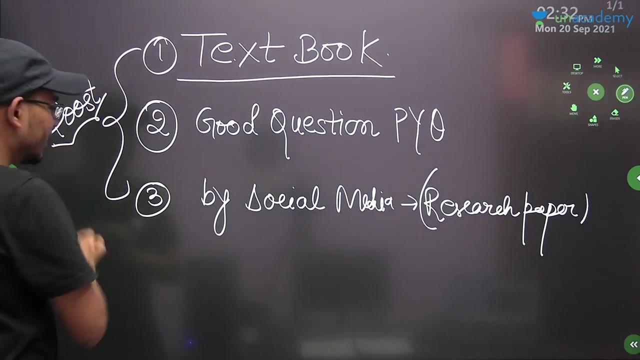 These will be yours. why social media? Okay, these are research papers. Research paper: Okay, you will get some questions from them, so you will automatically get boosted. Okay, These will be your boost up sessions, So you can boost yourself from here. this preparation, Okay. 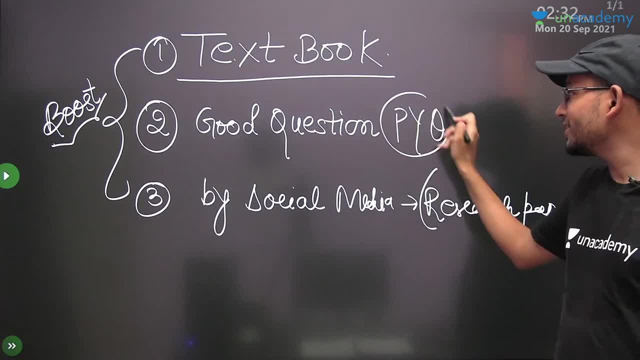 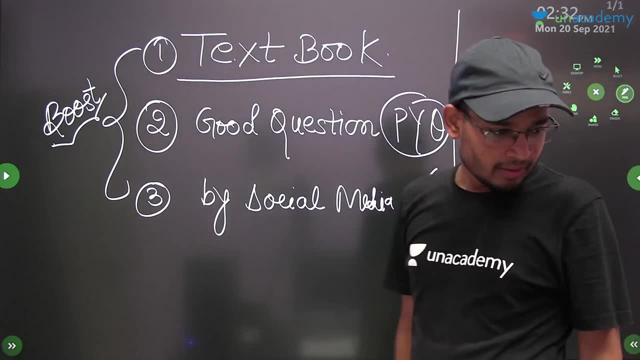 So I will take some questions from the research paper. I will take some good questions from your PYQ And some will be questions from your textbook. So if you want from tomorrow, I will start from tomorrow. say Yes, if you want PYQ, then I will start PYQ. 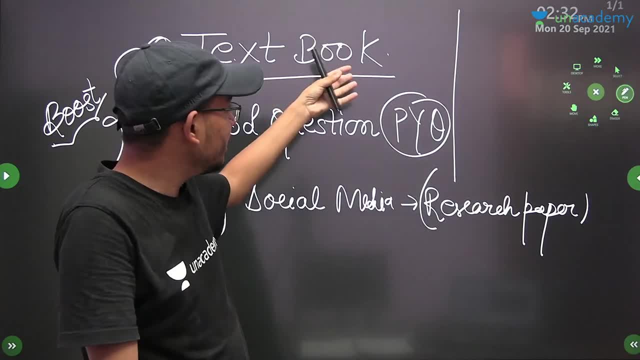 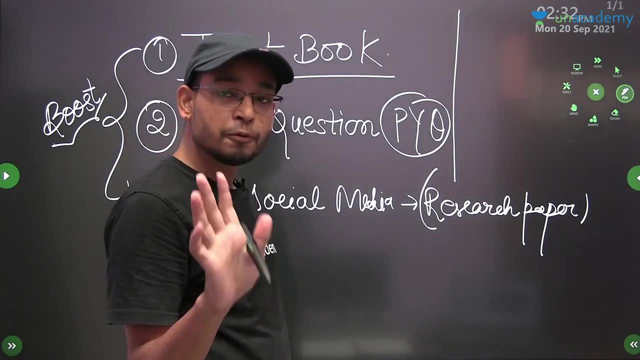 Whatever you say, In case, I think you will learn more quality than PYQ in this. If you want to learn, then other than PYQ, you will ask more questions. Yes, the timing of tomorrow. there will be no classes on YouTube tomorrow. There will be no classes on YouTube tomorrow. 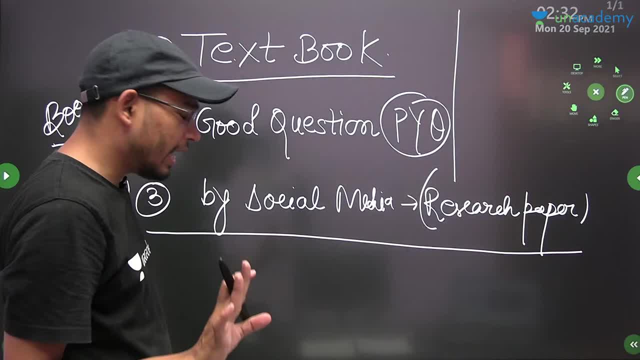 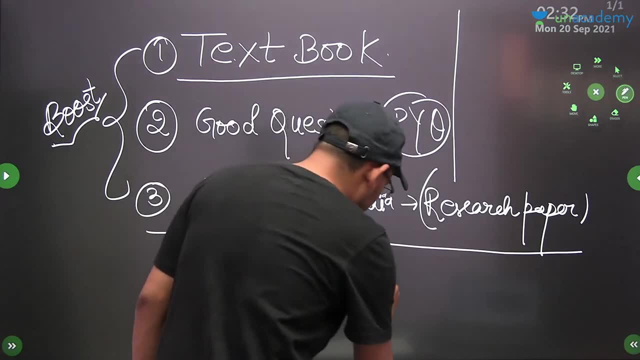 Let's make a gap of one or two days. Okay, there is IPC, you can revise it easily. Tomorrow you will have class on special. Tomorrow you will have class on special app. Okay, on Unacademy special app. Right, It will be on Unacademy special app. 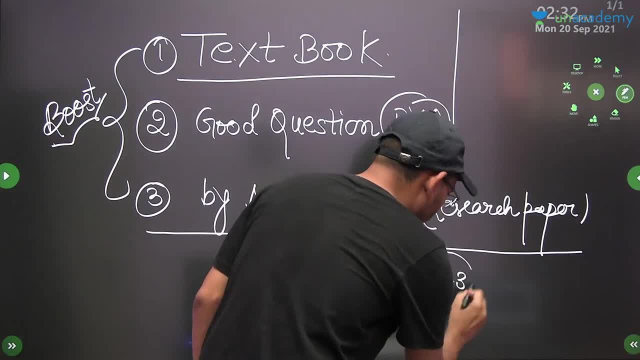 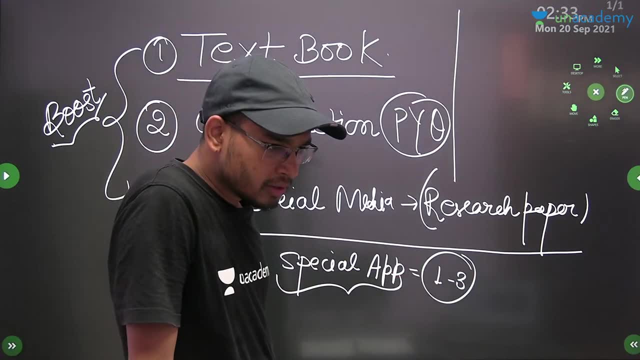 And I will put the timing of this 1 to 3, Two hours. Okay, I will put the timing of two hours. You will hardly finish it in one and a half to two hours. Yes, sir, practice questions are required. we will do PYQ. 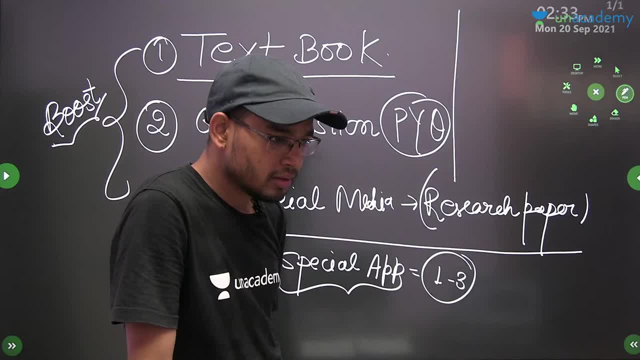 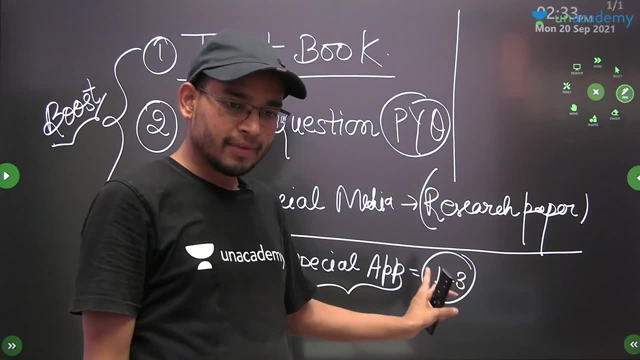 Yes, I will do PYQ Right. So this will be one to two sessions In this. yes, the BARC will also be covered. Rajat, In this you will do IPC also comes in BARC And this will be the complete syllabus. 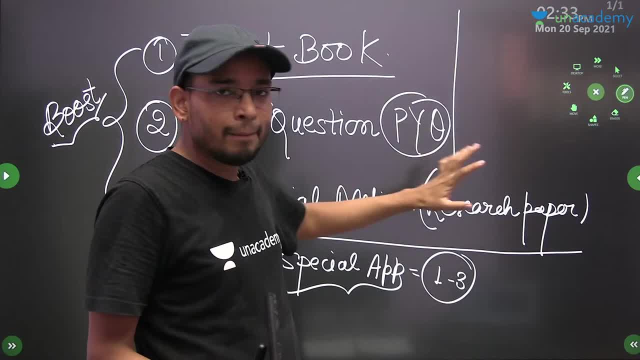 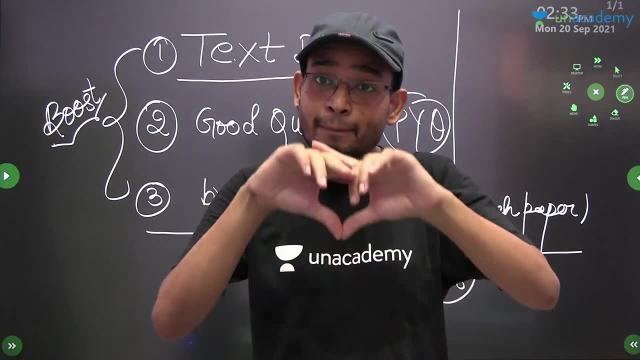 First of all, listen carefully. This will be your complete. One question will be done by you in the second order. One question will be done by the controller. One will be done by your frequency response analysis. Okay, when your syllabus will be complete, it will be fun. 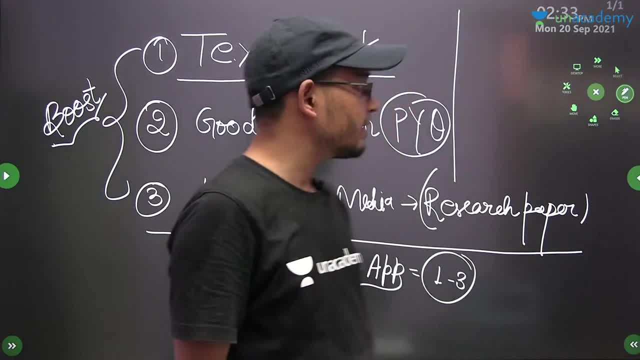 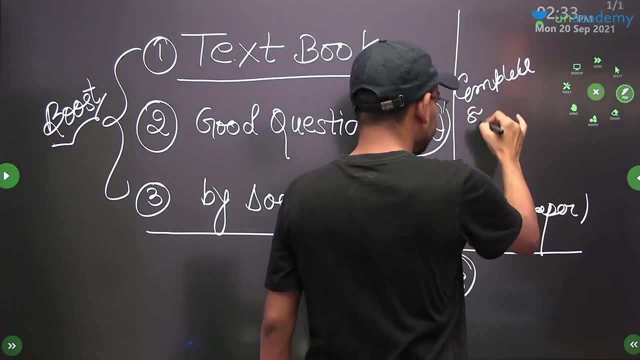 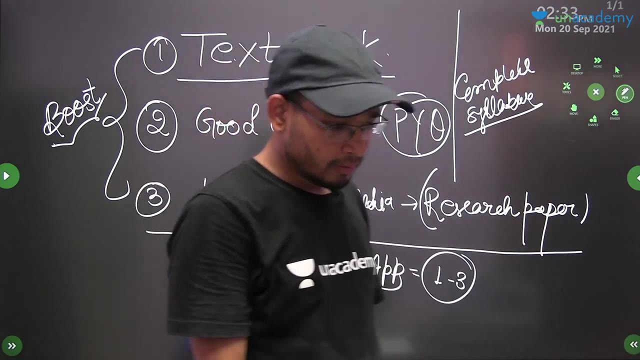 Now it will not work topic-wise. This will be done by your complete syllabus. Okay, You have now completed. Okay, it will be done by the complete syllabus. Okay, I will cover this with the complete syllabus, Okay, Okay, So in this, your BARC and NRL- both parts will be covered. 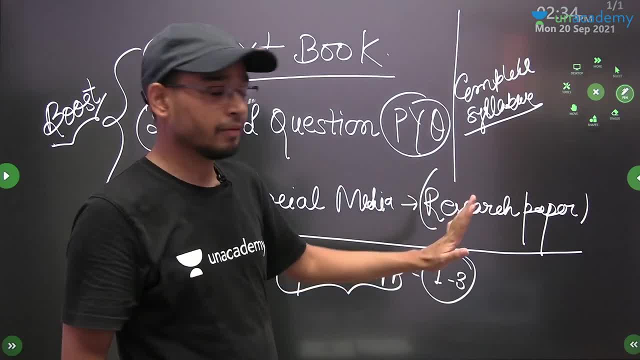 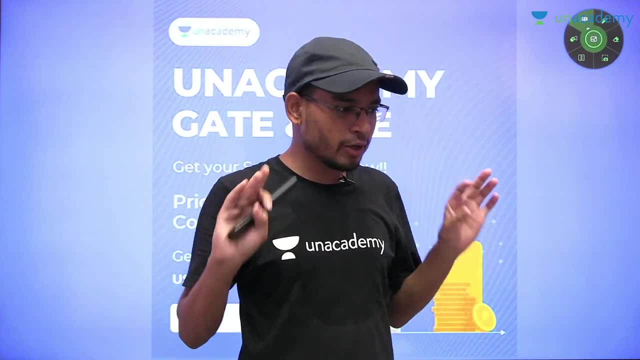 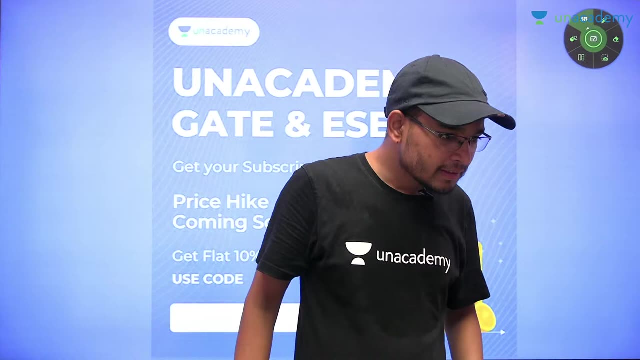 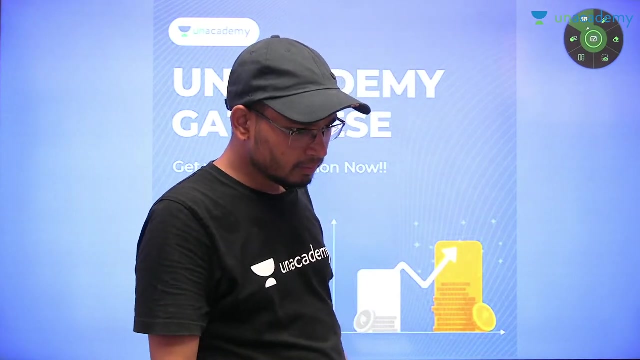 Okay, You will do one question. you will solve ten questions in BARC, Right? So this will be your upper class from tomorrow. From tomorrow on which Upper class? Fine, Okay, Vivek. Also in the summer, I will be going to revise the concepts, Okay. 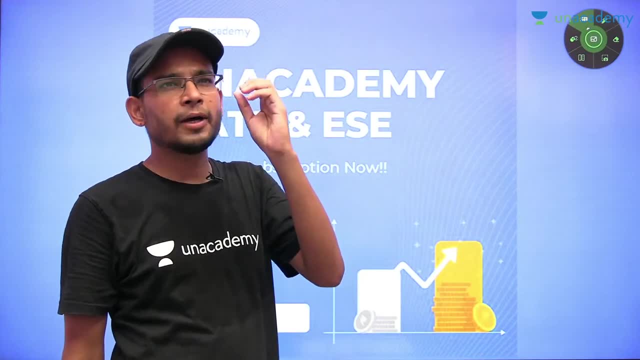 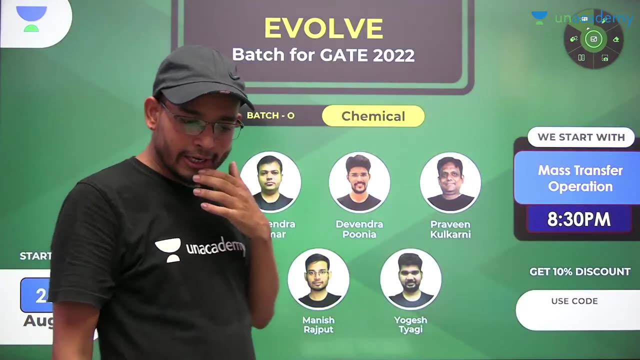 Yes, Vivek, I will do it from 1st October. I plan for it. From 1st October, you will get sessions for the interview, Alright. So yes, Oh, yes. And one more important thing: Those people who have to move with the mass transfer. 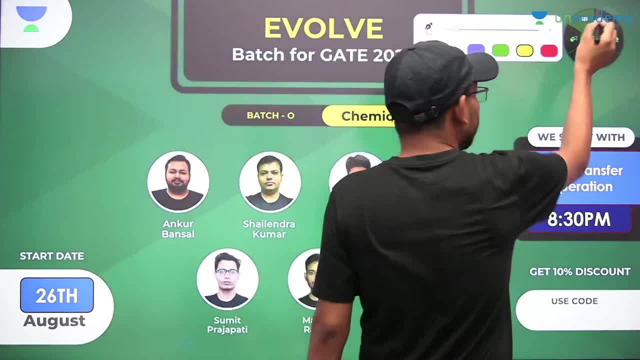 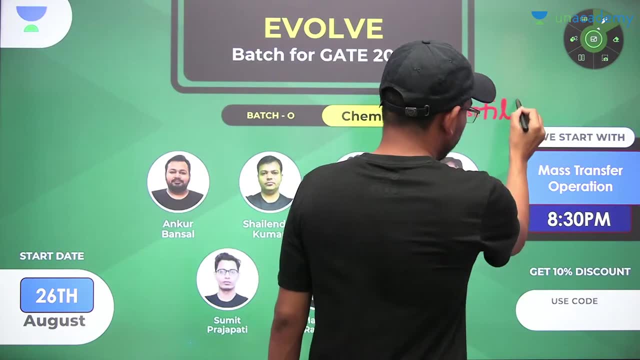 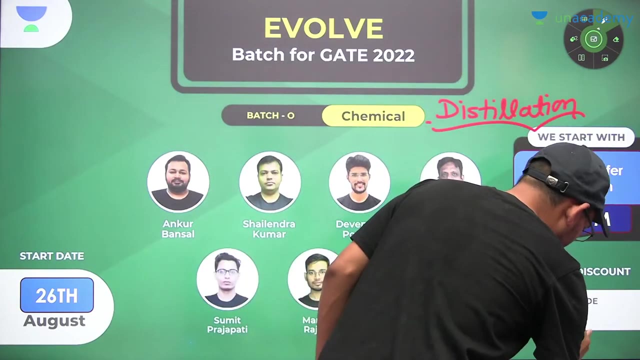 They can also move with the mass transfer. Those people who are interested Now. your distillation has started. the distillation has started here. the distillation has started so they can move properly and the timing of this is 730 pm. you have to use the code. 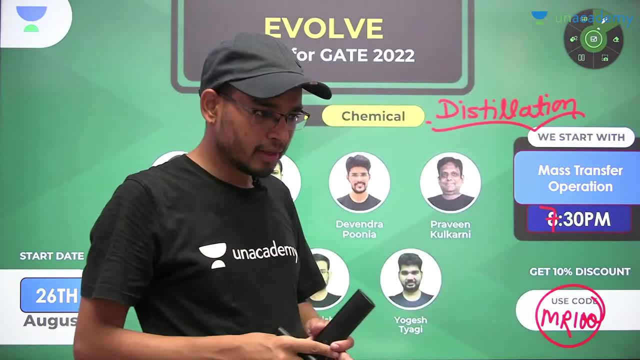 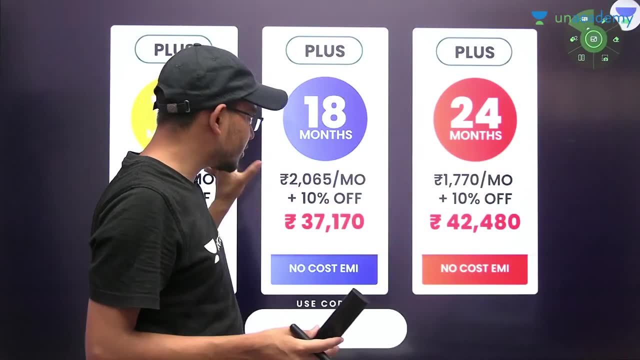 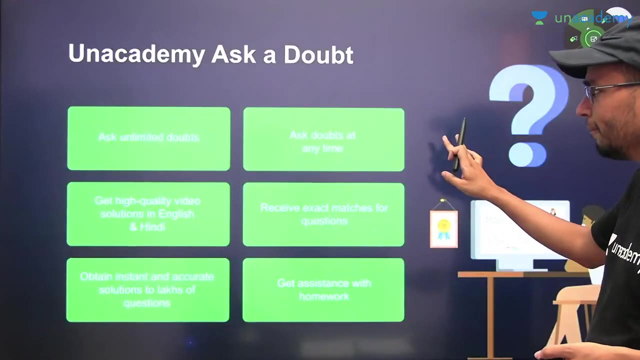 MR100, you can use the code MR100, you can move properly with this code. ok, after this I will talk. in case you have to move with 12 months, 18 months, 24 months, then this structure, you can move with this, this for iconic and ask any doubt. this is your live. 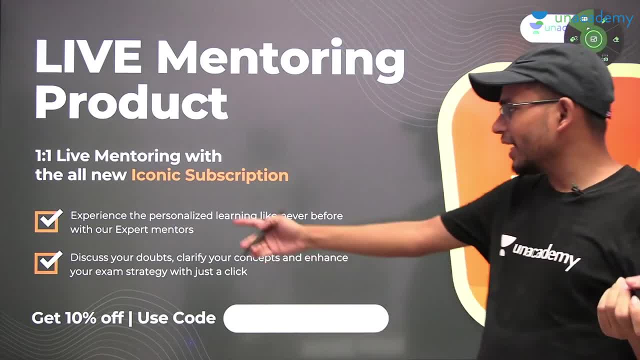 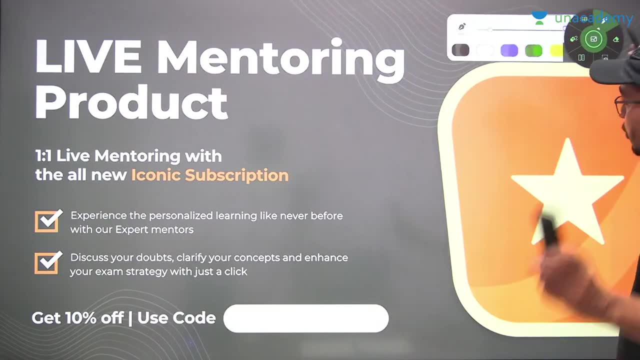 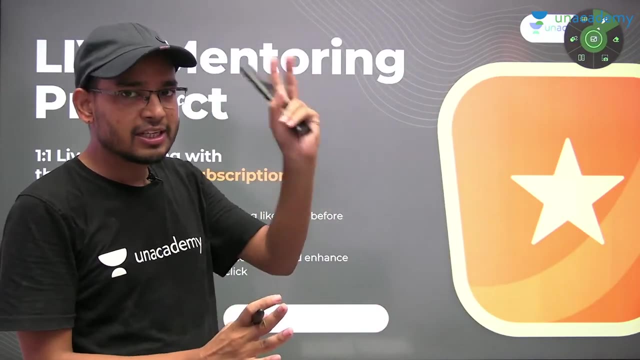 monitoring product. you guys take iconic subscription, so it will be properlyral to clear doubts here, correct And byvening your proper way, you will enjoy this part. yes, take the course and move. in case of you have to 200まで steps with us, you have to follow the strategy of us. 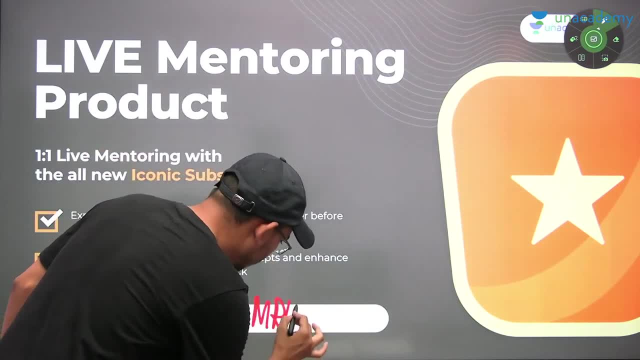 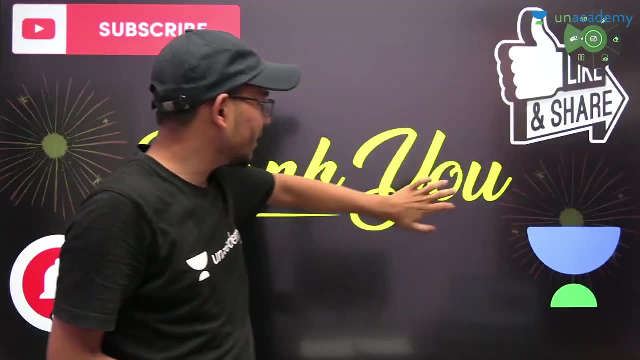 and have to take your journey properly with us. then you have to use the code MRHUND with the purpose of 200 Rogue 2019: medicines. bro, people can go ahead Right. Come on, After this, I will just talk, So. 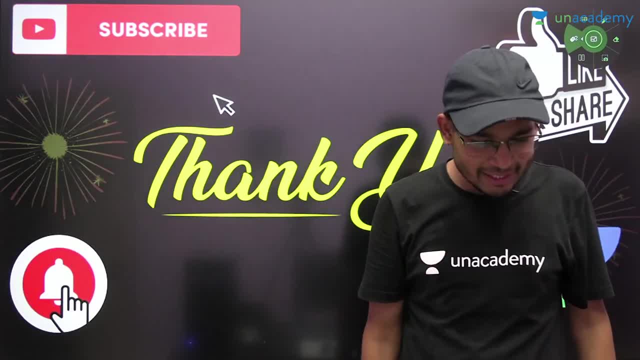 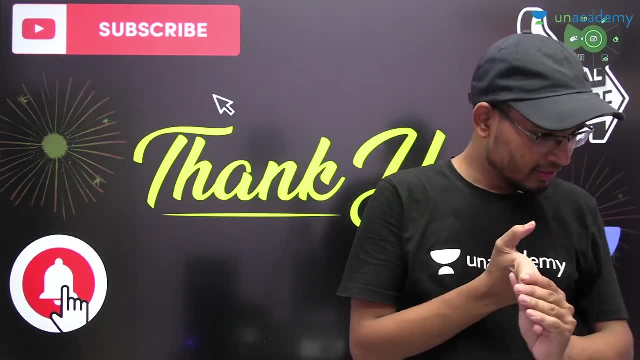 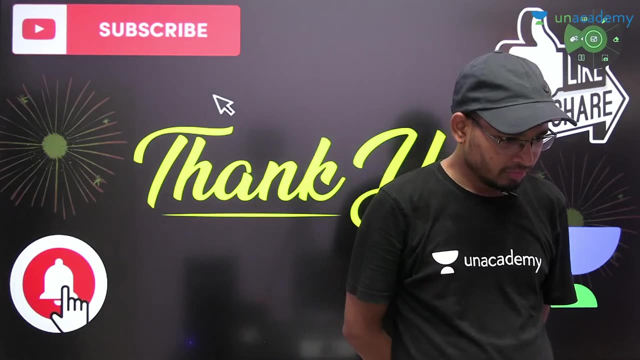 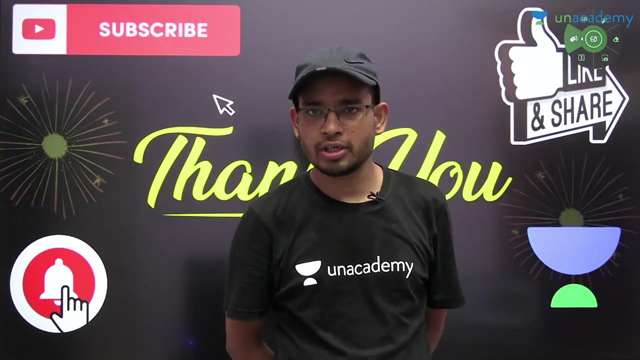 then let's end our session here. Hope so. you guys must have enjoyed it. Thank you everyone. Yes, Yes, doubt you go and ask any doubt. Ask any doubt. you can go there and you can ask. Okay, but it is for the subscribed students.